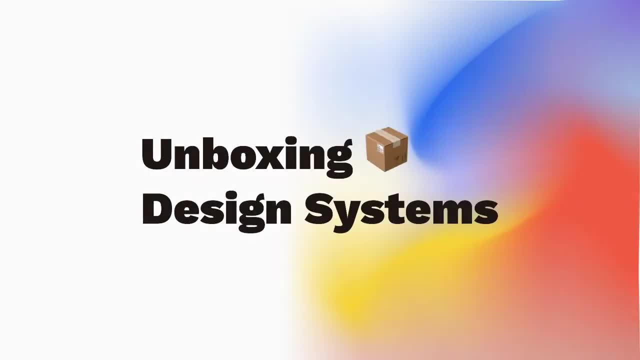 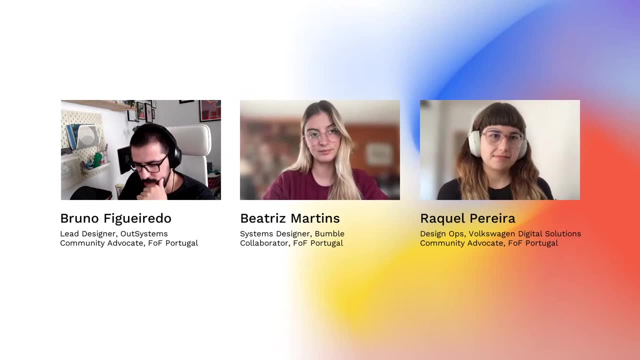 And I think we're live. Hello everyone, welcome to yet another live stream of the unboxing design system here from the Friends of Figma Portugal. I'm gonna start by already answering the last comment that says, hey, is this going to be in English only? Yes, 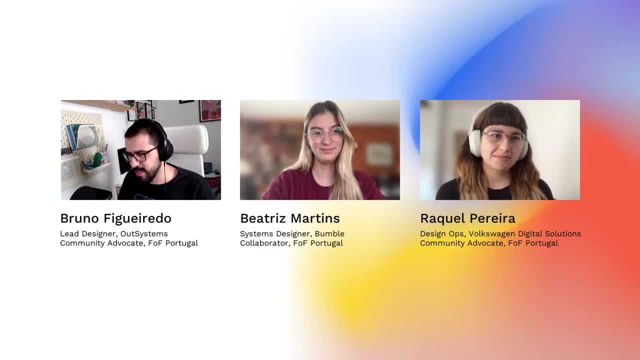 this is a. although we are Portuguese, we tend to do these in English so that most people can understand. so here you go, And yeah, so today the stream is gonna be three people again. We've been always rotating a little bit who's here for each episode and this: 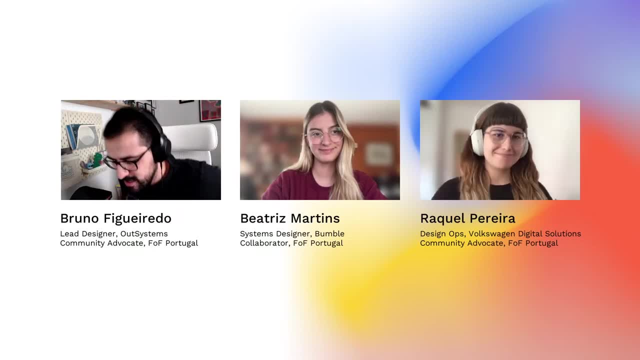 time we have, as always, Raquel, and today we have Beatriz. that has just joined our team, and maybe present yourself, Beatriz, a little bit. Sure, so I'm a systems designer at Bumble. Right now. we're doing a lot of stuff with the design system. of course, We have a multi-brand. 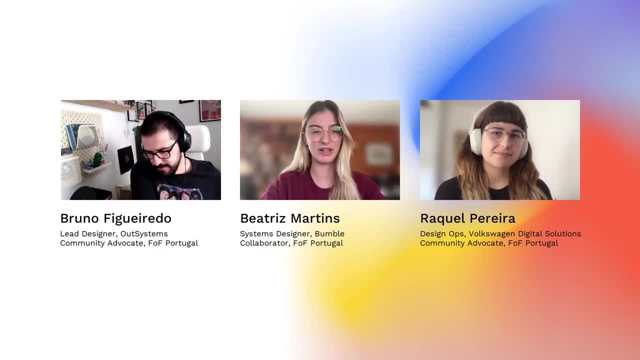 design system. so we're kind of working around with tokens, the variables at Figma, which it's given us a little bit of headaches, But I guess we're going there Little by little. of course there's a few things that 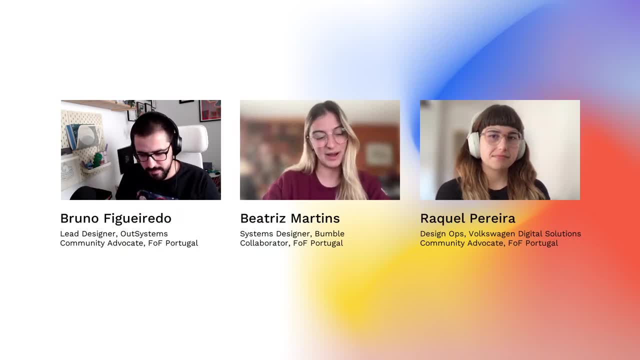 we didn't, like did yet, but we hope to do in the future. So yeah, basically we're trying to implement all of the releases that Figma did and we're really excited to do more stuff with that And I hope in the future we can actually deliver all of the things that we're 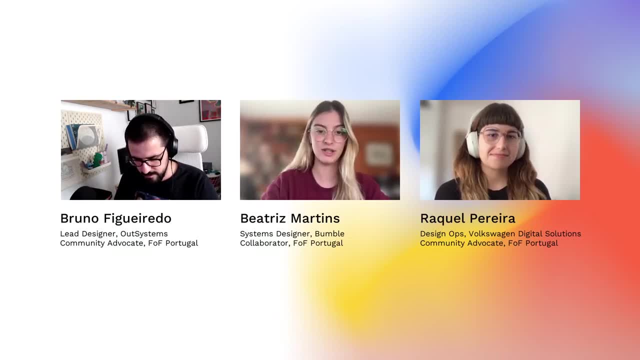 doing to the community, and just so you are able to see what we've done, and maybe an unboxing of Bumble's design system, who knows? ah, that could be interesting. I hope I don't participate in that one. cool, okay. so before we start digging in, I just drop. 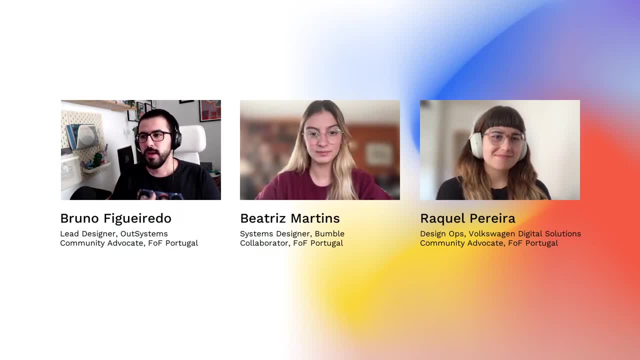 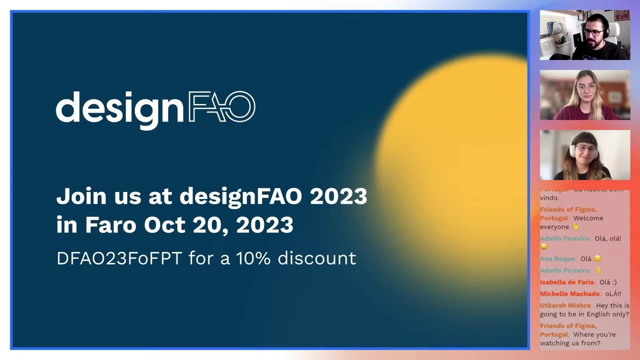 a question on the chat. we would love to know where you guys are watching us from. but first time for some of the housecleaning moments, and let's just start with our regular promos, letting everyone know that you guys should definitely join the list of attendees of design FAO, our partner conference. it's 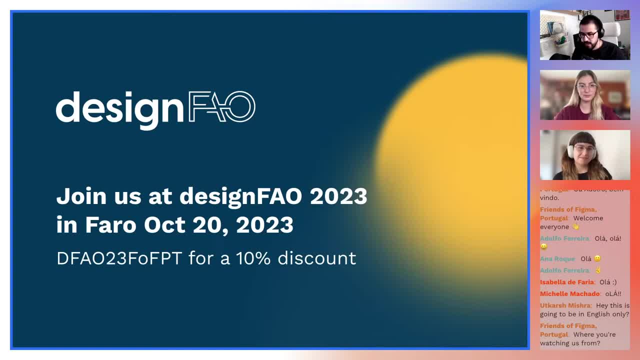 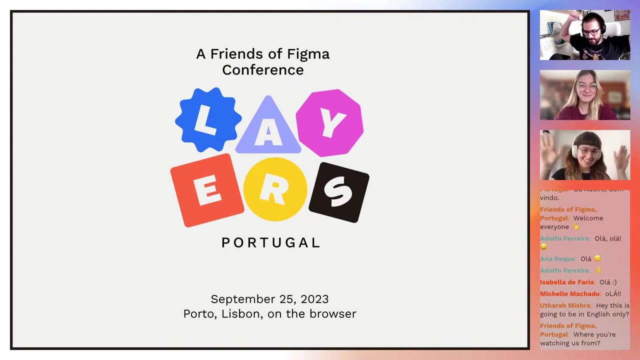 happening on October. it's a really interesting conference. it has amazing speakers. we would love to meet you guys there. and drumrolls, please you. and today I don't have music, so it's going to be a little bit like we have a conference, we have a conference and from friends of Figma Portugal, we're going to. 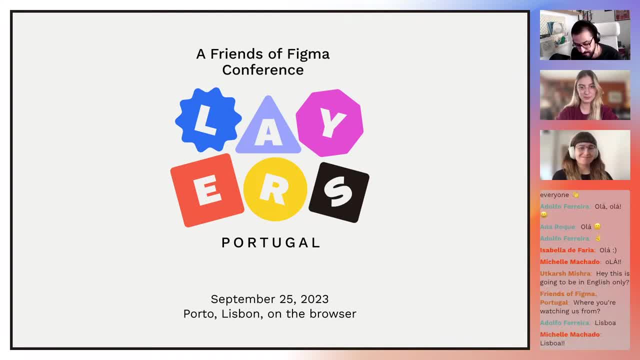 have a small conference one day, on September 25, and it's going to be actually a hybrid conference. we're going to have two locations, Porto and Lisbon, but we're also going to stream part of the content online so that everyone has access to the conference information. more news will be shared soon, but I'll 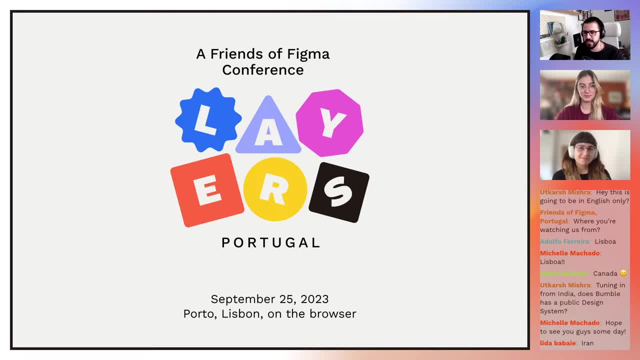 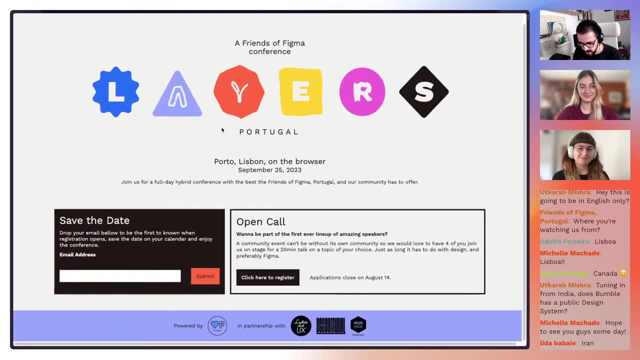 try to get the link to the conference so that you guys can get it. but yeah, you can. let me just also share the screen with the browser. right now we already have a website live. we're basically gonna open the doors for you guys to save the date and we'll be. 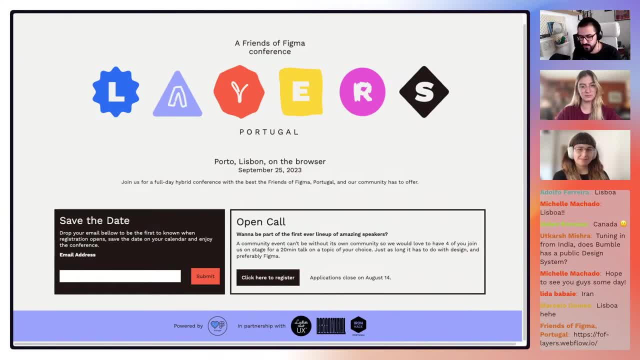 opening an, a call for speakers up until August 14th for people who can join us in Porto or Lisbon. um, community members will be waiting for you guys. uh, yeah, and that's it, and don't judge us, but the website will suffer updates because I was literally doing last minute edits, so 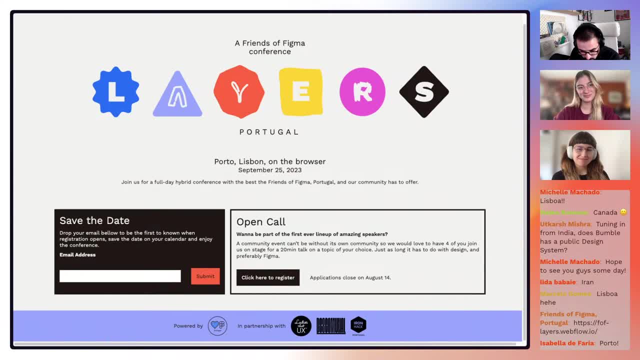 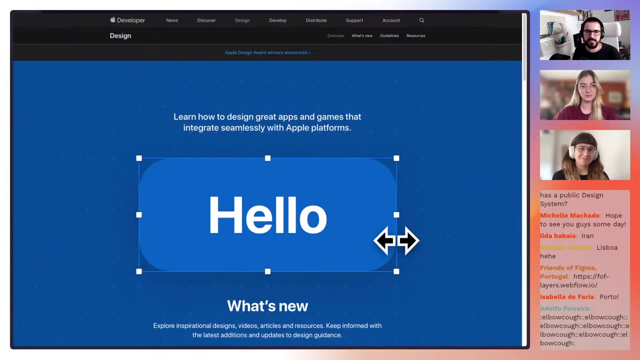 um, on top of that, uh, hi to everyone attending from India, Lisbon, Canada and Porto, apparently, and Iran. so, yeah, we have people from all around the globe right now. um, okay, and let's get to what we're actually talking about today, and that would be the Apple design files that I'm hoping that you guys 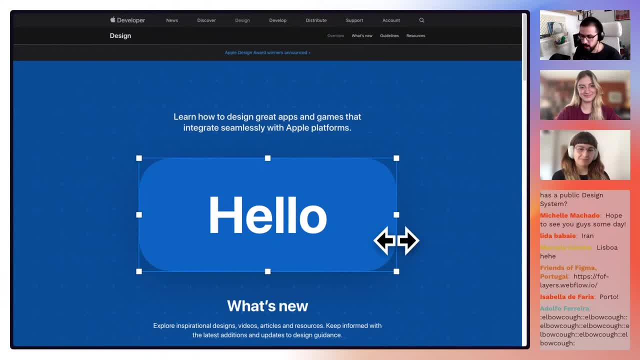 have already started looking at um and, on a side note, I love how the emojis on our chat right now are literally- yeah, I was just thinking about it while they were listening, but these are really, really fun to watch. on the left, the emojis, and then on the right, hello cough. 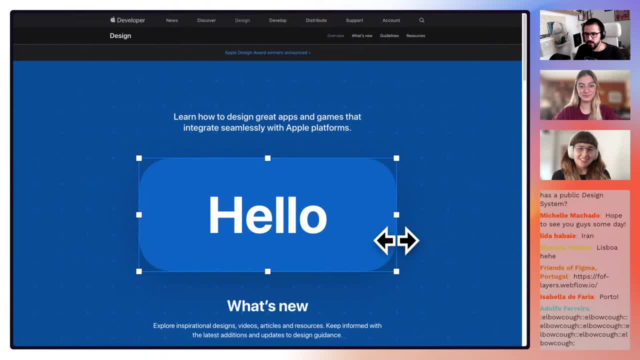 yeah, actually the for reference for those who don't, who are not looking at the emojis, it just feels like a dab. so very, very, um, I don't know Gen Z of us, I guess. um, but okay, so we're gonna talk about the Apple, uh, human interface guidelines, mostly because now I'm gonna switch to figma. 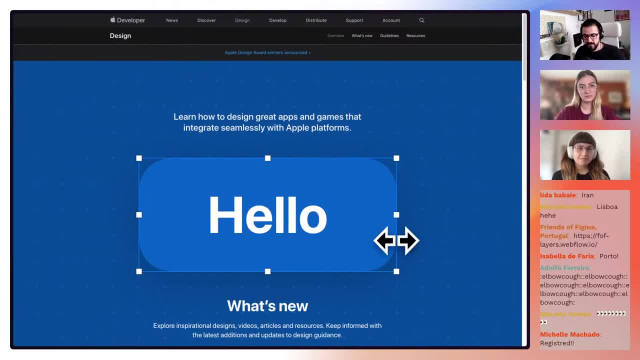 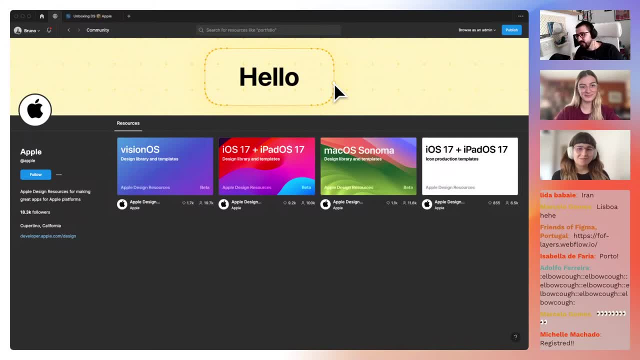 really fast. uh, they shared their documents in figma and I don't know who has been playing with them. uh, I have, uh I know that Raquel asked for sure because she has been um very much uh setting this up for us today. so big, big clap, round of applause for for because that, yeah, she's always. 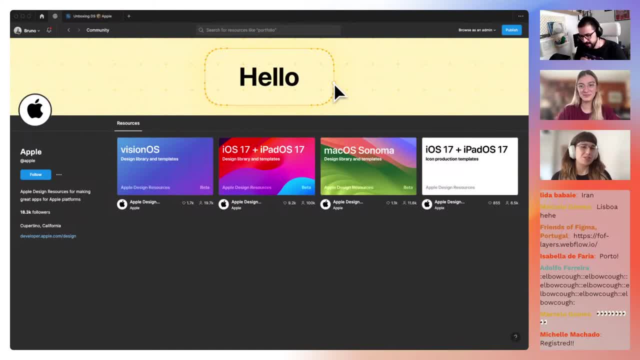 I don't have the vision always to test the templates, but eventually you can imagine how it will look like. next step for the next unboxing- actually the, I think the developer uh beta just opened this week. so even on that end I think most people are still waiting. they just registered for. 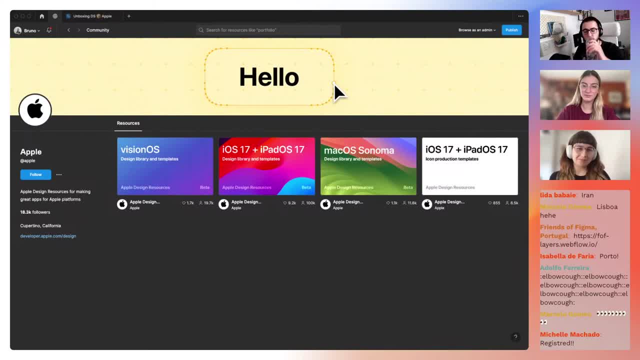 the developer beta. so let's see how that goes. yeah and uh, basically we're going to be doing a little bit of what um we do in all streams, which is we're gonna open these files, duplicate them, play around, um on them, um. but if you ever want to find these design system and others, uh, you can add to design. 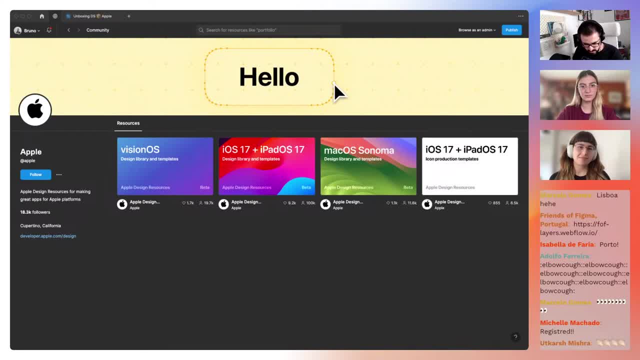 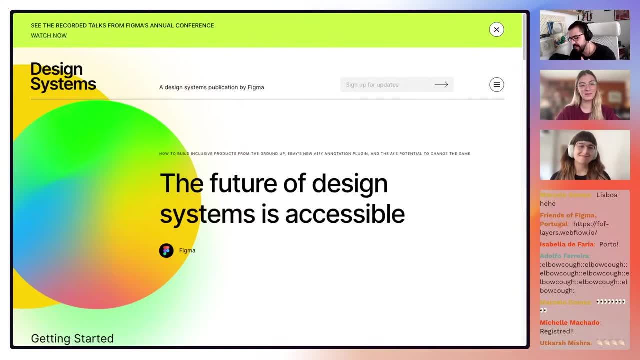 systemscom. if my system is working, which is not, let me just change here. um, there you go, which is a design systems publication by figma, where you can find a repository of probably- I don't know, is it dozens, or is it already- hundreds of design systems. I'm I'm still 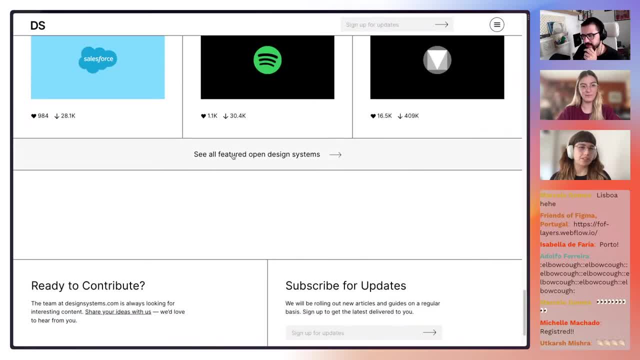 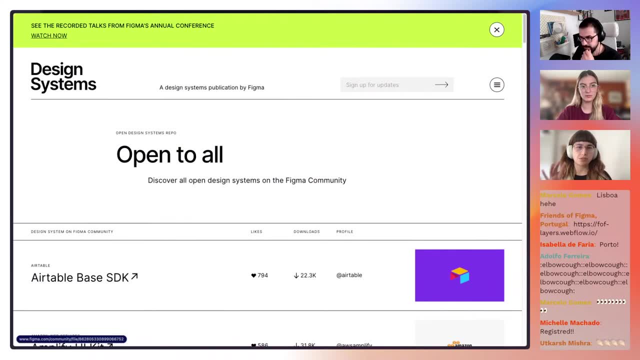 changing. I don't think there are hundreds, but perhaps it's already. uh, depending uh how much they update, because, for instance, I think, uh, Apple is still very recent, so it's still not here, but eventually I think it will be so probably there's a lot of design systems that already starting to. 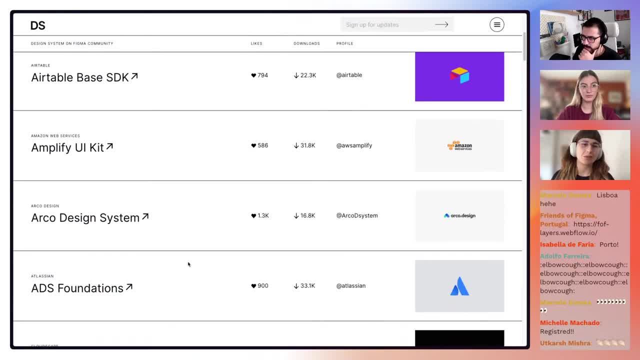 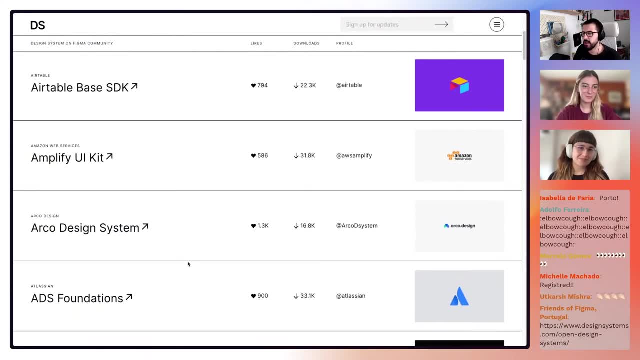 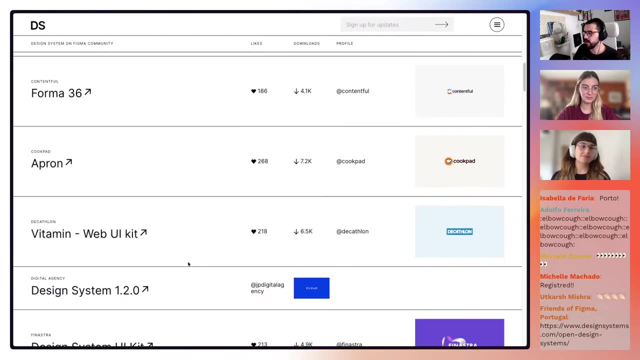 be at the figma community, but they still haven't been spotted here, so hopefully there will be a hundred. I think, yeah, and then you can already see a bunch of them here. air table: uh, um, Amazon Amplify UI ads from atlation that we already looked at here. uh, the catlon. 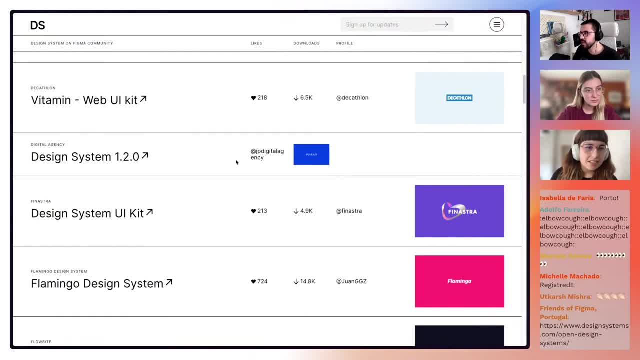 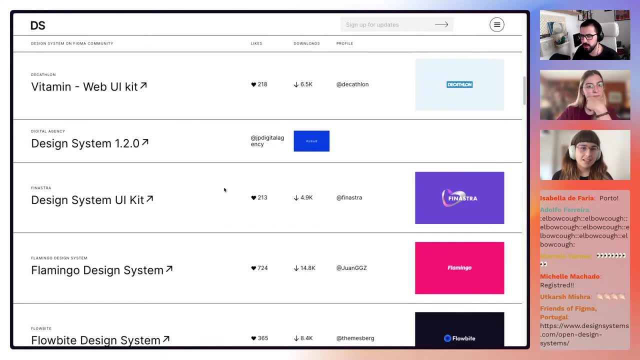 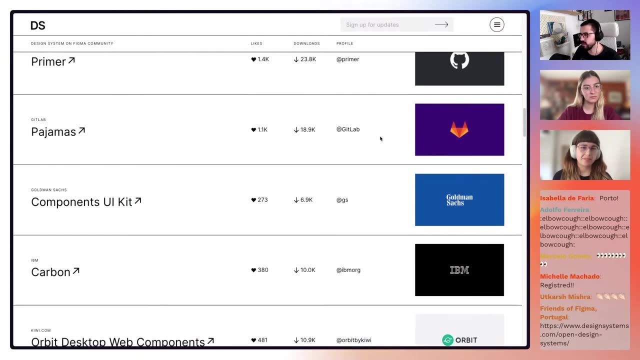 um, there's apparently a agency because, if I'm not mistaken, you can- that's new. yeah, you can submit your own design systems, and this one might not, uh, be available on the community anymore, or something like that. uh, finastra, Flamingo, GitHub, which is primer, and then gitlab, which is pajamas. 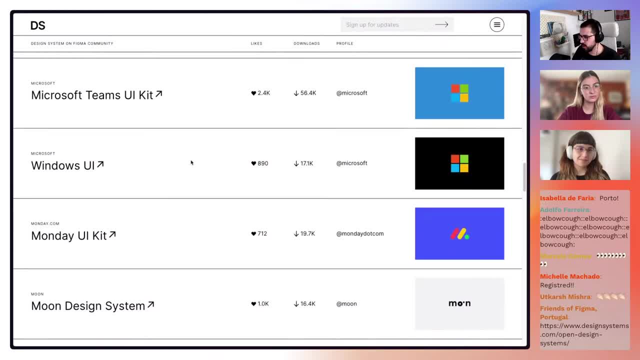 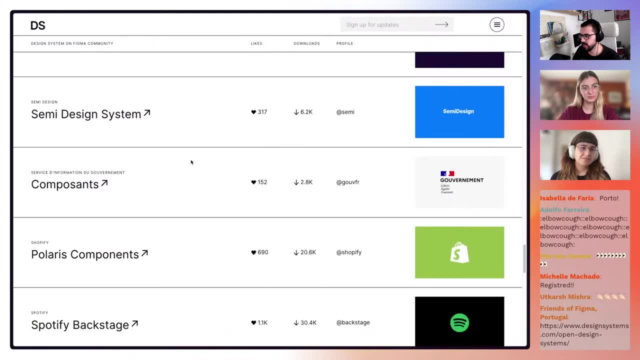 orbit. there's a bunch of them here: material design, which we already look at, uh, and design, which is an amazing design system, a lot of design systems here for you guys to take a look at, in case you have something in mind. you can also share a suggestion for the next unboxings and we 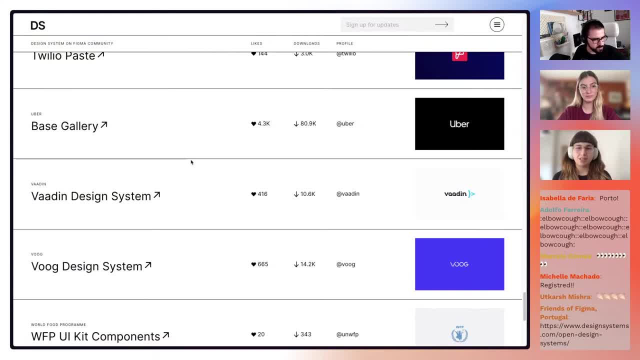 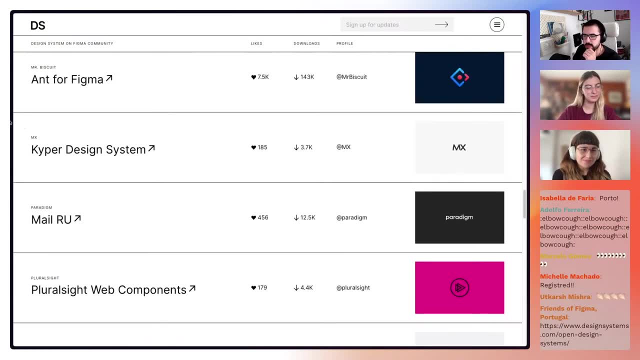 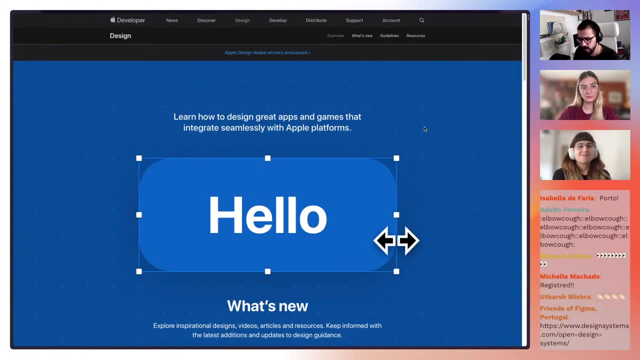 will have the pleasure to also to explore it. so feel free also to suggest what you you would like to hear from us exactly. so let's head here to the Apple website. um, Raquel, you have been looking at this a little bit longer. I think Beatriz has also done. 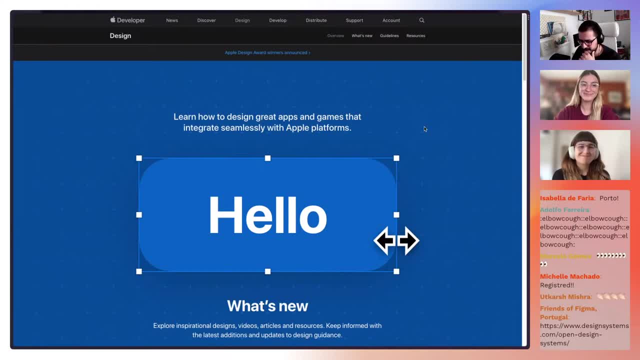 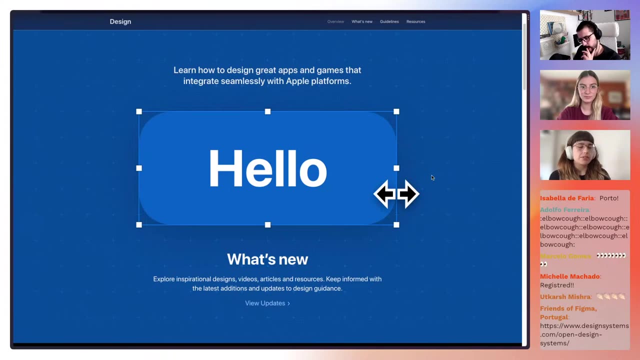 a better homework than me. so what do you guys think we should be looking at first? yeah, so I would like just to give like a review of the home page. I usually like to review home pages because I think really illustrates the goal of the with this big. 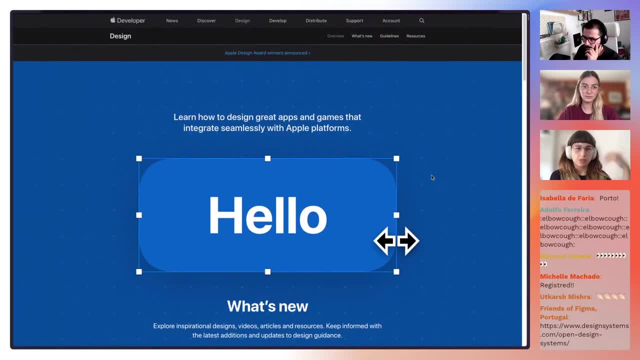 companies like how they want to, uh, you know, mirror themselves on the homepage and how's the goal that they want to communicate. and I found it very interesting, uh, that the big banner is actually what it's new, especially because it seems very recent. so they just I. 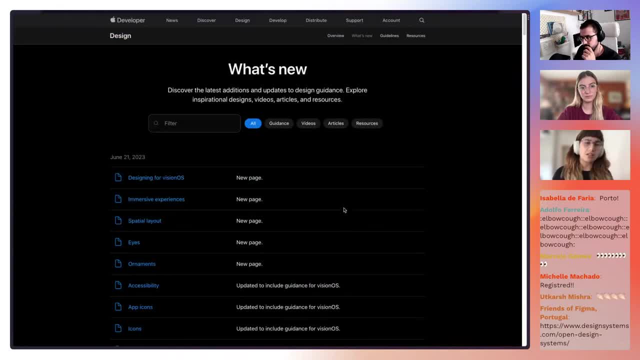 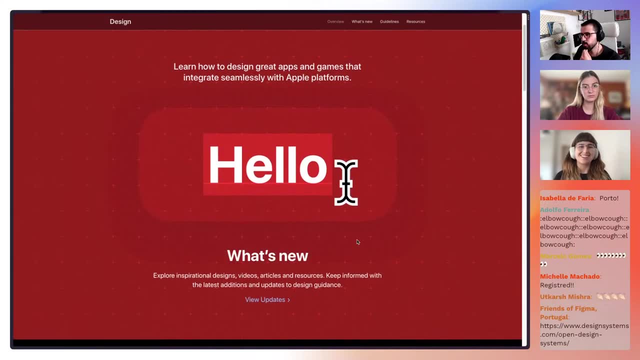 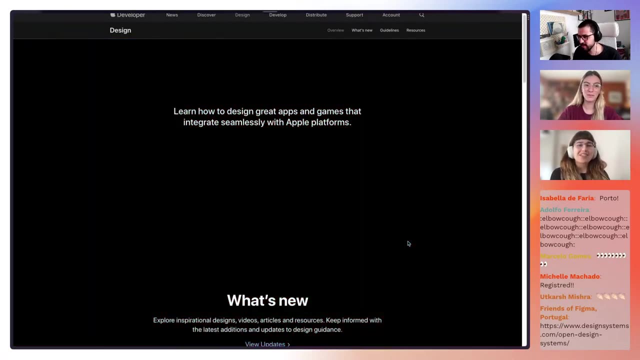 think they plan to have a lot of what's new updates and if you basically eventually, when you go back and then do a refresh, the banner actually changed color, which I found it was interesting. yeah, yeah, it's a very, very little thing, but I found it funny. yeah, and it's only blue and red. 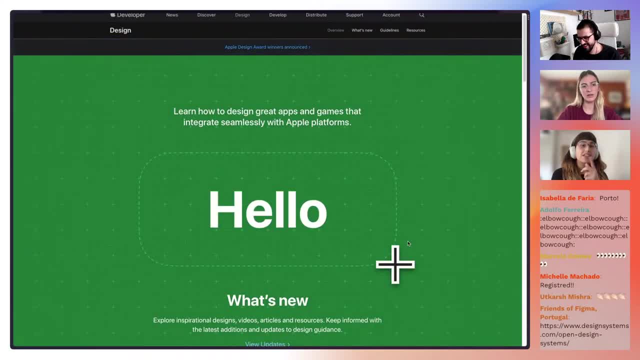 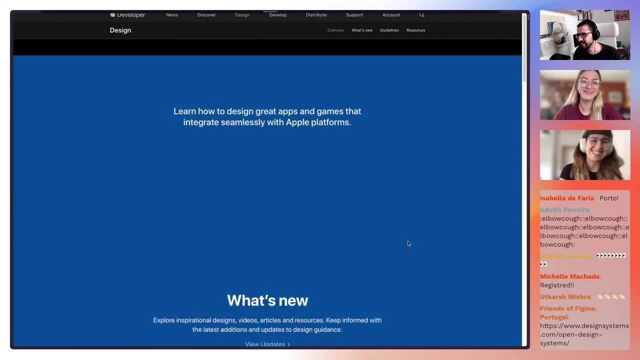 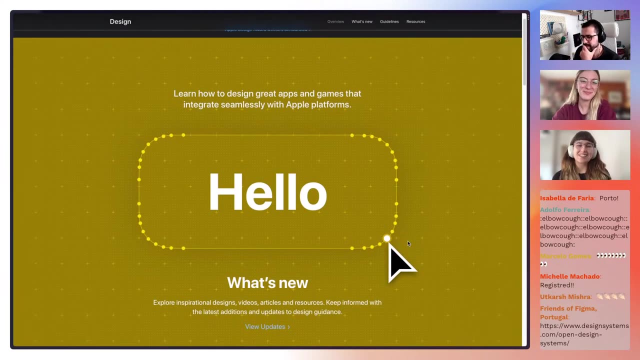 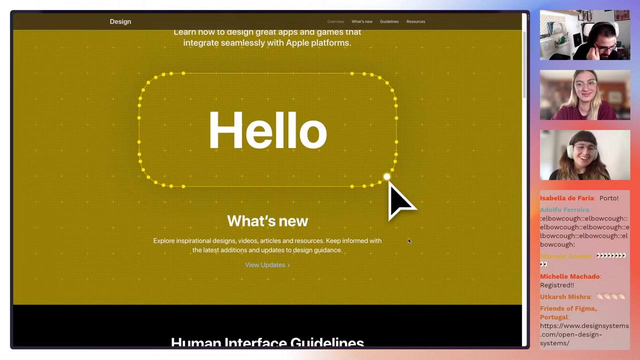 yeah, no, no, I think I also saw yellow. yeah, the yellow one I need. yeah, now I need to catch them all. so, orange, yeah, the same. green, blue, red, oh yeah, I can't. yellow, yes, okay, yellow, yeah, no worries, it's just my favorite. and then I've, yeah, I, I love it as well, mustard yellow, especially. uh, then I found it. 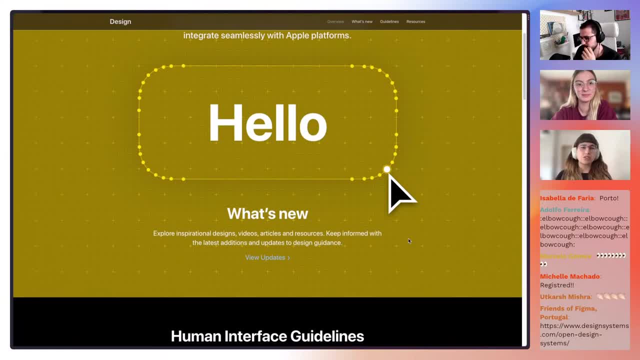 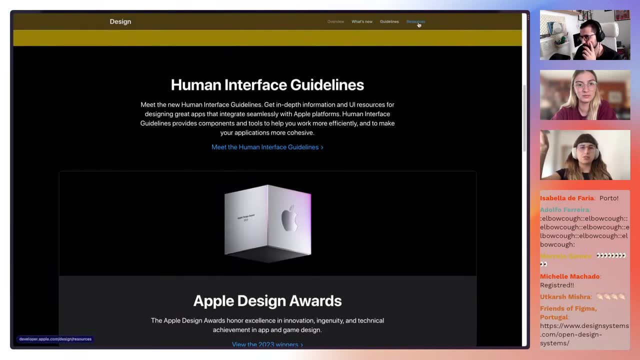 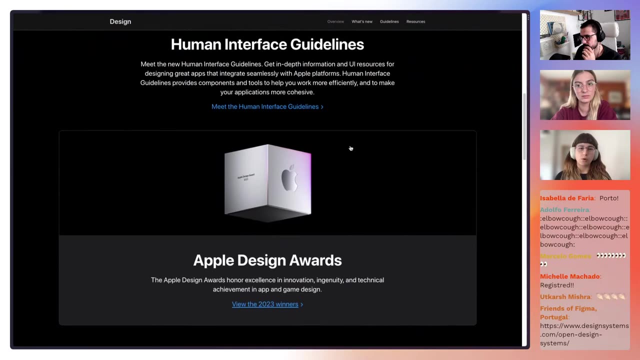 interesting, like the main goals that they pointed out and basically the structure that they use in Apple products. I think that you have like the tab and then you have the top uh corner at the right with the main sections and it's with new guidelines and resources. I found it interesting that they have like Awards and that one Apple's design Awards. 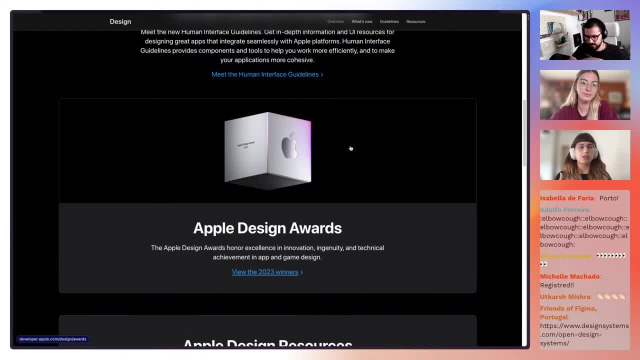 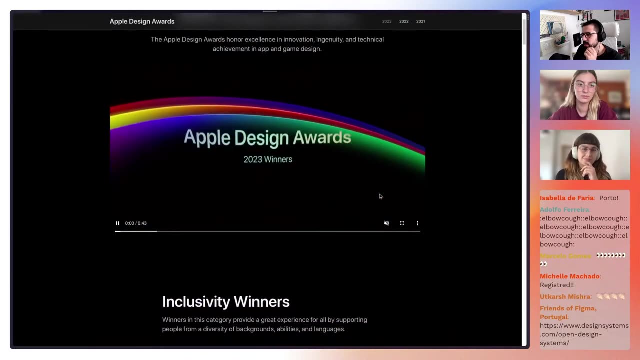 and I found it interesting that strategy of promoting their products, uh, with awards- because I don't think that Android does that, for instance- and I found it interesting like let's engage more and create more culture with design and give awards, uh to applications and games- and it was interesting. it's always interesting to see. 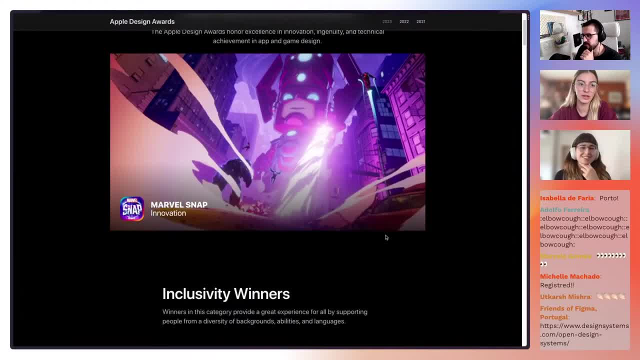 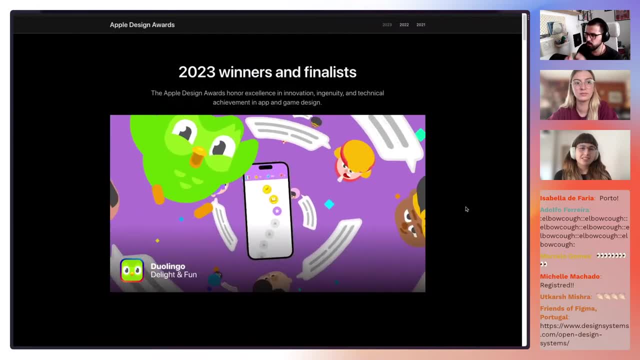 the, the people who win those Awards and log out. yeah, yeah, also affects the the way that these apps eventually get out into the world, because Apple doesn't give awards in design and and doesn't support these communities based on, like, how big an app is, it literally is how well designed it is. 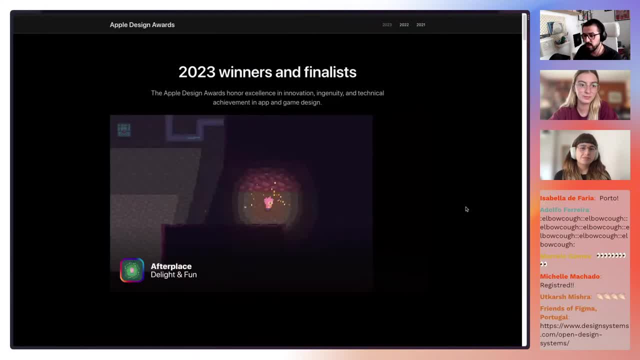 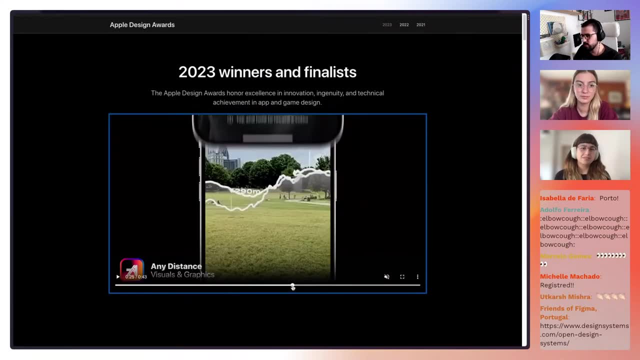 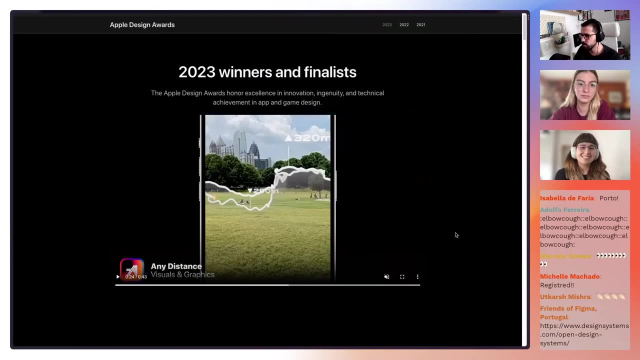 how well it works and some some of the award winners from this year, for example, are very indie business like. I know this app because they were people were using it on blue sky and they were sharing it, but it wasn't that well known and then all of a sudden they got a boom in users, so it's 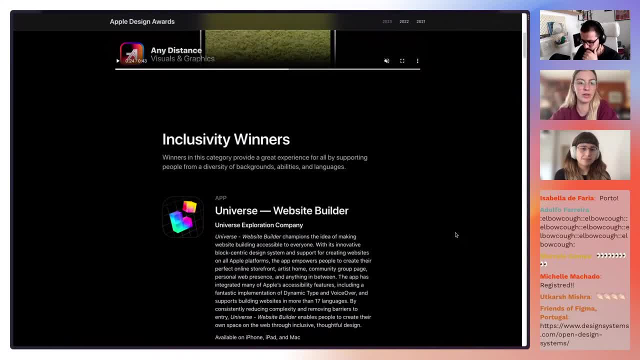 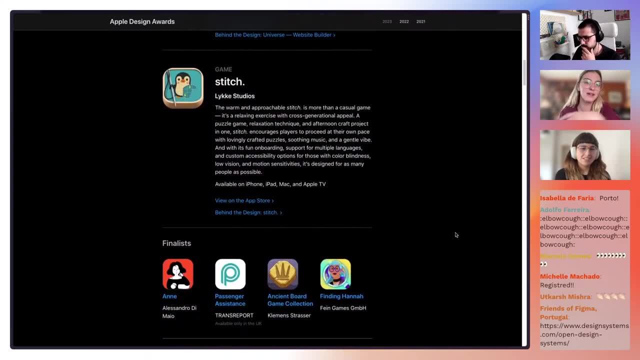 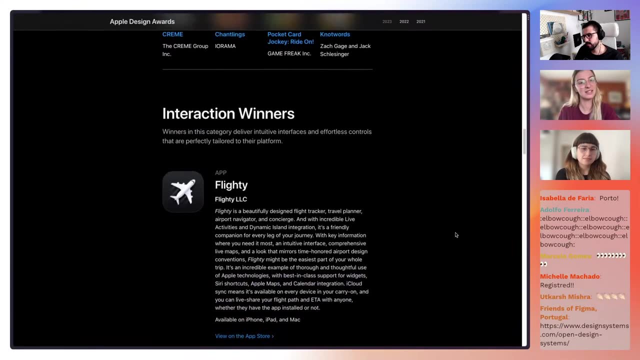 also a very interesting thing. yeah, I must say that there's a few of them that are actually known. I remember Bumble actually won one like two years ago. um, good of that I I must say I mean it's an amazing platform and app to get to know people. but it is true that design system it's 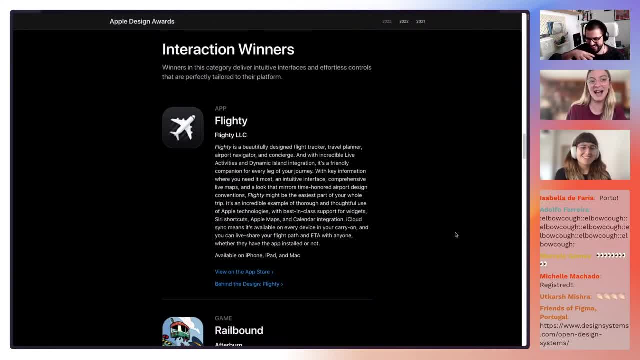 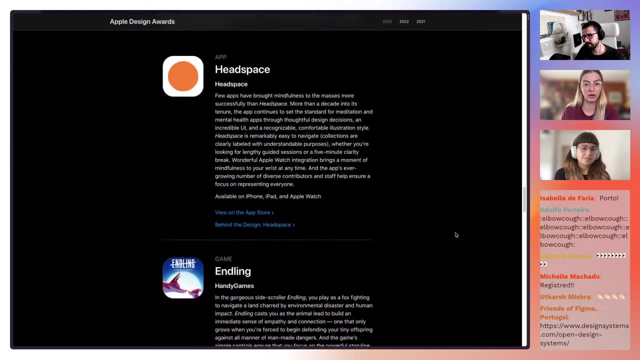 not the best, so of course it's not. this is not a design system Awards. it's a design Awards, um. but I do feel that sometimes the design systems are also important on the way you design. and, yeah, how this Awards? because, like we, we can see a lot of apps that are beautiful and are consistent, but 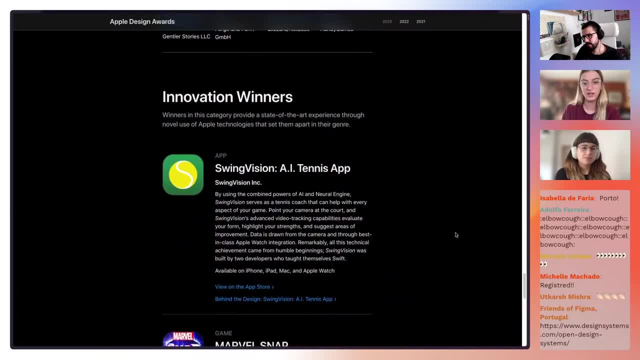 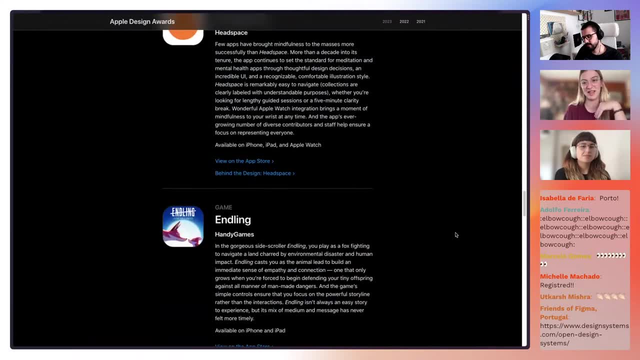 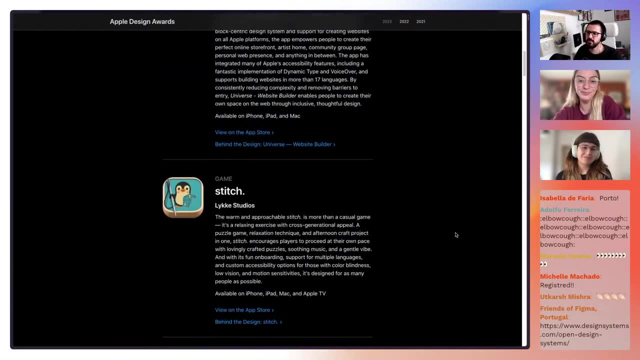 maybe behind that it's not that well done, it's just things that you find pretty um and you don't use, for example, the eight pixels grid, which for me that's like you have to um, but oh well, it depends right? yeah, yeah, and a lot of a lot. 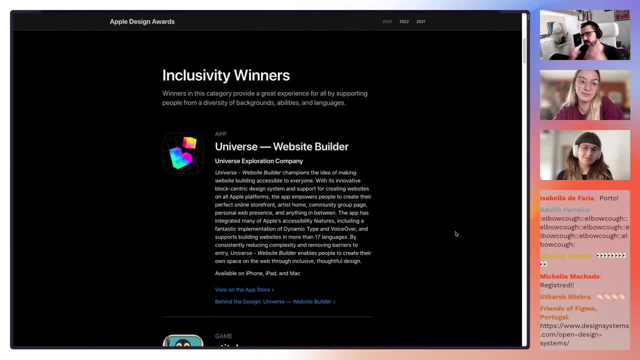 of it is not just like the, the, the way that the the system is needed for, the UI is needed or anything like. and a lot of these apps are very different. games are done in a way. others- yeah a lot of them- also don't use Apple design principles. they kind of just have their own design principles. 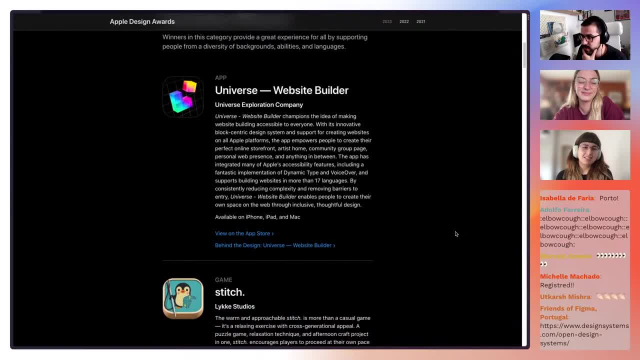 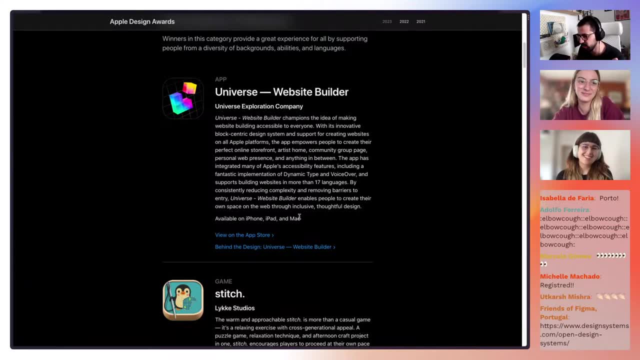 and things like that, and yeah, yeah, and- and some of them are very interesting. I could do an old universe or a whole episode of this just on universe, because I've been using universe for years, and just the fact that you can build websites directly on your phone, universe play and a few other apps that are like getting into this world of creativity. 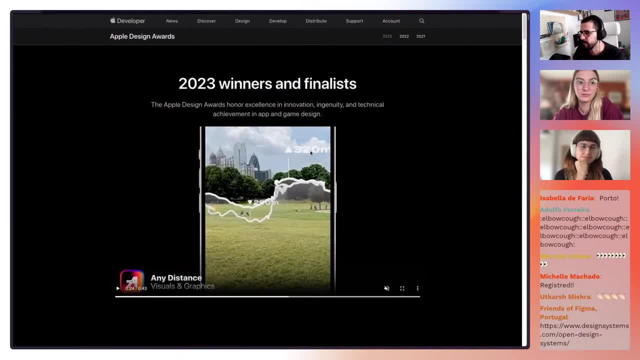 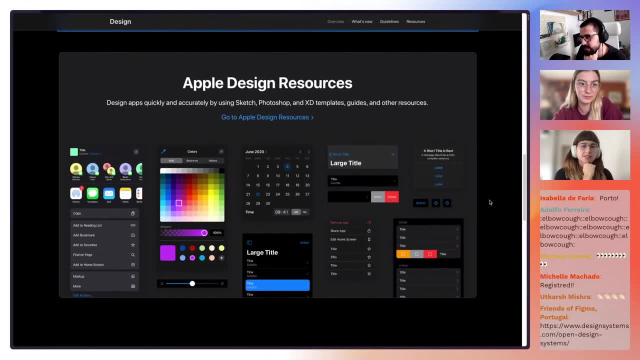 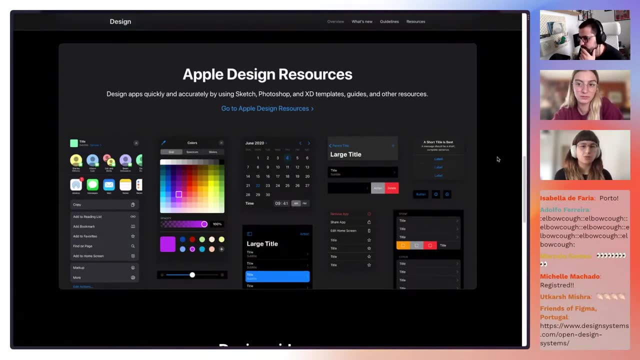 that works directly on your smartphone. it's really cool. but, yeah, and design Awards are always, uh, interesting. when you look at the Apple design Awards, then we have the resources. yeah, the resources. I found it very interesting because I think, from the design system that we've been analyzing so far, 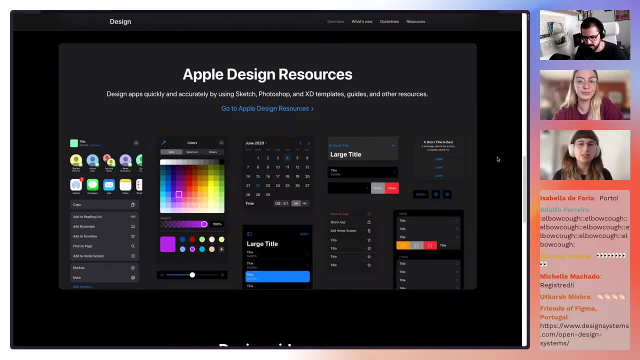 the fleet. regarding templates, like the most ready to use screens, which I think it's a very good sign of maturity. uh, when you have you have so much, much consistency, you can eventually share templates and you feel like, okay, people can use it and it's ready to use, uh, maybe, for instance, other realities. 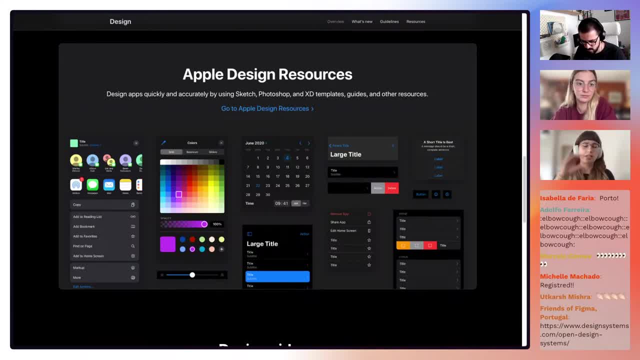 as we are seeing it in awards- that apply some marketing, uh, and then some brand inside. maybe it could be interesting how they eventually use these templates. from what I saw seems like the regular iOS user or macOS user, so I was just wondering to whom these templates might be. you know, in case you want to personalize something or just put a little bit of. 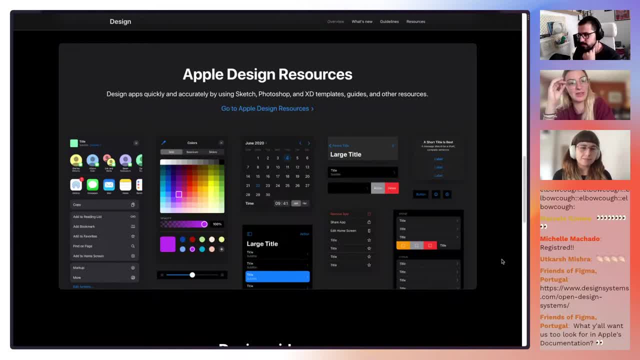 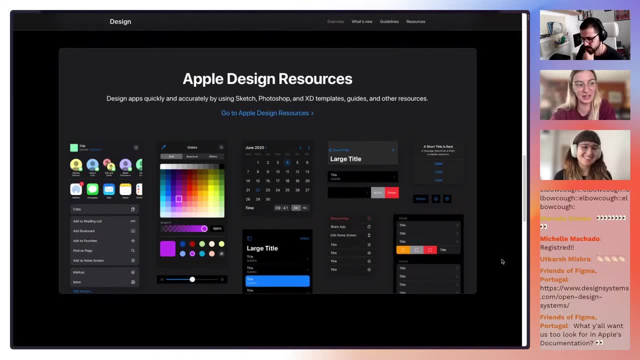 branding. that could be interesting. I'm gonna say that I think I'm gonna be the backup here and say like, honestly, I'm not the best fan at the human interface guidelines. I think there's like a lot of more design systems that are much better than this one. I mean, of course we're going to dive into. 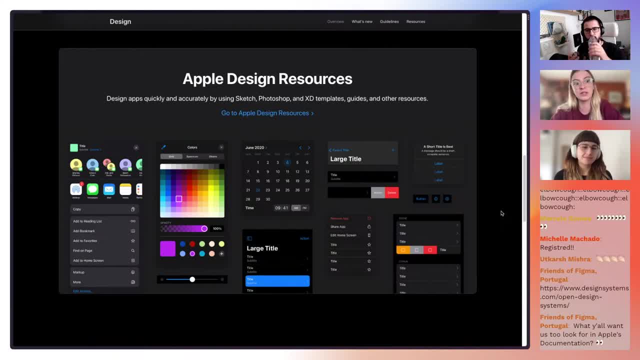 that in this episode, but I do feel resources with the templates at least, they're very good, but there's like a lack of foundations. where do they come from? how can we see them? um, what did they use on the templates and how they structure everything? because I feel like templates is the thing that 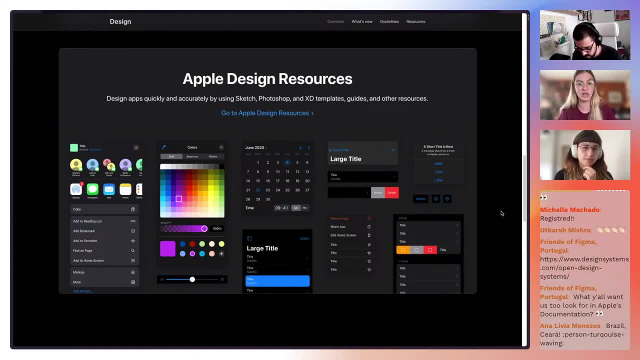 you see, as a as a user, but not the entrails, like the foundation is the components, like the small components or atoms, or whatever you want to use it. um, so I think that's something that Apple actually lacks, which, at least for me, makes no sense. um, because the design system, basically the foundations, 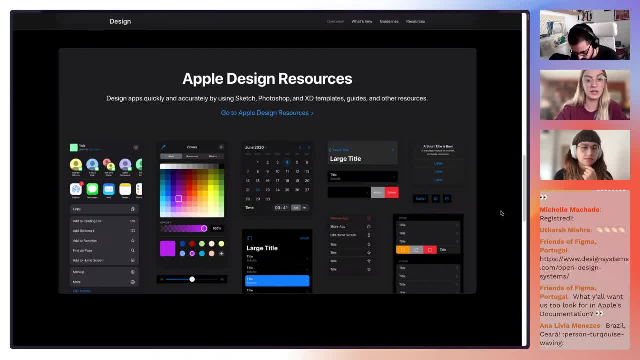 are the pillars of our design system. so why? why can't we see them? uh, maybe it's because of some Apple's big company thing, who knows? yeah, um, but I would love to see that honestly. yeah, and maybe on the demo part we can go dig in and try to inspect and see the sources until we get to the atom design. 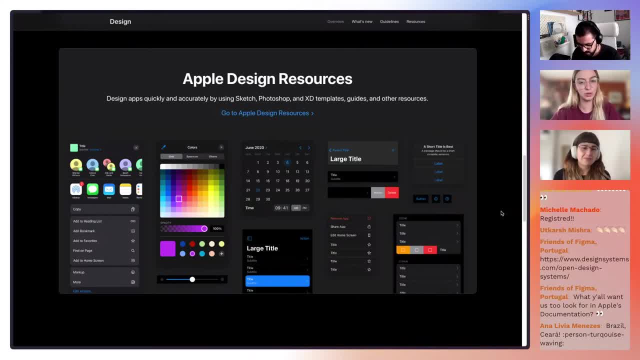 if they're public, because they might not be. that's why I do like a lot, a few design systems more than this one, like, for example, the spectrum, which is the Adobe one- um, I think it's really really nice. and decathlon, which uh released the vitamin design system on figma. that's also amazing, yeah and uh. 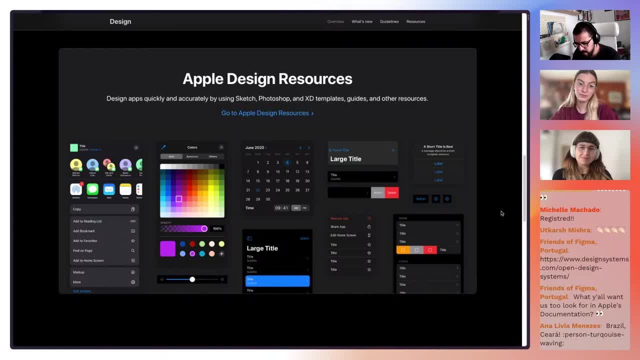 honestly, I think your, your criticism is not bad or anything like: oh, I'm against the like everyone else. I think for years, UX and UI designers have been critical of Apple's design system, mostly because during the Johnny Hive era, because if you look at it, you know that like they weren't the best. 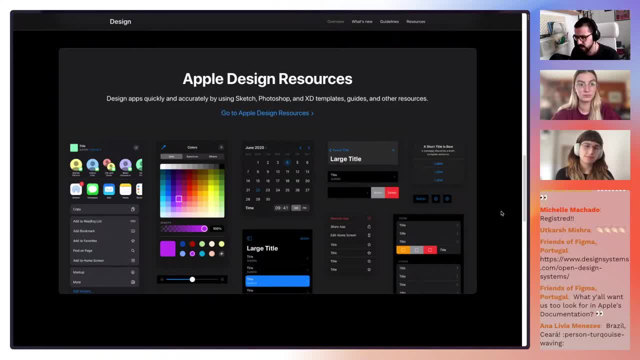 before. they evolved a lot in the last few years, but they, they always are this edge on it's. it's not. it's never like fully user-centric. it's like innovation is like the core of what Apple does. so they test a lot of things, they, they break a lot of barriers there. 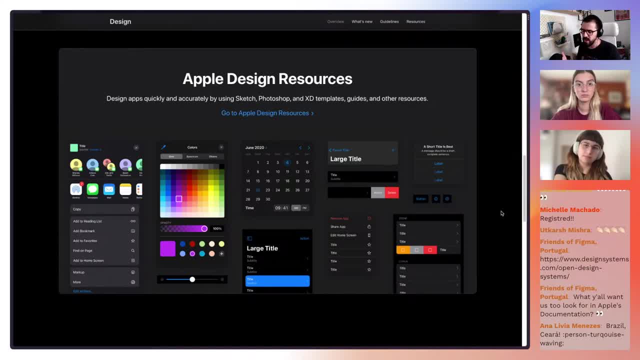 but I think they became better. post Johnny Hive here, because Johnny Hive was an amazing product designer in the sense of like industrial design, but then the same principles that were then being applied to design to the UX UI were not as well scaled up. there are some details that are fun. 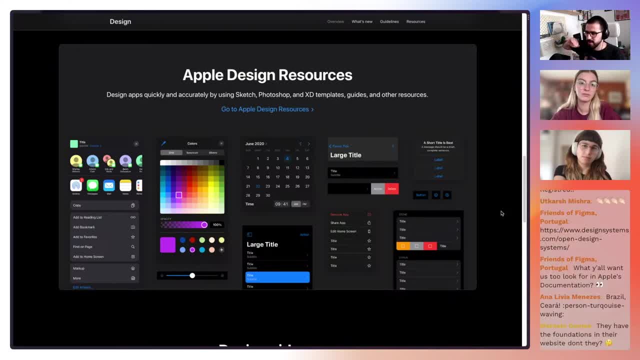 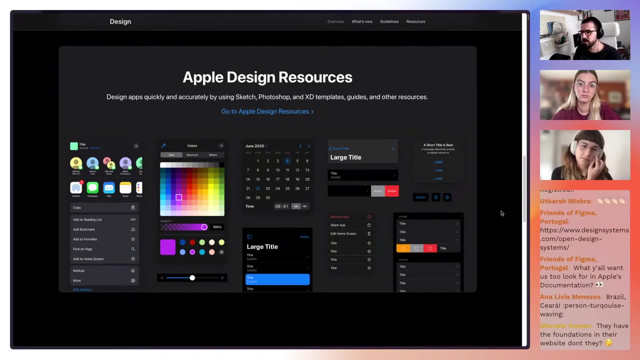 like the, the way that they went above and beyond to create the, the Apple curve, right like the, the whole algorithm to make sure that the curving on the Apple objects and everything are very interesting. but in any case it's, it's one of those things there's like it's. it's about the craft, but 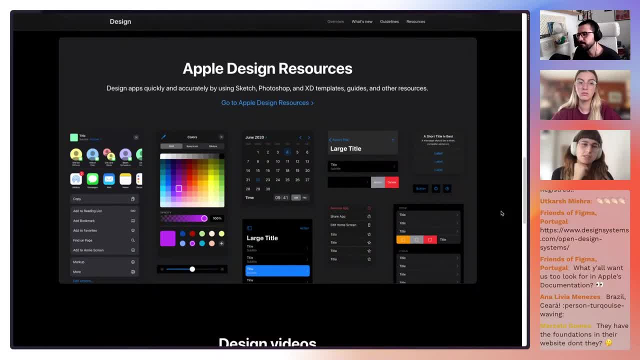 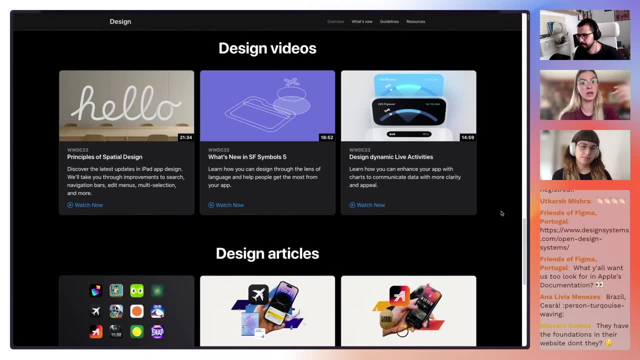 many times it's not about the best experience, I guess, and I also feel like, for example, they- yeah, they've been amazing at design, of course, because they have the resources for that, and they're also a company that it's old, or let's say that they've been here since the beginning. 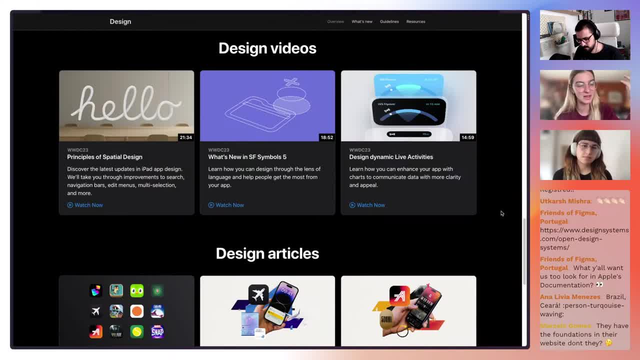 um, but I I do feel like they could be doing more. you know, the design systems community or the design Community itself, um, there's not a lot of the things that we see on the human interface. skylines actually are usable, they're just really nice. UI, yes, um, because they're beautiful, of course. 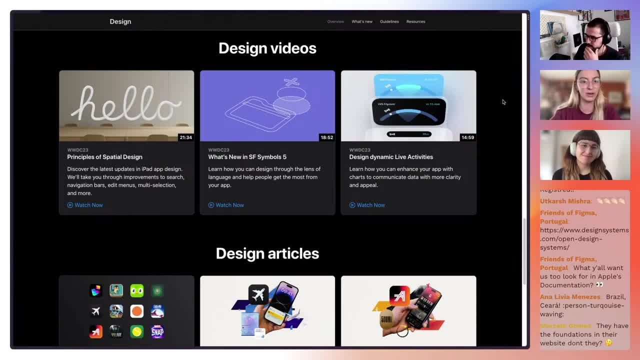 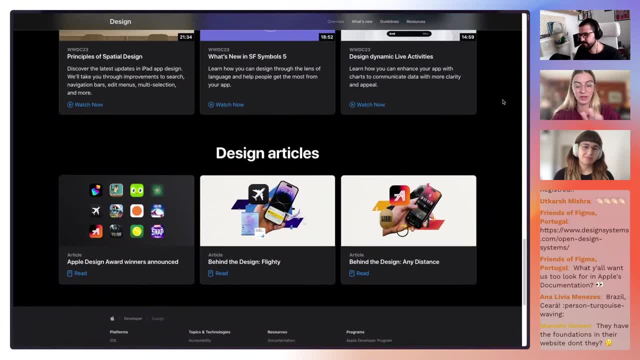 they have a lot of designers and like they, they are amazing at their job, but it's not like they. uh, I don't feel that useful um the human interface skylines, so that's why I'm a little bit of it like um and actually, for example, 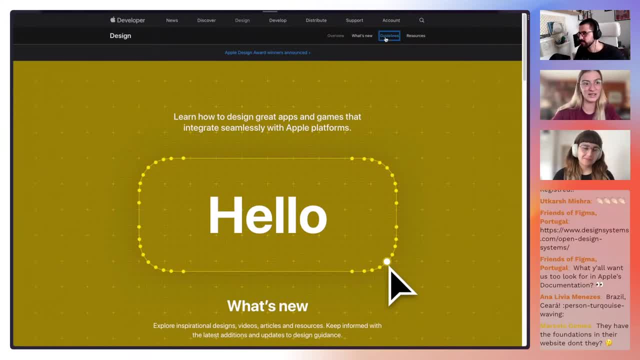 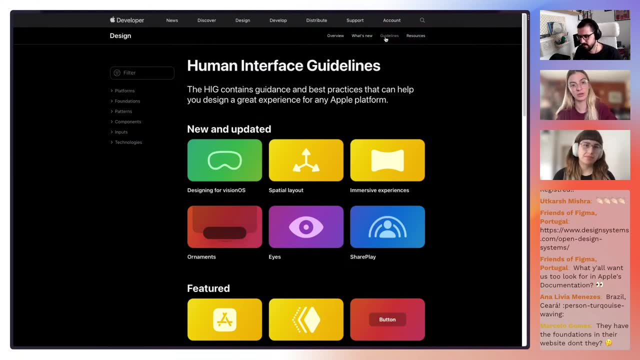 one of the things that gets me crazy the most is that they don't have a design website. they have a developer's one. so when you enter, you go into developers one, so it's not like another thing for design, it's everything. they give more power to developer, which I don't think. um, that's good. 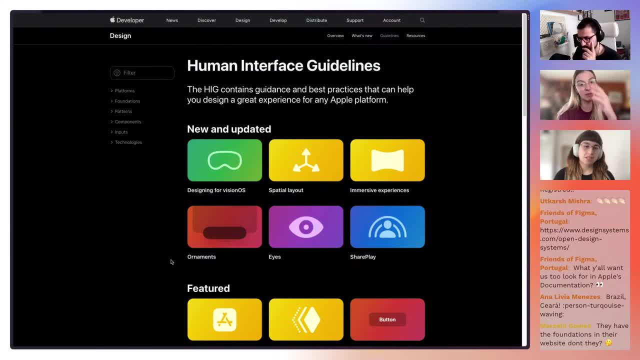 of course, development is what makes you use the app or whatever, but I feel like design should be on another platform or on or on another website. um, that's at least some of my points, which I'm not, as I said, I'm not very keen into the Apple's design, but, um, yeah, they're the best at what they do. I mean, they release a new um frame. 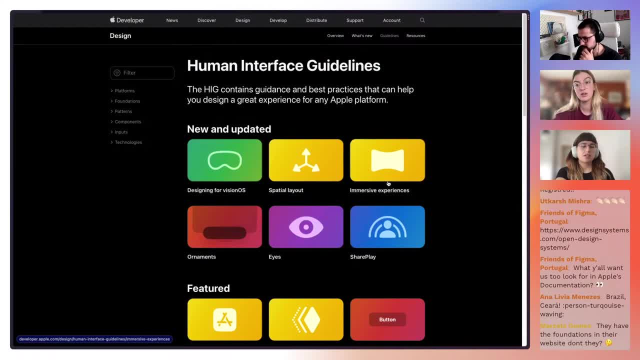 or a new website and everyone starts copying the things that they did. so, yeah, they are referenced, but I don't feel like they're the best, honestly. I think they also. we create a lot of high standards for them, a lot of high expectations, so every time they're doing something new or changing, we're kind of like, ah, they do this like. 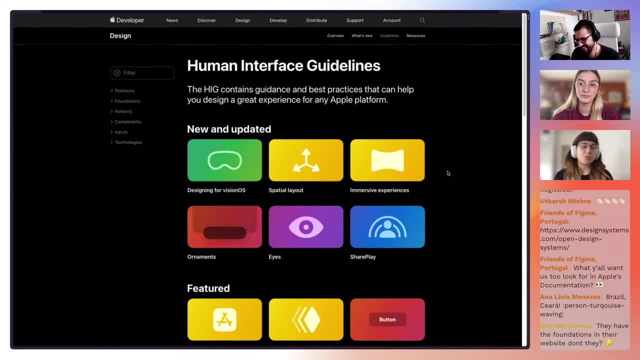 that why, because we have that high expectation also, perhaps the way that the website is organized probably could be something like related to the how the company uh sees the organization inside and for them probably could be more suitable for design, be inside of the development cycle, perhaps not sure. yeah, I just wanted to point there was a funny fact that they had a Photoshop. 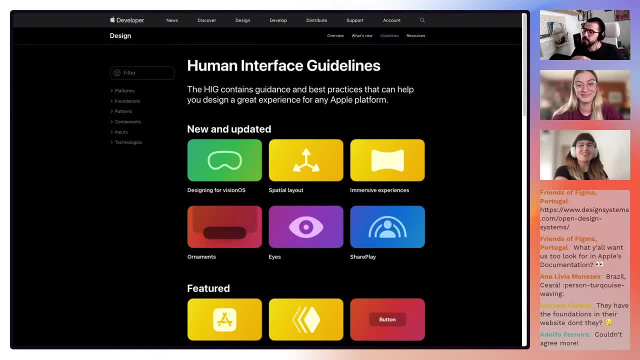 also like how long they they are in in the long way with assets. it's also the thing on that I understand the need to have what is sometimes still are outdated types of files and specs. these platforms don't work for, although Apple devices are mostly like the new Apple devices. 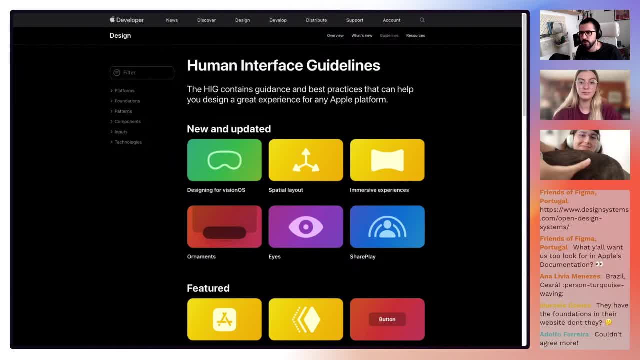 and the new stuff, but their customers might not just use the latest technology and things like that. like the company that I work for also has a type of worry. it was like: can these softwares work on, or can we help people design for these softwares on? 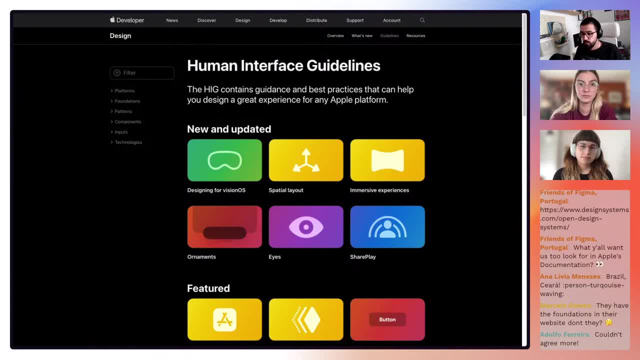 the whatever limitations they have in in companies like we're really, I'm gonna say, lucky to be able to be here and use Figma, for example, as our tool days today, because we are at the we're front runners, like we're front runners in this, like the world is still mostly designing in other tools and then 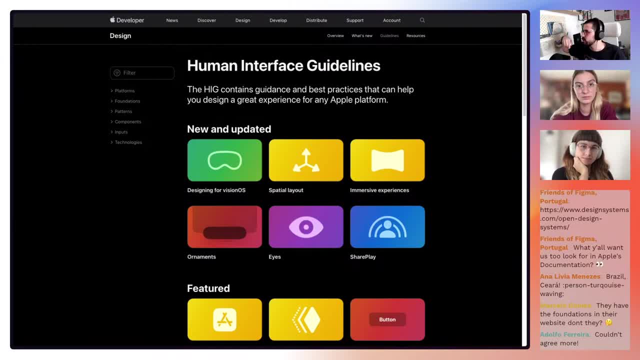 there's other people that just jump the phases of: okay, I used to use- I don't know- Photoshop and Illustrator and I need new things, but I'm not gonna waste time, so I'm gonna jump into Canva directly or something like that. they're not going through this type of tool, right, which is not a bad thing. again, Canva is an amazing. 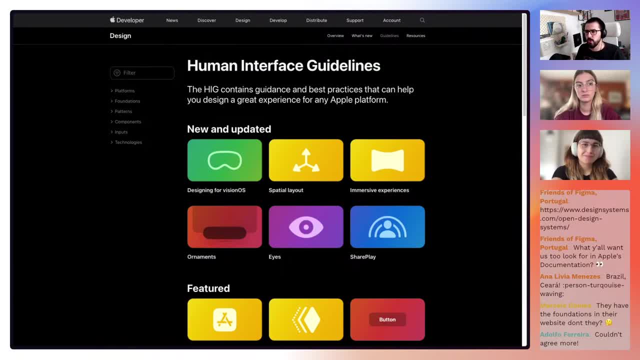 tool, but having this type of guidelines for older, older softwares or older frameworks makes sense under that context, right like we don't know how many people actually understand what design systems even are and I can say that, yeah, people that I studied with, uh, it's really, really hard on that end. it's like I probably half of the people that I studied with. 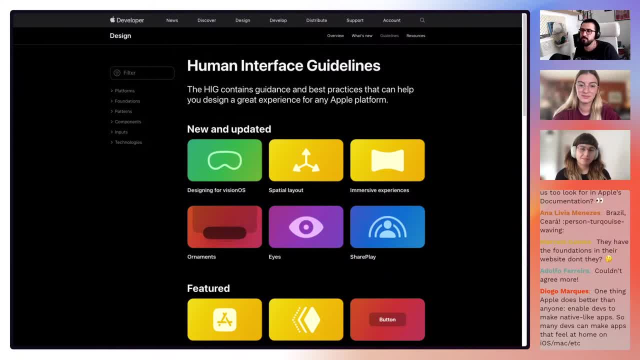 only learned what the design system was because me and a couple of other friends that worked in tech taught them like a year or two ago. yeah for sure that's also like. design system is still a new thing in the market. even that doesn't seem like it, they're very geek set, I think doesn't. 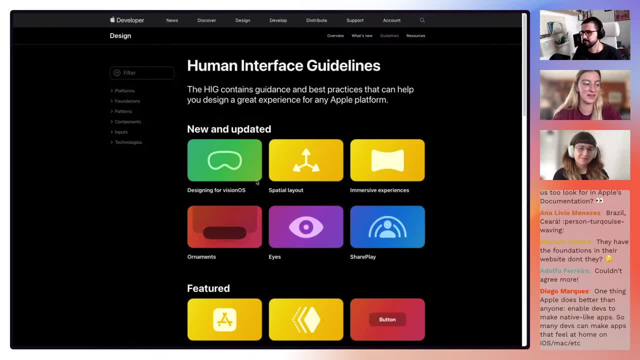 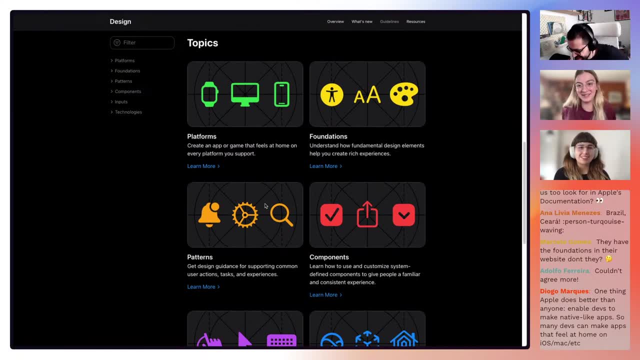 happen. doesn't it happen to you that when you're like family asks you like what do you do, you're like I really don't know what I do, just say designer, and it's already a lot there you go. okay, just giving you a couple of updates on the comments on the chat. so Adolfo says that he couldn't agree. 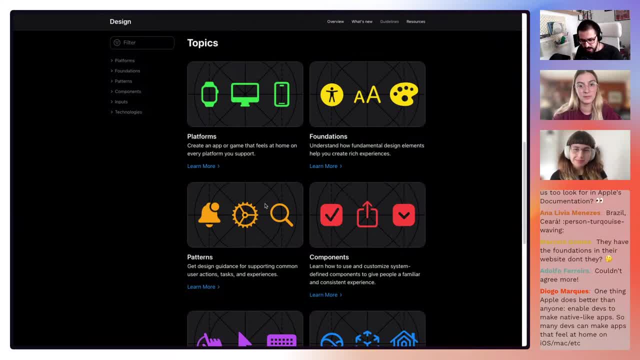 more with everything that utilities were saying, and Diogo added one thing. he says that one thing that Apple does better than anyone is enable developers to make native-like apps, like so many developers can make apps that feel at home in iOS, Mac and Etc, which I don't disagree like I do. 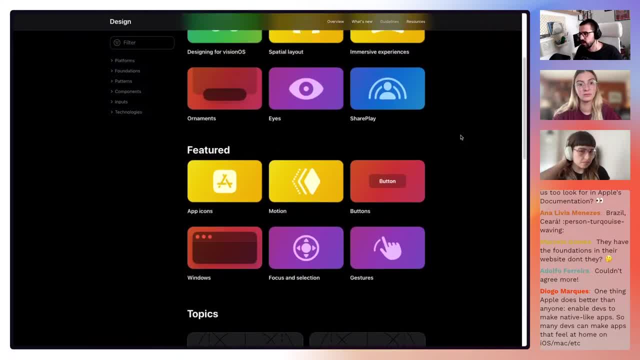 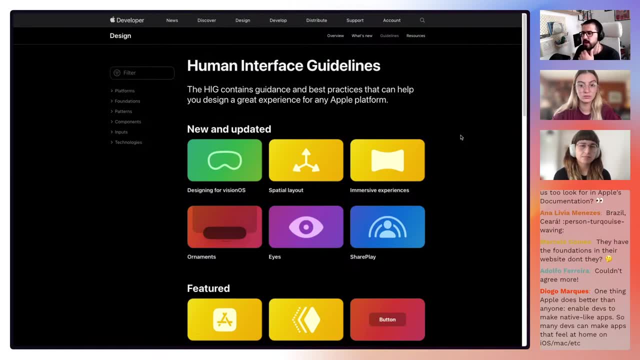 think the way that their system works is. they are very much focused on making sure that people understand that that app acts the same way as the rest of the system and and they push for that in their guidelines, in the way that they they talk about things that and especially. I'm gonna just 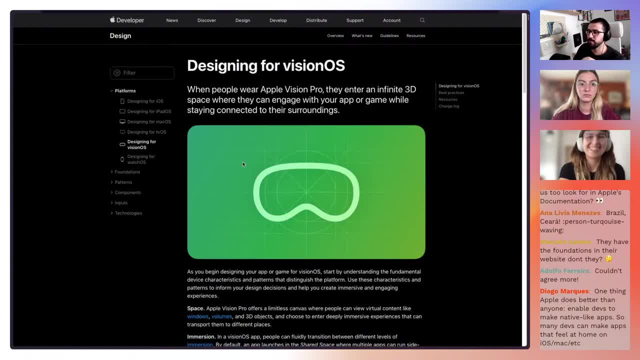 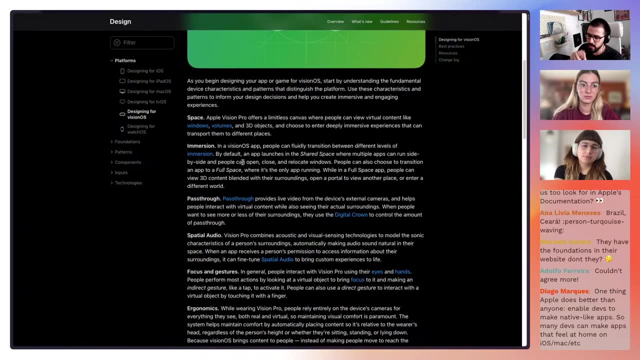 come here and click on the yeah Vision OS because, for example, just just because this is the latest iteration on that, but I remember, yeah on WWDC, when they were announcing it, um, and, and they started sharing the stuff about Vision Pro, they immediately like some of the main sessions. 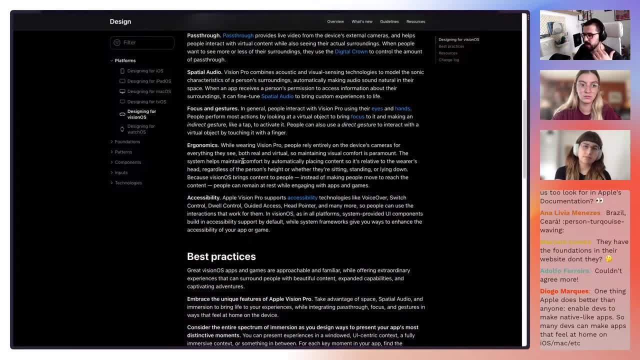 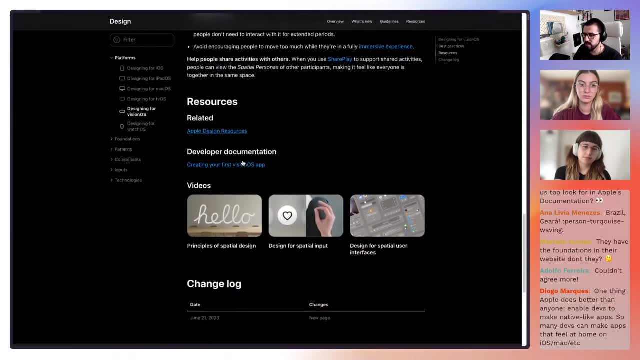 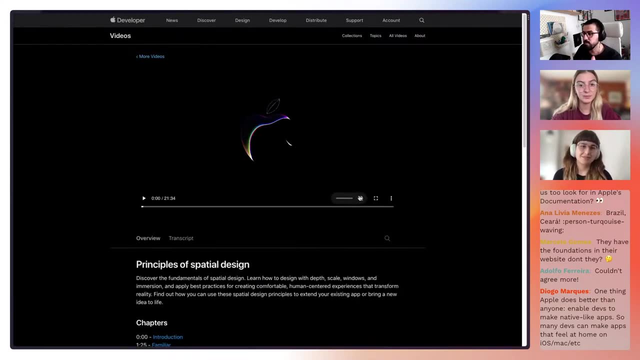 of the day outside of the keynote were literally people starting to tell you best practices on how to design and develop for the system. right, it's, and it's very interesting because they you have videos with this. right, like we can come here. yeah, like, there's principles of spatial design which 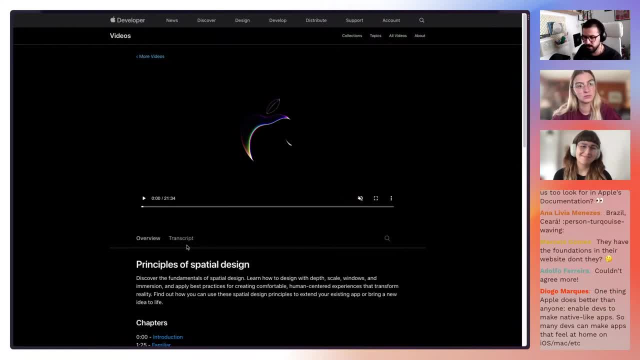 by the way- and this is where, again, Apple is usually very smart of this- it's a great marketing tactic to not call it mixed media or amended reality, right? it's like: yeah, yeah, they create already a concept, they create a, create their own. yeah, they created their own name so that. 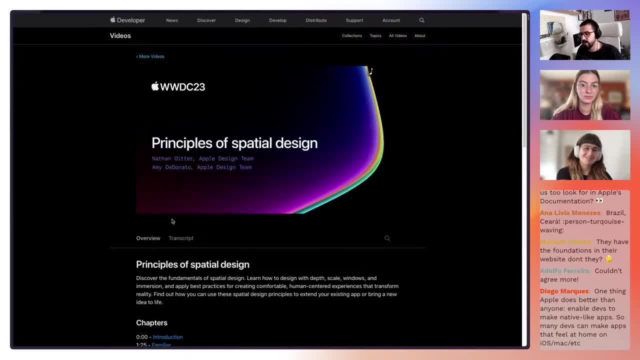 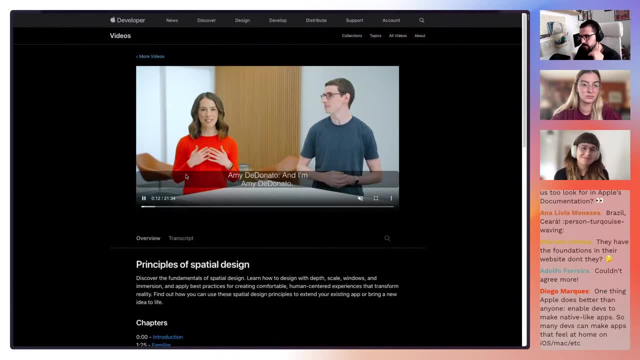 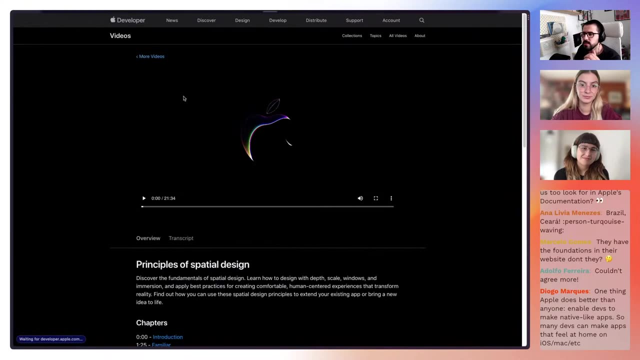 no one else can copy it, but the fact is like there's a bunch of companies already working in this space. but but it's interesting how now they basically went and they created a good um set of guidelines to help people start to create and develop for this um, and then, and actually this, 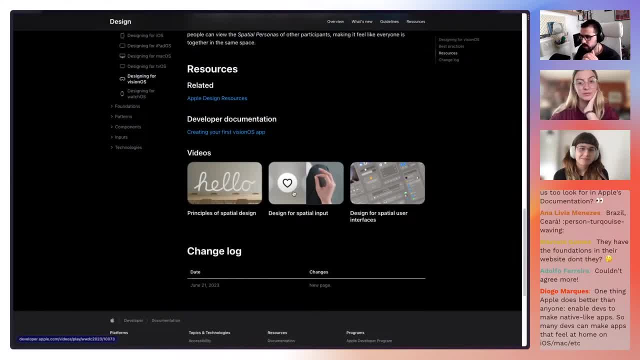 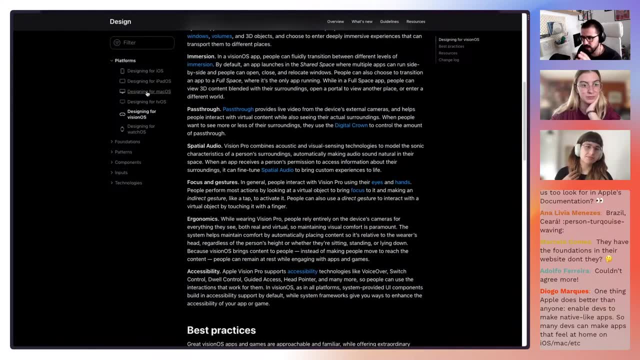 wwdc, so i don't know if this i need to go back yet. there's like designing for special inputs, designed for special user interfaces. they have a bunch of small things, but if you look at the way that the system works is there's designing for devices, but everything else- patterns, foundations. 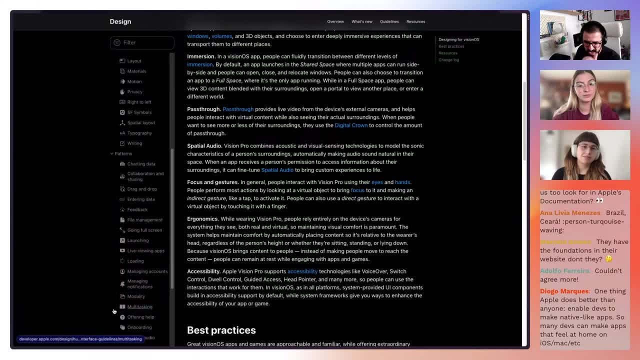 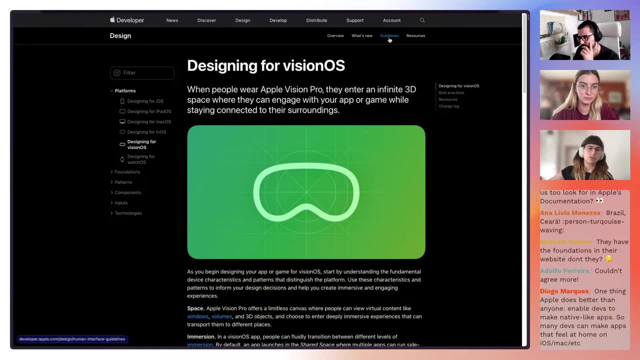 and everything is the same across their system, which many times i don't think it's as scalable on others for for sure. yeah, i was actually going to comment that. i found it weird, but interesting as well, that they have the first organization for platforms and then they eventually focus on that. 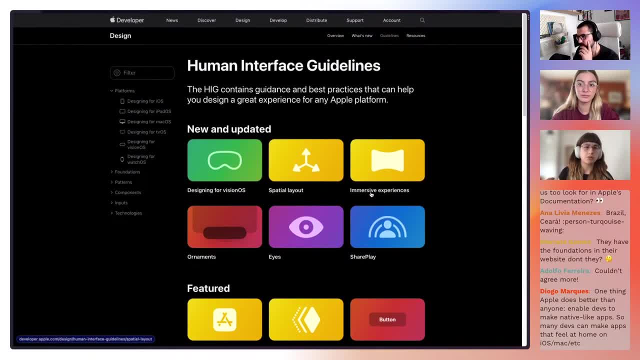 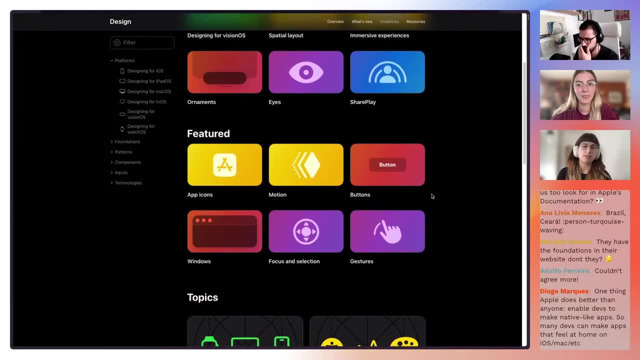 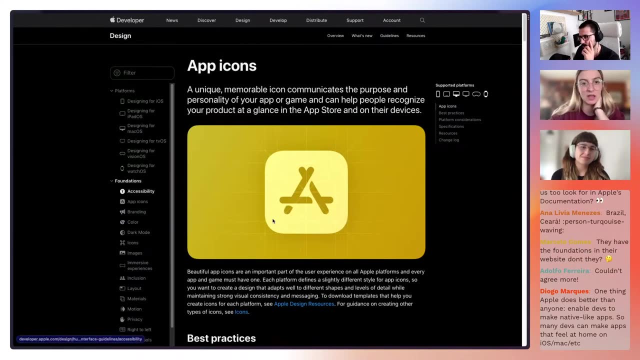 platform. but then when i was digging with foundations and components etc. i felt like, oh, this is for every uh platform which i found it interesting, if it was good or bad. you know like, um, yeah, i agree, i also don't think if that's good or bad. i mean, they say what's the 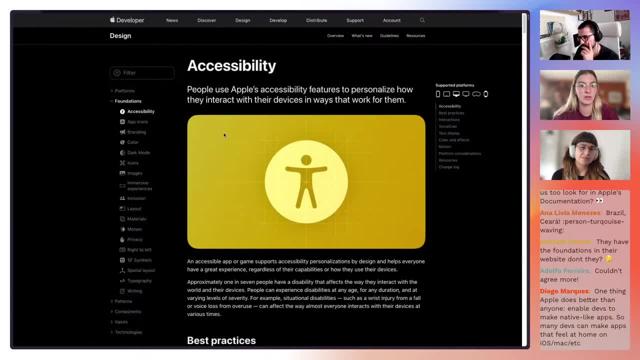 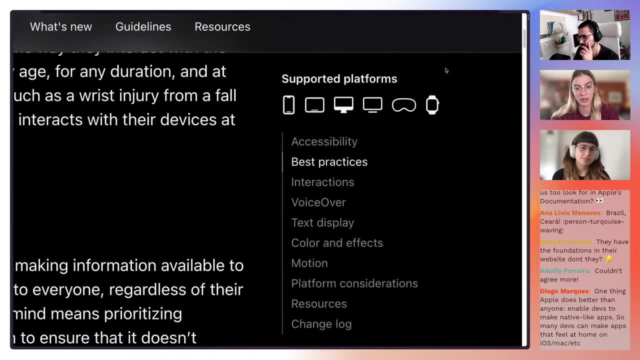 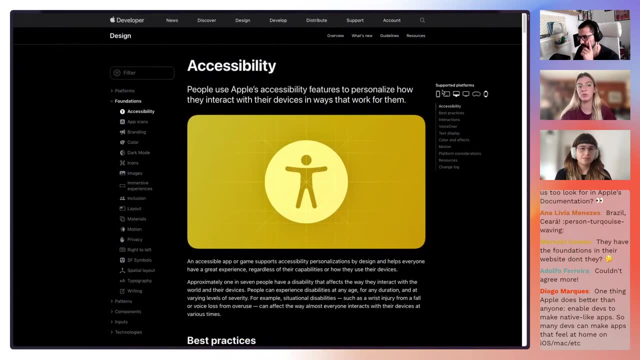 device that it's supported. so it might be some. some of them are, some of them are not. um, yeah, i don't know. maybe i just want to see special things for uh, a macbook or the vision pro, which sometimes so- for example, a macbook and a smartwatch. they have such different uh resolution. 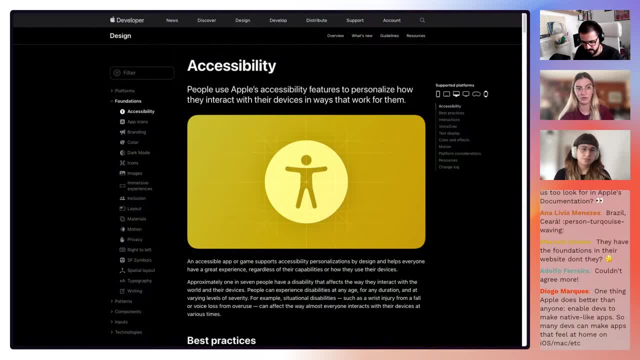 and, like the frame, it's so small that i don't feel like everything you actually do for one, uh, you can do it for another one, so for me that's a little bit weird the way they do it, of course. for example, maybe accessibility- that, of course, needs to be the key thing of a design system, and it doesn't matter if. 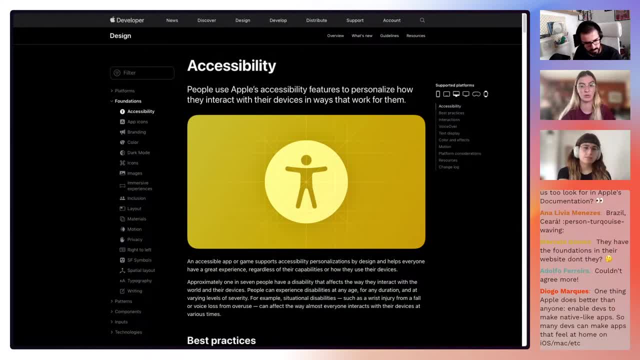 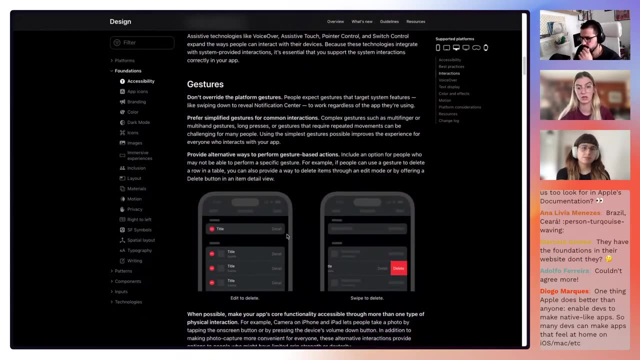 it's a car, if it's an apple watch or if it's a macbook, you need to have accessibility, but of course, accessibility on a mobile phone or on a macbook it's totally different. so the the sizes of the tax is different, the minimum that you can actually have, or the way you perceive colors on a 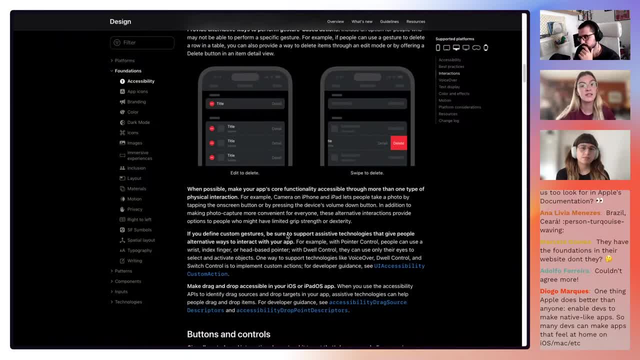 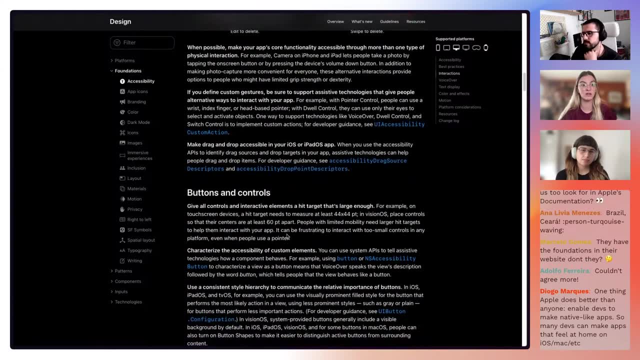 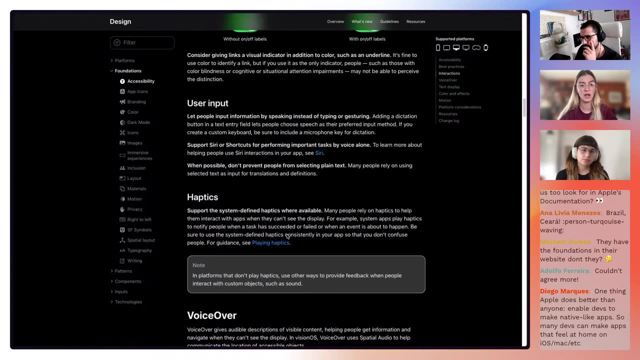 macbook or on a phone because of like the, the sun or an apple watch or whatever you're doing at that time. so i do feel like sometimes i mean, of course they're the best, um, that's undeniable. um, they have a lot of things, they have a lot of text, they have a lot of um great things to look at. but i do 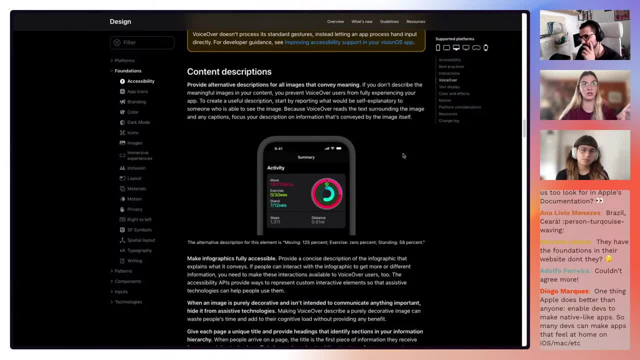 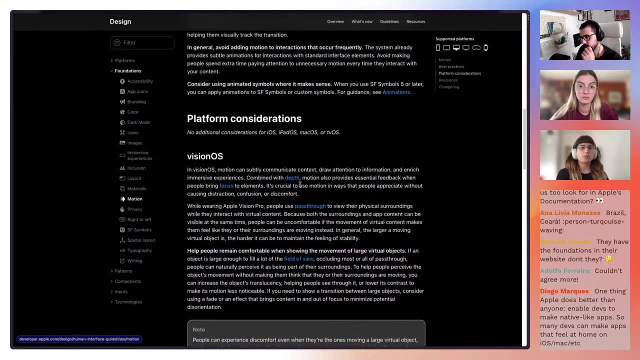 feel like they should be a little bit more careful on the different platforms that they have. uh, or maybe consistent with the things that they actually like a filter or something on youtube, i don't know like at glance the best solution. probably they do that for not consuming a lot of documentation for each. 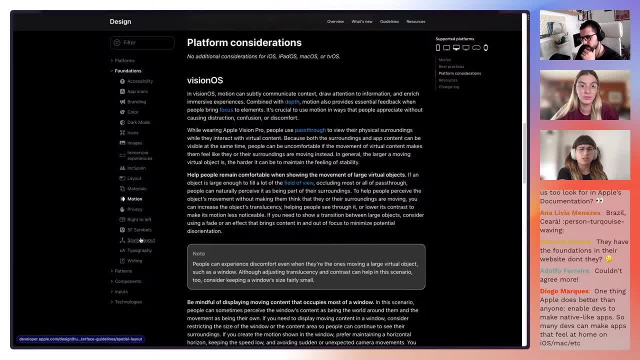 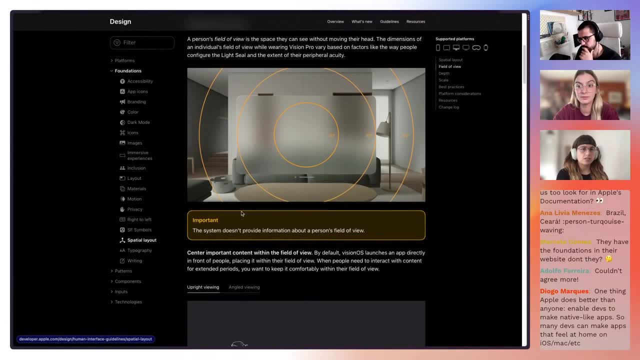 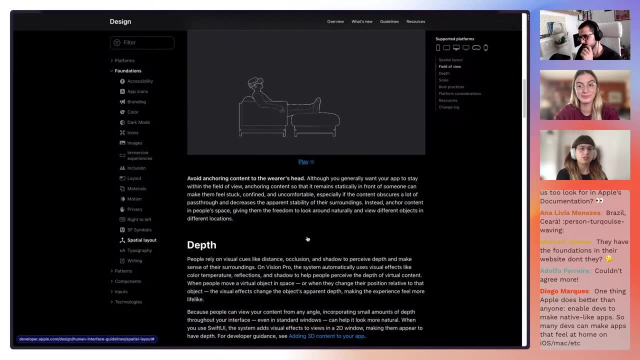 platform. so, because it's all this is also for a public statement. i believe that probably they have more doc, internal documents, for instance- and also i found it interesting accessibility to be the top, because they also, uh, launched a bunch of features regarding accessibility on the last year, so it's also, i think, a marketing position in there, but maybe, for instance, with icons, it could. 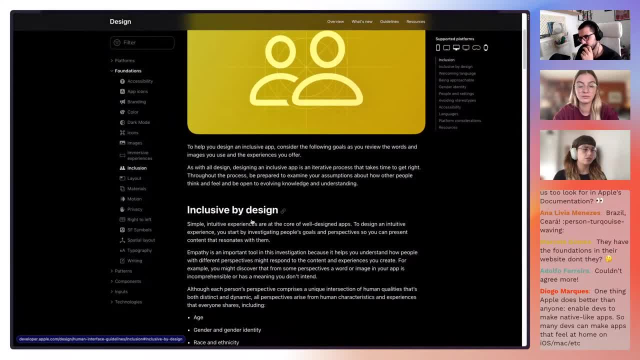 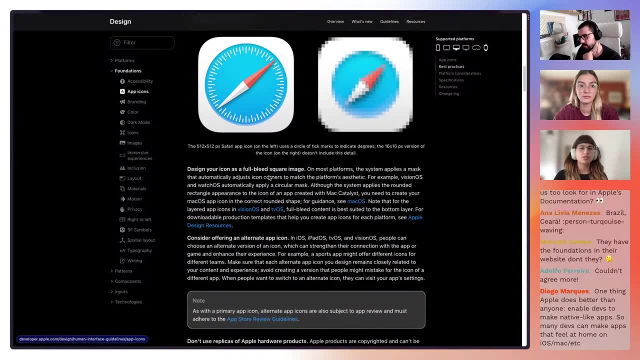 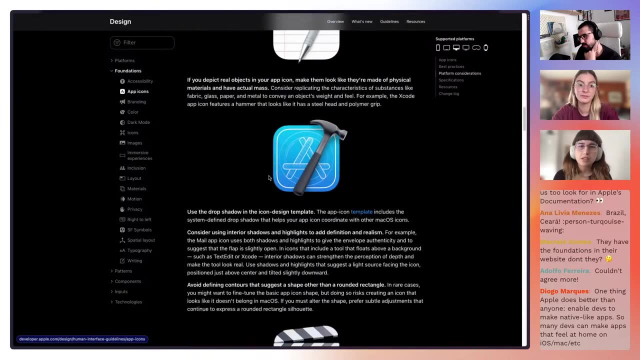 make sense to have overall pages because, regardless if it's a watch or a macbook or vision, you want the icons to be the same, for instance. so i i get their difficulty of uh dividing by each platform but at the same time having a common one, and that because you were exploring that filter on the right side. 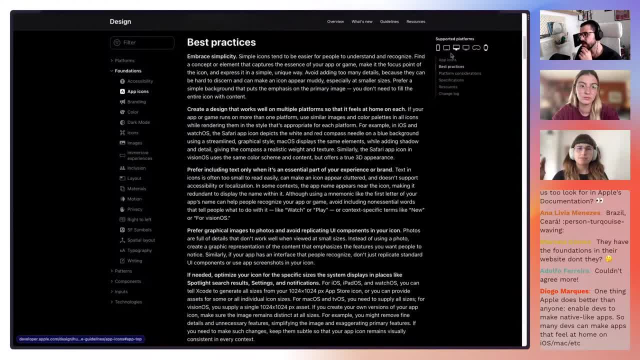 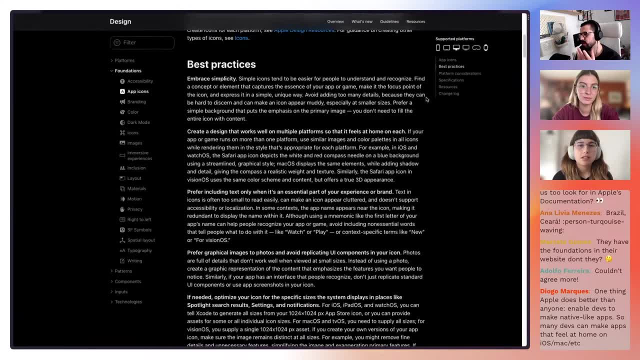 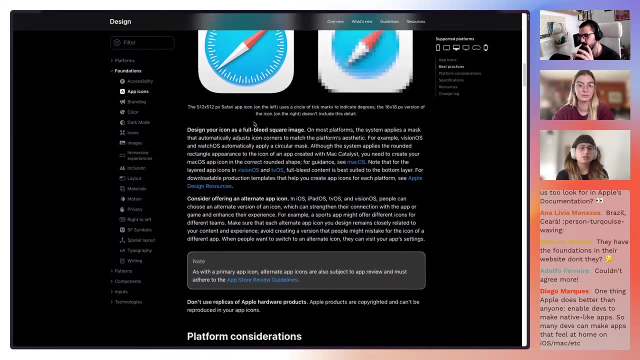 filter information: okay, for each one. this thing here is not clickable right the, the supported platform, okay, but it says. it says okay, like it gives you whatever platforms you're, you're supported in this area. so, on app icons, what you get is like best practices overall, and then starts to go into details on ios, ipad, on each one which macos. 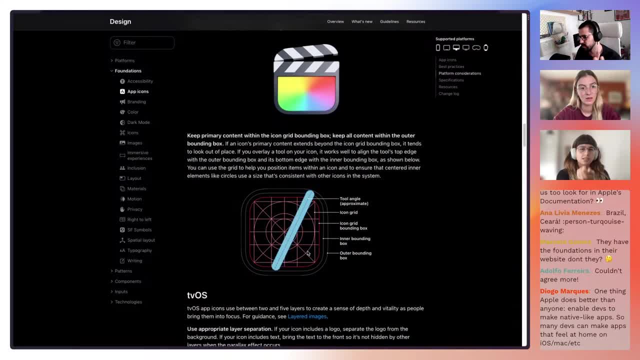 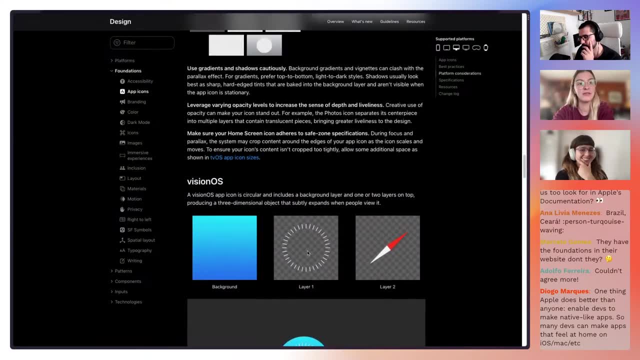 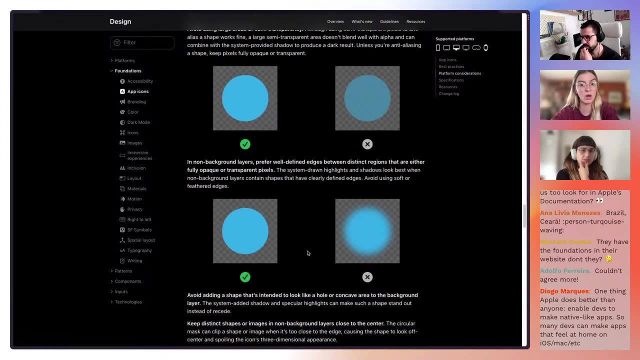 basically has this guideline with a tall angle thing. that is like i think they're still studying the options much to do that, like what happens if i want to design just for a smart watch, i would need to see everything from every other platform, which i don't want. like imagine i'm 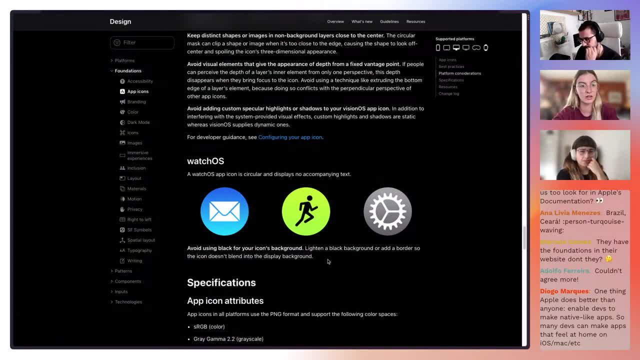 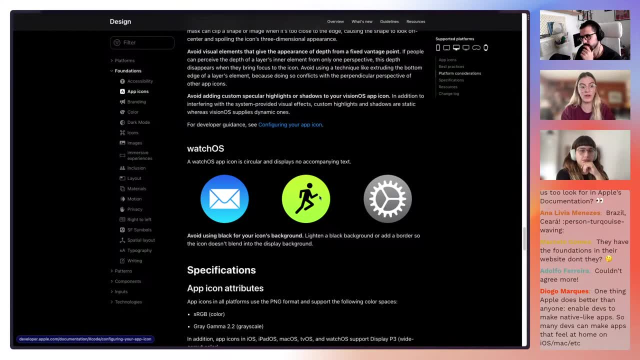 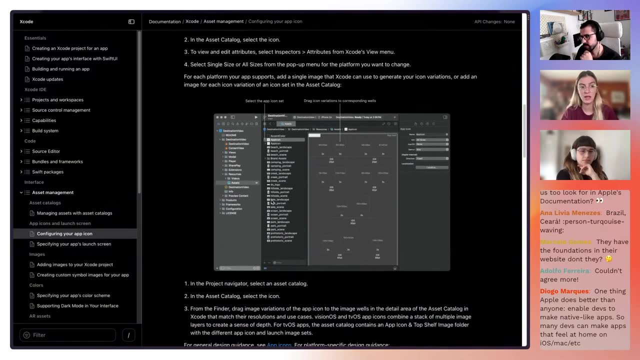 a designer apple, yeah, focuses on watches. like: why do i need to see everything for every single uh platform? um, it's not going to affect. it's not going to affect my job because i'm only working with one platform, so having that much content might distract you and 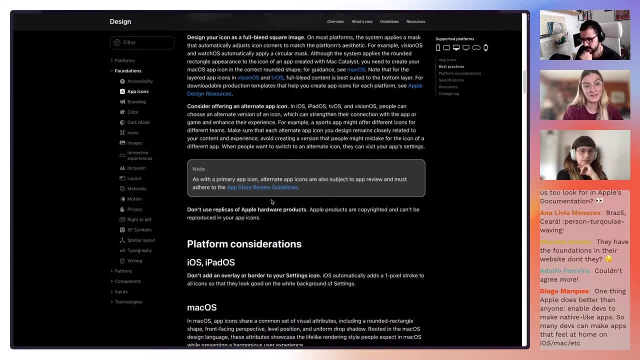 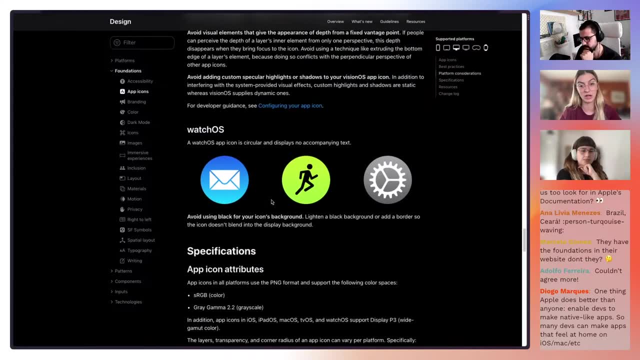 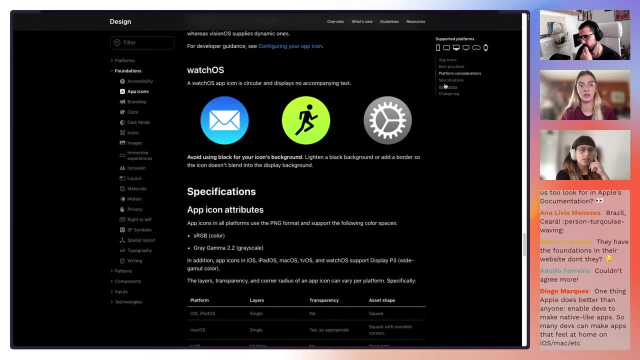 And maybe you see watchOS and maybe you're on the iOS part and you don't even realize that Maybe you're designing with things that are not correct. So that's why I do feel like they should have different pages for the different things that they have and be more consistent with that. 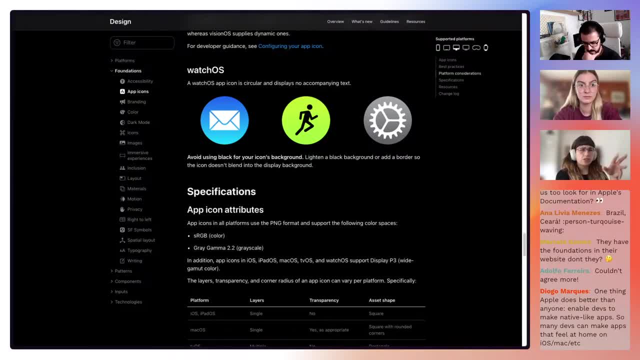 But like the way they have it now. maybe they are just exploring or even testing with us, For instance, but also maybe to educate you for the whole platform, So you can be like a guru on the topic, perhaps because they are very devoted to the design culture. 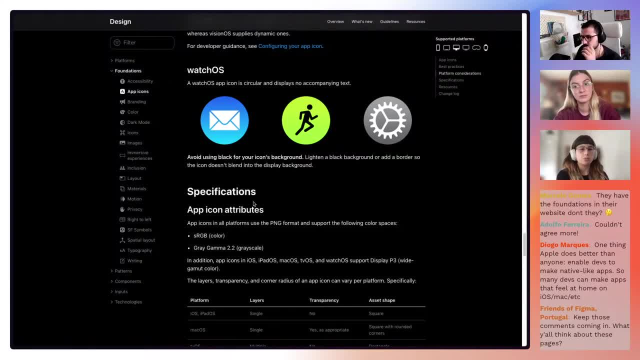 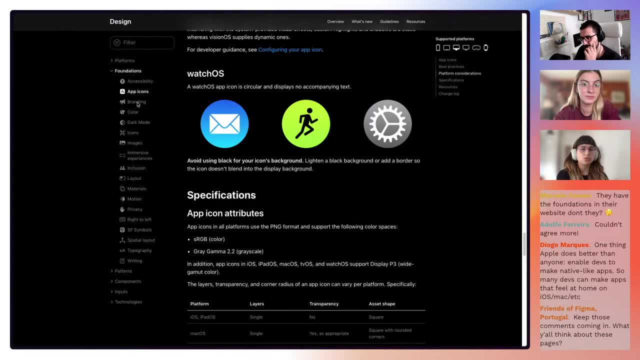 So perhaps when you're scrolling, you eventually also impact with the other platforms And in case you, you know, subconsciously you think, OK, this is consistent like this: I have to design today for watchOS, but maybe tomorrow I have to design for another one. 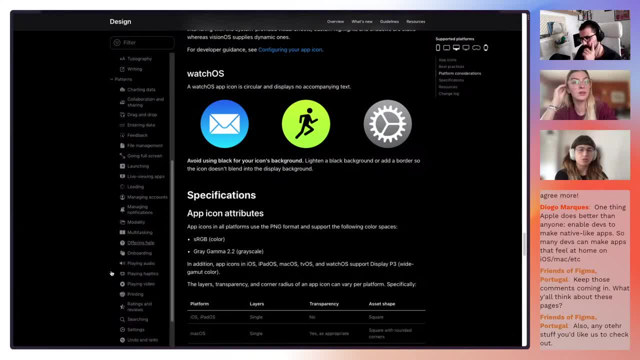 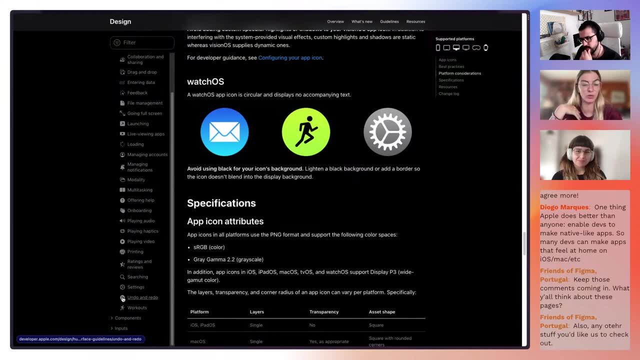 And you already have something in mind, But this is just a suspicion, of course, And it's not that efficient, as you were mentioned. It seems like no one- at least for me, on my point of view, and from what I've heard, almost no one- actually reads documentation honestly. 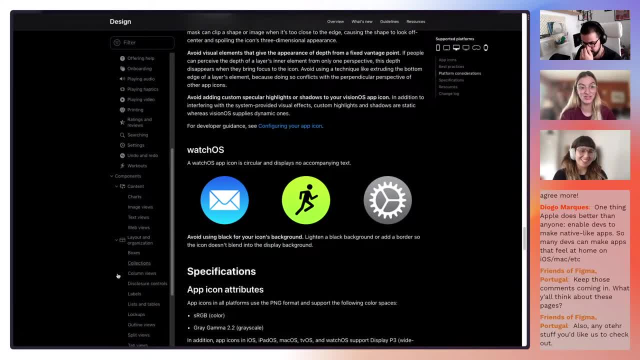 Yeah, yeah, yeah. So having so much text is just distracting. I mean, it is what it is, of course. I mean I do love to see the documentation, I do love to write documentation And I do love to see, like, all of the examples and everything. 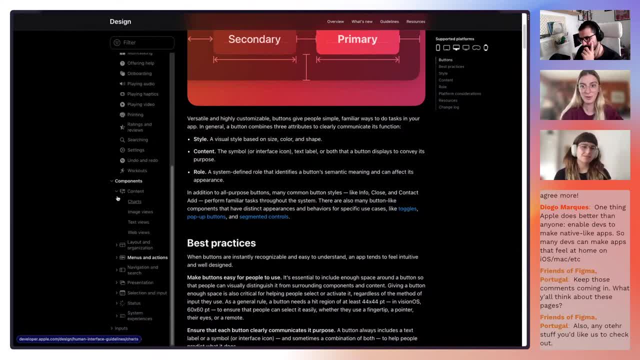 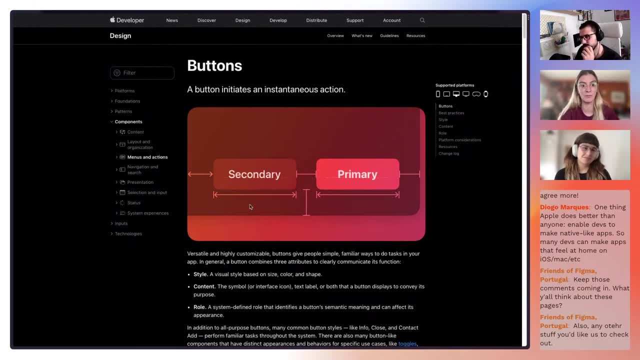 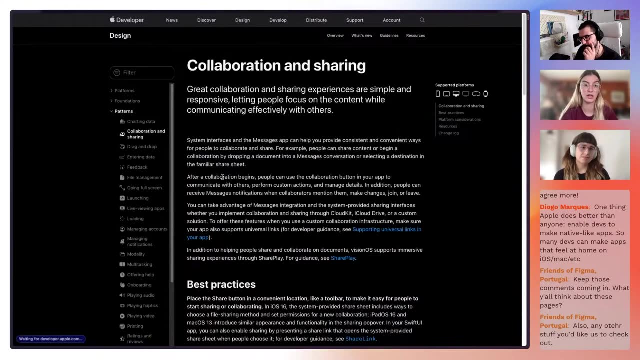 But do you actually read All of this page? You haven't just read the things that you want. So, as I was telling you before, having so much text it distracts me, at least, like a lot. There's just a lot of things that you can actually do with an example, with an image, which I do feel like it's lacking here. 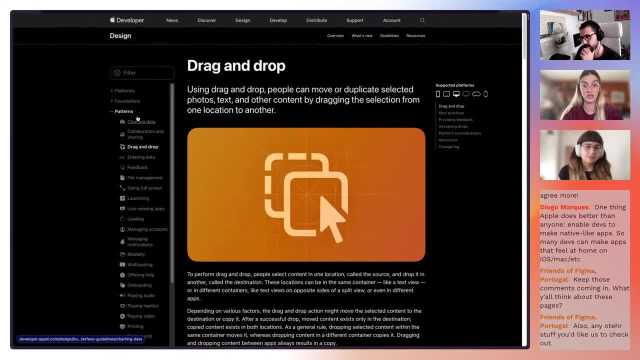 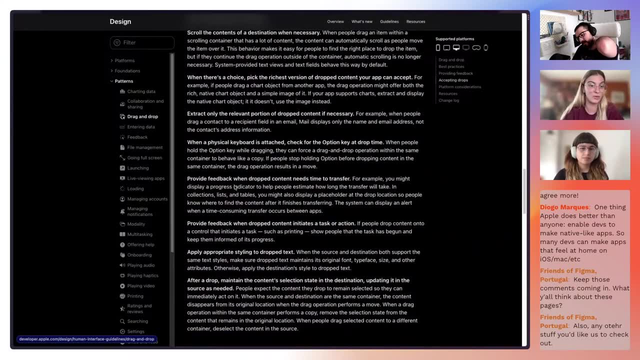 Like there's a lot of text here on this page that Brian is doing, but there is no example, real example. I mean, we're designers. What we do like to see is examples like things with our eyes. We don't like to read, or at least I don't usually read, documentation. 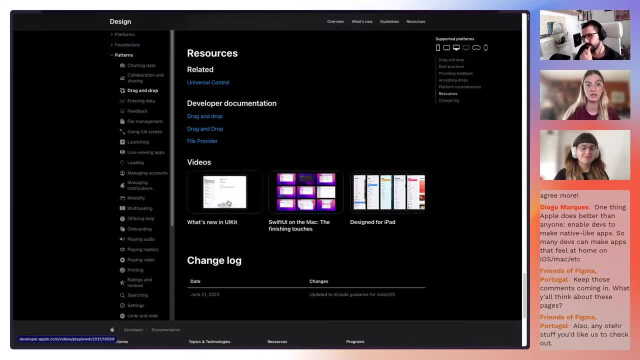 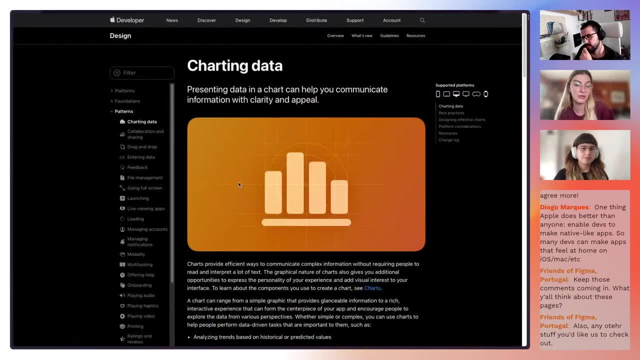 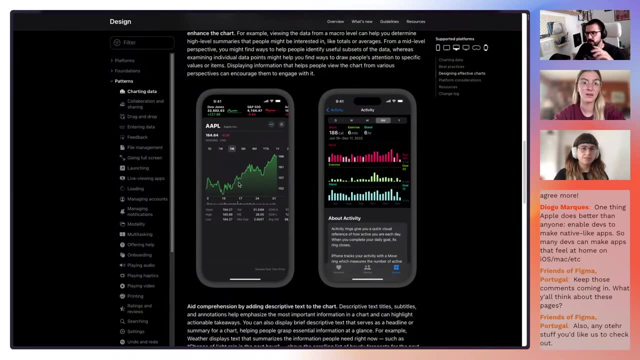 I just see the examples and I'm like, okay, fine, This is what I need to do. So I think it's lacking a lot of stuff that might not be the most user-friendly for designers. Yeah, it has some examples, but I think here's the kicker about the way that they do their documentation. 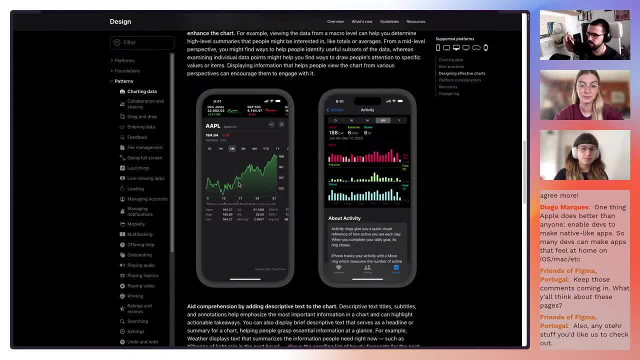 And this is something that I've lacked in my stuff but I've also seen lacking in others. So their way of setting up documentation is starting with platforms, as we've seen. Cool Just talking about what it takes to design for each one of these systems. 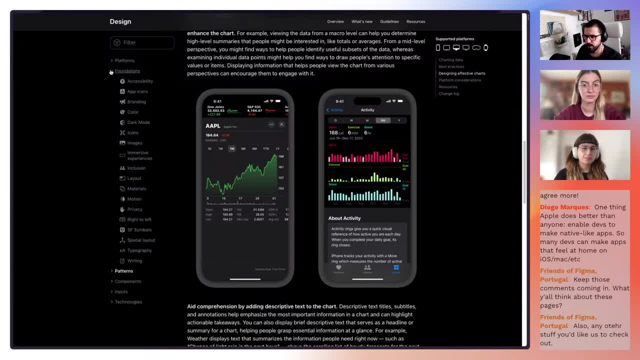 Interesting- Okay, Foundations, which most people do, but then they go to patterns first and then they go to components. A bunch of the companies and a bunch of the people that we work with- they don't have the patterns area. It's like components, and components basically include patterns. 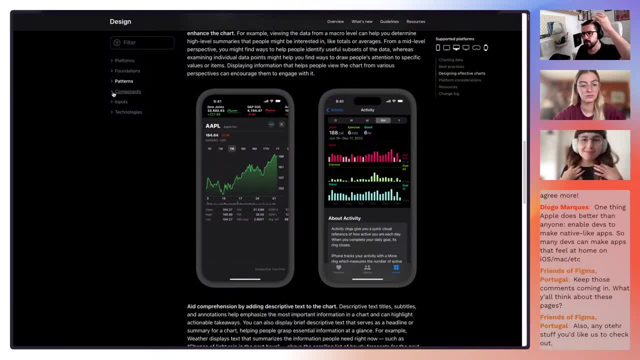 And then you go to either layouts or templates. Yeah, Templates, like there's no other thing, Like the technologies, the inputs, the type of stuff that they have here do feel like an higher level of consideration, which then might mean that, like when you look at the UI, it's not as perfect. 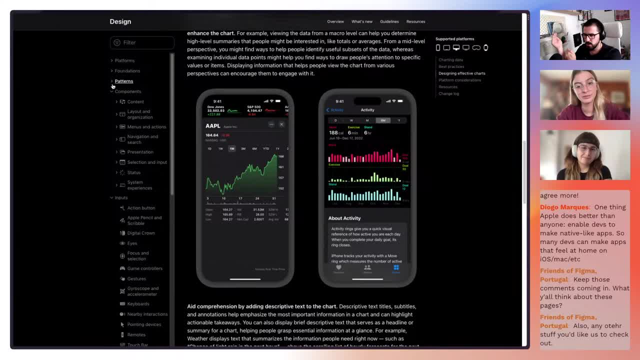 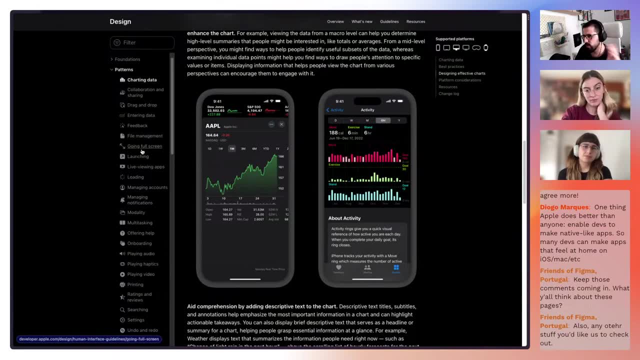 But if the pattern is the same, maybe it is what you're looking for. I think that's a good way of setting things up. It doesn't mean that it's perfect, but I actually like the way that they go through the logic of patterns first. 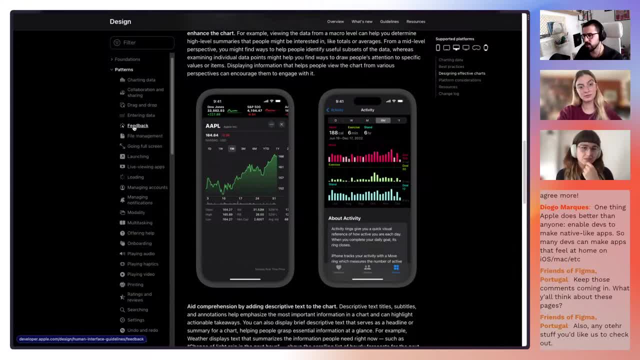 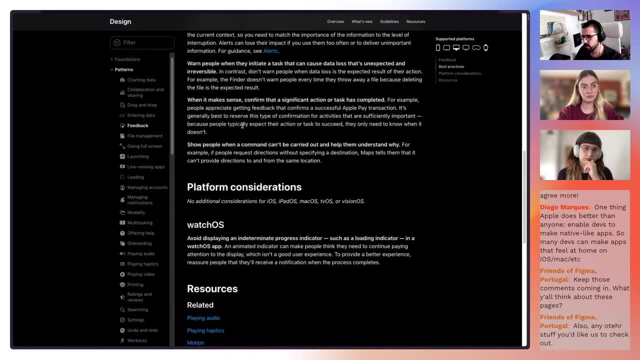 And that's why maybe there's too much content. The narratives, yeah, Like the content that you're looking for here, tells you more about the details, about patterns, but they can be overly descriptive on things like feedback, But they do have some things like videos and other related resources that might help. 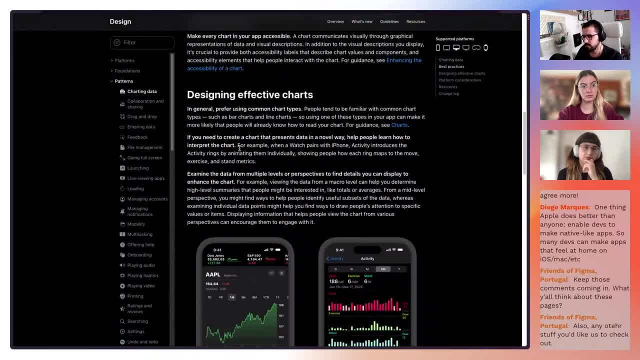 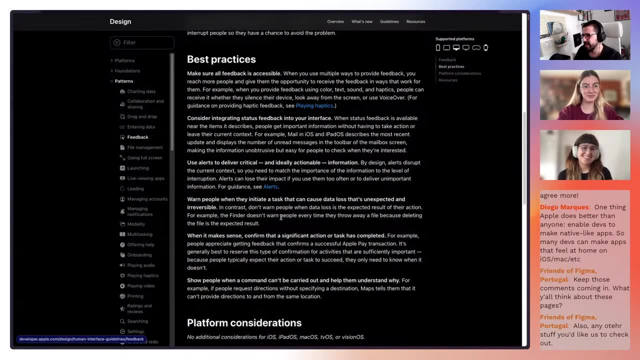 But yeah, like, for example, the data, one comes with an example because it's easy to talk about showing charts. But the moment about feedback, there's so many variables that I get, For example, one thing is Well, that's probably to showcase a video or anything to represent how Figma uses apptick feedback, for example. 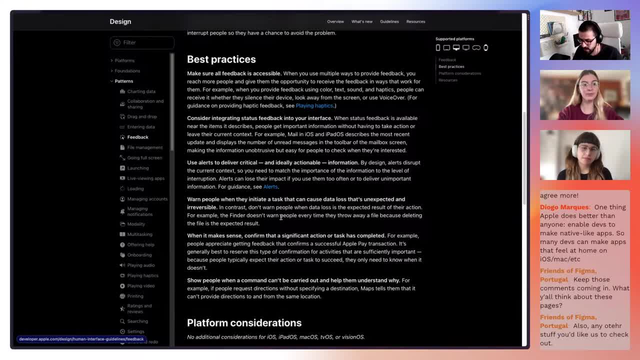 I don't know if you guys noticed, but they introduced that right When you're using, if you have an M1, M2 MacBook or anything that has an apptick feedback on the trackpad. it is amazing to just click on things on Figma now whenever you know, and then you're dragging them and you're literally dragging and feeling it going like it feels like you're pushing your finger against the surface. 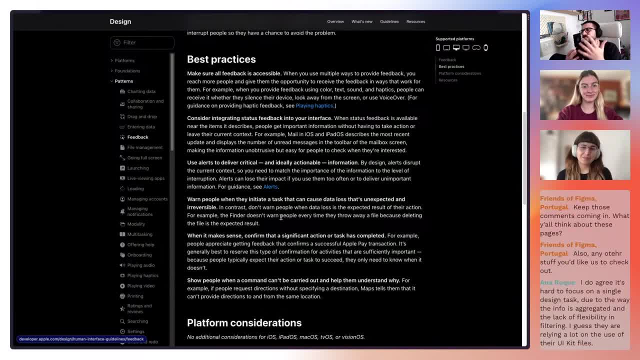 And it's fun, Like is it something that it's? It's really necessary for us to do our job And we know I'm like most of my days I'm just end on mouse and not actually on the appticks. 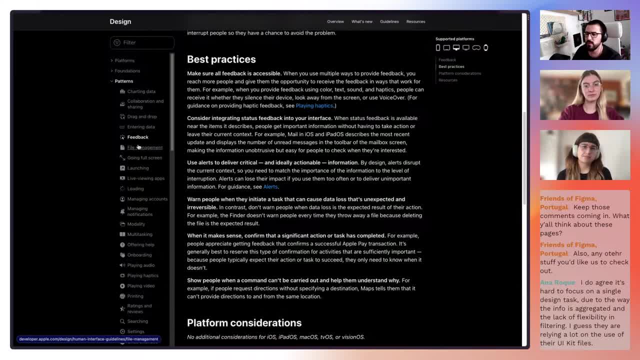 But I love the detail, because the logic of like feedback is very interesting And Apple thinks about it in a way that many times I don't feel like other companies think as much. Yeah, Again, it's the resources at the end of the day, right. 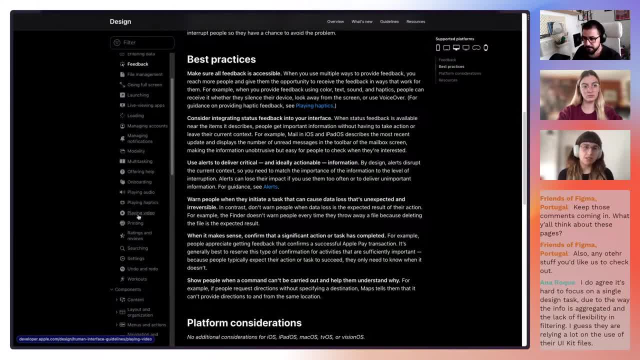 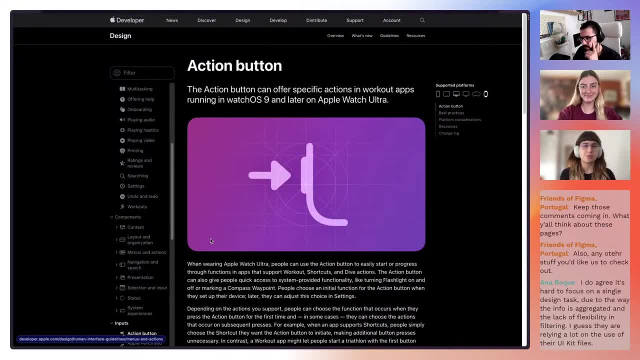 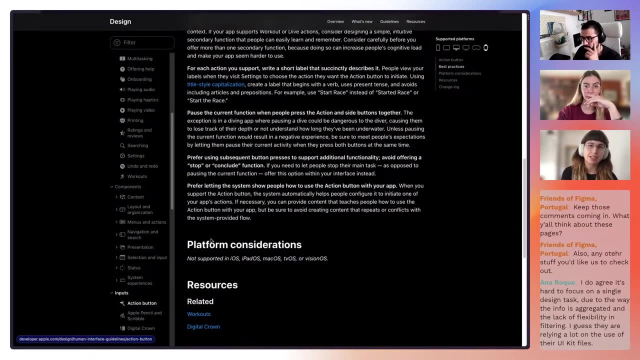 Like they have the resources that many don't have. Yeah, And I really give a big kudos to them that they have the luxury like the power to create patterns, Because I think that's the most utopic things when it comes to design system: when they are so mature that you can actually document a pattern. 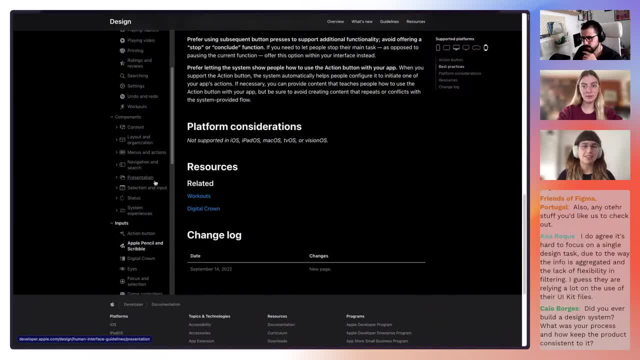 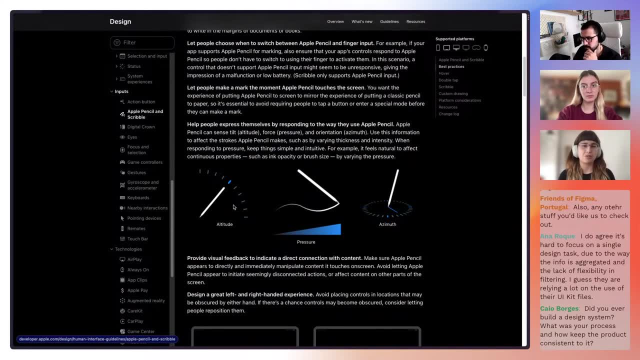 At least for me, it's like a huge accomplishment, Like, oh, I can patternize how people all around the company do a certain behavior. So of course there would be like the fathers of that matter. But yeah, I read a little bit with Bia. 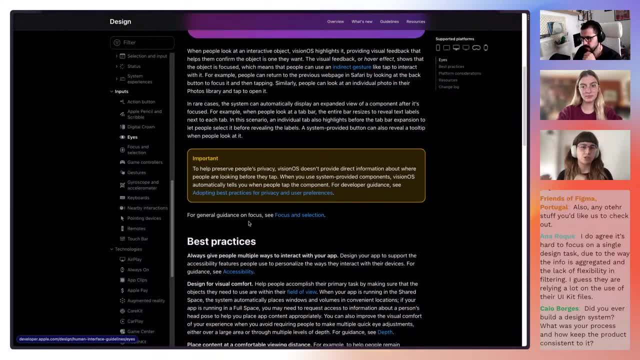 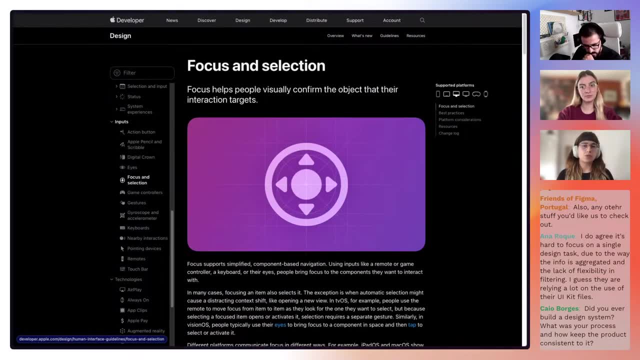 Maybe they can do a little bit. you know a mix of documentation, but also have more images and more videos for the more Lazy ones. Maybe documentation could be good when you're talking to a more dev or management wise to justify why things are done in that way. 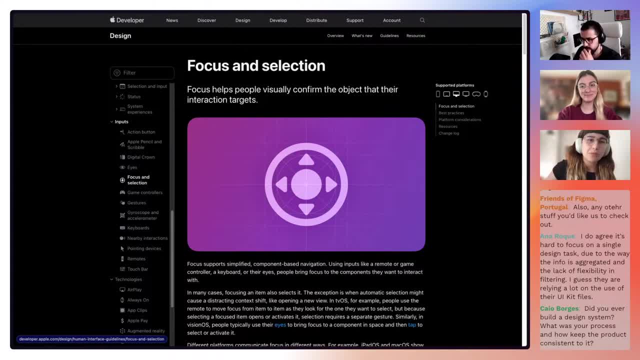 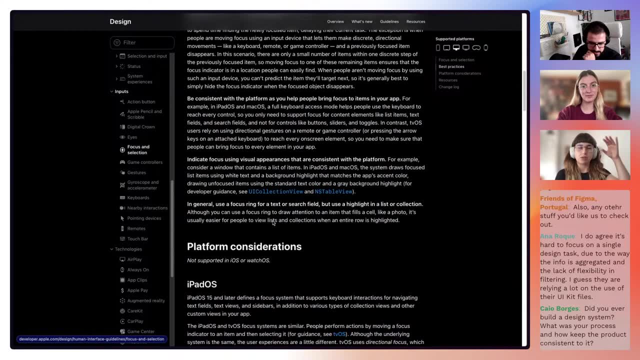 Like people that read more, let's say So. maybe they can do a mix a bit of the both worlds, because for sure I think they will have examples. But yeah, I also really like the way that they put it. So patterns came first. 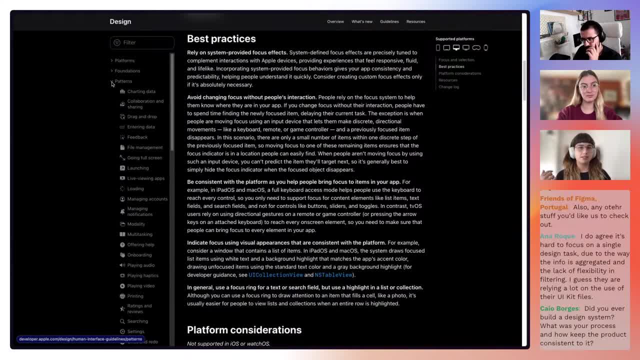 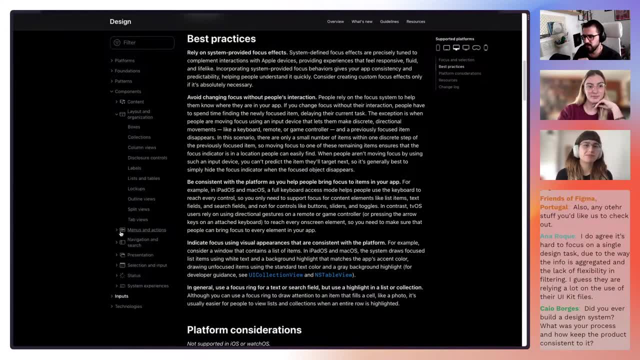 You have to understand what you want to design and how, and then then you have the components to do it. For me, it's really amazing, Yeah, That's why I was basically just going down and trying to figure out where things were. Yeah. 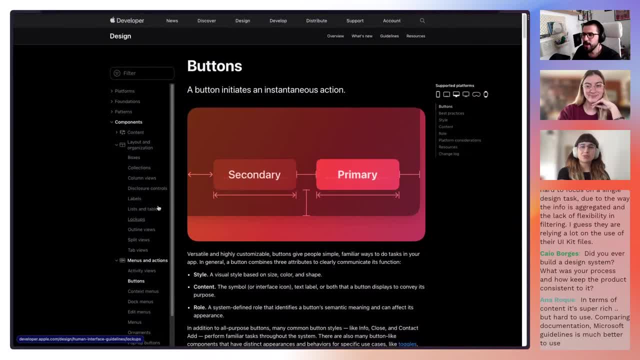 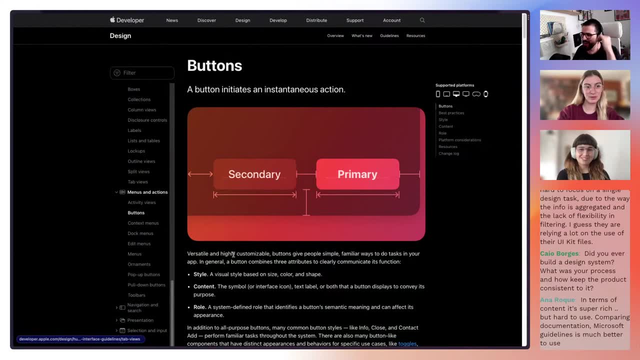 Because like buttons, usually like top item- Yeah Yeah, That's the most cliche, right. Like: oh, look how low this is. If you start opening these things, look how low buttons are on the system, which is like everyone on Figma starts by designing buttons and things like that. 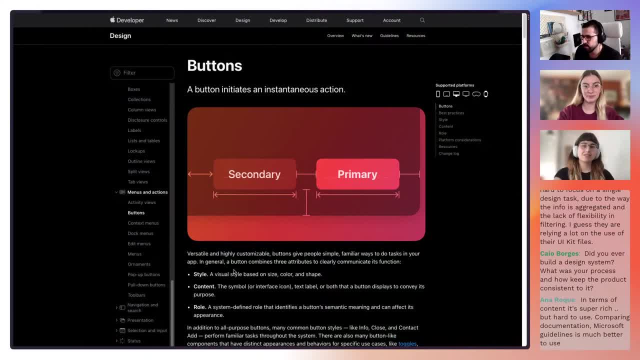 And again it is like UI wise. It is fun to start with this because it feels like very much of a primary add-on to a bunch of UIs, But at the end of the day, everything else above feels more important if you think about it on the long term. 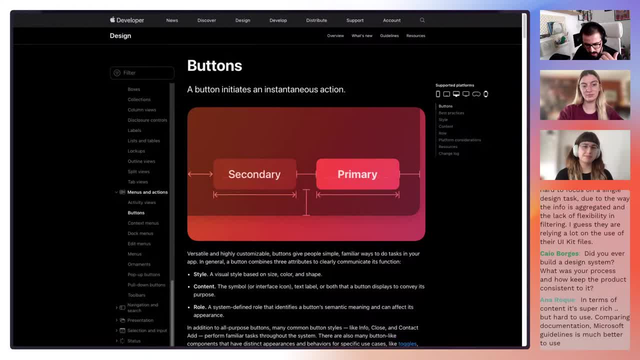 And on that end, I think that's a really interesting thing. By the way, Anna Hawke said that she does agree that this is hard to focus because of the way the information is aggregated, And I guess they are relying a lot on the use of their UIKit files, which we'll be looking in a second, because we've been looking at this website for a while now. 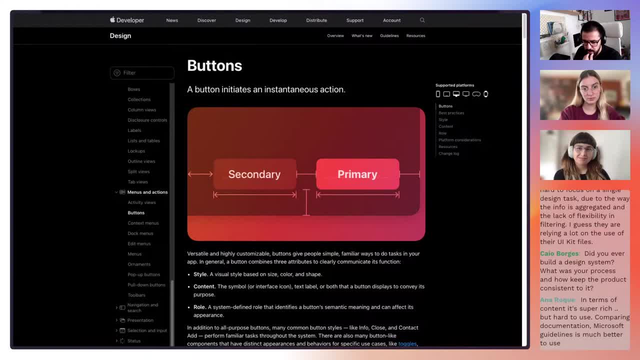 Caio Borges did ask us if we have built a design system and what was the process and what was our process, And what was the process and how. what was our process And how? what was our process And how? what was our process? 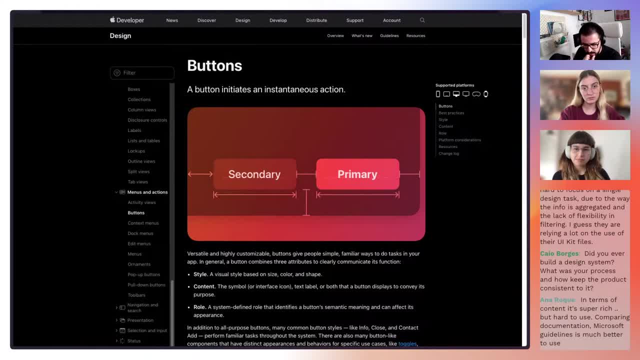 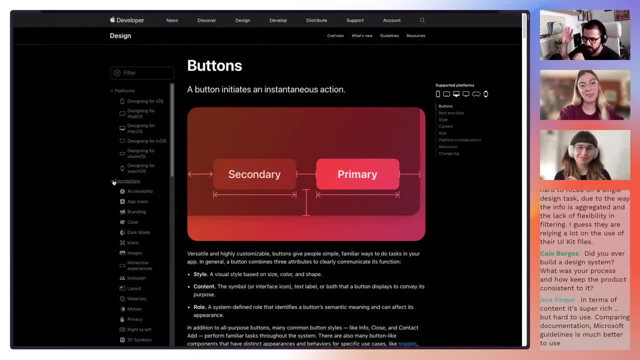 But I think, I don't know. I built a design system. I'm probably on the V3 or V4 of our design system. We're overhauling it again because we did the rebranding, So we're literally just starting back from scratch on a lot of things. 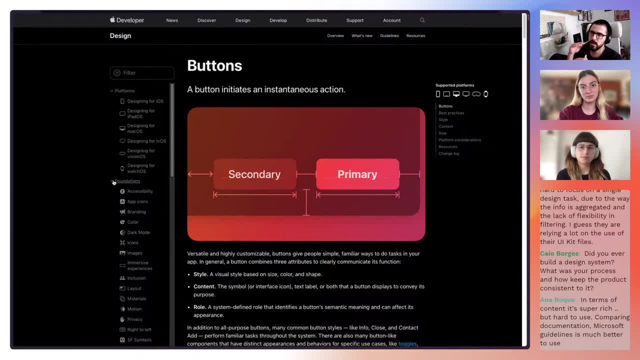 So we're attacking our design system, for example, right now, not on just a system-based level, but on a brand-led level. We're talking about brand system, So the design acts with the brand in mind, but user experience is always a layer on top. 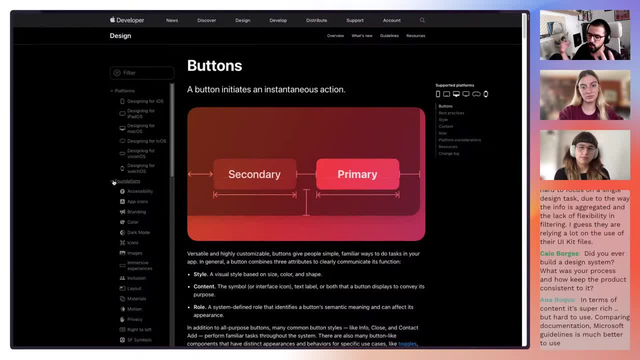 So it allows us to use a design system not just for UIs, but also for communication, for the way that we build our stuff on every level. So that's, for us, was the way that we managed to start getting consistency. It was like we created some pillars, including accessibility and usability, pillars that are set on the top of our brand system. 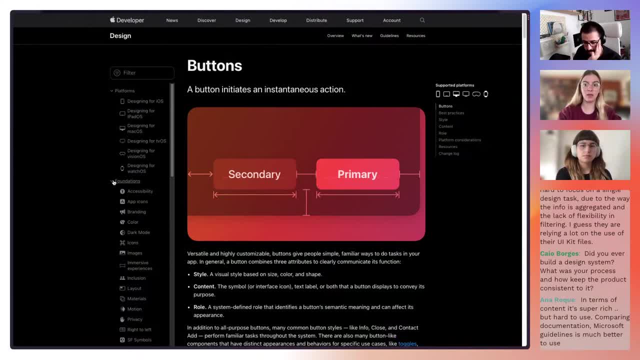 And then we're building from that now, Which is, I think, interesting. I do feel like, for example, there's not a perfect design system, And you always like to start with first a set of foundations and then you do the components and then you do the documentation. 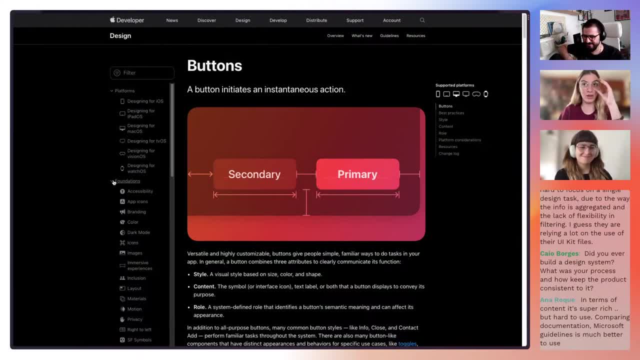 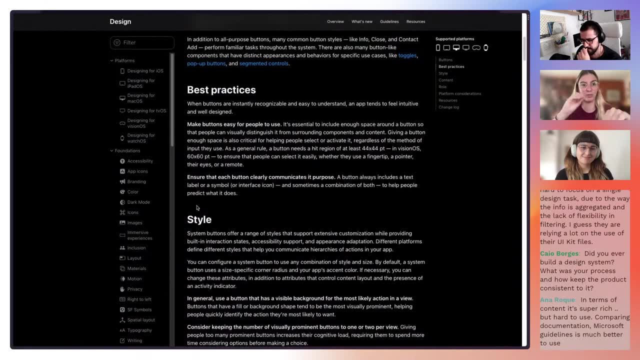 But that's not the real thing. You just start with components because you have the platform done, So you just take all the components. you have all of the buttons. Maybe you do an audit and see that, oh shit, there's like 50 different buttons. 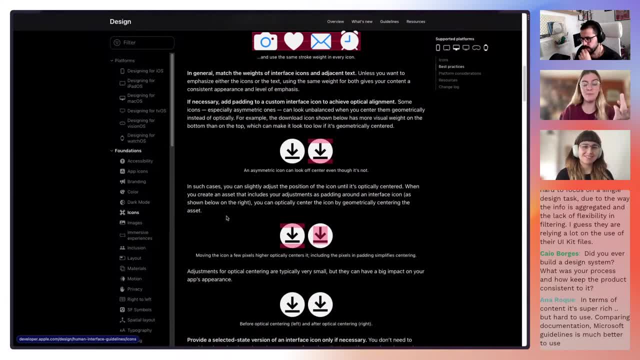 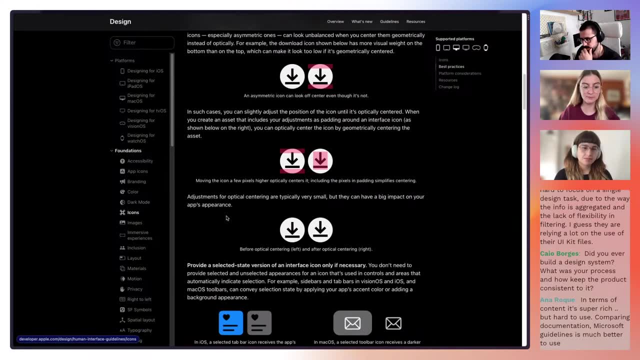 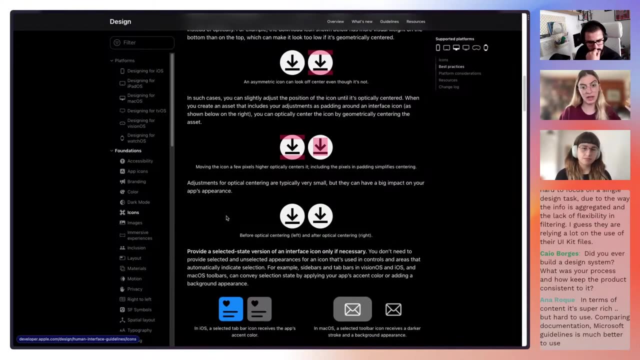 So I need to reduce them all to only three. And that is when you start doing the foundations. At least, that was my case. We had all the components, We had all of the colors that we were using on the components And then we were like, okay, we need to expand that a lot. 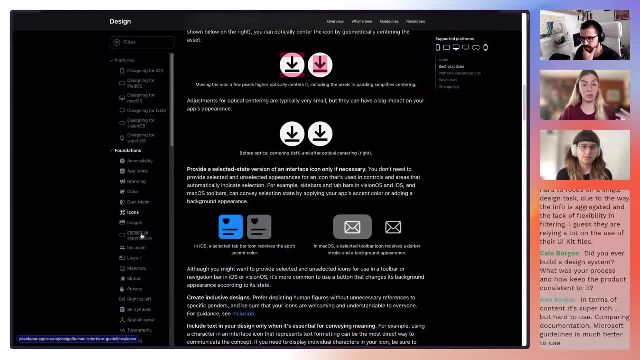 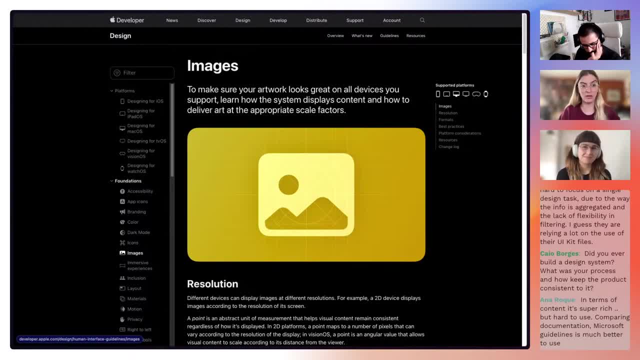 It's not always a perfect. It's not always a perfect. It's not always a perfect way of working with that. And now we're doing the tokens, which we would have done at the beginning of the design system or when we had the components, for example, or when we had the foundations. 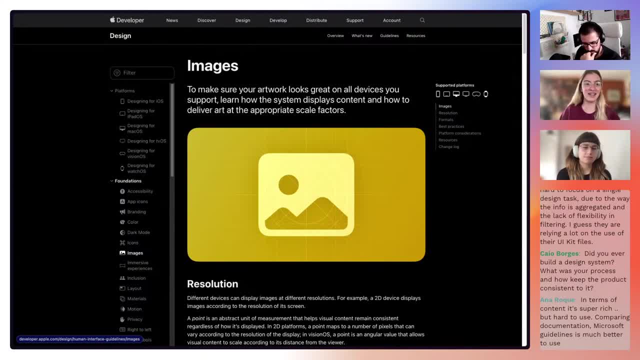 The documentation is something that it's a little bit hard because there's a lot of things, There's a lot of frames that you need to take a look at and put examples or ways to use that component. So, I think, keeping the product consistent. 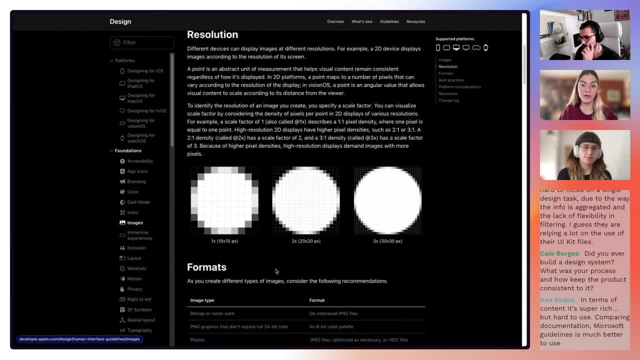 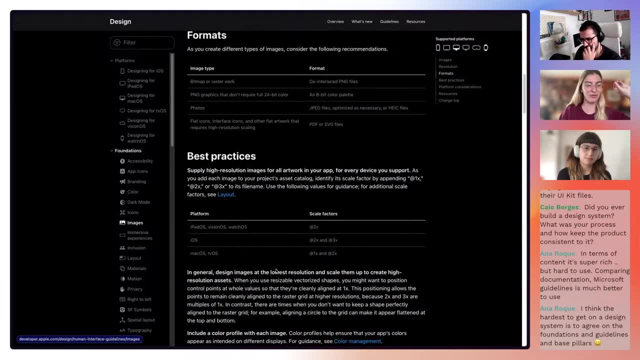 That's the. that's the most important part and also the hardest one, because there's a lot of things, Like when you have a product already released. you'll see that you'll have a frame that has a button that it's- I don't know, maybe gray, and you don't have grays on your palette. 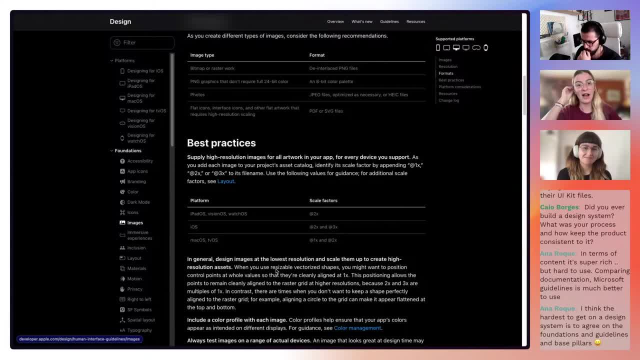 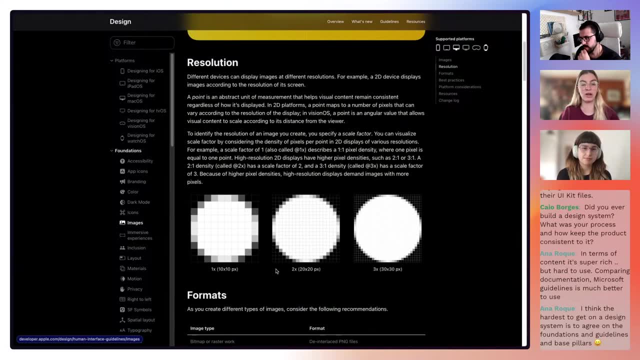 And you're like: why is this happening? So it's sad. Consistency is a little bit hard to have, But I guess when you have all of the design system and when you're You're like you're all of the money that you spend on the design system. 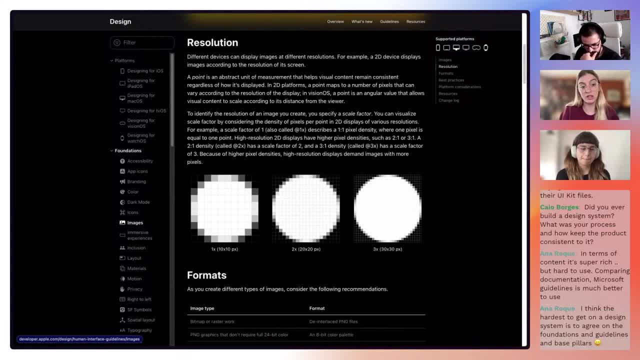 system, um, ends up getting you results. that's where you see that, okay, this is a product, that it is consistent, um, we're using all the things that we want. and then it's just: you need to rebrand or do new components or do a lot more stuff. basically, yeah, definitely and yeah from. 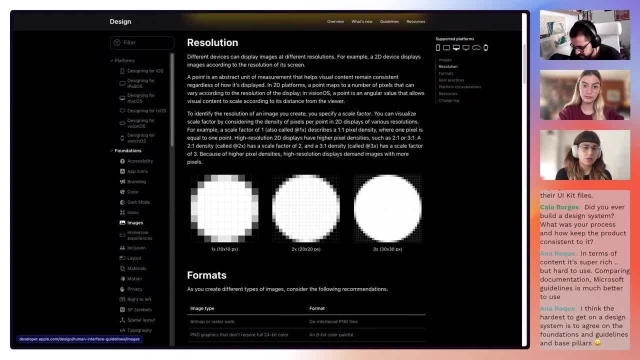 my side, i can just recommend one or two quick advices. so, as we were saying, i launched one in march, a new one and what i would recommend to you, in case that's your scenario, to do design audits so the products are released, so you can create consistent and mostly a realistic backlog for your 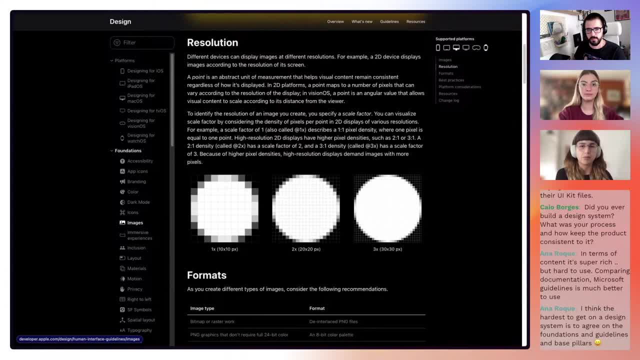 components, not just you like- oh, i just download the ui kit and i'm ready to go- and then, with the documentation, try to also document the real use cases and then, in case something shows up new, you add it to the documentation and also try to create a structure that reflects the way your company is. 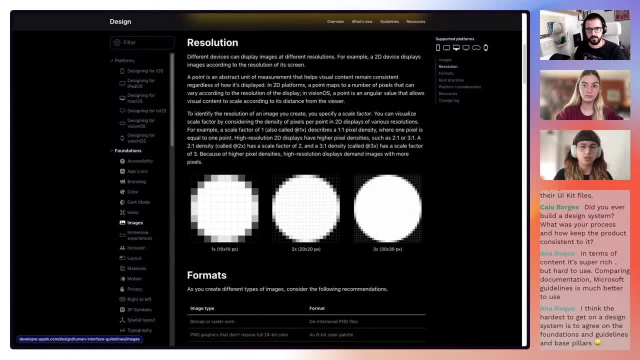 it's also important. uh, of course you can have inspiration on the internet, but just keep it in mind that the design system should also helps how the company should move forward. um, and yeah, basically that's the two and two tips, tips. this is also another conversation that we already have. 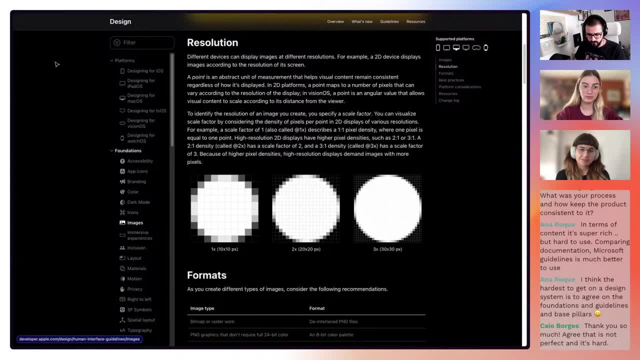 depending on um, on what you end up creating. honestly, even the language can be very different from companies to company, because many times people prefer like internal language. right, like, yeah, yeah, it's easier for us to communicate with internal language when then we jump into these files as external facing. 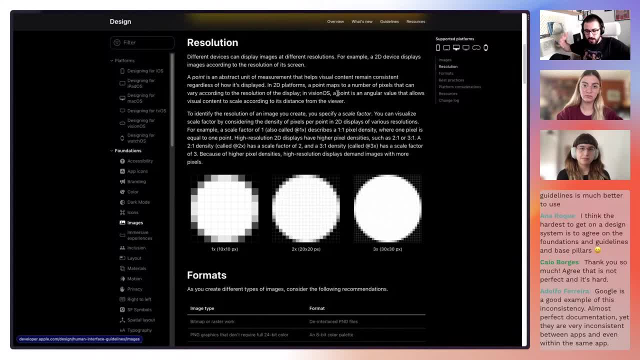 people, like we're looking at their, trying to understand their culture, their way of working. yeah, yeah, yeah, yeah, we saw, we seen it like it when two or three different files that we found before, right, we saw that we, we saw that these things are very different from. 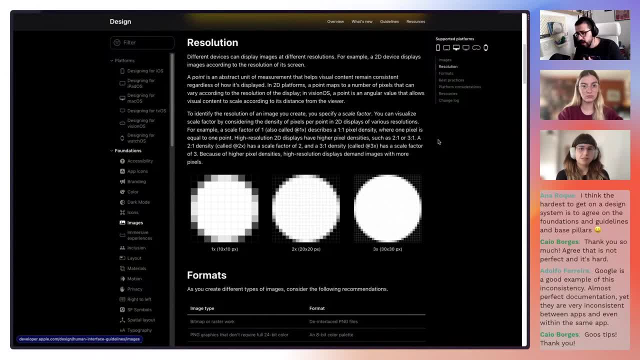 company to company, and apple is not different in that way. um, but one thing that i think is really important is really important for us to get to the, the design system, and how can we do that and how can we get it in a way that is more. 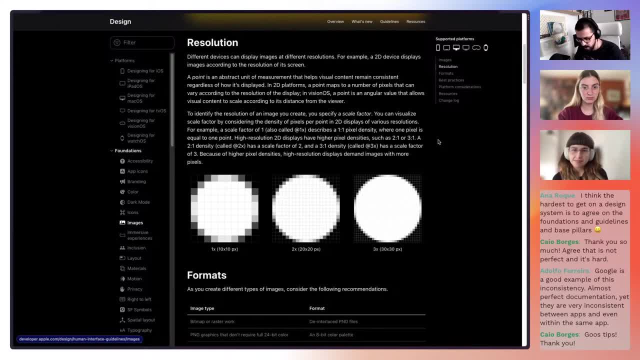 uh, open and more open and a more open, you know, and open to the public and to the people. yeah, i think that's a really good point and i think, you know, i think it's really important to get into the figma files, because we really need to get there. by the way, um, just looking at 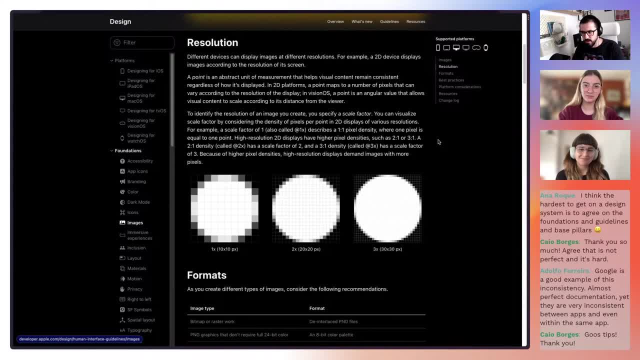 That's also why usually it's easier to do that type of solutions when it's not a group decision like too many people in the room. It can be a group decision, yes, But if you have the decision by committee on a design system, it's a great way to also start having a lot of issues. 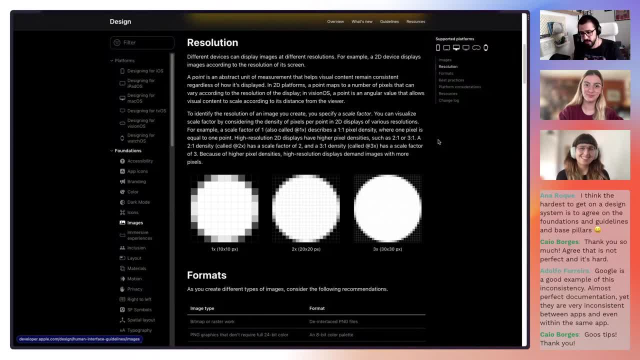 So great inputs from everyone, but make sure that the decisions are centralized into whatever people have to deal with or handle the documents For sure. And then we also have Adolfo saying that Google isn't a good example of inconsistency. Almost perfect documentation, yet they are very inconsistent between apps and even within the same app. 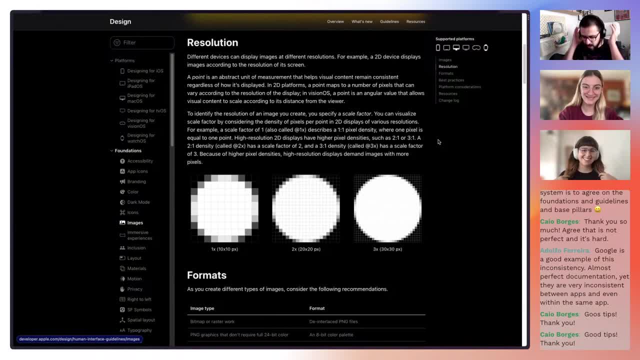 Let's not bring Gmail to the chat. please, The four blues, not again, not again. One last thing on Apple's documentation, but I think this is actually one of the best things that they ever did is the way that they handle sizes. 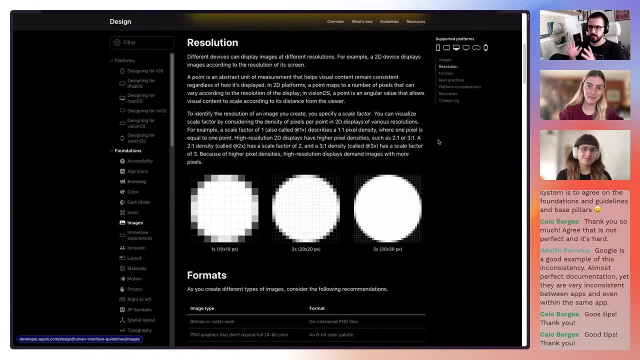 Just because they don't use final pixel dimensions. they use a point system, which is great and not great, But I still feel like it's. It's a better way to scale up things, because they use baseline logic of resolutions And this is a side-by-side. 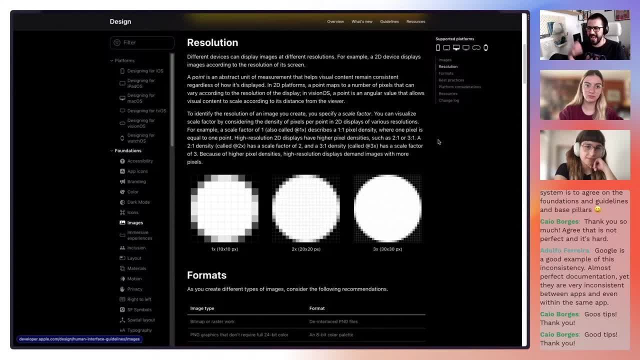 This happened. well, because it's a technology thing that they did. They didn't add new pixels to the screen, They created a technology that duplicates or triplicates pixels, So their baseline resolution is always the same base of points. So you design for an iPhone on half the resolution or three times or a third of the resolution. 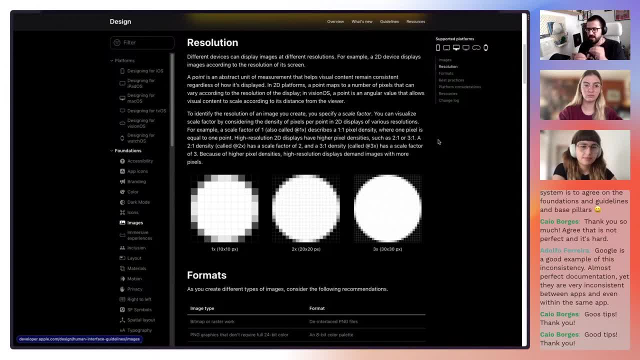 But since they are all based on the same point system, the dimensions, It's kind of scaled very well between screens because it's like the point system is based on the physical size of their screens, which is interesting, I think, While Androids are not the other end. 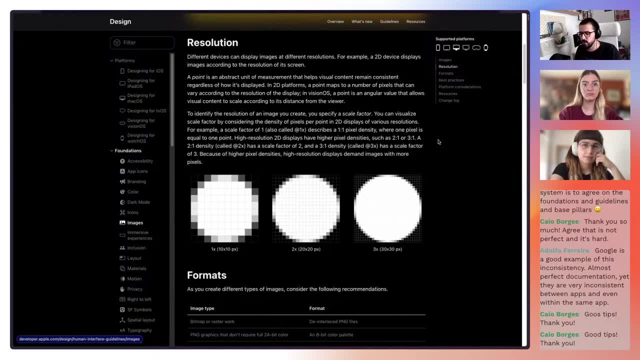 A lot of companies, a lot of systems. they go by resolution. So, like a 16-point font, we design with pixels, So we would be designing with. Instead of a 16-pixel font, we would be designing with a 32-pixel font. 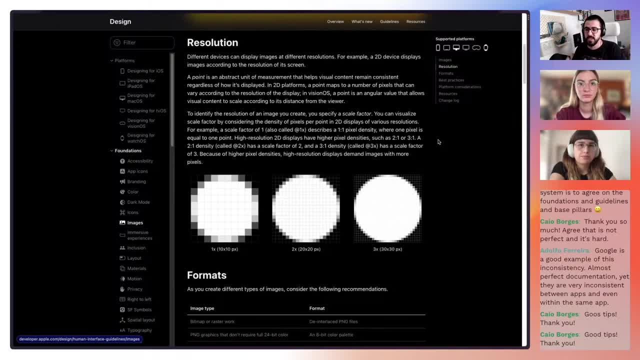 And it creates weird stuff, And that is very consistent. It helps us, designers at least, and developers too, to scale better, because they multiply things. They do a very great work on that. Now Androids has that too, with the resolution things. 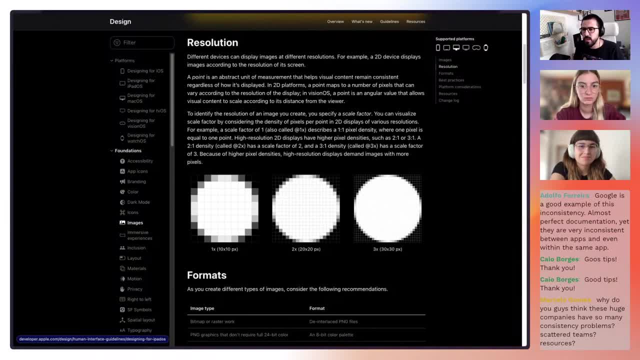 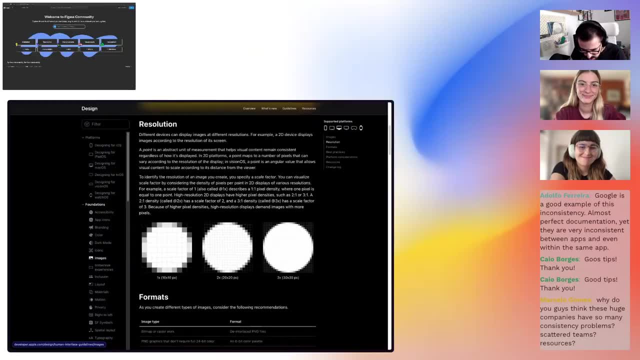 But yeah, it's interesting. Okay, We really need to jump to Figma because we're already on 45 minutes of stream, So I'm just going to jump here to Figma. Marcelo is asking: why do we think that these huge companies have so many consistency problems? 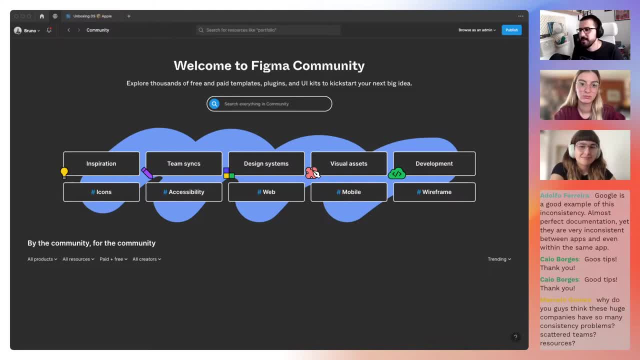 Are there teams resources? You answered yourself, man. Like that's exactly it, At least in my opinion. UX maturity as well. on the company. Like maybe design is still a cliche. Like what is UX, What is UI? 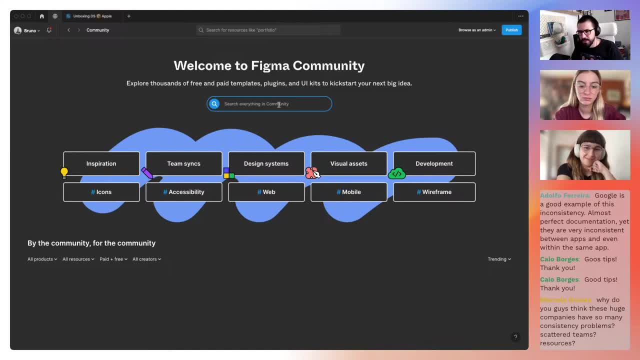 Maybe they do what some people in my company do, which is they come and like: where are the guys that do the drawings? Yeah, that does the screens. Ugh, Yeah, Such a cliche. It's a type of stuff. 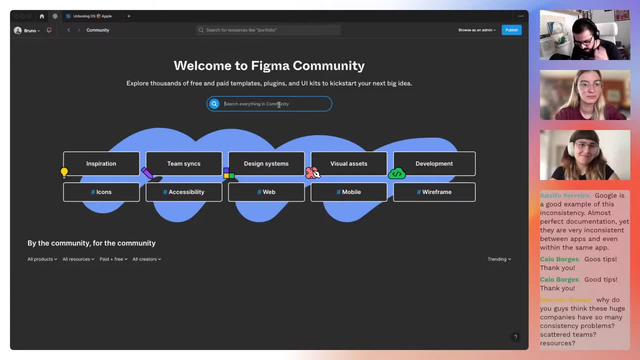 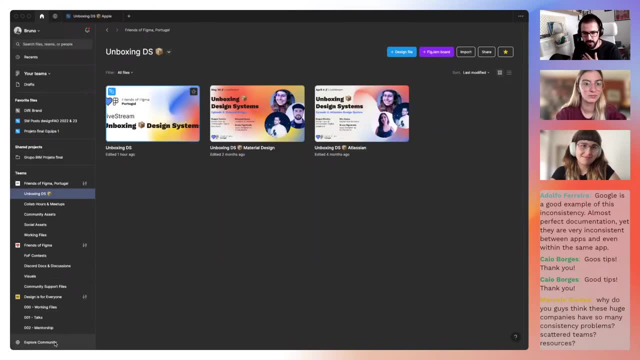 Okay, Yeah, Let's do this, as every other user would. If you want to find All documents in the community, you go to Figma. You look for the community tab that now is available here on the bottom. Or if you click on your profile, there's also here the thing that says community profile. 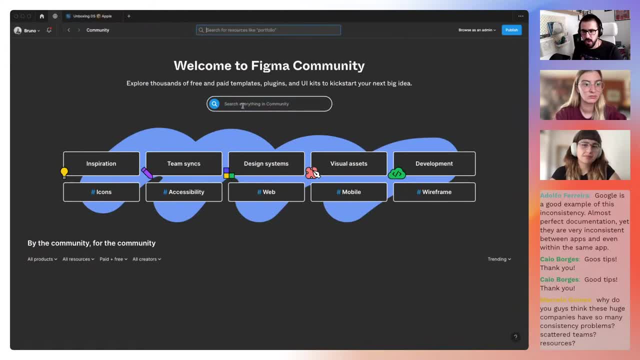 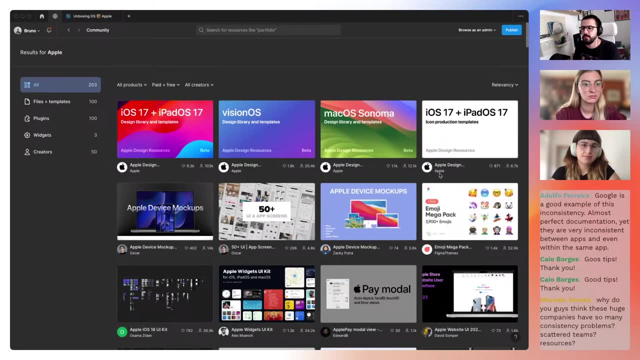 Takes you to the community, And then you can search over here on the top or on the homepage of the community- Search for Apple. You're going to get all the things, But usually the top elements are immediately from them, because they also are some of the most duplicated documents. 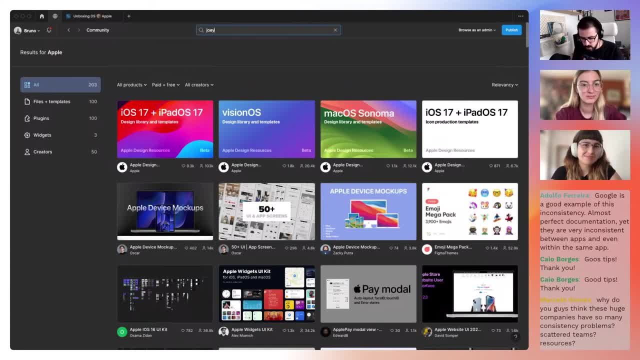 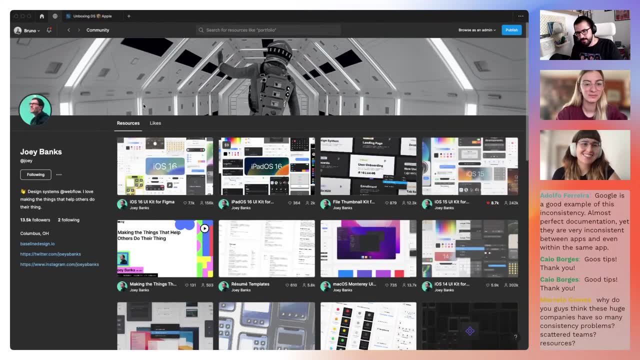 And because it needs to be saved, I'm just going to drop this gentleman here. Of course, We need to thank Joey for being the guy that made all the Apple systems before Apple did it, So bowing to the master. I don't know how this guy had the patience to do it, but he did an amazing job of bringing these systems to life. 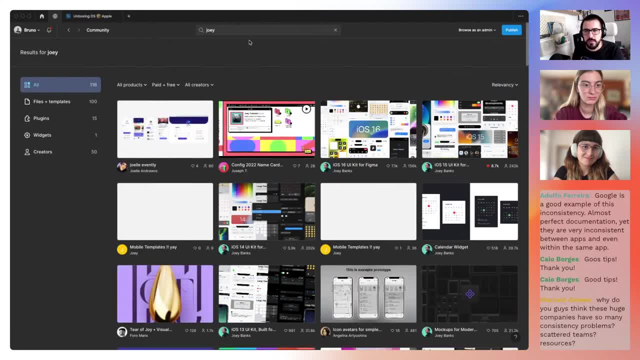 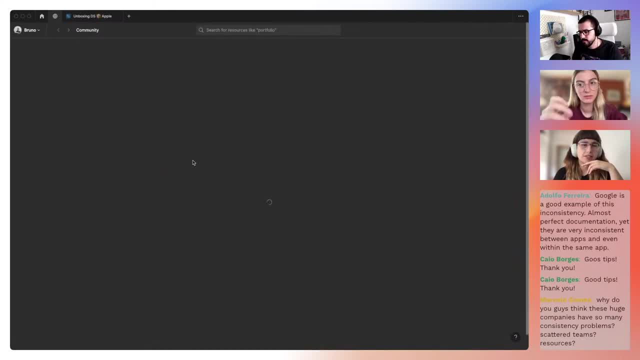 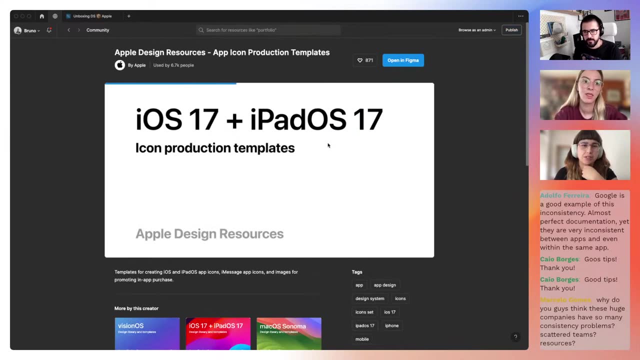 But yeah, let's look for Apple really fast. Yeah, I didn't put the Mac OS in our unboxing file, but maybe we can just see the pages, the preview, because I don't think most of people actually do that before open and Figma. 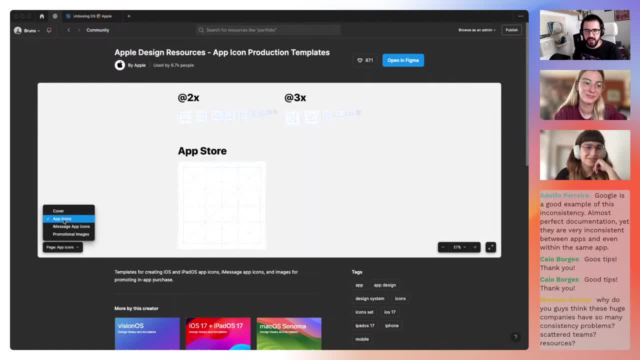 So, yeah, so they have a couple of different files, but they never call it like the scientists and files or anything like that. Yeah, libraries and templates, which again culture. they also have documents like this for the, for the creation of their icons. 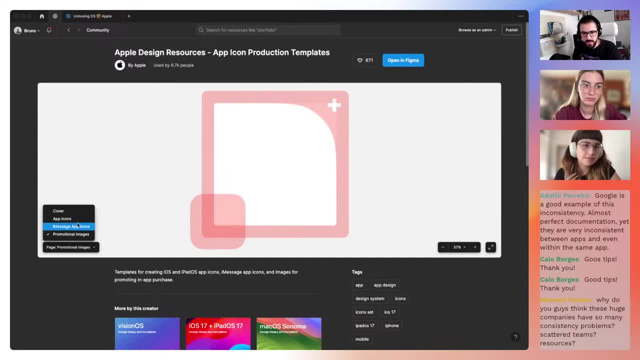 And if you look at these, usually these are a little bit different in the way that they talk about The icons, because they are mostly focused on iOS and iPad OS, but they also include, for example, the iMessage app icons, which is something that I don't think we've ever thought that much about it, but they exist. 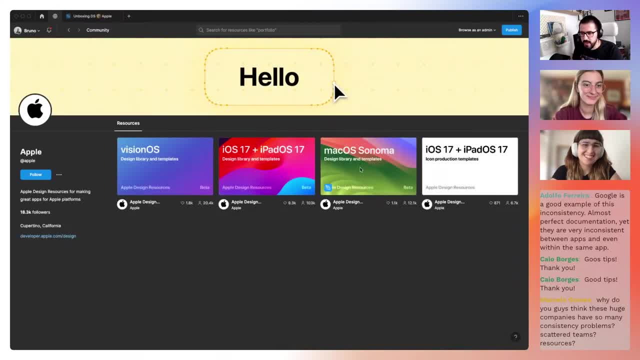 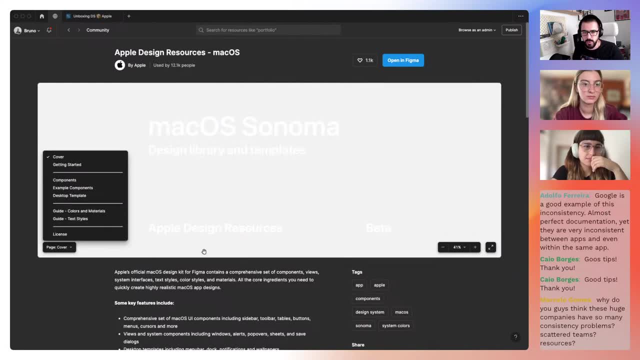 That's clear, Yeah, Yeah. And let's look at Mac OS: Sonoma. We're not going to be looking at it today, but we can already look at how these components will be looking into the new Mac OS. that is still not out. 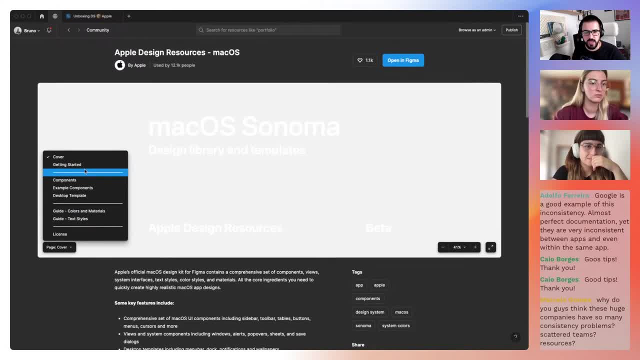 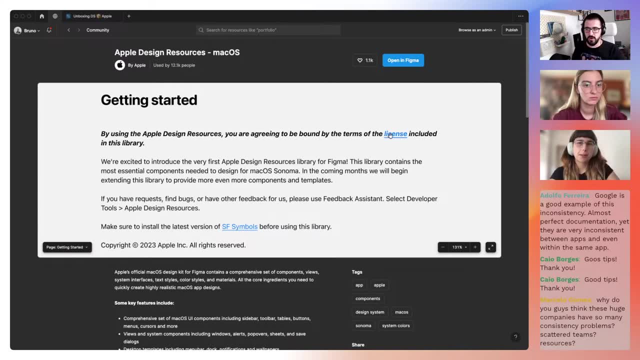 It's still in beta. Most of their files are built the same way. We have a get Started page with documentation. They have a cool thing that I haven't seen on any other Figma files, which is when you want to open them, some of them you actually have to accept. 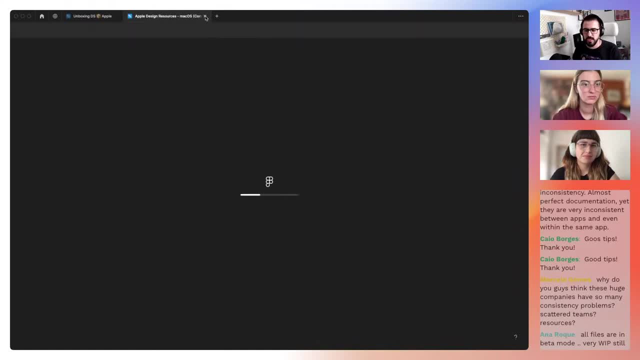 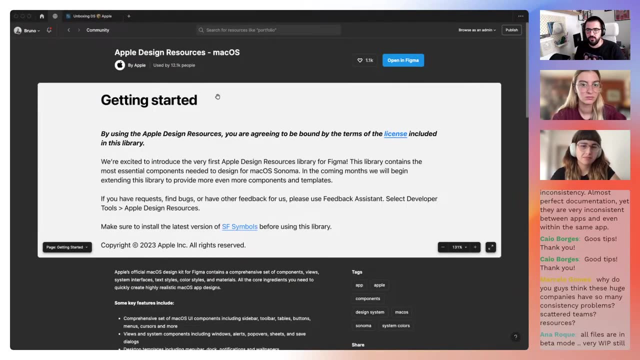 Let's see this. This one doesn't, but I think iOS and some others- you have to accept the terms and conditions, or I don't know if it's because I already accepted them that this doesn't show up. But FYI, if it shows a little terms and conditions page, now you know why. 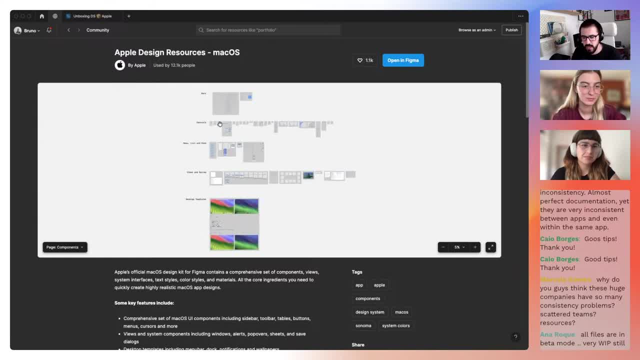 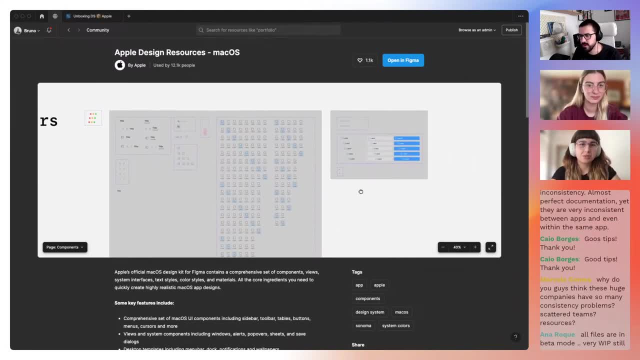 And then they have their components very neatly Organized. you can see the elements here and it's already using sections, which is interesting. Yeah, I was just going to say it's always when I do live streams that my cat starts to meow. 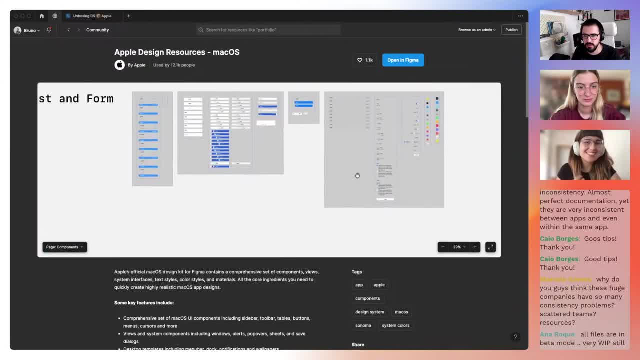 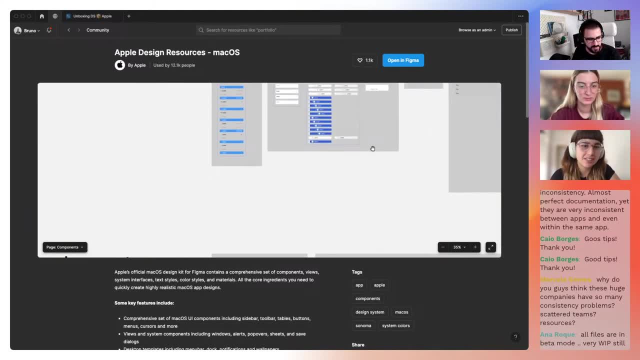 Don't worry. Yeah, we were missing cats on this live stream. All one of them already appear here. So yeah, I have three. So in case you see three cats differently or not crazy um. all files are in beta mode. 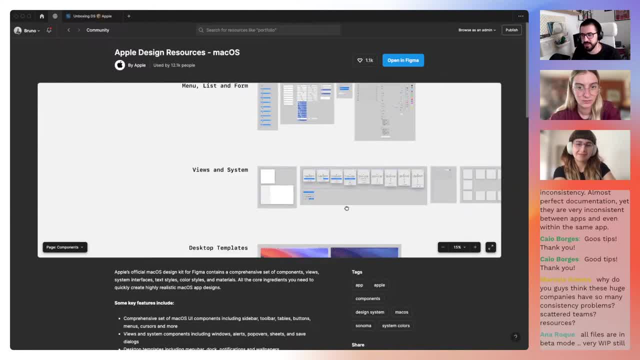 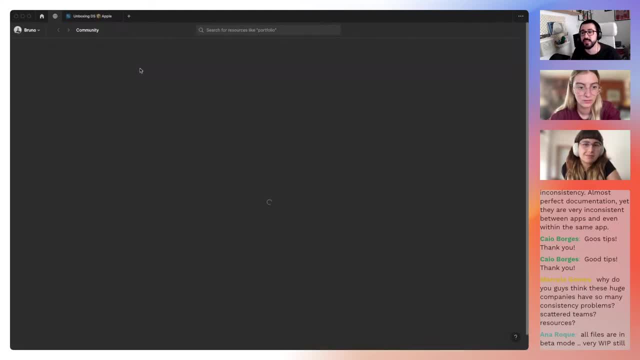 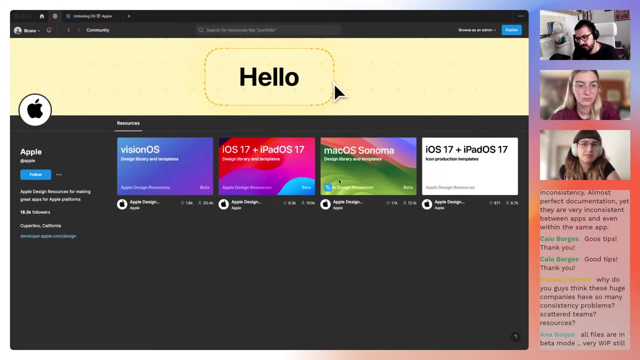 Very working Progress. still, Yeah, of course, because they just moved into Figma, or at least they just started publishing into Figma, because, let's not forget, Apple has been designed in sketch for a long time. Uh, yeah, to be honest, it's still a great product and it's native for the Apple ecosystem. 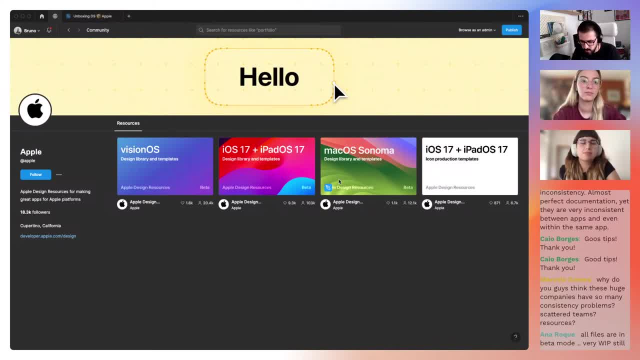 So it makes sense in their way of working. It makes it perfect for them to just do that. Um, and today we're going to be looking into the iOS and iPad OS and vision OS, uh files and playing around with it, Right. 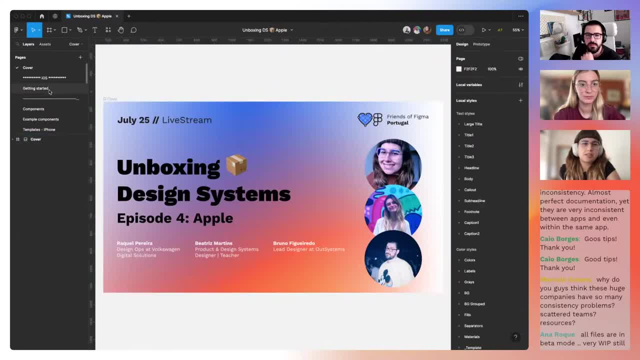 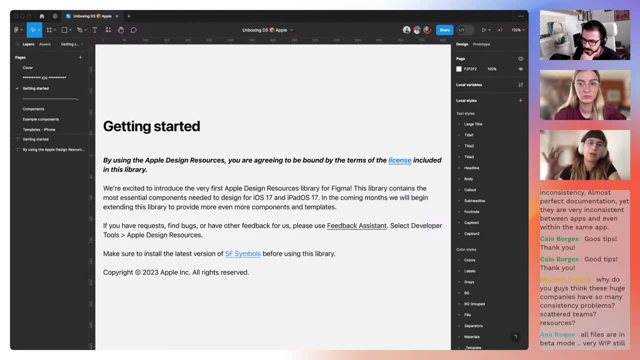 Yeah, I found it interesting that at least um it's on beta but they shared because I think at least my perspective as a user. with April I only see things very polished or very finished, but in the design world as we are seeing today, I think it's. 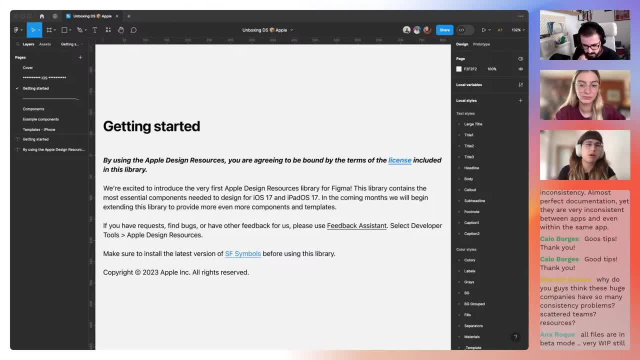 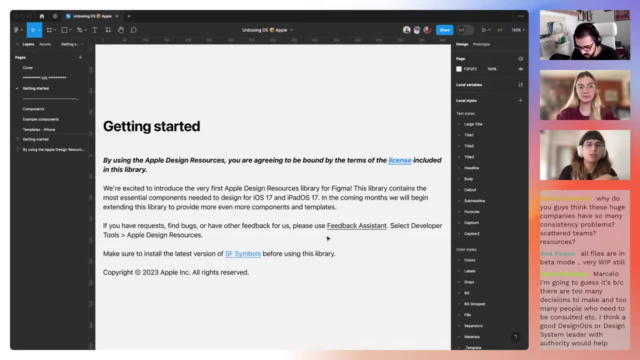 interesting that they show a little bit more progress, like: okay, their website is still not 100% well done because they do a revamp. their components are also with notes that we are better. We're still working, So it's good that they. 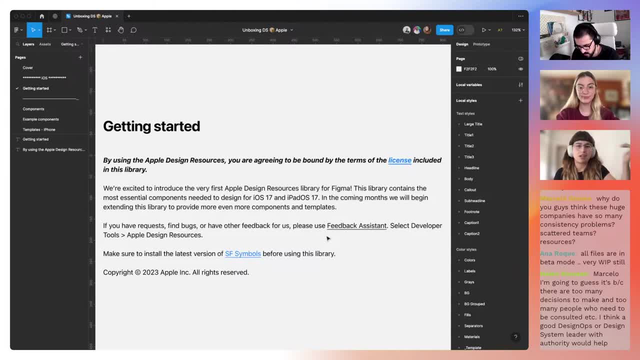 Shared that to the world and not create that high expectation or high standards. you know that we also, uh, put them and maybe they we can humanize them as well. You know things that I found that it would be nice. 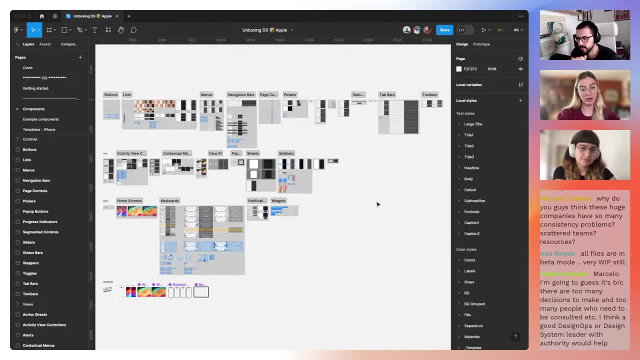 You have, for example, um, like a version history where you see like all of the design system has suffered just because, of course, like 10 years ago or five years ago, they didn't have that much things. So just seeing the transition or the 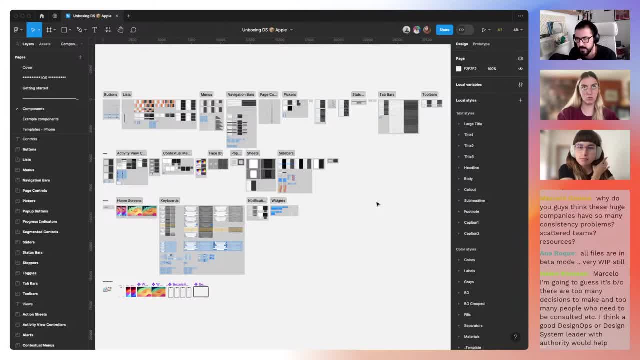 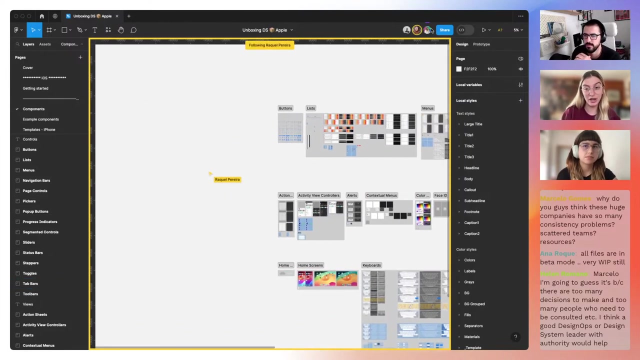 Evolution of the design system would be amazing, And maybe we would be able to see: okay, wait, they have done a lot of stuff. Um, maybe we don't really acknowledge, but they have. So I think that would be also a thing to take a look at, because right now they're designing for, I don't know, iPhone 14 or iPhone 13,. but, like what happens with the design system that we had for the iPhone three or the iPhone four, 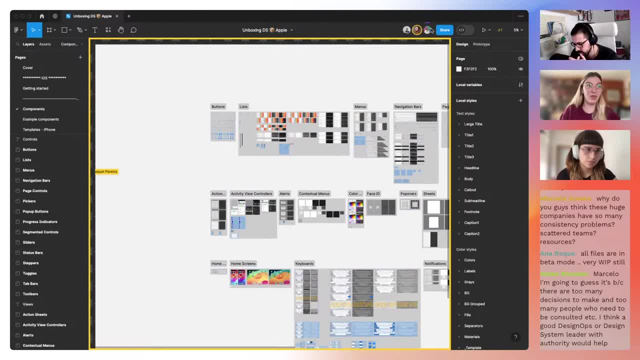 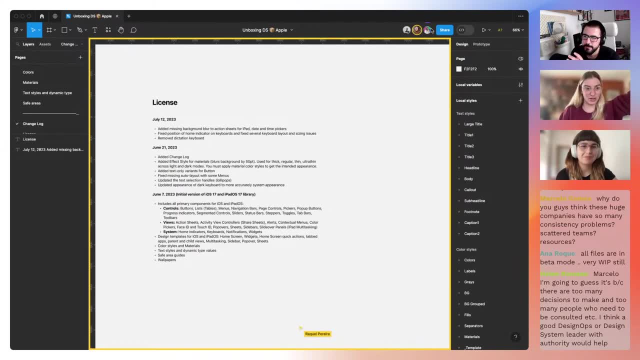 I mean, that's, that's something, that's a A thing That I would love to see you know and see, like how it was done before, like before, like on the dinosaurs age, you know, because they were pioneers. 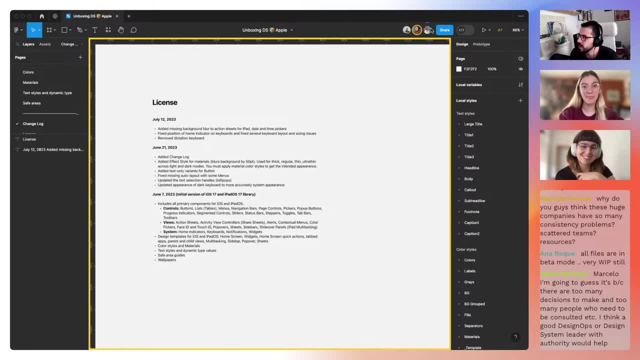 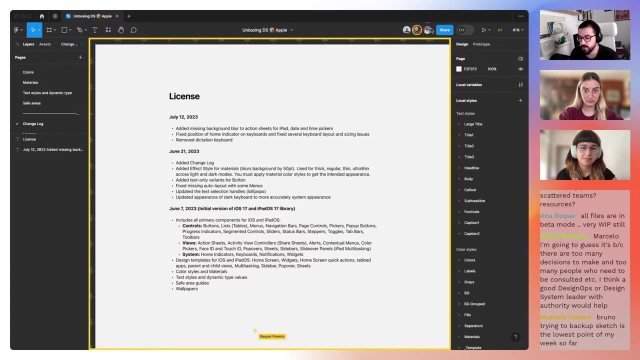 Yeah, But I'm, I'm, I'm, do. I am gonna say one thing, though: Um, that also has a lot of weight from technology, in the sense that, yes, again the same way that we were talking about the whole Photoshop thing, people were using a bunch of different tools before and migrating that information from. 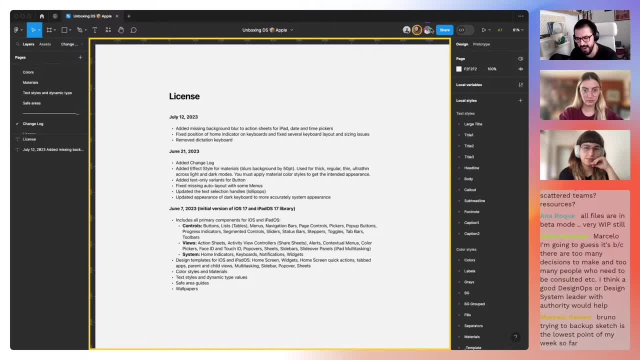 Yeah, One end to the other. I don't think we as humans are very good at it, right, We, we, we record, then we have like, that's why we have files like PDFs and JPEGs, which are very portable and easy, and people kind of save those to make sure that they last longer. 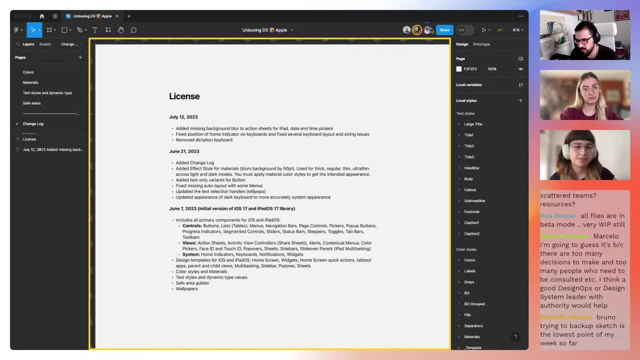 But probably you lost a lot of work in, uh, fireworks and Photoshop files into Carl files and things that were in the past. Right, And it's not that we don't want to keep that history, It's just that we're very bad at digital spaces, specifically to do the type of archiving that we did before digital spaces existed. 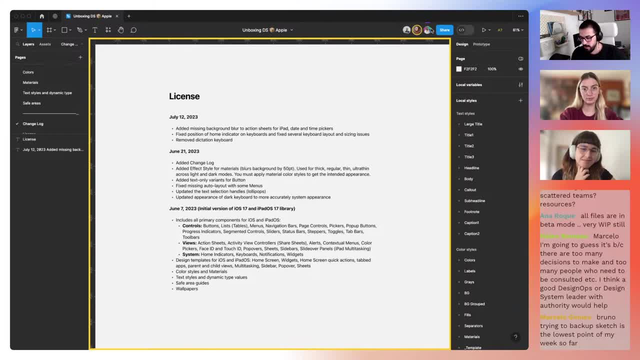 Right, Um, yeah, the way back machine is probably one of the best tools online And even then, for you to save a website there, you need to actually go and do the job of giving the website to the page, to the system, so that it starts archiving it, which is not something that happens and not many people do, and they can use web scrapers and things like that. 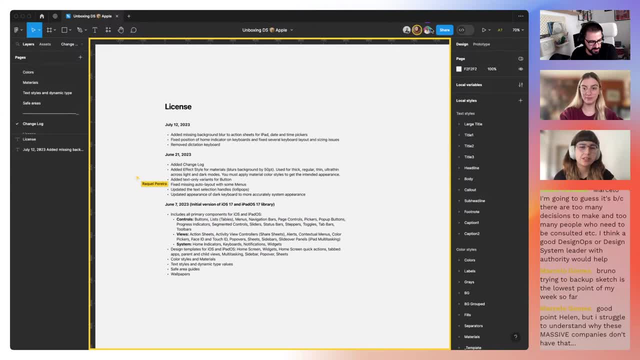 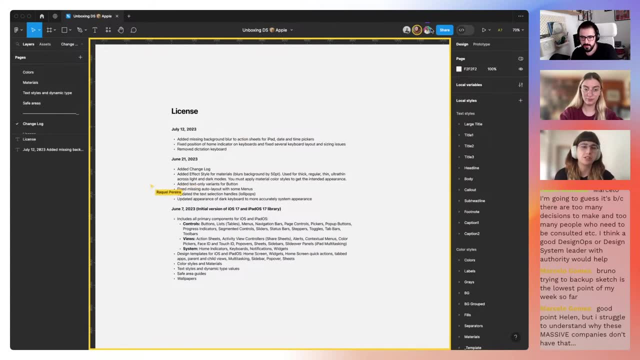 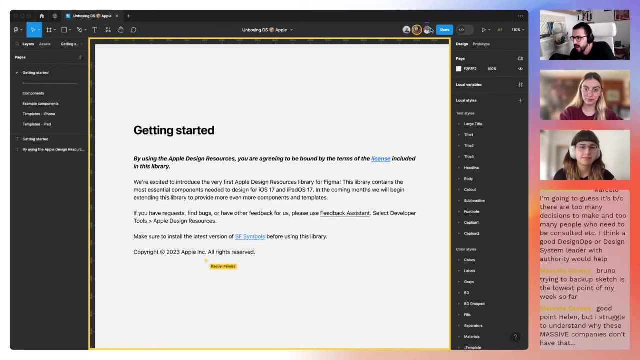 But yeah, it's yeah, Yeah, Hopefully be. uh, they improve their change log at the moment. It's this. it's really recent, but I for sure think that in one Yeah Year we will see a lot of progress on this funnel. one thing that could be amazing, but this is more like: Hey, Figma, can you do this? 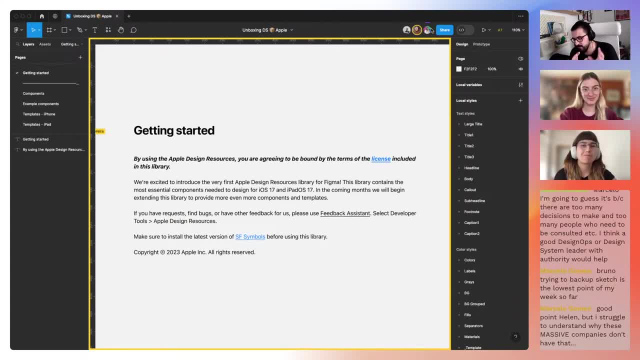 It's like use the native version history on these tools for the community files or things like that to actually have that type of record. Uh, we use it a lot internally, Um, me and my team. when you have version history here, you can actually create a lot of documentation and stuff like that. 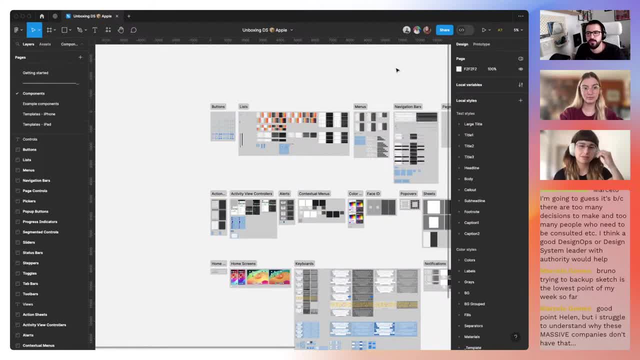 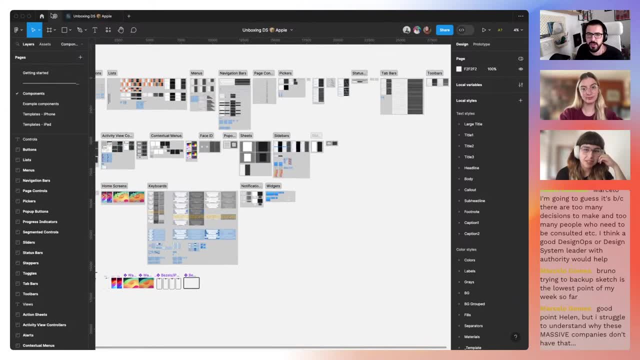 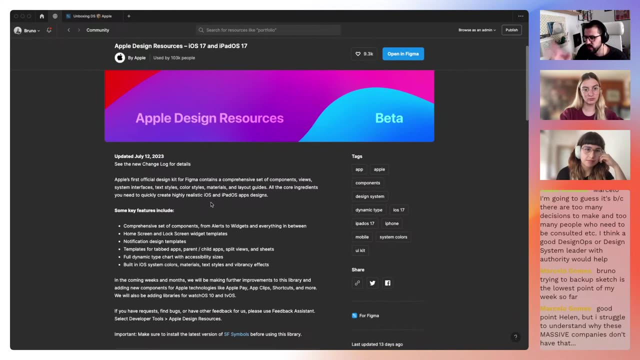 Yeah, But everything that comes, yeah, but everything that comes from the community, you really don't have that. You don't have access to like versions and things like that. You can really do updates. The best you can do is you can come here and drop updates and do a change log in the file, or here and put like version numbers and things like that. 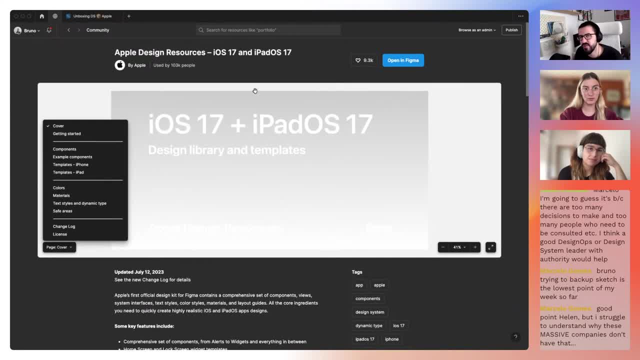 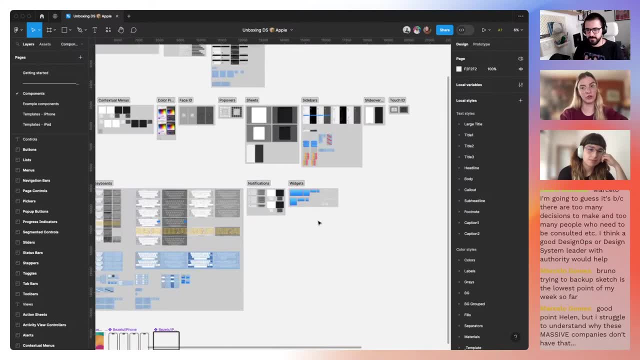 Yeah, But it isn't the perfect way to see how these files evolved and how actually we we went. Yeah, Or even on the documentation. I mean there could be a place where you just select the version, Like I know Decathlon on this on zero height. they have that. 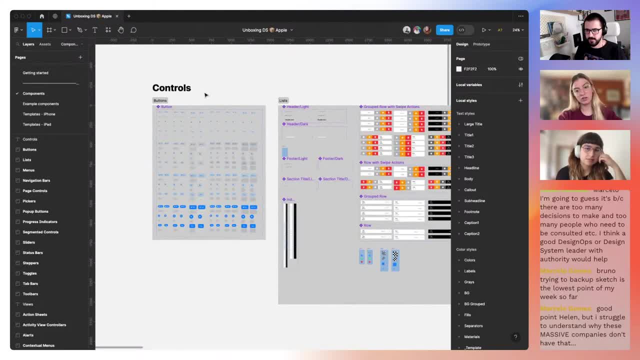 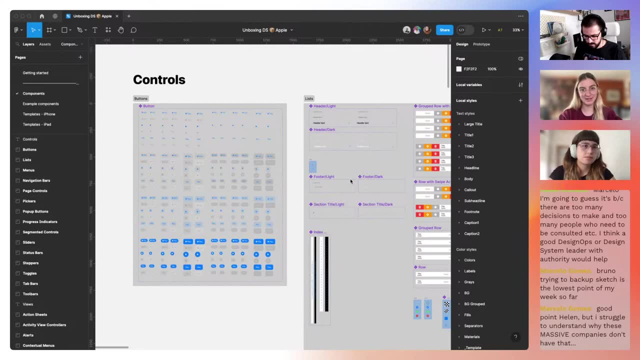 You can see like Mm-hmm Three years ago or something like that, even spectrum, I think. you can see like the old uh stuff which would be really like see what designers are you doing, Cause they haven't changed much. 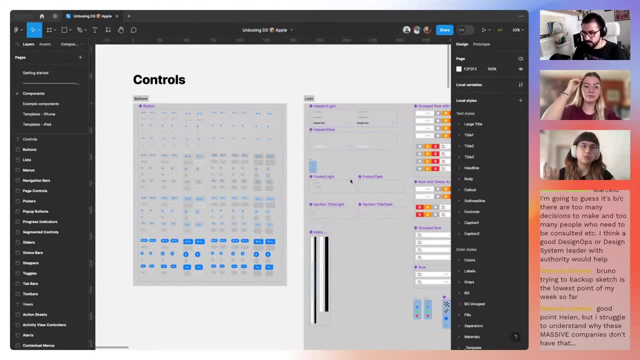 Um, they actually have the what's new page. maybe there in the future could be more involved. You know, uh, we didn't go dig in on that page, but they have a what's new page and it was interesting. Uh, maybe there we can see a little bit better that progress. 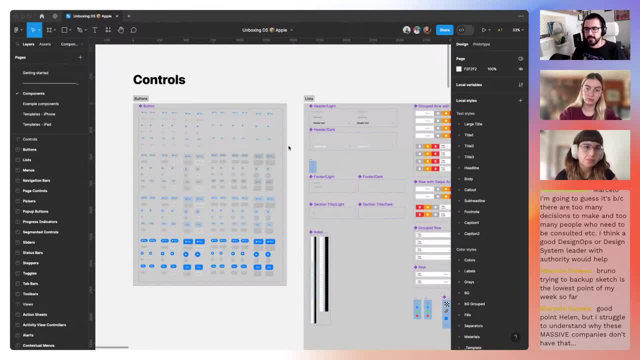 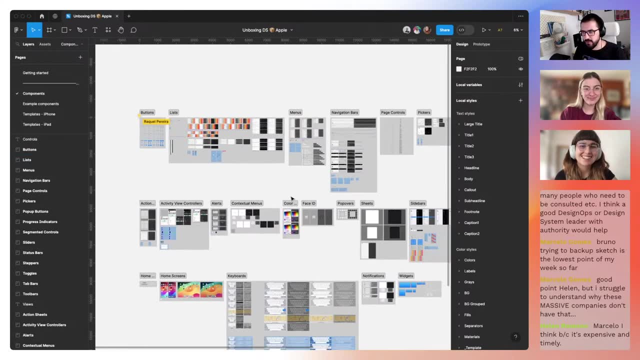 Let's hope. Yeah, guys, We need to start designing, uh. we can already see, like the way that these things are organized. I feel like it's very nice using, uh, our sections to do this. It's like it's a really cool thing. 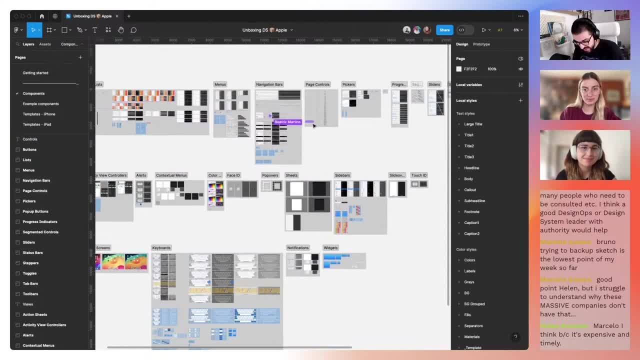 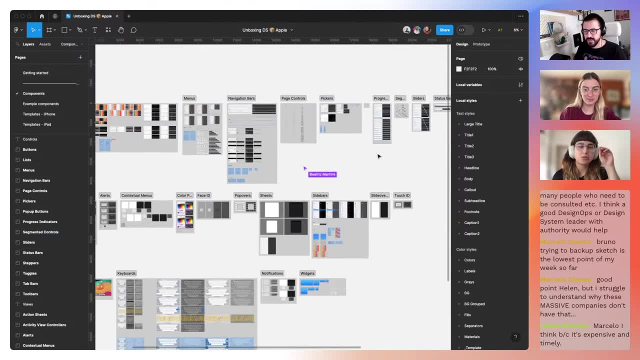 Uh, I'm gonna be honest. up until variables I didn't use sections for anything. So seeing it used now it's just it's it's interesting. I actually start to use section to put ready for dev. There you go. 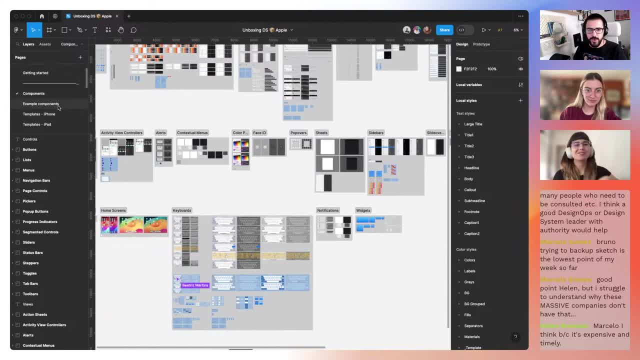 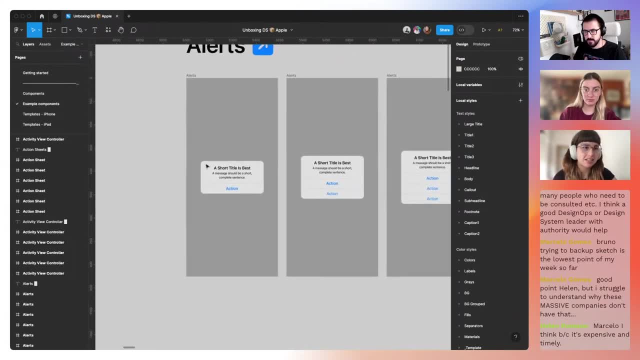 I like: no, I I wasn't using, but I know that, Yeah, We have a bunch of like example components already here, like prebuilt, which is cool, Yeah. Yeah, That's the thing, the magic of this uh file, I think, because, even though that's not that different from the way they are, 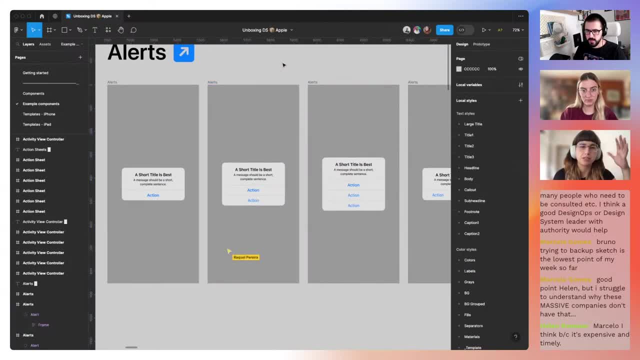 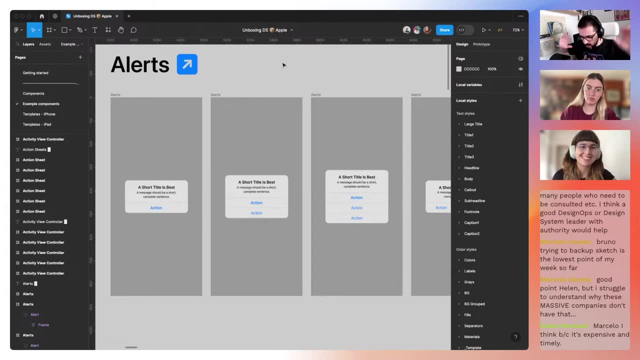 organizing the libraries. at least here they have a little bit of minimalistic context, which was interesting and honest, And this is like pro tip for the juniors in the room. There's no juniors in the room, but maybe someone is gonna watch the recording. um, use this on your prototypes. 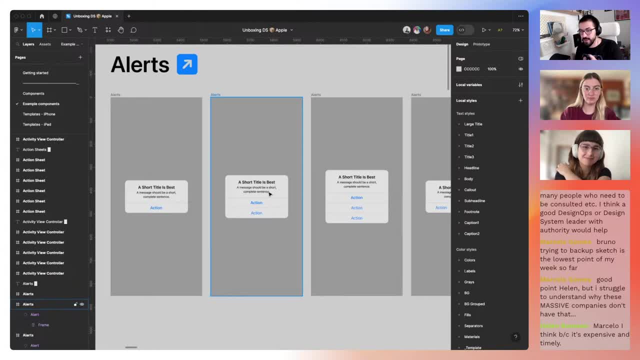 So, yeah, I think it's cool, Okay, And I think it's also nice cause it is a good tool. It's so easy to take off the, to take it off a lot of the time And you can start to get familiar with it. 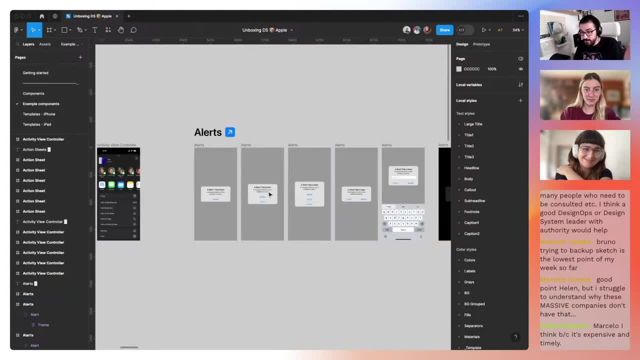 Yeah, So I don't know if it's reactivated. Yeah, it's good, I know, I mean it's very nice, It's really nice. I'm kind of curious, but I don't know, I'm not sure who has done it. 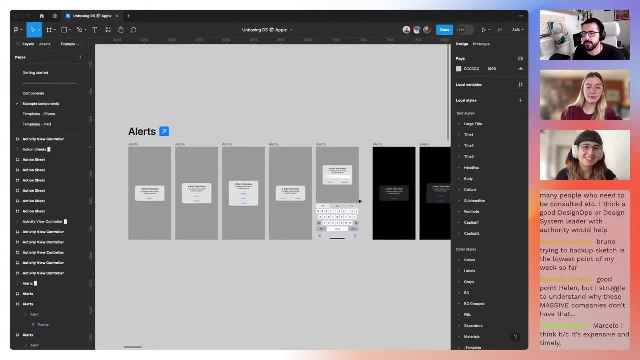 Maybe it's the same existed before. I mean, what was it? I mean maybe it's the same, but I don't know, I'm not sure. I have been doing it for months now, Like it's a little weird. 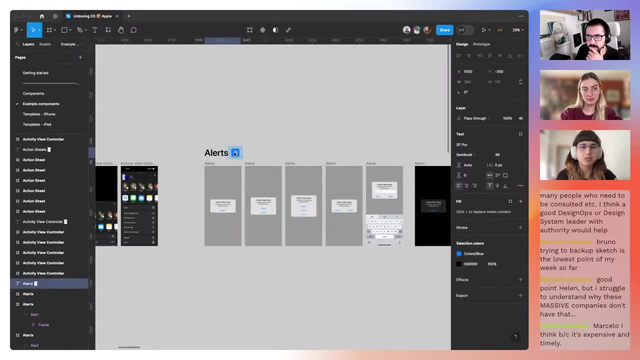 But yeah, it's really smart, It looks really cool. simple icon with a link to go to the documentation for the lazy ones, to the page. okay, nice, yeah. yeah, it's just a very uh small thing, but yeah, i think it was interesting. now i'm gonna, i'm gonna give. 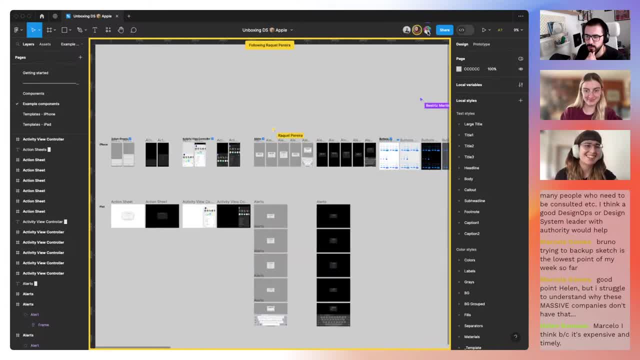 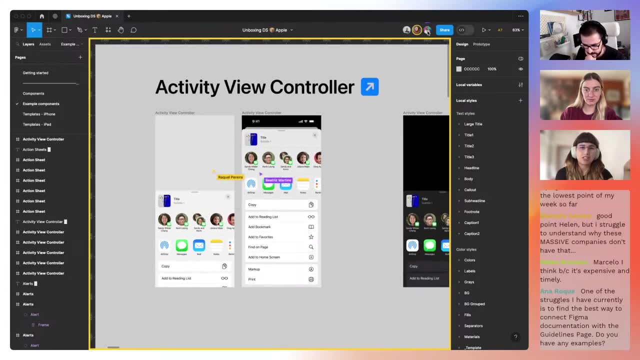 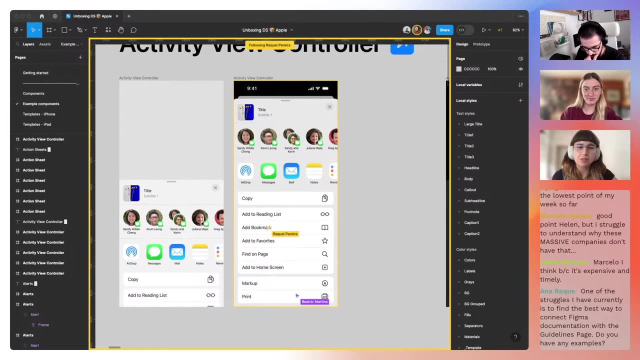 you control. i'm just gonna follow you. tell us what are some cool things also that you've seen in the document that we should be looking at. yeah, i can share like my 20 seconds thought when i saw this is like: this looks so pretty, like i don't know how they do it because the read, i mean the. 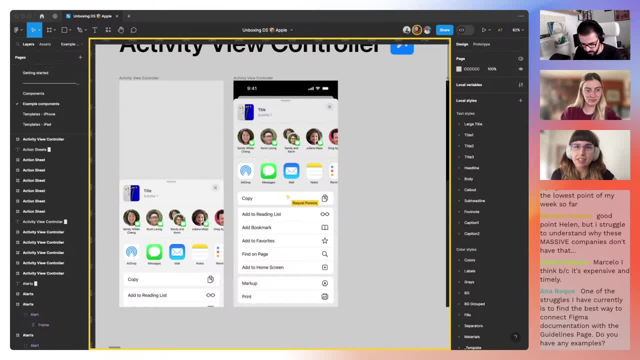 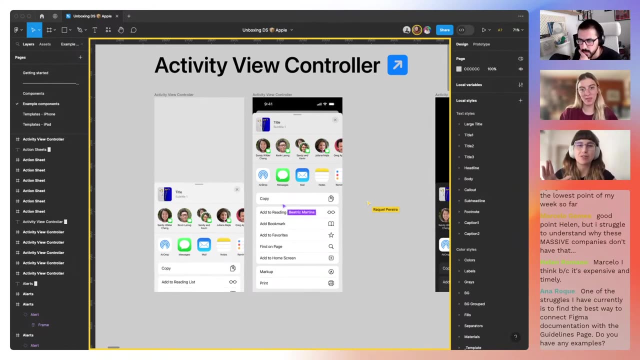 the text is not. it's like it's not alvetica but s, s, s, s, s, c pro. but i don't know the way that they have the ui design here. it seems just so good and i wonder why i don't have that feeling sometimes with my proposals. but i think it's the magic of ios and apple in general. uh, that's the first 20. 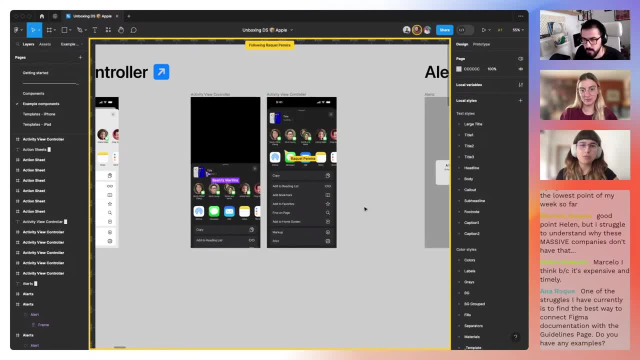 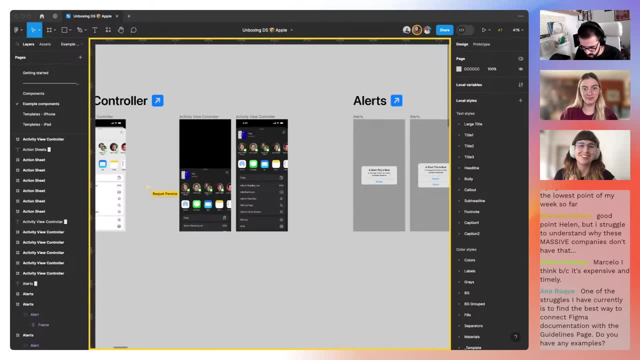 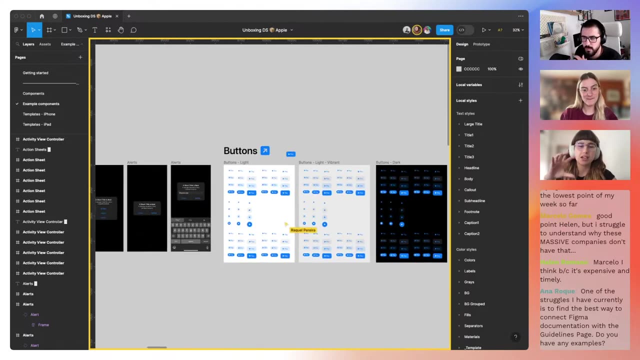 seconds, that i got late because i was imagining like, oh, i'll go to figma and i will have this feeling like things are not done, but i don't know how they do it. i feel this pixel perfect even here, you know, yeah, so it's really interesting. uh, i also find it funny the buttons, uh, the colors, because in some 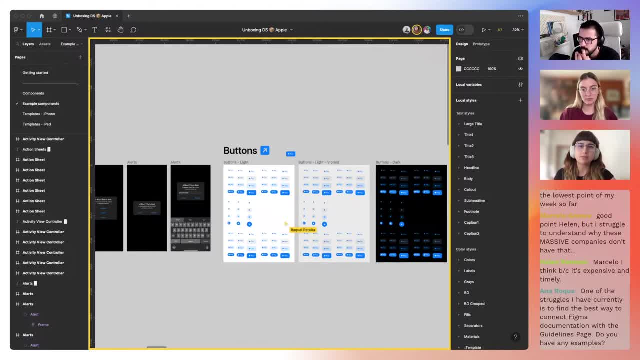 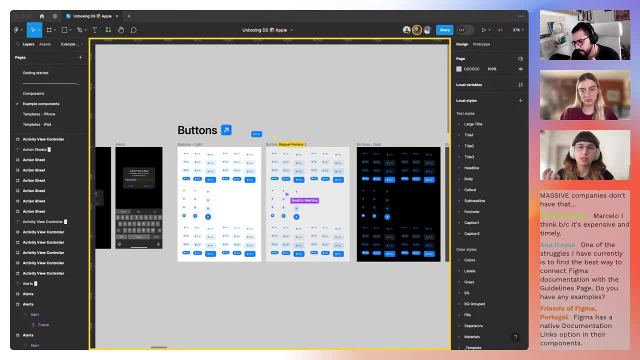 themes, at least mac os. you can also personalize the colors, but i think this is a standard uh button for that. that's the, the, the, the dilemma that we are uh talking like to whom this button would be right? because we don't know for sure, you know, like for each. 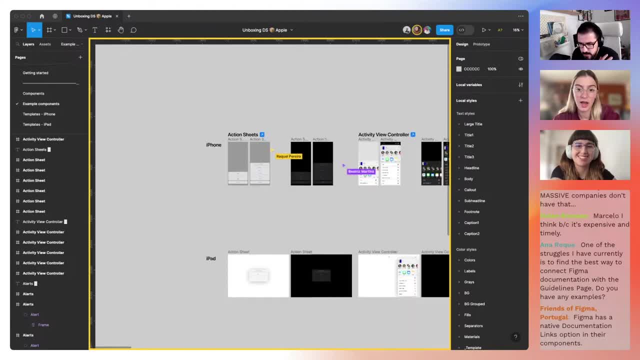 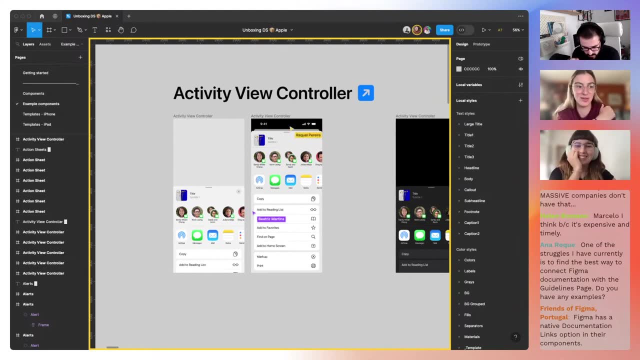 platform. you were saying something. sorry, i get excited. i was just gonna say that i mean these are amazing, like i, i love to see these files like the, yeah, how they get to work, uh, everything developed like really nicely on your phone or on your macbook or whatever. but then 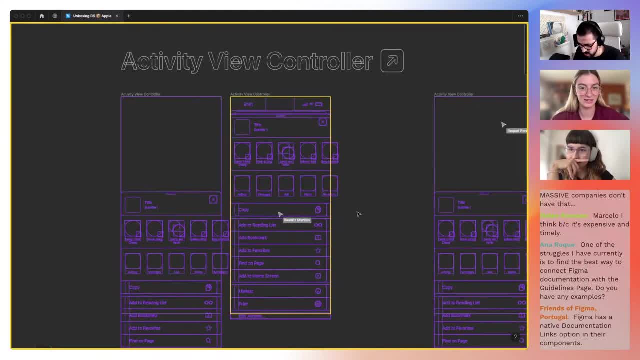 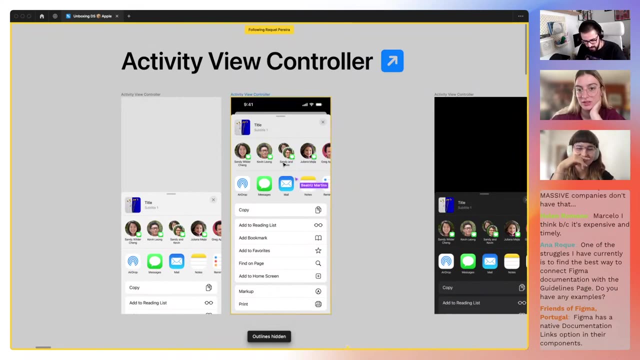 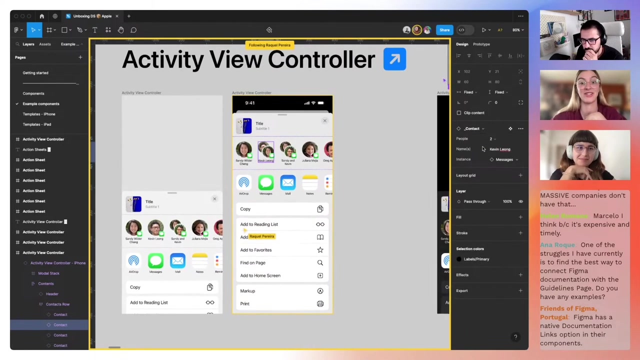 this is like the entrails. um, i just turned on the outline mode to see how these files are clean or not. yeah, yeah, and also the variance. if you dig in Bruno and start to switch, you'll get a lot of fun. there you go. what i've seen is that, i mean, this is something that i i use every single time. 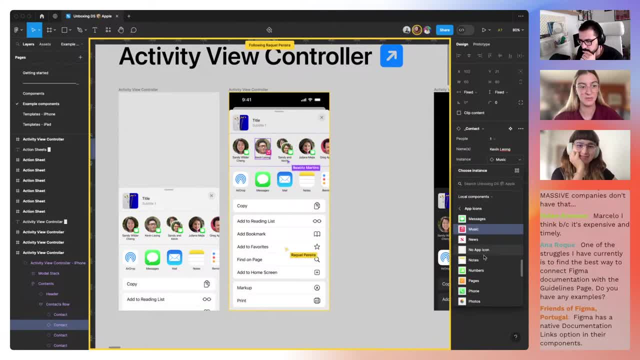 it's the outer layout and they don't use that like if you go to the atoms, for example, to theontac, this one, like they just have frames and frames and frames. of course they have to trigger accuracy to go from kind of consistent ability to really find life. in that way it will be hard for a lot of people. you guys, we're gonna to do this, Wolfgang. 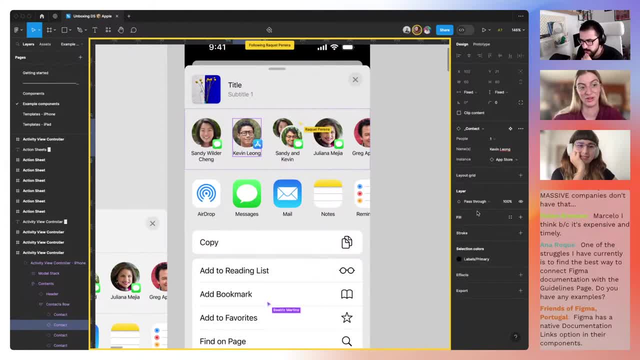 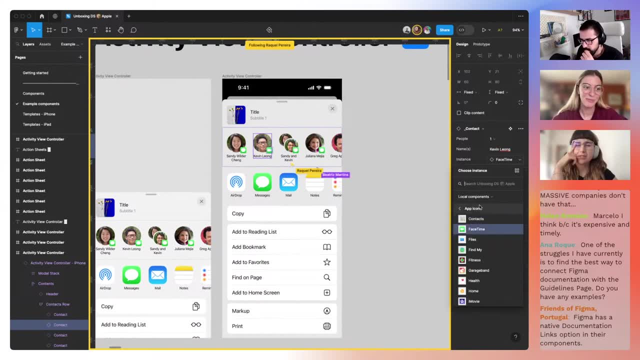 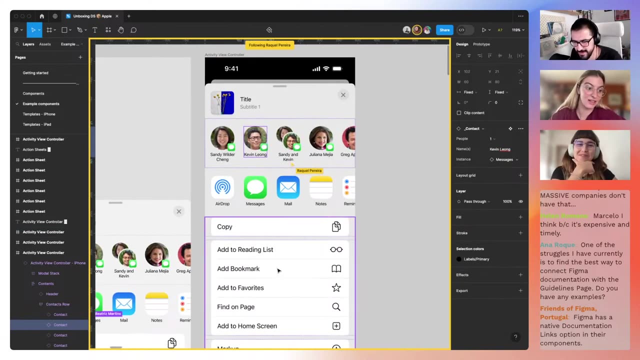 them renamed. so this is amazing. i i almost never rename my, my frames. they're just like frame 1346. yeah, yeah, it's a very good practice to rename, but sometimes it's a pain in the ass, but it just it looks. it looks weird not having bodily out. honestly, i i don't really know why. 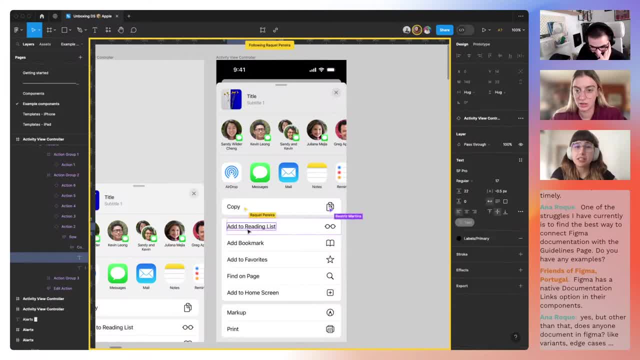 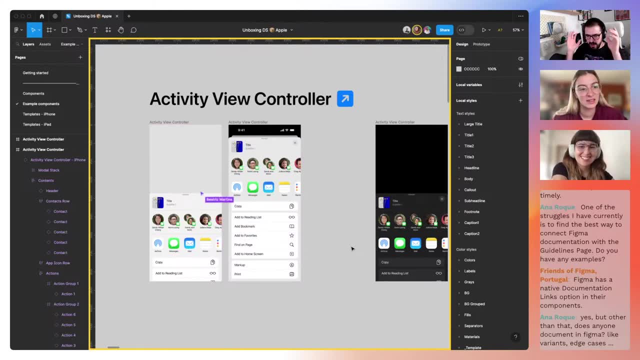 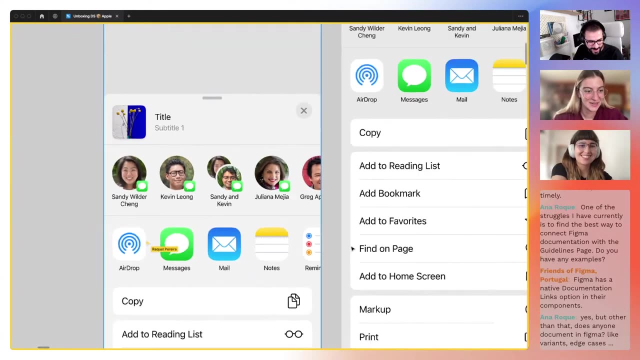 i know, probably because they were searching sketch for here, exactly like my i have. my whole thing is like they are doing a great job of bringing these here, but of course they are struggling with the sketch migration, like everyone that we know that has to do a sketch migration. yeah, okay, quick note. anna hawk is asking one of the struggles that she has. 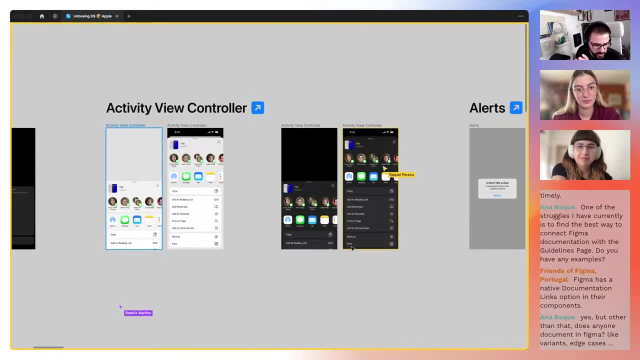 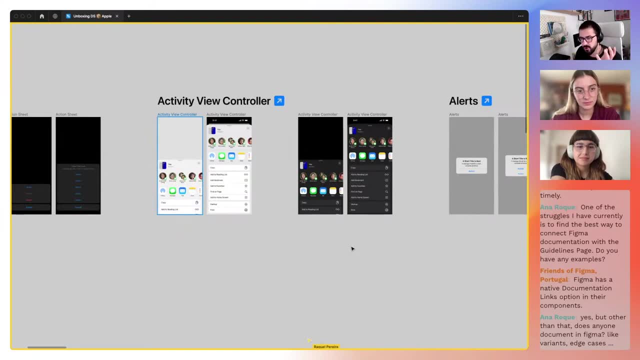 is currently finding the best way to connect figure figma documentation with the guidelines page, if we do have any examples. i answered with the figma native feature for documentation. i don't know if you guys use that, but like i tend to use it when, whenever we build the systems. so 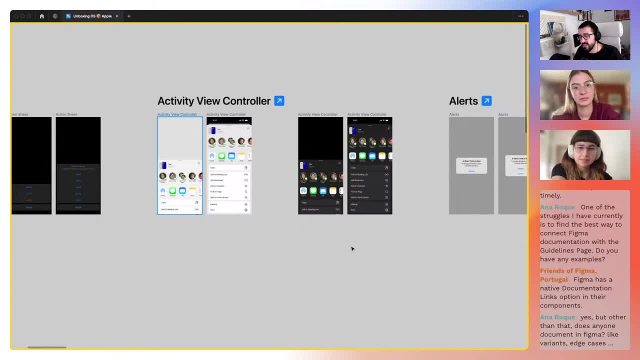 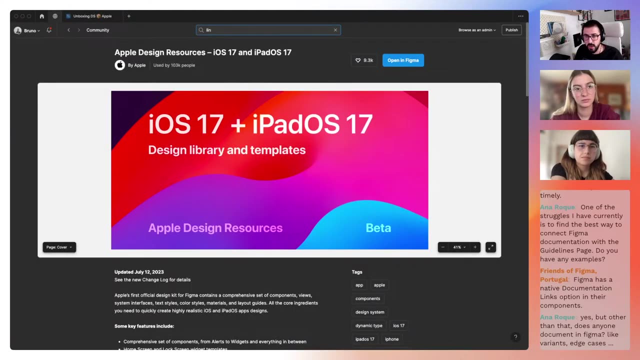 it's already in dev mode and everything outside of that. usually it's just creating widgets for documentation or like little boxes and arrows, like they did here. um, there are a couple of figma files on the community that already exist for that. uh, let me just look here, like uh, 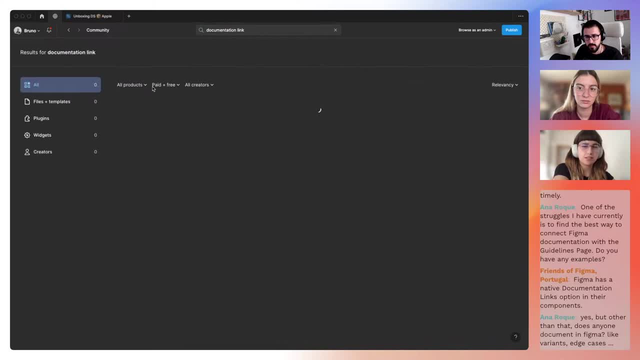 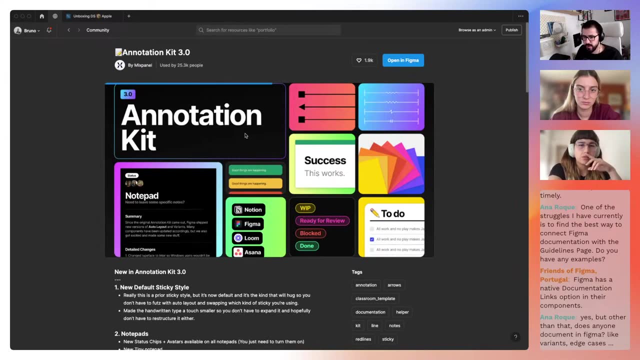 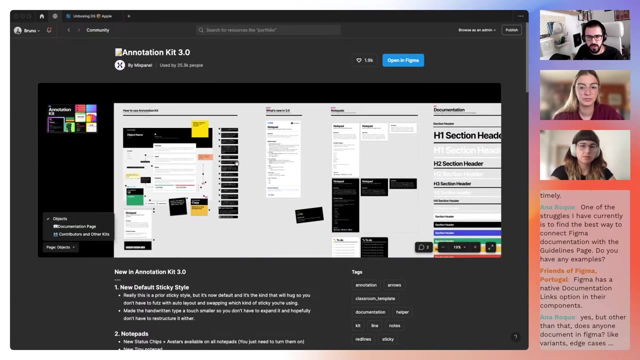 i think- uh, i didn't explore that much, but i think also figma has now the possibility of doing specific documentation for each variant as well. yeah, so you can actually do documentation on different levels, for example things like that, if you prefer more visual stuff. annotation kit. 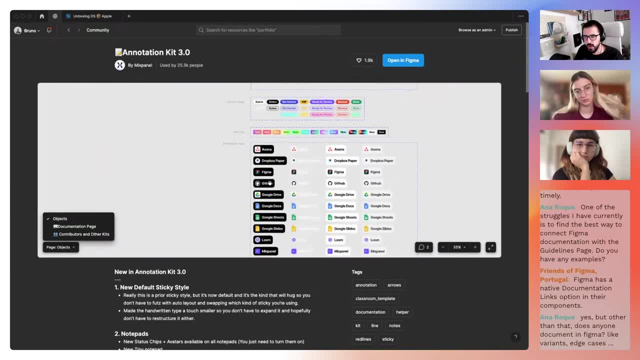 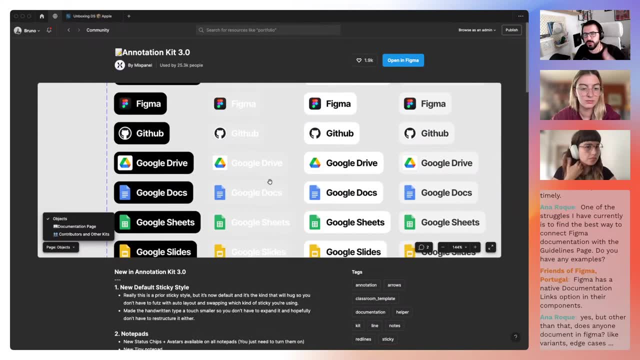 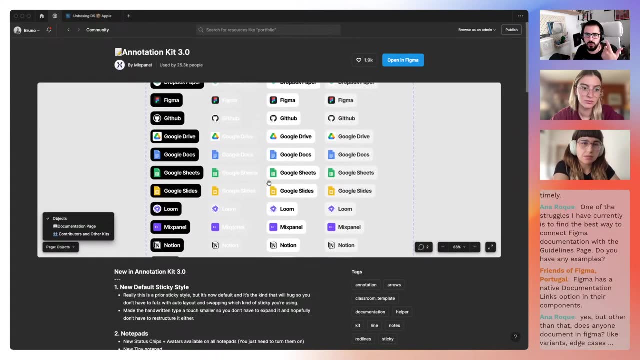 ad. let me see if i can find it. there you go. these type of things, we use these type of things in our system, which is like little labels for github, google drop, google drive, i don't know, jira, things like that, or you know, or whatever we use as documentation tools and we literally drop this with either comments or 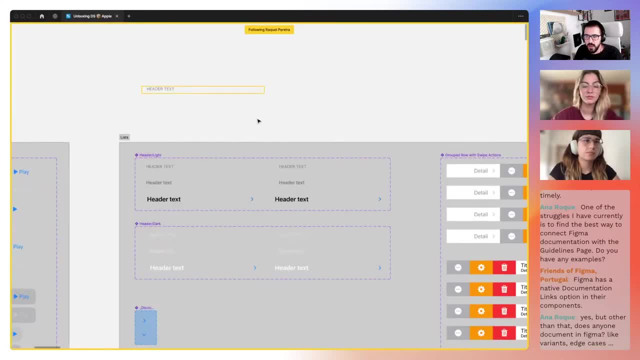 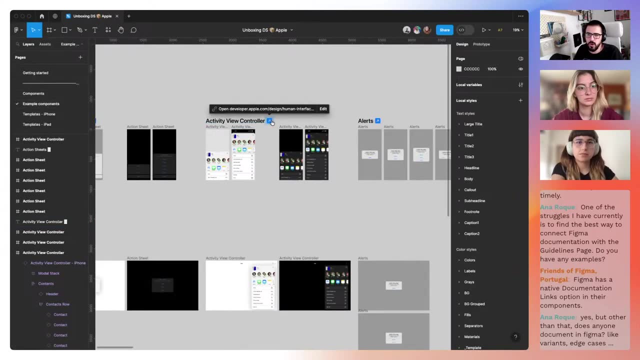 labels, just making it easier for everyone to find. um, it's fun to see like these guys did the basics. they just dropped little arrows there where people can just click on them and go and see. but yeah, that's basically what we can do now. right, like, yeah, they also made some upgrades on documentation. inside that you have, like, uh, you can put bold and. 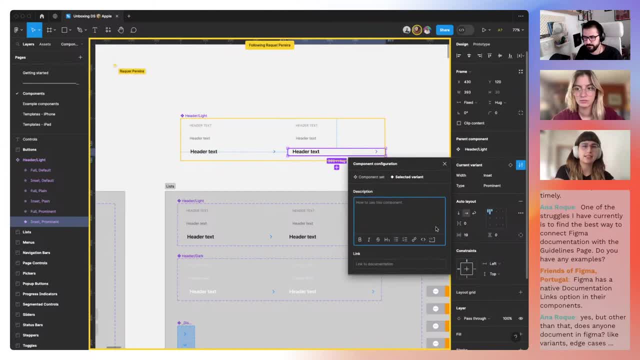 the link for documentation and once you're in assets and you do the over uh up front of the on the component, it will appear that. so maybe you can try and explore a little bit the company, the documentation inside of the component. um, and i didn't try it out, but i found it interesting. 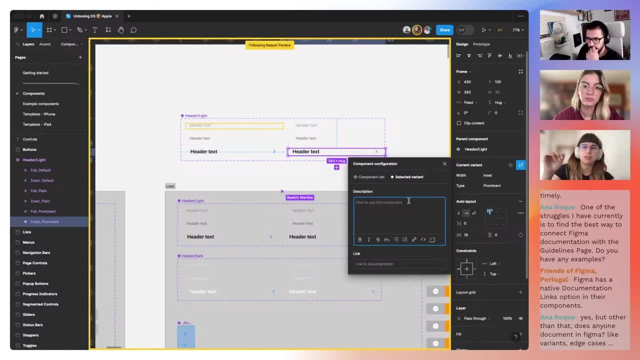 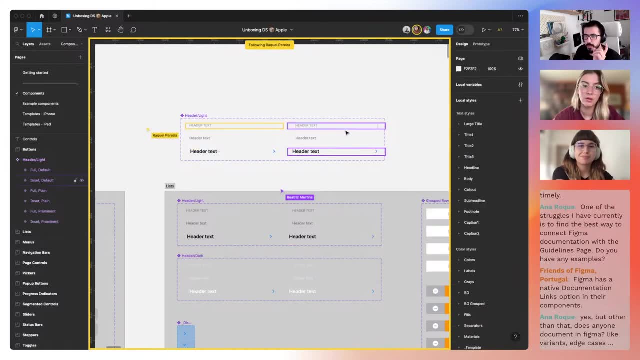 if you want, if you would like to explain specifically one variant and just add the documentation for the variant, so maybe that's something that you can dig in. also, don't forget, i don't know, i don't think they did the prototyping things and stuff like that. 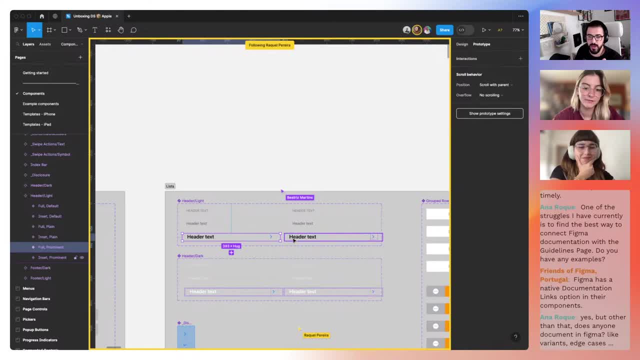 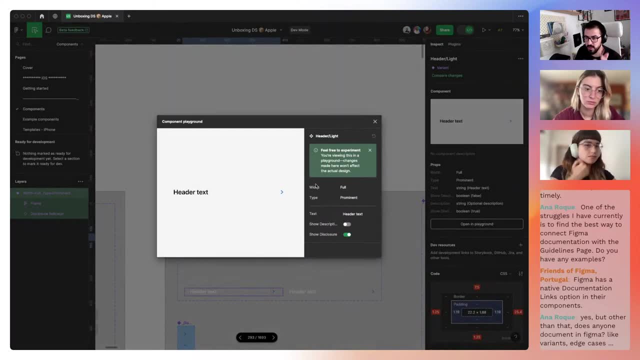 but, for example, probably not. yeah, but one thing that you can actually look at in dev mode now is the playground which, for example, for prototypes and things like that. if you view the documentation natively, it's it's simpler to then actually see, like not only the documentation written on the 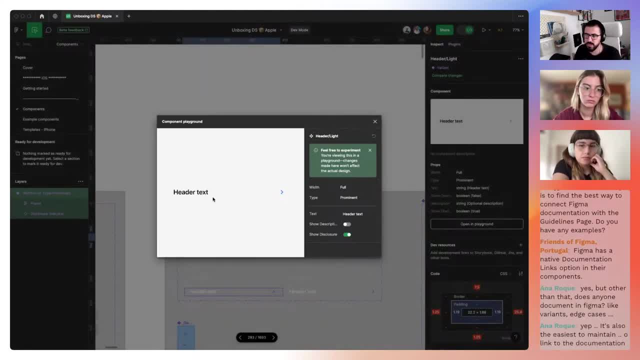 side, but also, for example, the behavior happening on the left, which is amazing. like buttons, cards, things that you build as interactive components, they become live for the developers to look at. so if you want to build components, the dev mode now has a bunch of other things for documentation that. 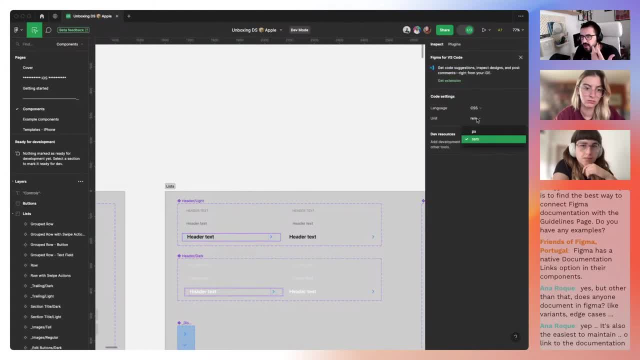 makes it easier. uh, yeah, including basic things like the fact that they can use the ram systems. i still need to understand. i don't remember where you can change the ram value, but yeah, i still haven't found it yet, but it works somewhere like mine is working, specifically like mine. 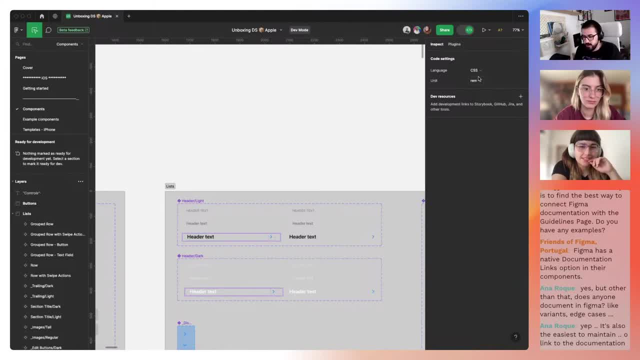 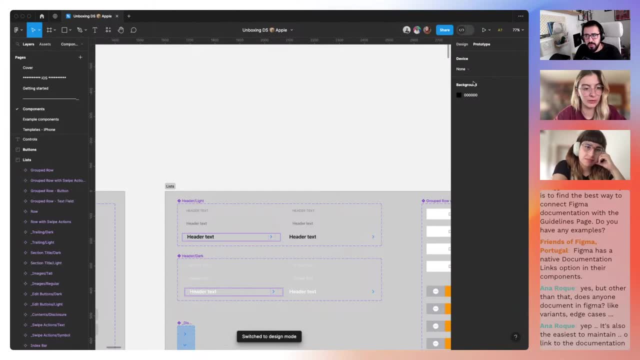 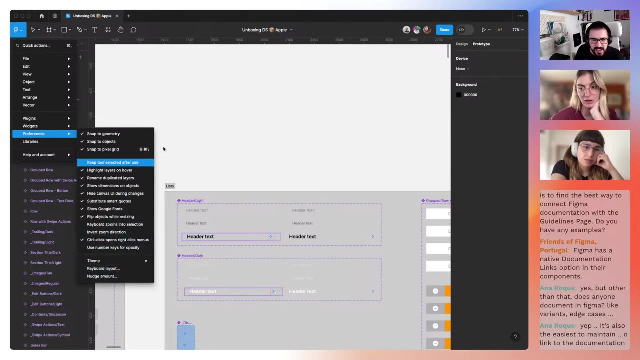 is set to 16 pixels and it's working and all my system is like: ram is 16. everything else is based on ram marvels. so yeah, um, i know that it can be changed. by the way, it probably is something somewhere under your preferences or something. i mean, i do use that like the documentation. 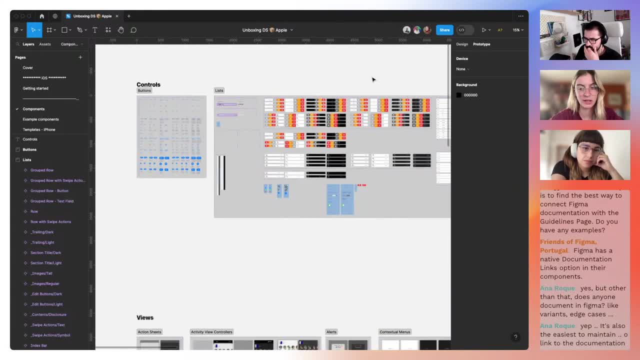 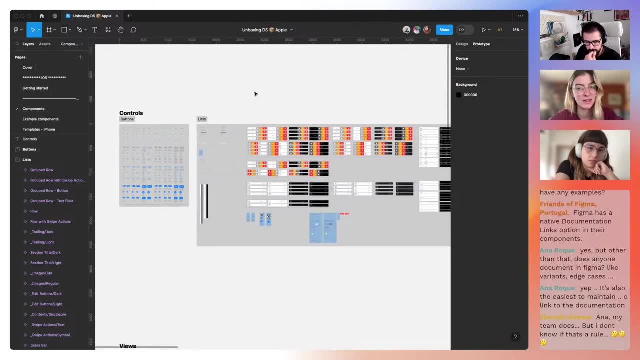 inside figma, but not all of the documentation. i just feel like that's useful to say, um, what the component does, uh, a few do's and don'ts and that's it, because, like, if you put all the documentation that you see on apple, apple human interface guidelines, it's just yeah, yeah. 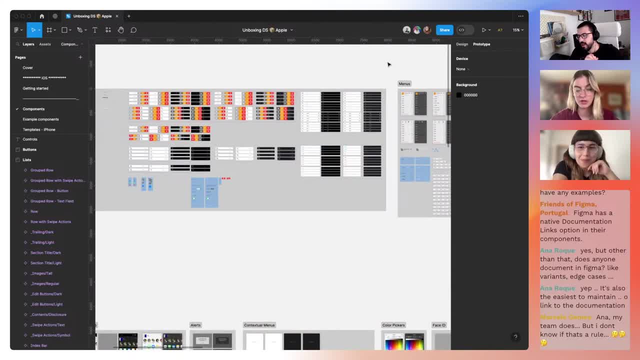 it will be overwhelming, yeah, yeah, i'd say a few things you know, like the description of the component, because sometimes we don't really know what the name is or we don't realize, uh, what component we're actually using, and then just maybe some do's and don'ts, or 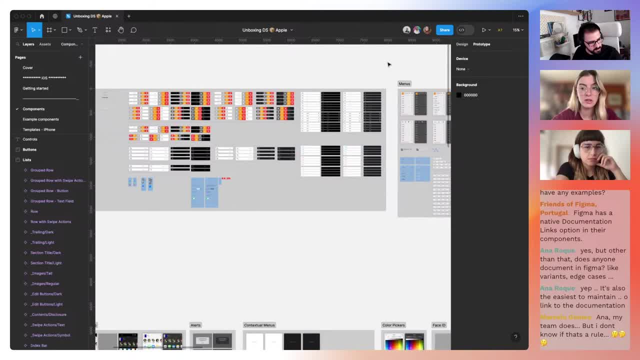 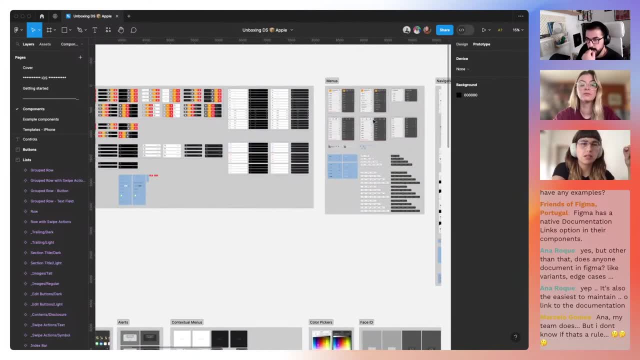 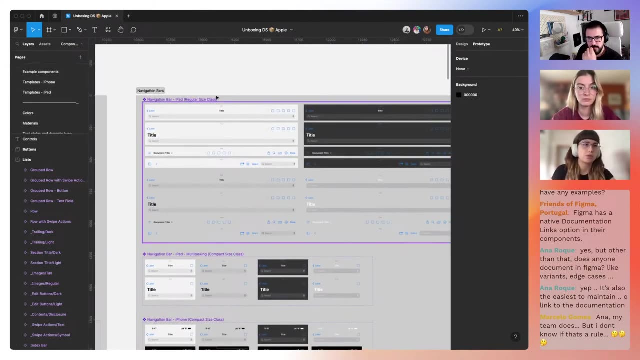 some minimum max uh widths, something like that i'd say, but not everything. yeah, at the moment i use description just to do like a very simple statement and i also put keywords for assets research. it's really useful thought. maybe i call it a switch, but you call it toggle- exactly what are? 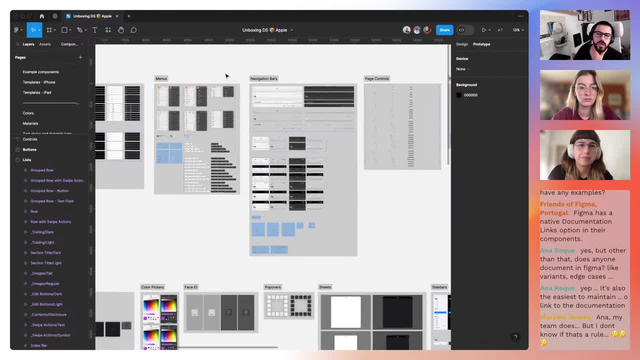 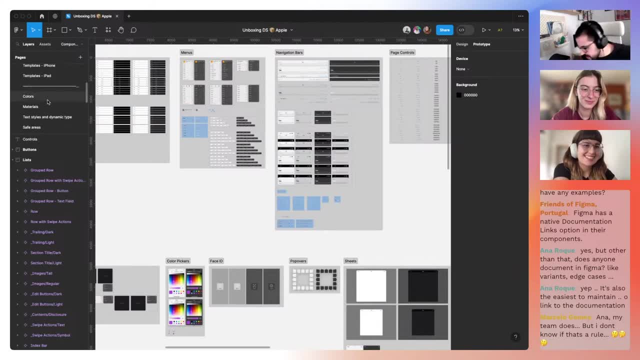 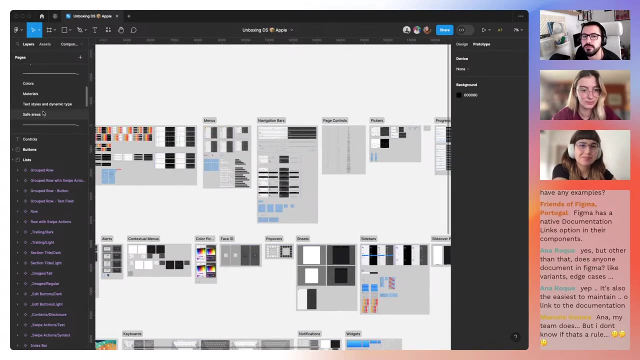 the keywords and then eventually people find out. anyway, i'm gonna be mean and just go like we don't have the time. so my question now is, since we have about less than 30 minutes to to end this, um, what will we build? i thought that maybe we shouldn't build anything specific today, because, if you see, 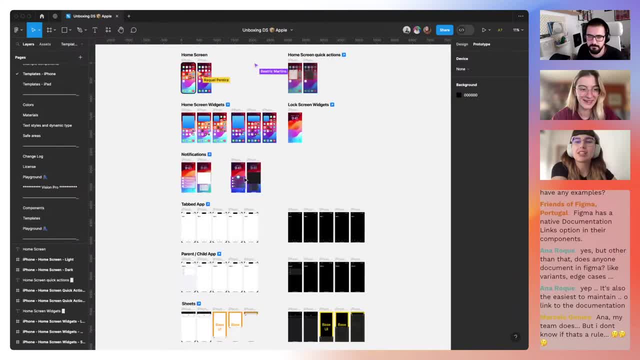 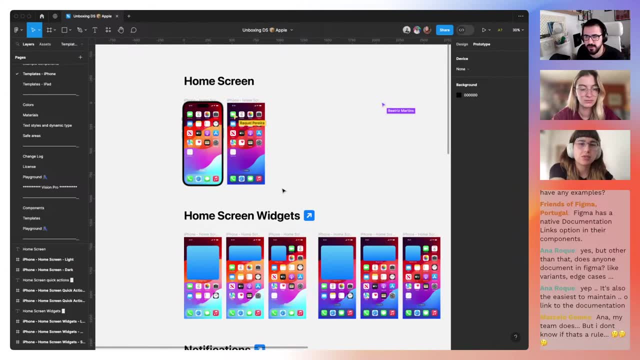 they already have a lot of templates done, but maybe we can uh, try to do a home screen, for instance, without something like that, okay, and try to dig in, for instance, the foundation, atomic design, for instance, via, and maybe inspect or detach and understand how they manage to. 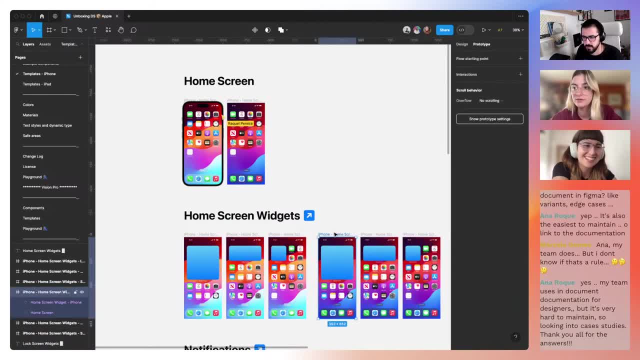 eventually i think it will be very sketch logic. so, yeah, let's see. and also, maybe we should explore- at least i would like to play around- uh, the templates for vision i, os, because that's the reality that i don't think that much of us really know, so maybe we can just 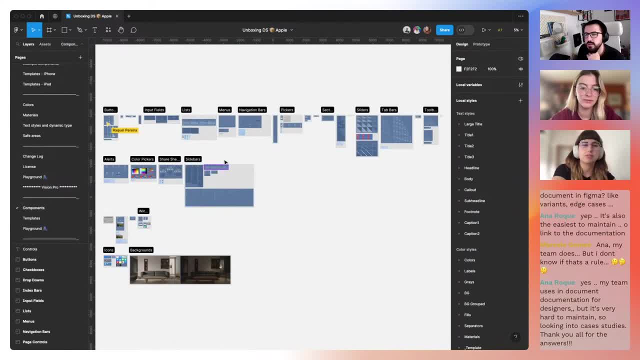 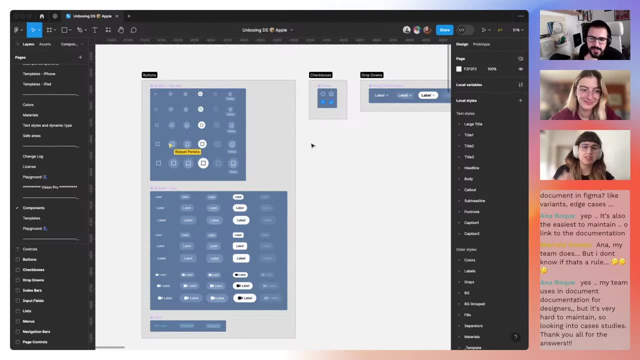 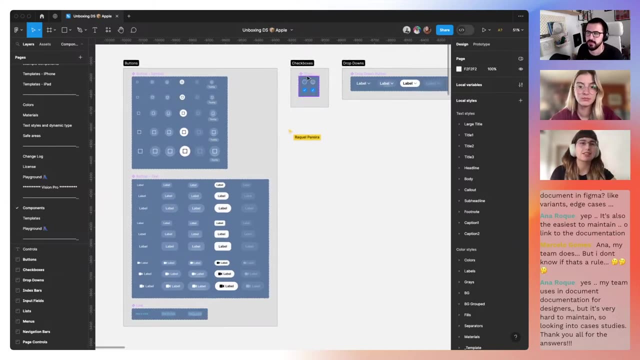 take a look at the components there perhaps, and then eventually start with the templates of vision ios, because they're vision, i think they're more. i really like the vision ios here because they can manage to pull uh, the backgrounds, like the, the opacities here, by just putting like a background. 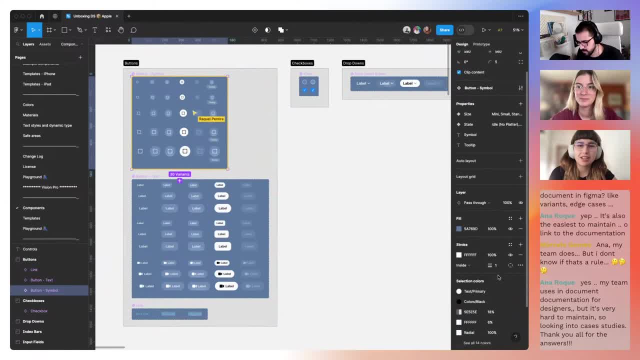 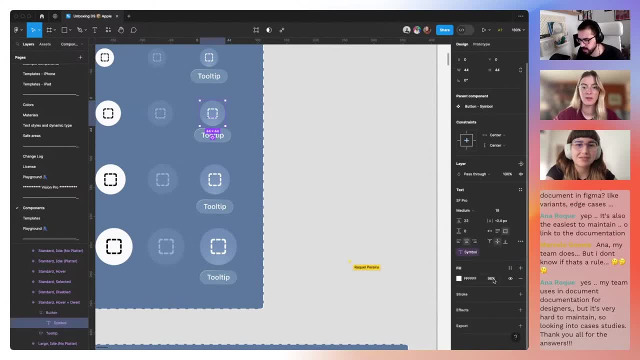 of the component and so we can understand when they're not. uh, the the amount of opacity and i think it's really cool. i'm just gonna try and see how they are doing the background. so they have a 96 percent. yeah, they have a lot of styles for what i see at glance. 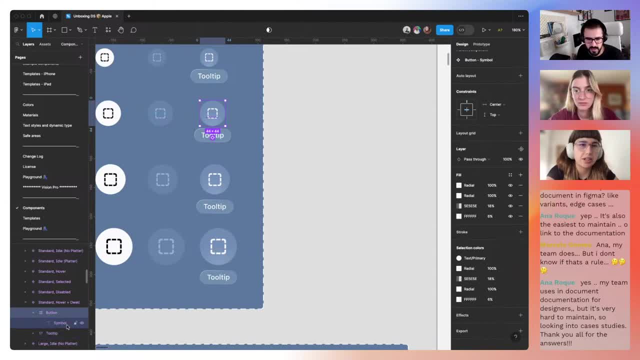 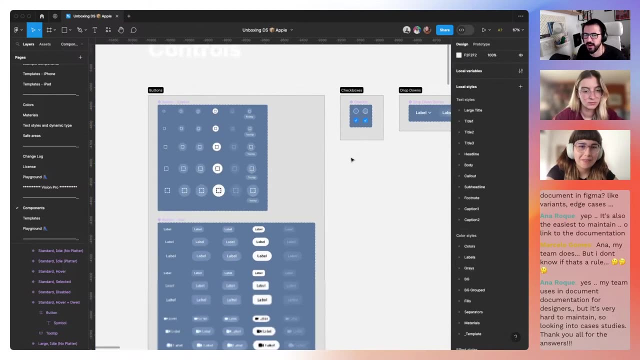 so it was interesting to understand how they managed to work and it's it's very minimal, clean, okay. so the tooltip, for example, i can see it up to the element of background blur, but yeah, button doesn't have a background blur. interesting, yeah, yeah, uh, but yeah, we could, we could look into creating a little uh example, for example, on vision os. 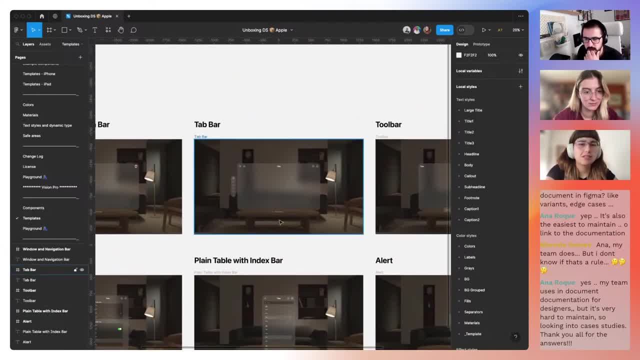 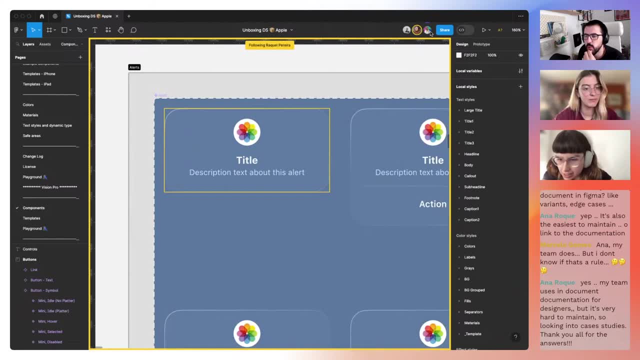 because it's a little bit different and more out of. yeah, so we already have also like this border on, on the alert, for instance, like this gradient: yes, yeah, they must have used it, because i think strokes- i'm not sure you have that struggle- but sometimes backgrounds, uh, shadows, are used as. 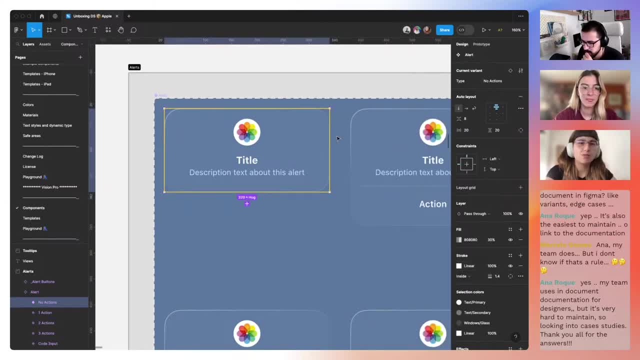 strokes and vice versa. i don't know why sometimes on css eventually they propose that, but it's also really weird sometimes to do strokes and shadows and because they on each one of them- maybe figma should dig in about that. uh, but this stroke is very interesting. i didn't know how they did it. 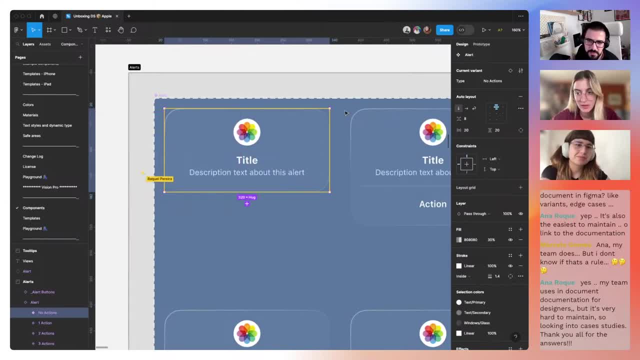 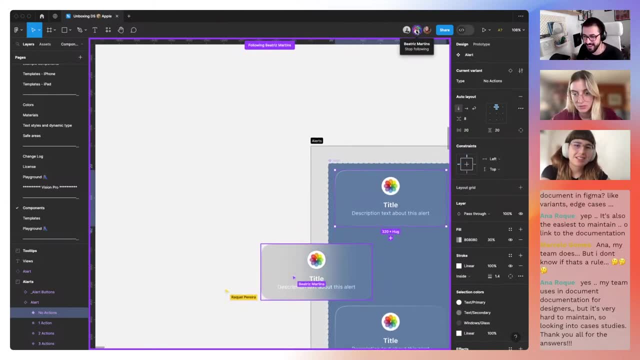 it's a, it's a gradient, it's a gradient stroke. it's a very simple thing. on one end i'm gonna say that i- i don't know if it's me- but i've played around with that type of stroke and like morphic thing a while now. it isn't new for me, but i don't. but it's. 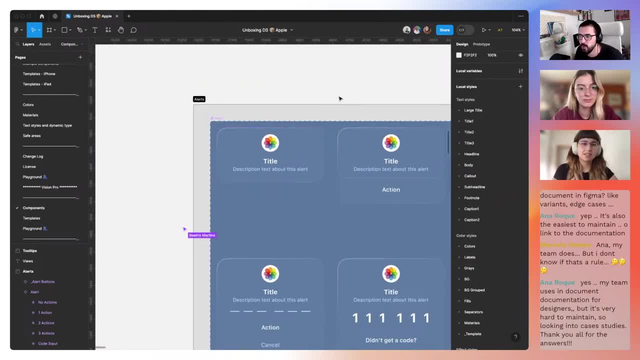 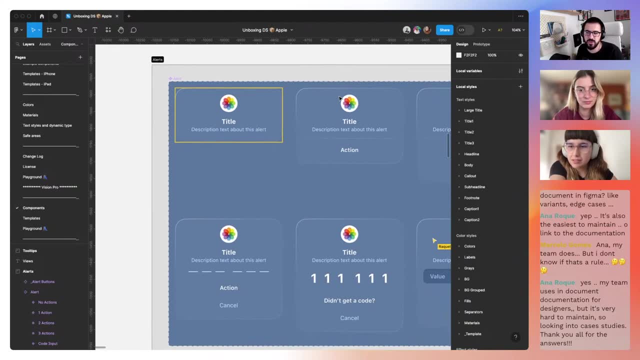 it's mostly about, like what you're trying to build with your system, right, like we went so much into minimalism that a lot of these things that give texture and dimension to the stuff that we build were lost. and now, with vision os, you're going to see the glass morphism. 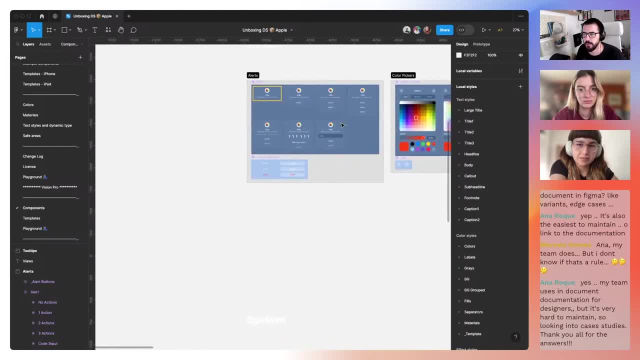 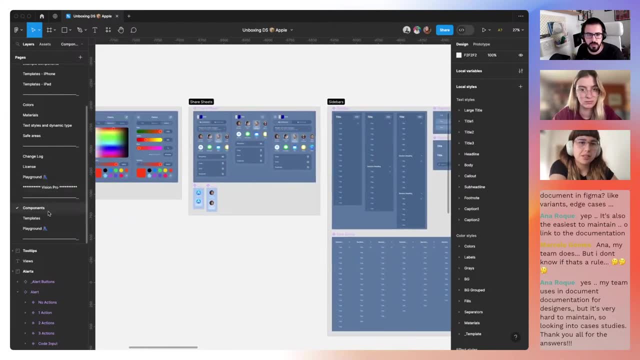 mixed with minimalism. on a different level, i think, um, and they did a good job talking about, like, the way that light influences the way that you're building and things like that- right, because, yeah, if we go ahead and, like, we go to the templates page on vision os, right, and we have a 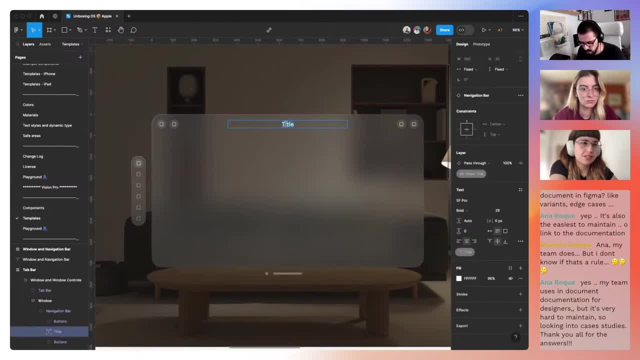 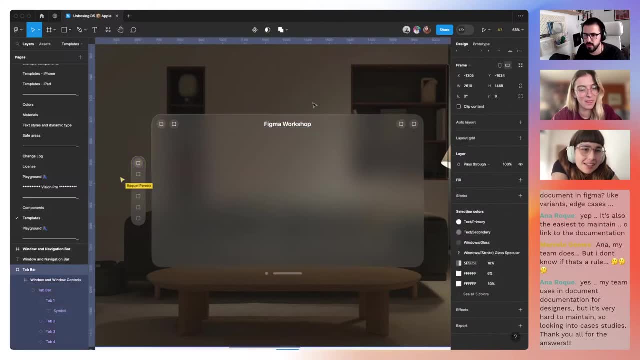 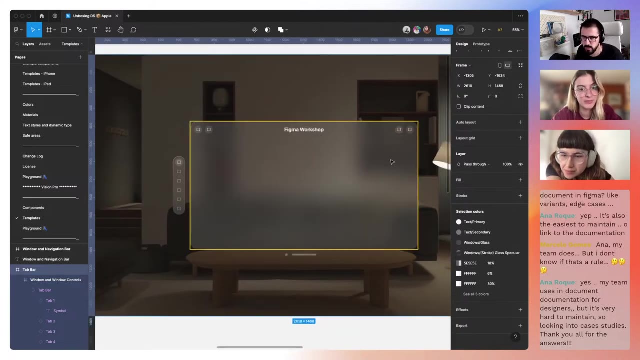 little ui here. let's say that this is our figma template, so i'm just gonna- i'm gonna call it our figma workshop. yeah, like the way that, the way that they use the simple background blur, they use a very contra, ambient, controlled image to be to just- let's make this sure- like they are using. 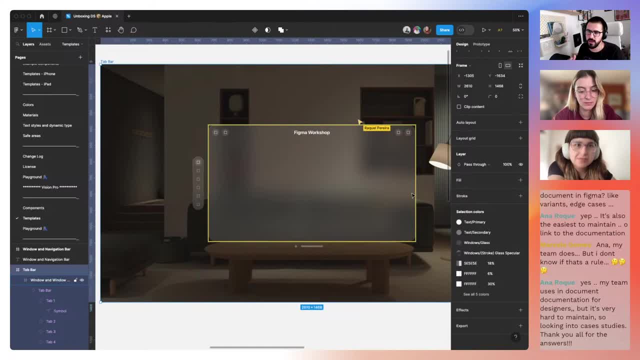 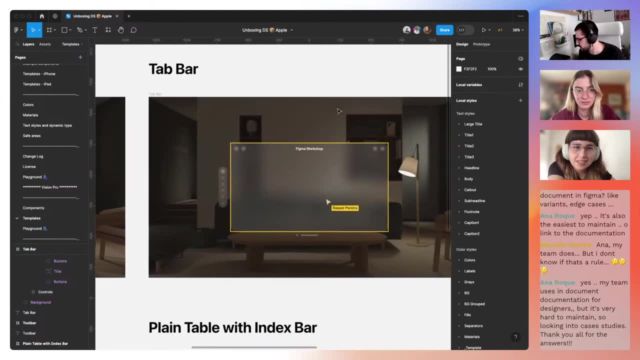 an example of what they would do in a very good lighting, i guess. but if you talk about, for example, if you want to make it a little bit more realistic, i'm going to say: let me see if i can do something. i'm going to try and do something stupid. i'm going to take a photo of my living room. 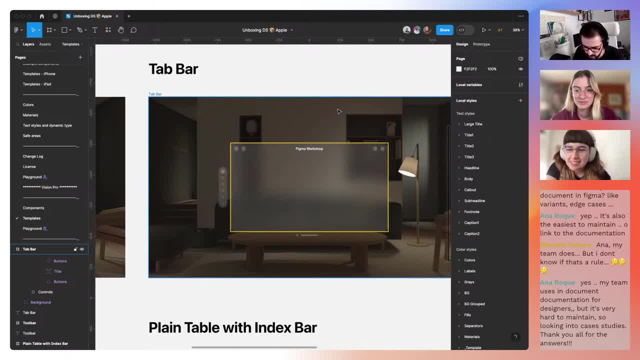 yeah, no problem, and i'm going to try and send it here and replace that background with a photo of my living room really fast and see like how we feel like it reacts to the yeah. yeah, in case it's smart enough for that right. i think they have a lot of potential to do a lot of variables for. 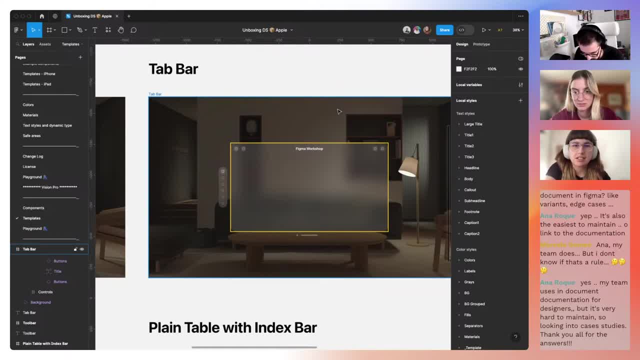 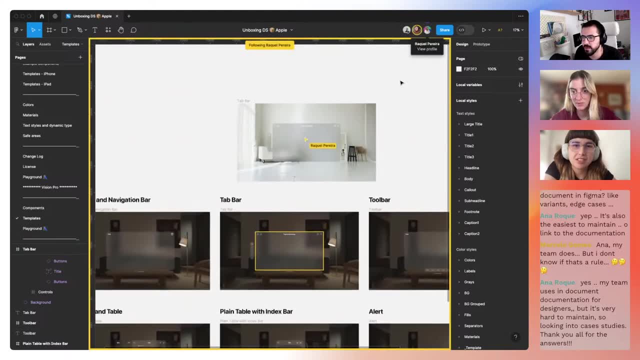 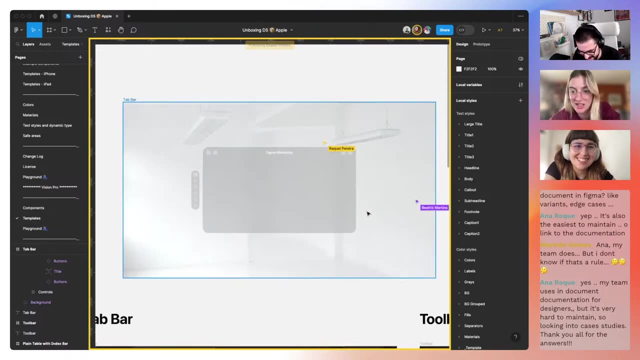 instance, i noticed that the stroke is still not a style that could be very interesting for them to explore. ah, good, i'm going to follow you, because i'm not looking at things, so they have a white background. yeah, yeah, they do work. and what about a great work? 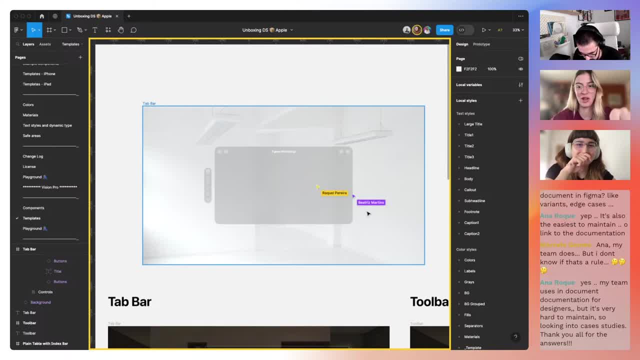 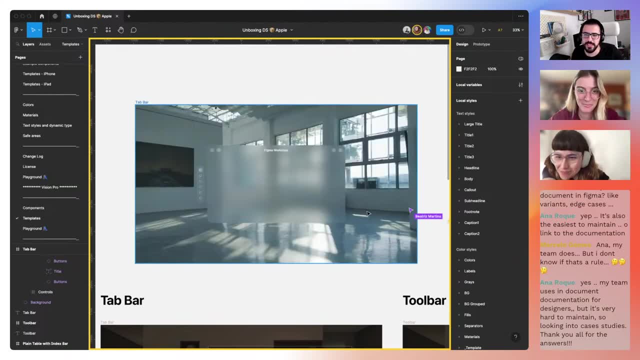 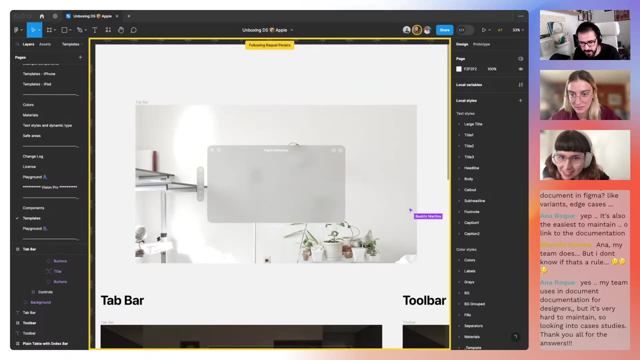 maybe gray one doesn't work. we're just trying to catch here, like the flaws like it, so i have fun here. yeah, it's just. again, it's using a background blur, which is not a bad technique. it's simple enough so that you don't really have to worry too much about it. but at the 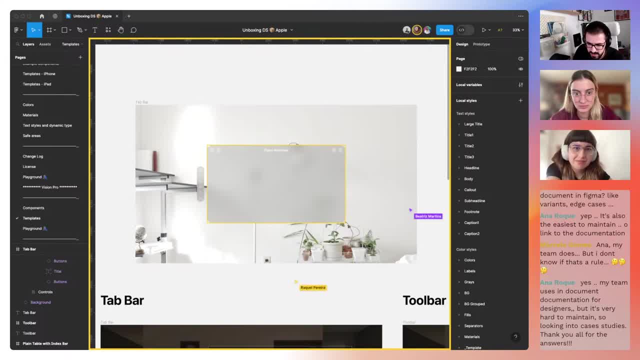 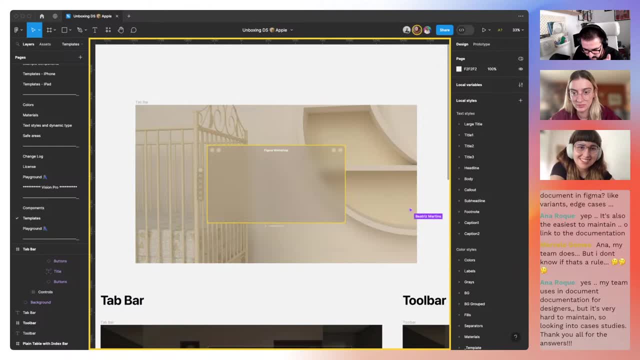 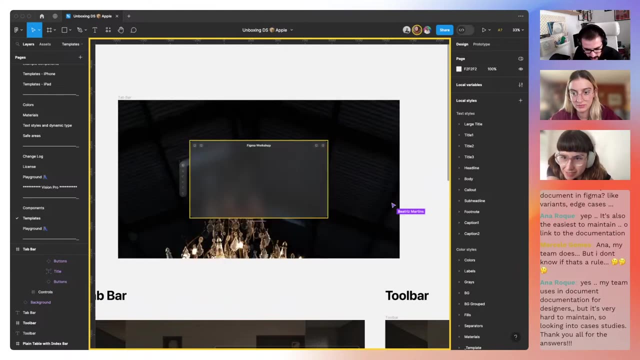 same time, i feel like one of the things that they did with all their demos- which they always do, let's be honest- is they were very, very, um very, very controlled to the point with the way that those things work right. so i don't know it's. i'm still very much interested in seeing how it will. 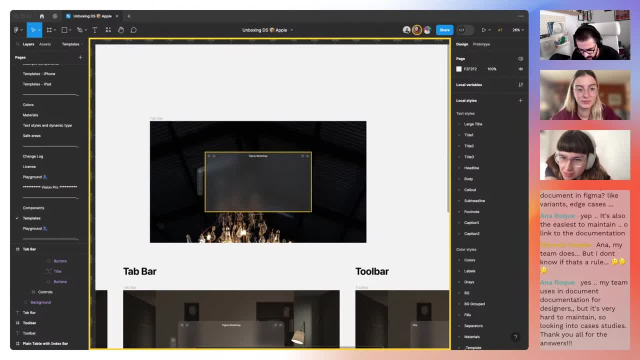 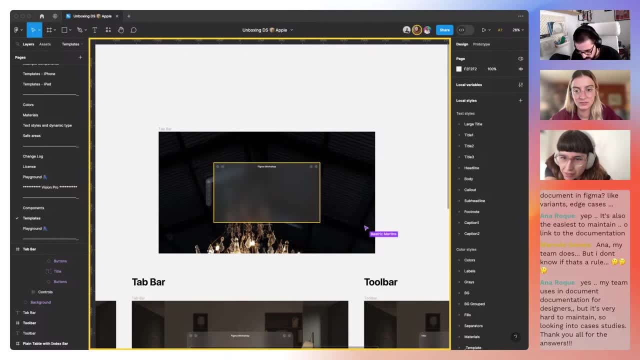 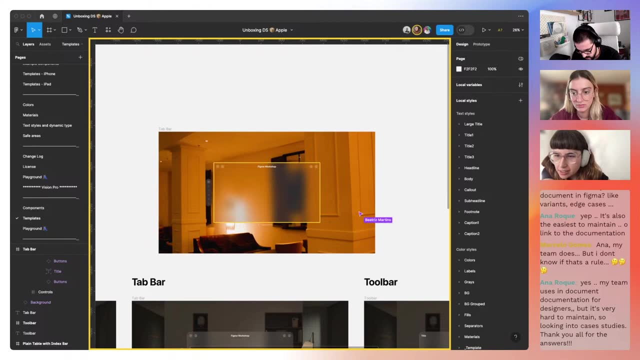 actually act in the real world, how people will see this thing, things, how they will navigate through how these products work and and what they do. i find it very interesting the color, because for some reason they i was. i was expecting that the glass would be an effect here above, but it's also a color i never seen like that. it's probably a. 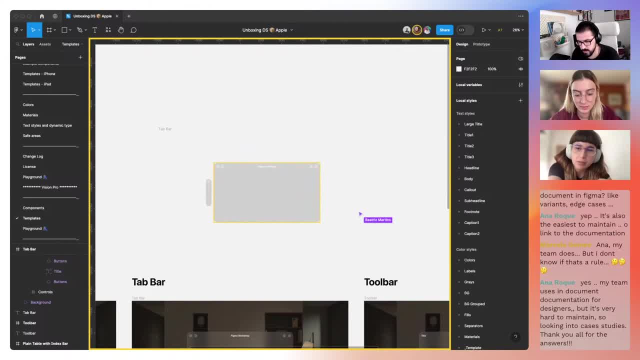 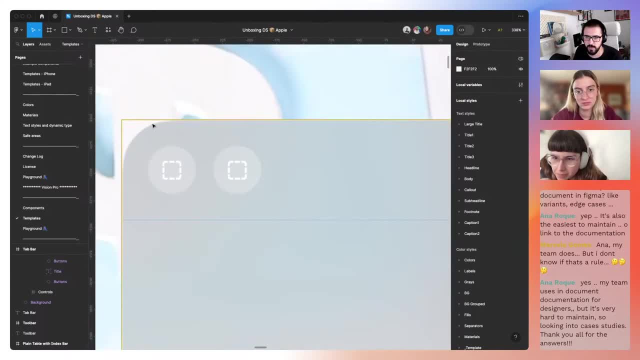 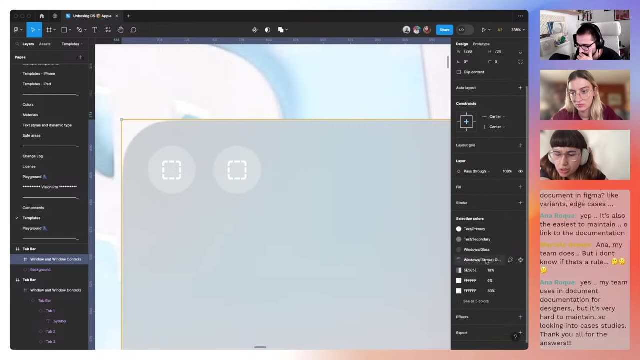 very specific gradient and combining with the black, brown, black ground blur, they do that effect. so it's interesting: are we talking about the background blur or are we talking about the outline? but both of them. so if you see the selection colors, when you're selecting the window, you have a color which is called window strokes, glass, specular, and then yeah, and also 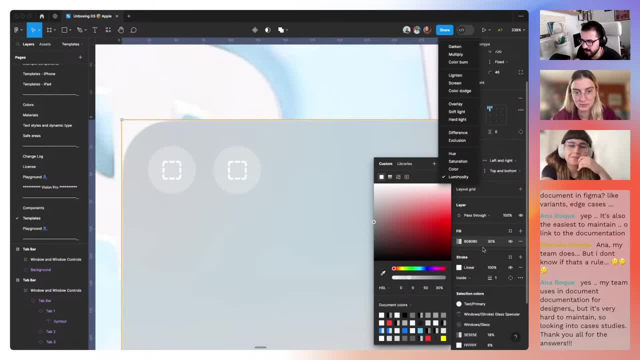 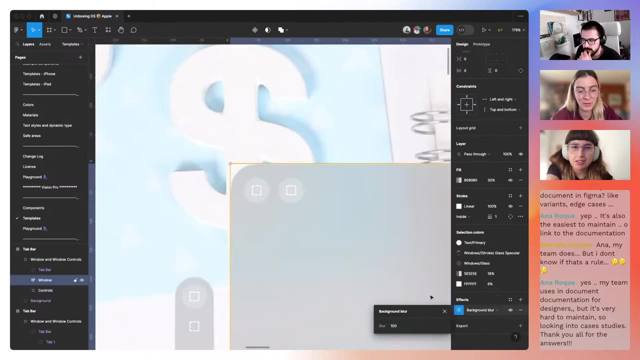 the window glass they use. then they also use luminosity, uh, mixed on the colors, so interesting. using using the layer blend modes, you get that type of stuff right. so yeah, and the blur is like 100 interesting one of the pixels. okay, am i the only one that it's really bland with this stuff like 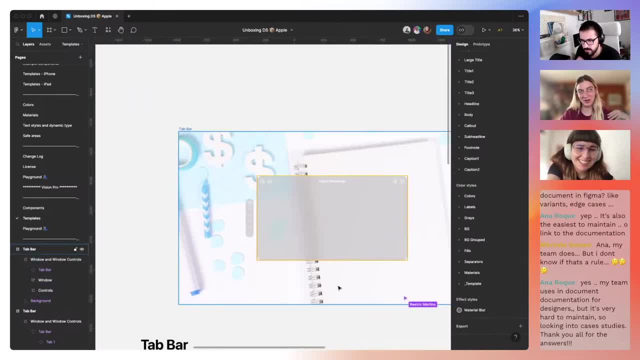 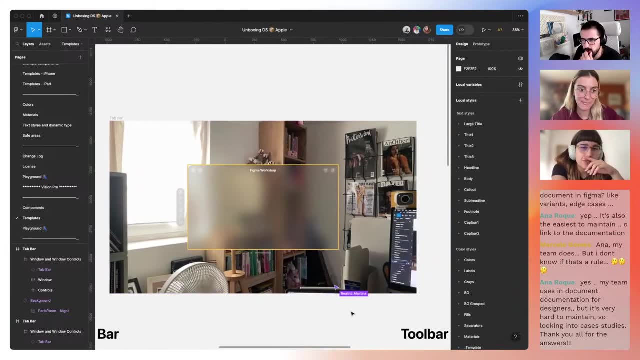 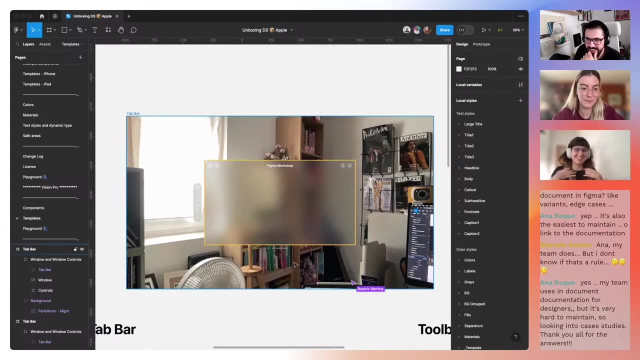 i've never thought about using like linear grading with opacity, with lightning, with whatever, to actually yeah, yeah, yeah. that's why i'm a little bit fascinated because i never combined that example. there you go: yeah, ah, good, bad, bad photo taken with my, taken with my phone. it works, yeah. 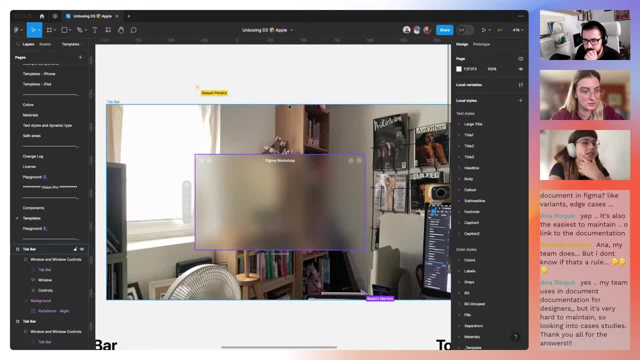 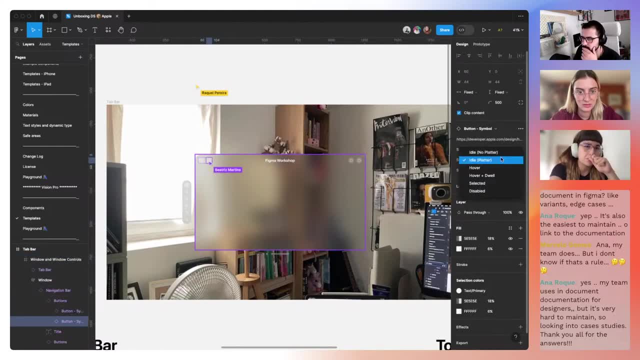 but it's good, right, it's bulletproof. i think they are very, um, even though that they might not be 100 figma yet on the templates, at least the basic ones are bulletproof, i think. and then that's good. buttons on the left and right and corners, and 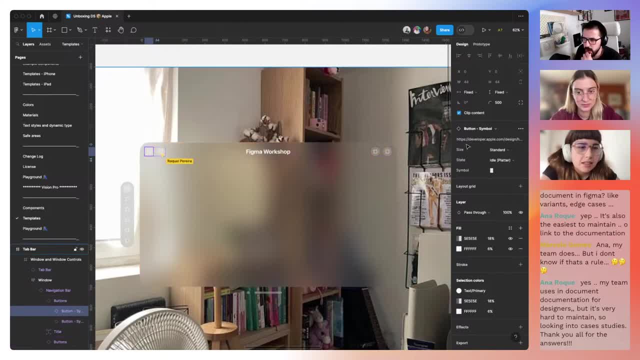 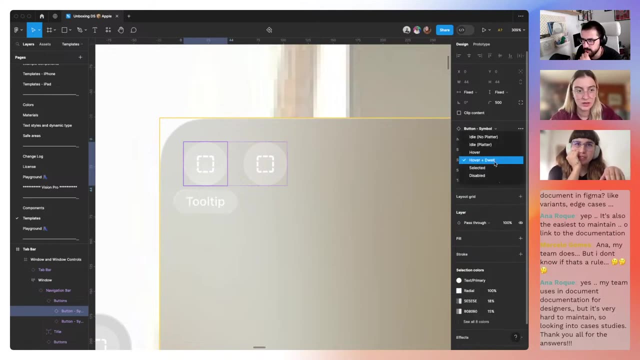 things like that. i'm trying to understand, like, would these be uh elements of, like closing or anything like that? like, yeah, what, what are these for? yeah, what's, what are the possibilities? right, and because for now i only saw that video presentation, not sure if you know about it- uh, it's really cool, uh, it's. 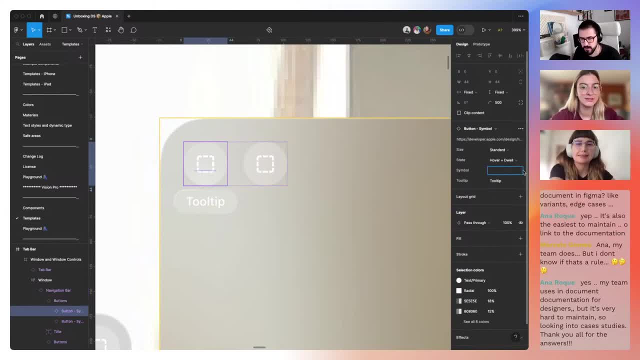 really fascinating, like i really want them, and then i see the price. i think no. they actually use a very interesting thing for symbols, which is they basically have their own library. it's a text-based symbol, so we can basically put any emoji there, any symbol there, and apple symbols are also part of the library. so, like they, they are assuming that you can use, like 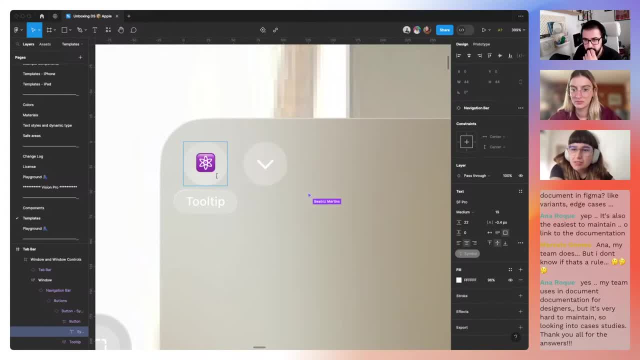 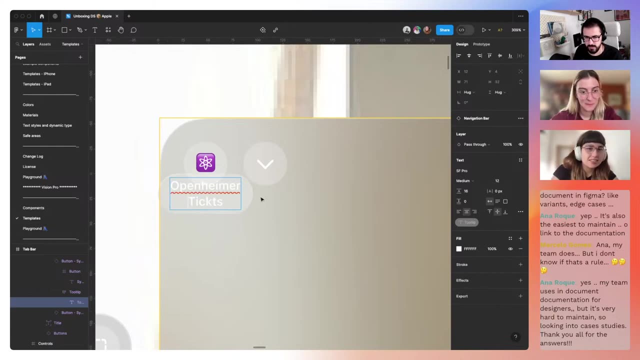 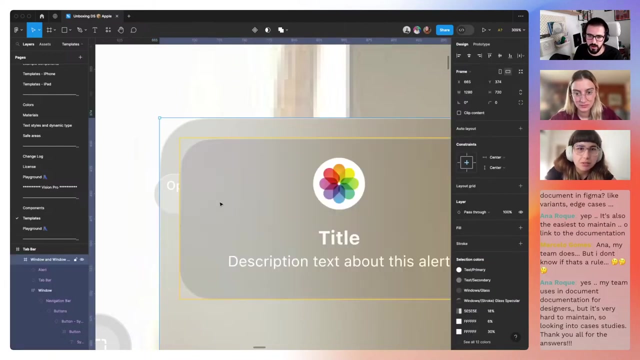 text-based icons: cool, interesting, interesting. how are they since? third, i hate them. interesting, uh. and then, regarding the components, we maybe might have their like an alert thing. i created a component that says open ama tickets and it has like the album, so i hope i don't hurt any. 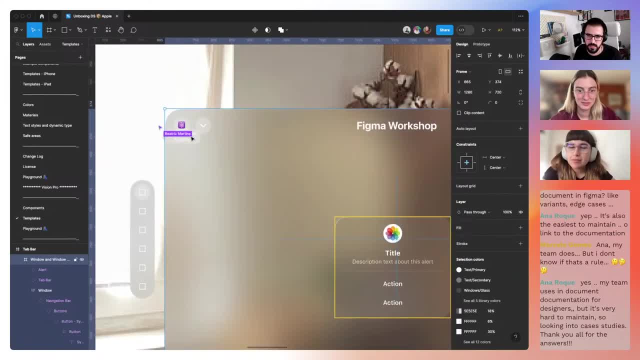 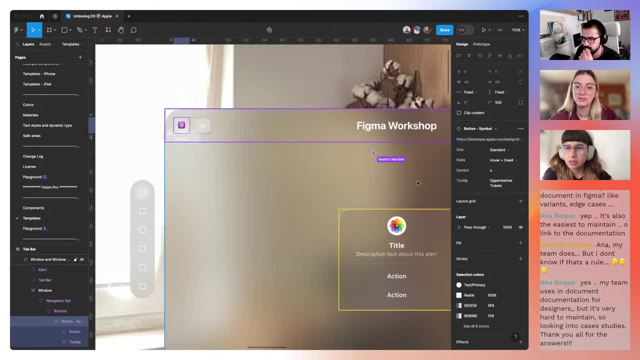 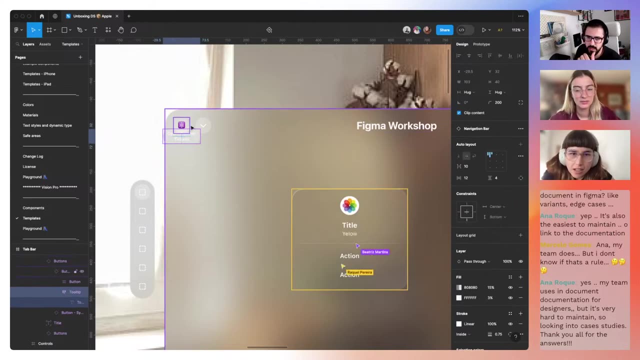 anyone's. ah good, but at least it's funny because they don't use auto layout. but they are quite strong on the variance uh topic. they are very organized, at least because they use the correct like the the way that it's built. it's using the correct uh anchors in the way that it's built. 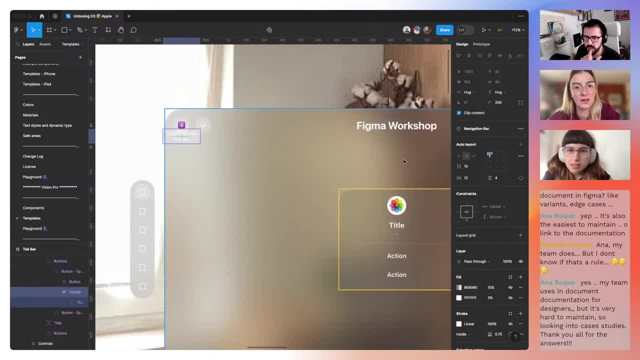 they do use auto layout, but usually they don't use it in the same way that we would expect, like the whole system to be auto layout, like, uh, there's some stuff that he felt that probably they felt like he needed to be i don't know. uh, he needed to be like stuck and i don't know when. 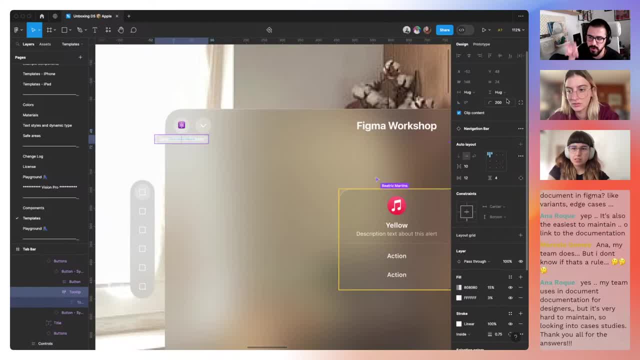 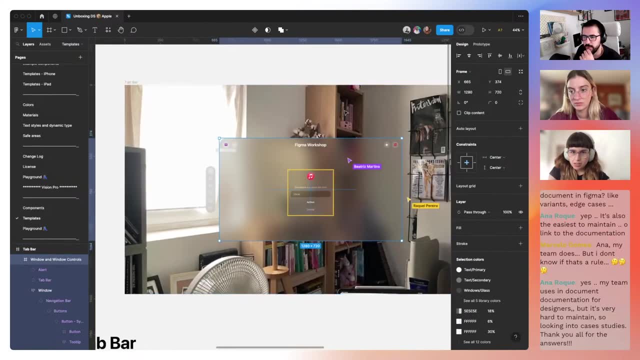 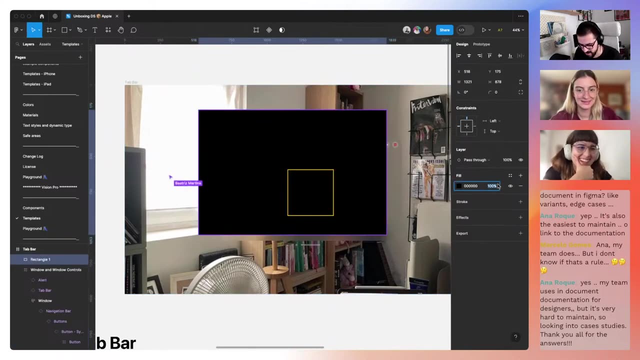 they did this, but maybe they didn't use the auto layout fixed component, they used others. so, okay, interesting. so this is an action thing. so what would happen when you get something like that on screen we maybe need? we're probably missing something like this. yeah, at least i'm just trying to use their components, uh, like 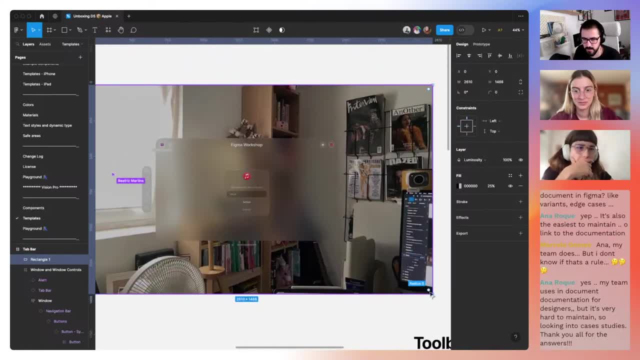 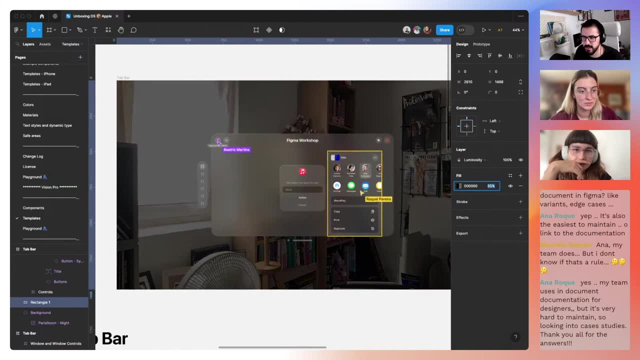 i don't even know for what this is, probably for calls. let me put it here, let's see. but they are very strong regarding so you get, you get an alert. the world gets dark. yeah, and, by the way, for those who are still with us in the chat, if you feel like we could, 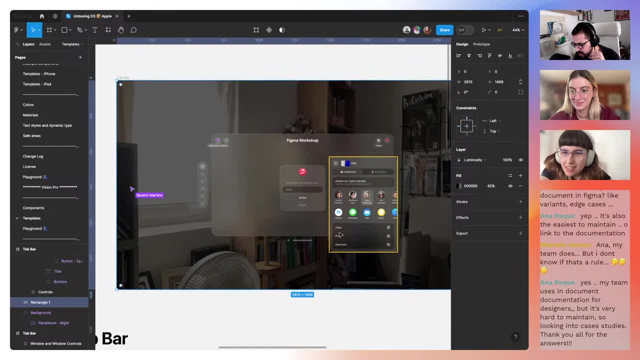 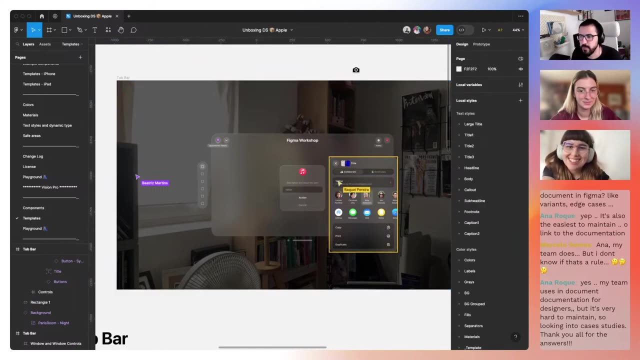 we should create something here. tell us what you want us to play around with. we still have about 15 minutes, so we're literally not making any sense right now. so maybe, if you feel like we could do something cool here, we can try. i know what i'm gonna do. i know what i'm gonna do. i'm gonna go all meta. give me a second, okay. 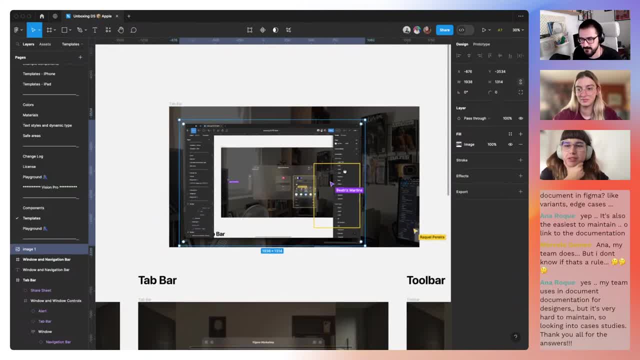 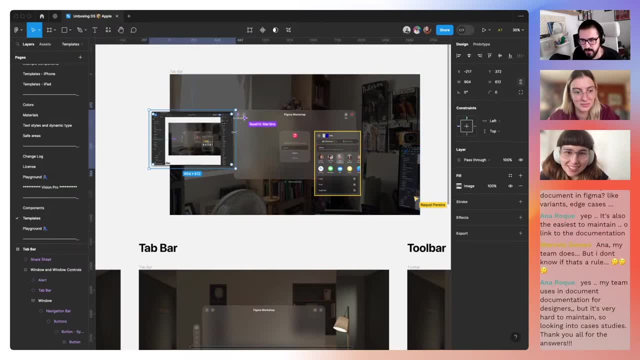 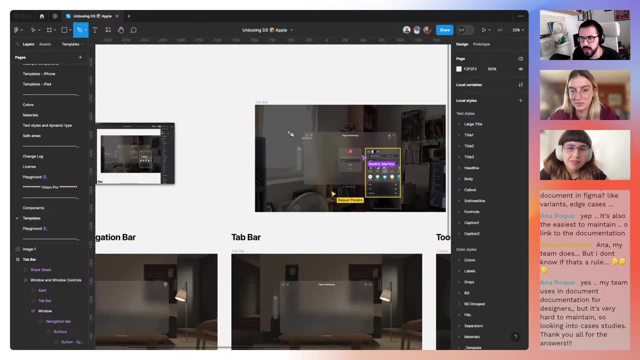 but at least regarding variant wise, i think they are very good for the start, i think, exception. so we have figma inside figma inside vision os and i'm actually i'm actually going to try something. i don't know if you guys know this plugin, but there's this plugin called 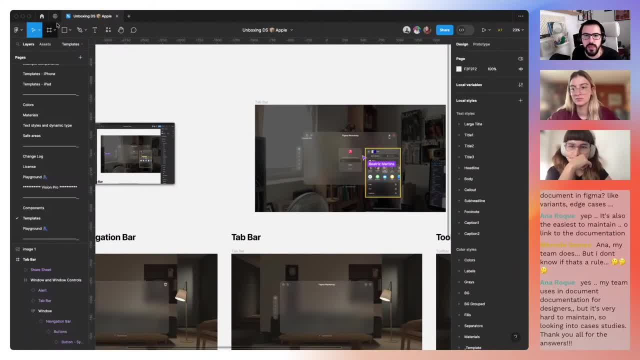 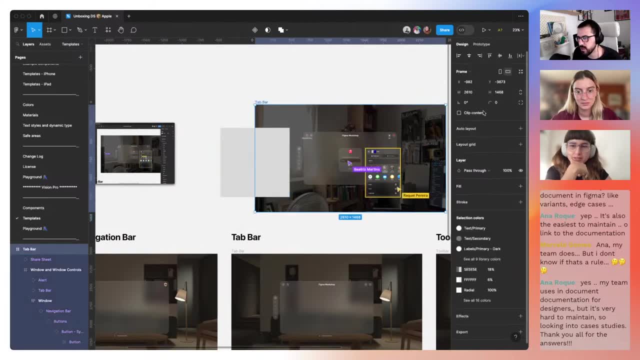 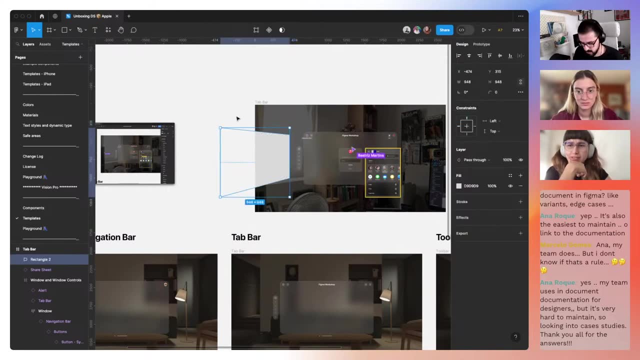 um angle mockups. i think you need to start with a rectangle to for it to actually work. but let me see, i'm going to try it with, like, figma on the side of the screen and i just need to do something like this. so amazing, for so far i haven't seen any variant. 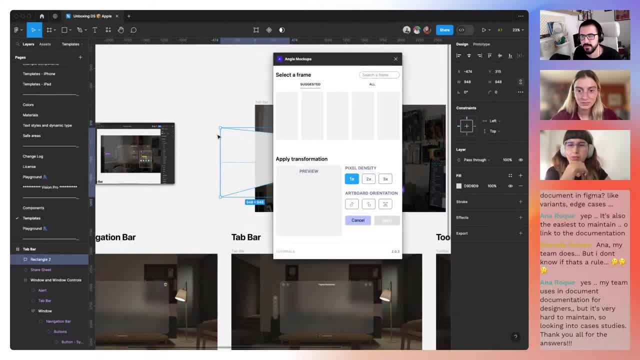 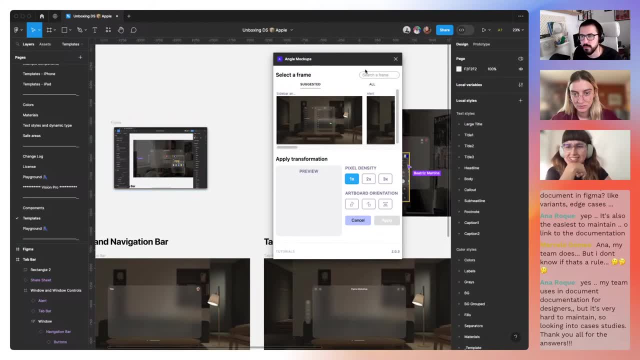 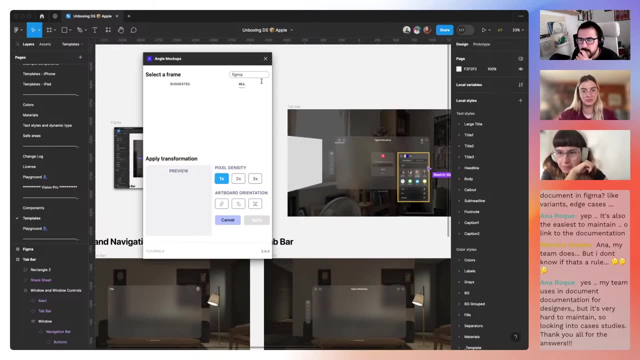 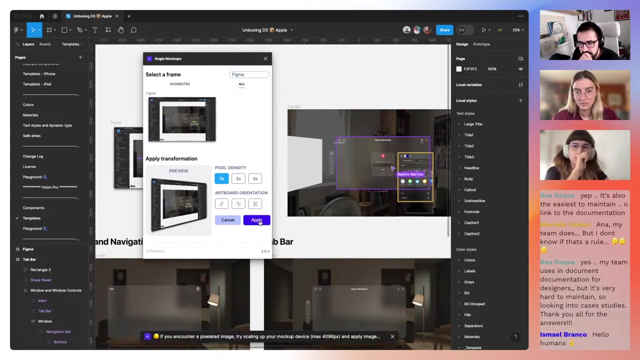 broken uh inside when i'm just like going around. so someone's just tried this and study and tested this really hard. i think- or at least they probably are so consistent already in their sketch files- that going here could be more easier. but it's interesting, at least variant ones. i think it's interesting, like with the swap instance and so on. 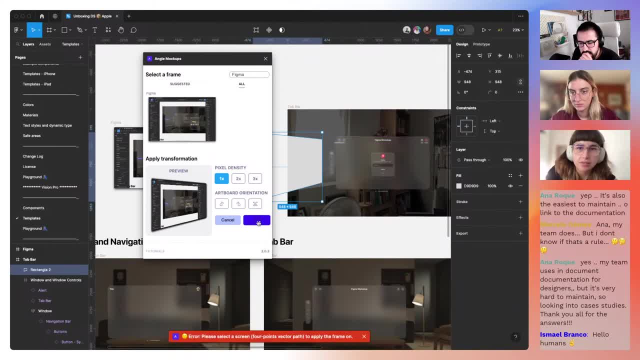 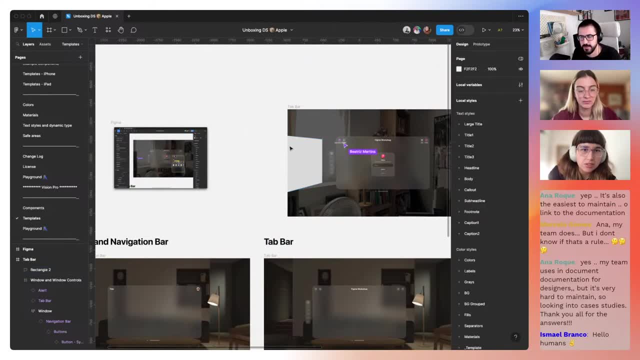 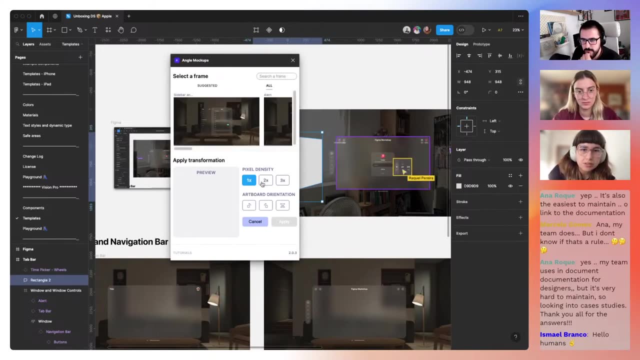 good, let's see other components that they have. ah, jesus christ, i think they also don't have that much features, to be honest, because it's still new for them. i also really like this time picker at least it was cool because it's already their personality to have that kind of uh timers at. 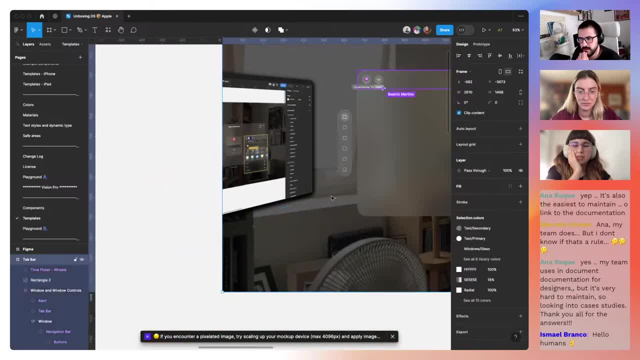 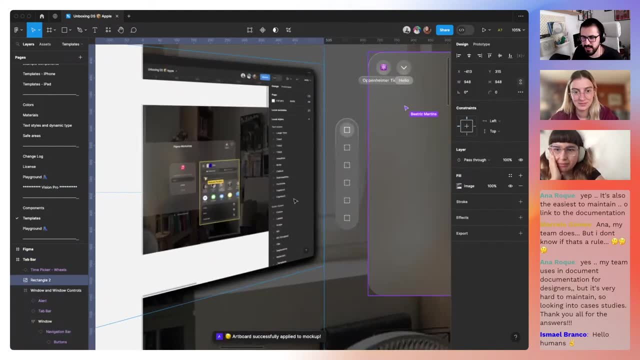 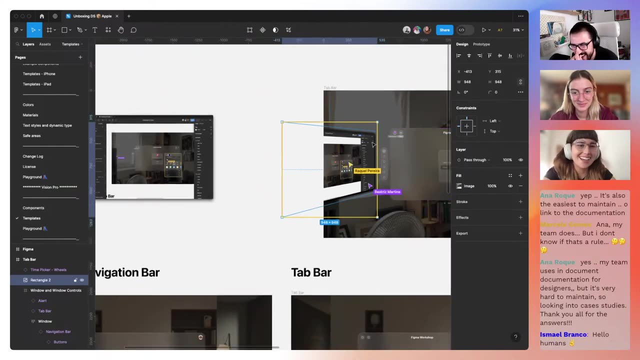 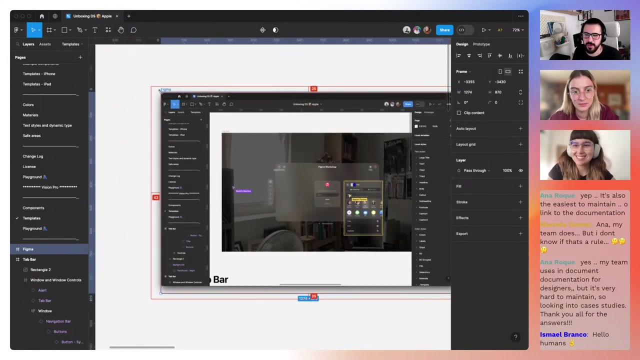 least, sometimes the hours on the android is a little bit ugly and this one is a little bit more fancy. so, oh, amazing, figma is floating inside the system and we are inside figma and the shadow just looks creepy and weird. wow, i don't know about you guys, but i actually, when i when i'm using um apple systems, the this thing is: 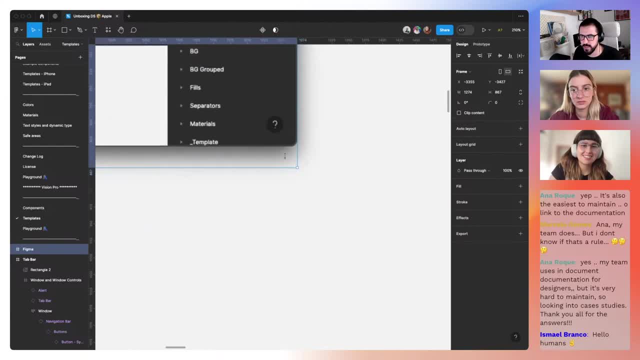 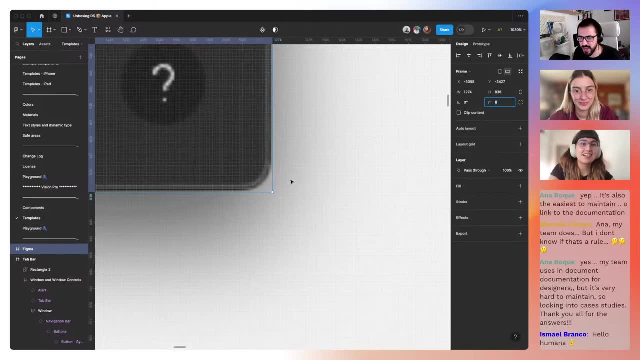 something that i need that i didn't knew up until very recently. so if you do common shift five, you can actually take a screenshot of a window very clean, but it always comes with the shadow, and it's the shadow that i get like i'm i'm pissed at because the shadow creates that weird effect. 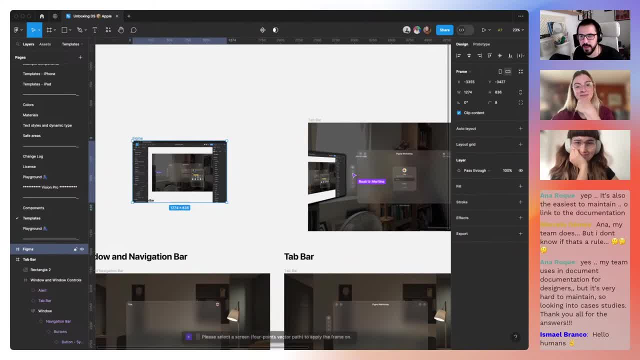 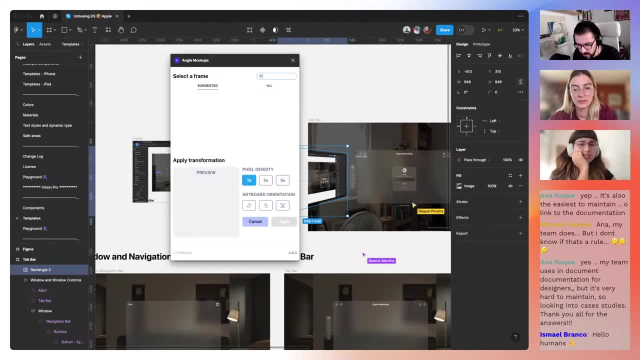 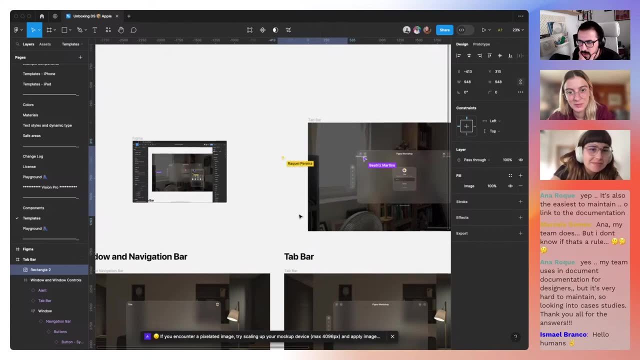 and it it just breaks the thing. so let me see if i can fix that really fast. select this angle mock-ups: i really like the shadows. so yeah, it's a little bit ungrateful and you want to get rid of it. no, i'm gonna. i'm gonna take it out, but i'm gonna use native ones. 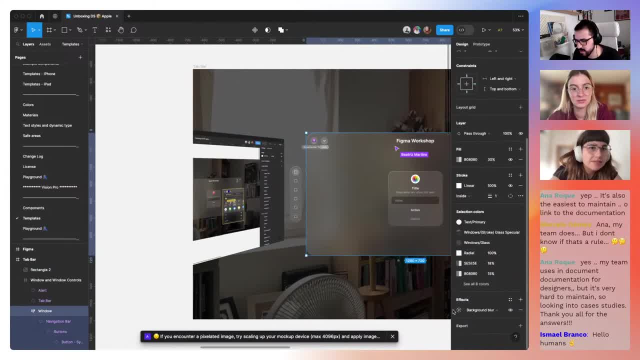 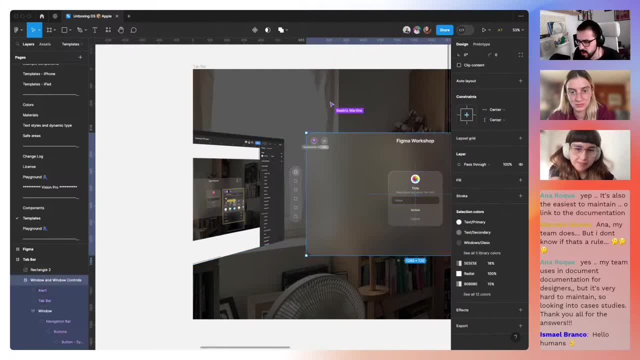 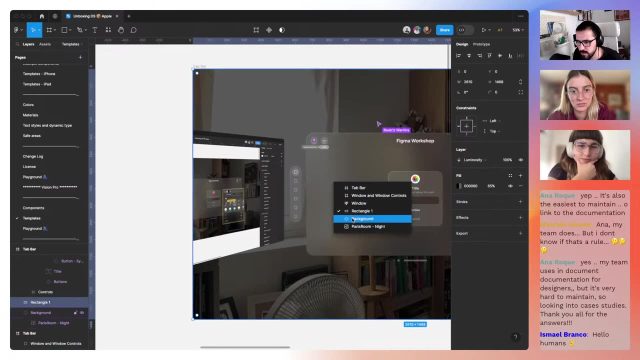 right like let's. let's try and get the stuff that these guys use, um like, for example, if they do have the little shine around. so we have window, window and window controls. where is it that i can find the background? no window. where is the stroke? i can probably apply the same stroke. 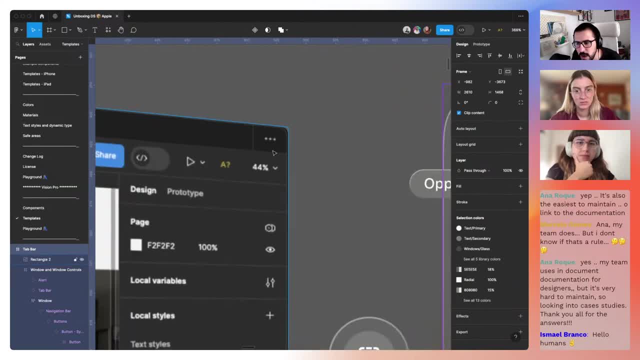 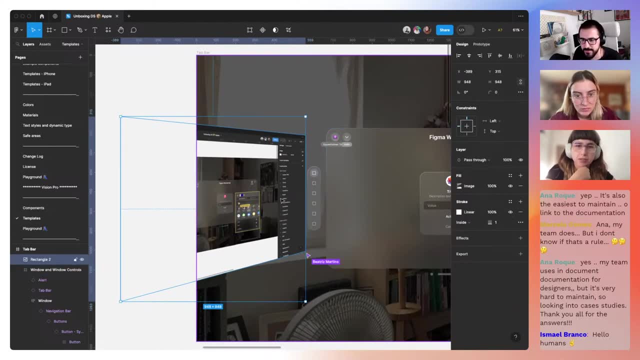 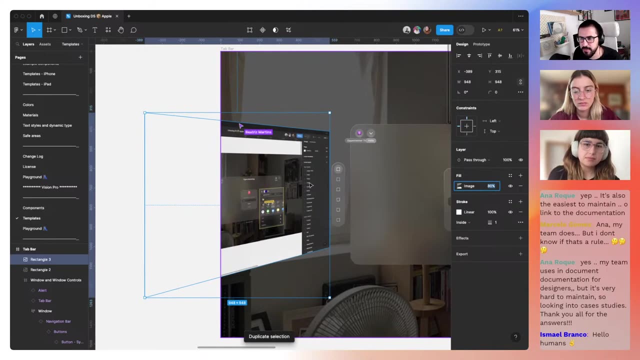 on the window of figma. see how it looks? yeah, it's. it's because it's not a style. it could be tricky. i think you have to manually. yeah, go for it. you can also, like, do something like this, where the ui is like half like, and then we do a little masking here and, yeah, i mean it is showing. 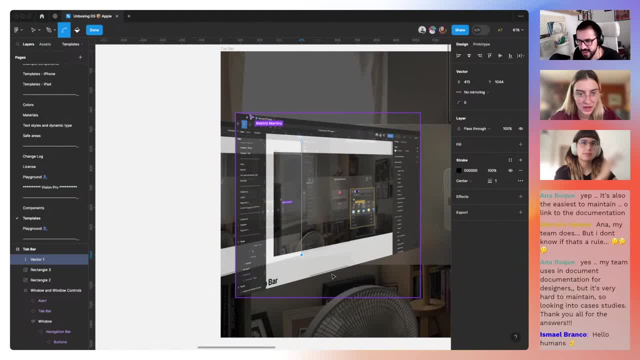 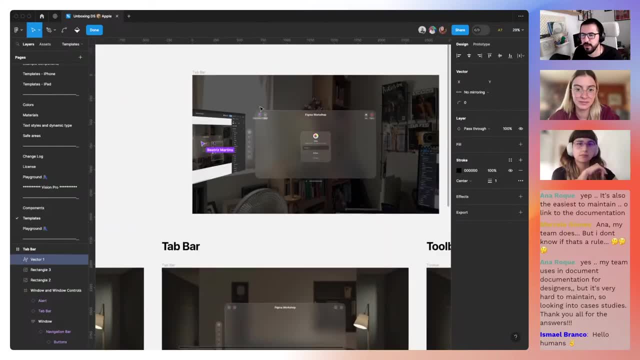 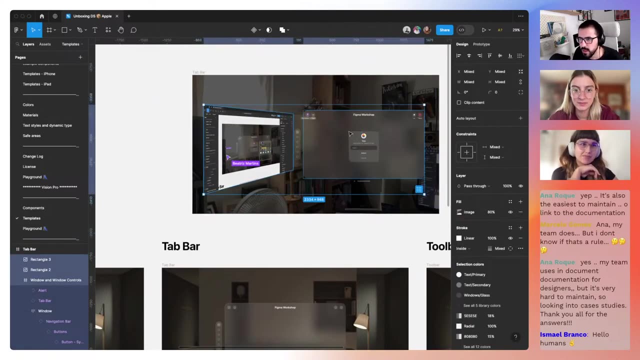 but it's just like wait, sorry, you see there, like on the, yeah, but it needs to be put in, and like we're, we're actually using it like this: i'm gonna do something there that probably seculages for apple, which is: i'm just gonna do this, i'm gonna select this and okay, now it feels more like vision. 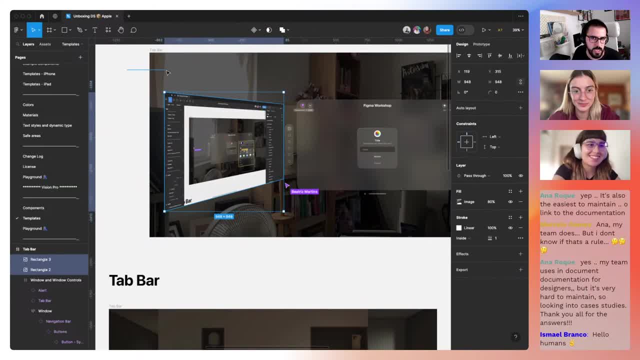 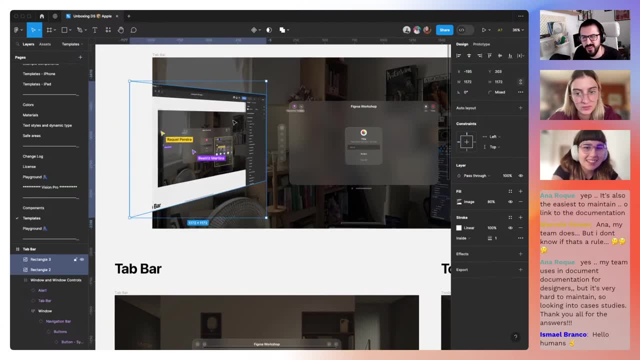 os with people like having multiple. yeah, because one of the things that i usually get bummed with this is like when people are trying to design for the systems and they use these very clean files, it's great, but like you're designing this, but this is going to be affected by your field of. 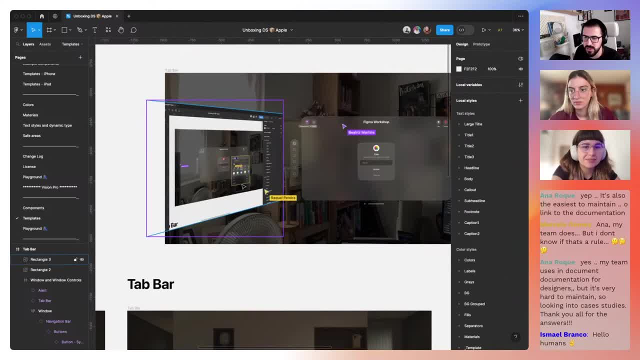 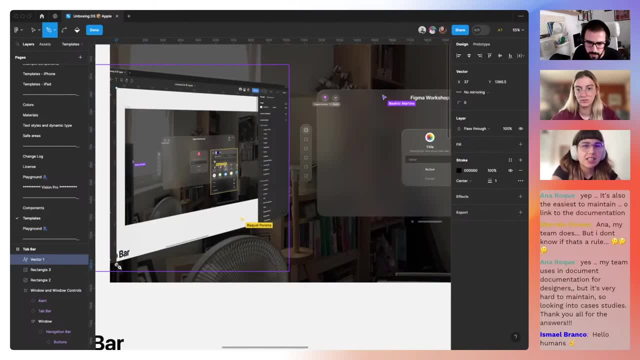 view and you need to test out with other windows and things like that. i feel like, yeah, didn't do a good example, a good job of creating examples like that, like what would happen if you have a few of these open at the same time. yeah, i think they're still doing baby steps on the windows. 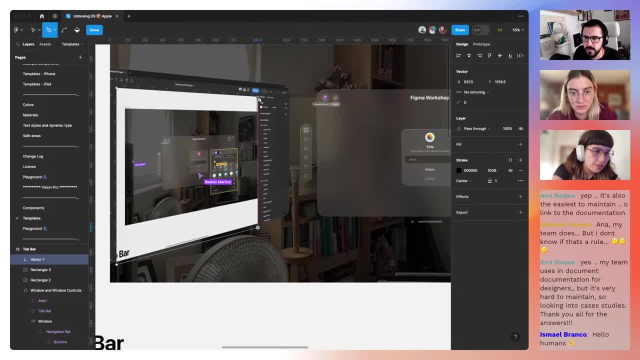 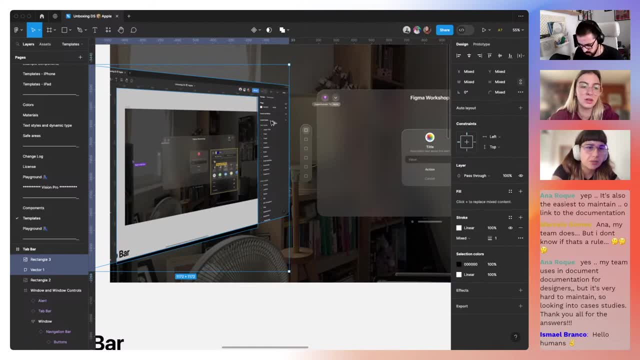 that matter. they also have here, uh, regarding foundations, they have a little bit of colors and textiles, yeah, and also some stage areas, which is also a very funny topic, yeah, but the colors are very minimalistic, yeah, yeah, which makes me think, like what happens if they need like a really light? 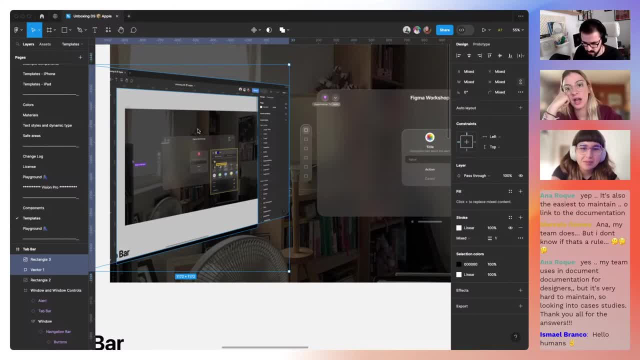 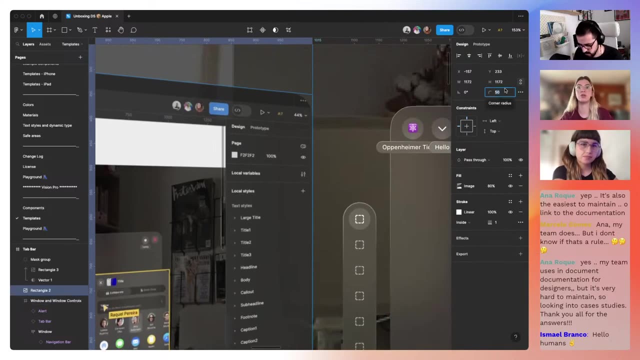 red, like i don't feel like it has that much uh potential, while doing new components. i mean, i feel like this design system is very closed. um, you cannot do pretty much anything, uh, or be creative or i don't know. allow designers to actually do new things. so that's yeah. i don't know, i don't. yeah, i. 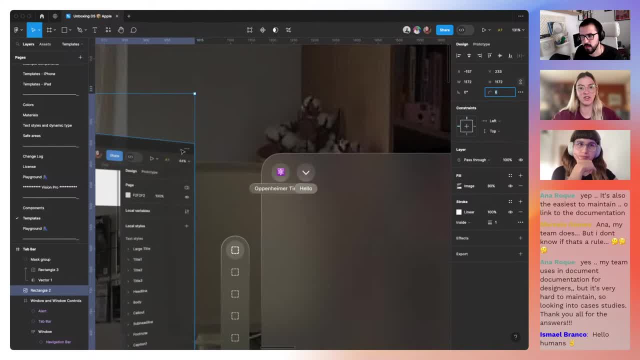 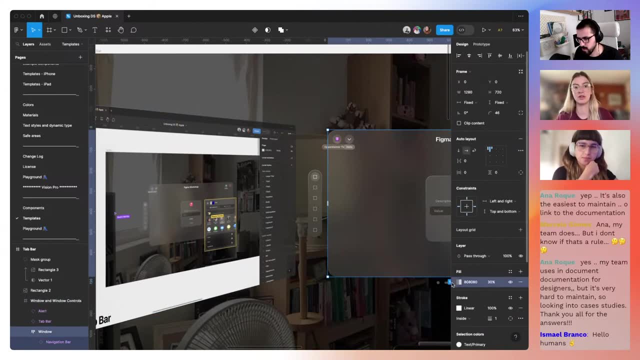 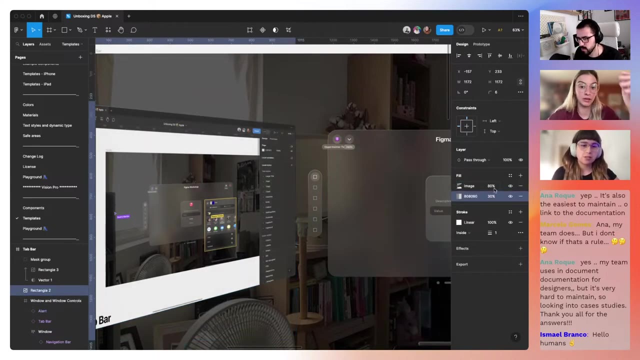 mean, i do, i do like uh, designers in my company to actually do whatever they want and then we can review that component and see if the- um, the colors they are using are the good ones or not. but here it feels much more strict. um, yeah, and probably that's the goal, you know, not to give that all the assets that they have. 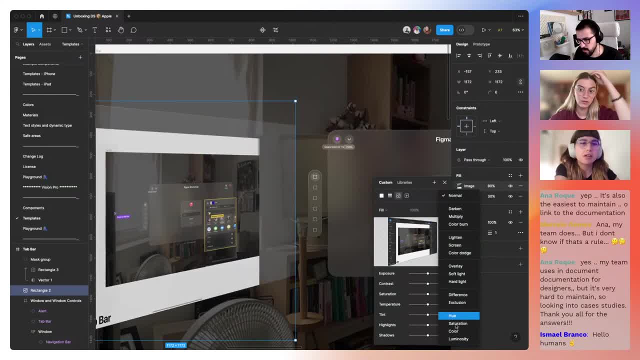 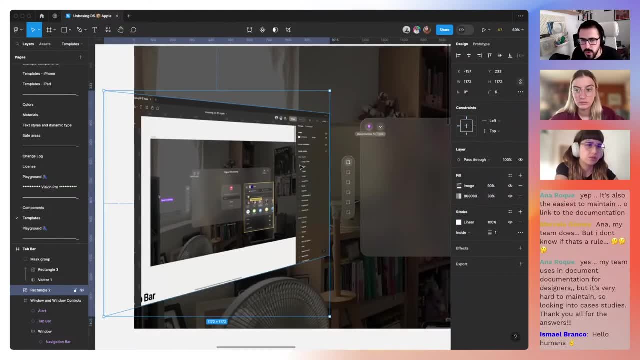 internally, because i suspect that internally they might have a lot more. so maybe this is just the main colors for the overall basic stuff, like, if you want to- i'm not a wizard but i'm managing to make the window work kind of like it's we. we made figma for the vision os, i think. 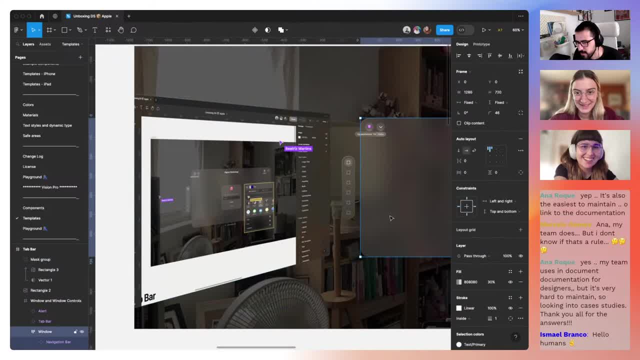 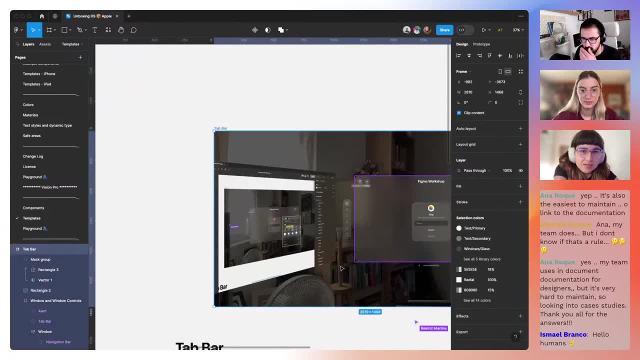 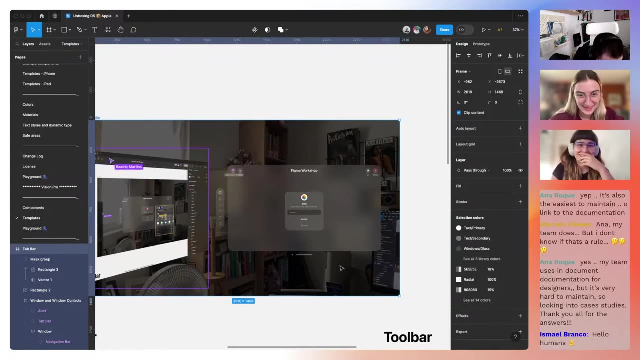 we're starting to get there. i'm missing the background. where's the background? let's see, there you go. figma for the vision of us. it's done. thank me later, by the way, a low email for joining us, as we are basically just ignoring. no, i'm just kidding, it's. 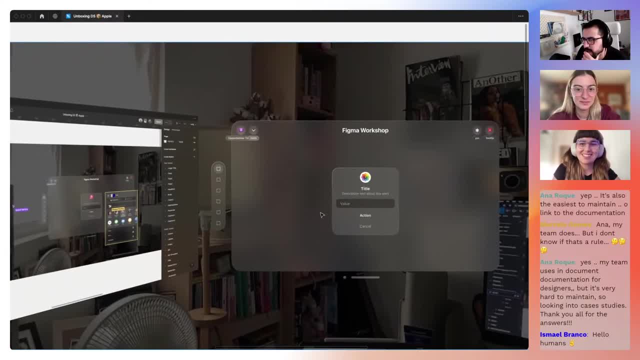 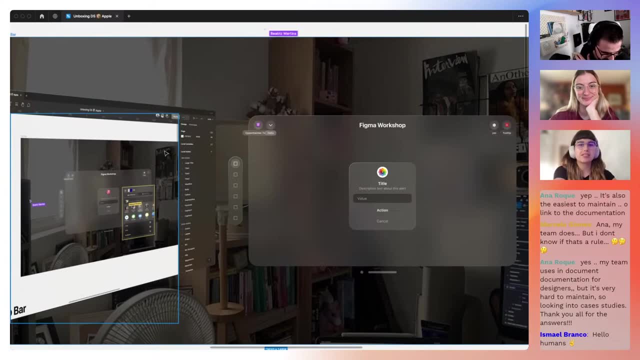 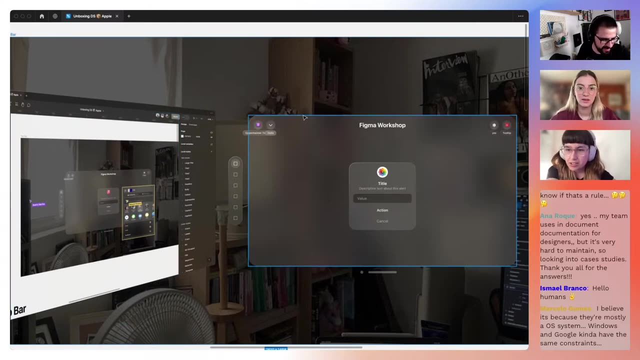 just me. they are doing the job i. i just got lost with time. no, no problem, you're also entertaining me and you are taking a tip of the iceberg about how you talked about the here in sigma. ah, i found one with auto layout. so it depends on the situation, at least on templates. 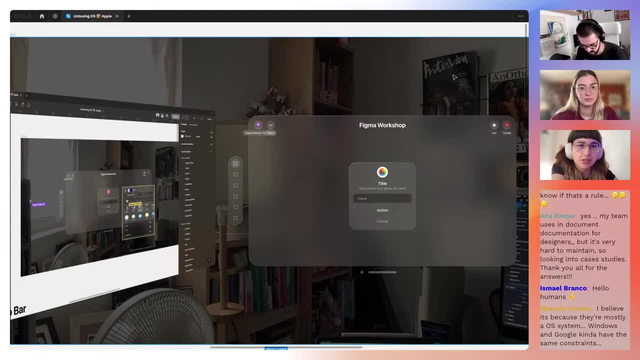 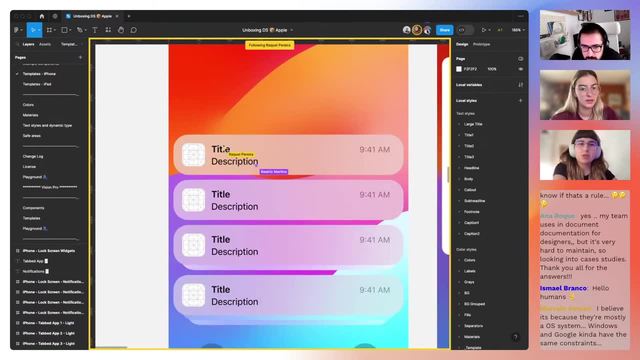 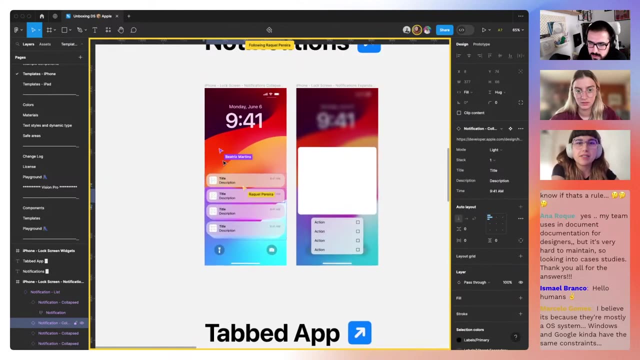 if you follow me, this one has already an auto layout. give me a second. i need to look for you. this one is so. maybe it depends on the effort. sometimes they probably just did it, others don't. maybe they didn't have this one so when they're creating they already considered auto layout. 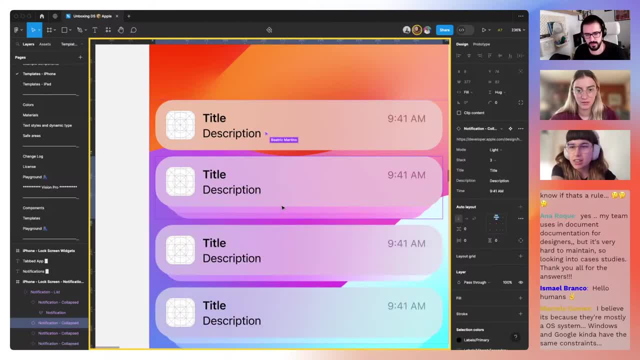 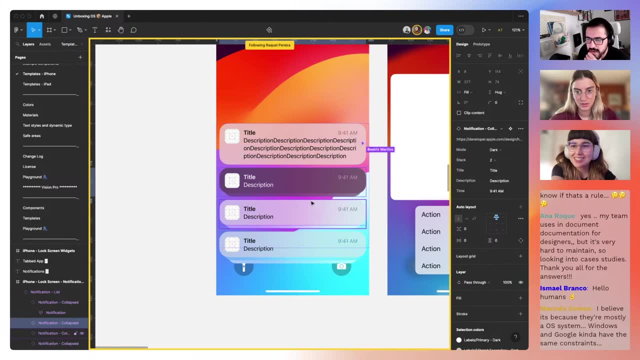 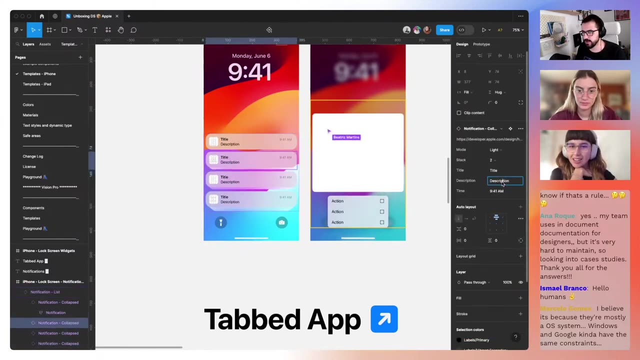 and this is very interesting, like, even though that you change anything, they don't break, which is amazing. yeah, no, it's. it's always fun to see how these things work like. and again, one of the things is they are still. they are still trying to- uh, they are still trying to. 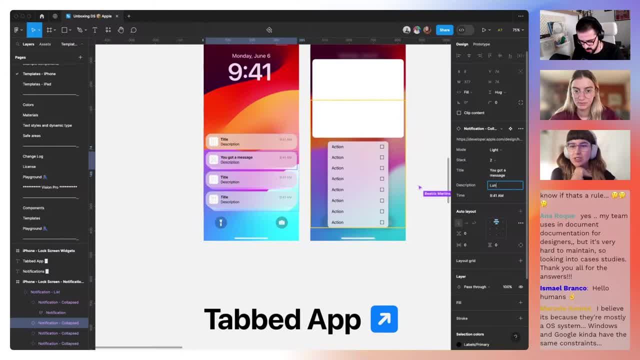 build the system for sure if they are coming it. uh, look at this one. it's insane. wow, you know what that one reminded me of? right, i'm gonna try and open the video that i shared the other day on x? um. while i open x, i'll i'll share the the video with everyone. um. 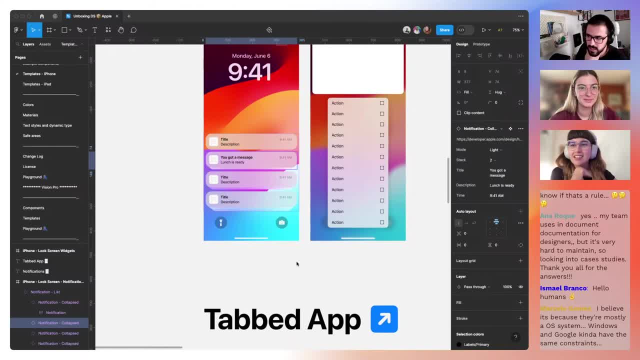 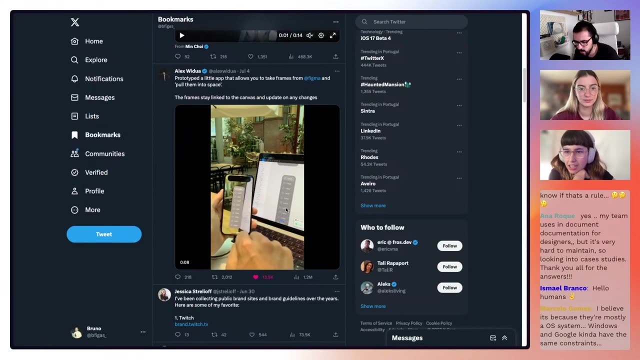 really, as soon as i have it, which was? there's this uh guy, alex wida, uh widua, i'm gonna, i'm butchering his name. that is actually using figma's api to catch these components that are vision os, the ones that you were just playing with- and he is making this video. let's see if i can zoom in. 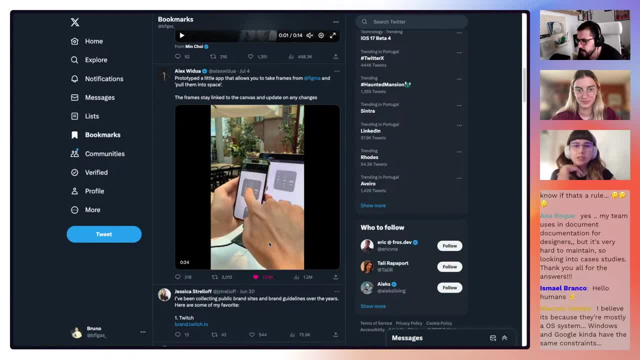 no, i can't. but like here's the whole world on the templates, he's just picking up those components and like testing them out. that's a very good video. it's inspiration. so if anyone here wants to create something like this that it's easy to use and put it on the community, thank you, yeah. 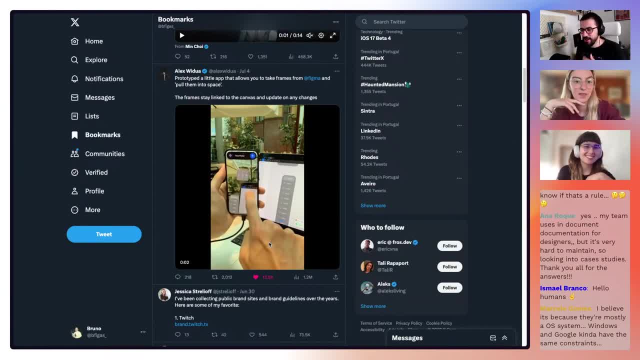 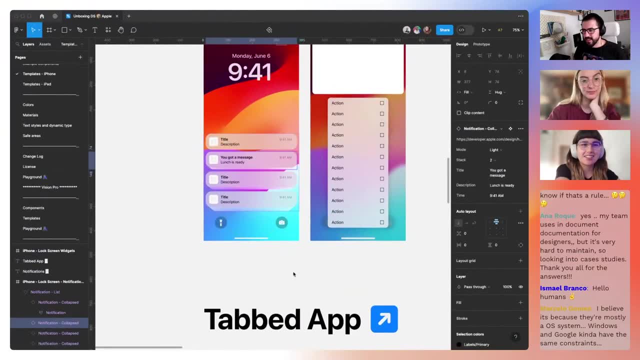 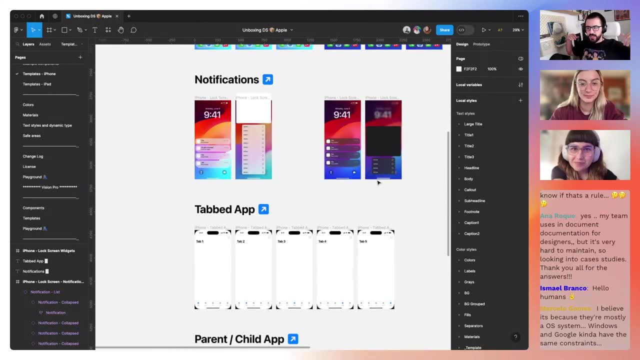 uh, playing around and testing these things, yeah, it's so cool, um- and i'm just gonna go back to figma, but yeah, testing ai with ai it's, it's almost like the same thing, so i don't know like it's. it's one of those things where i would love to see. 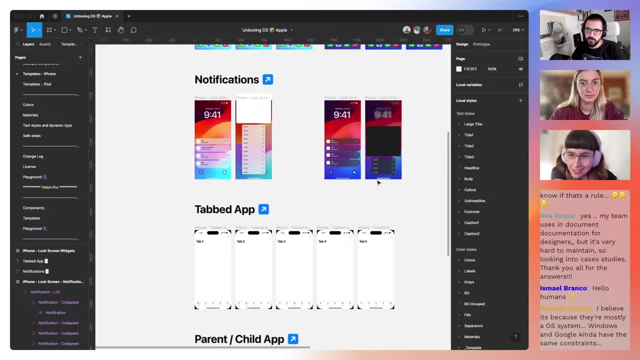 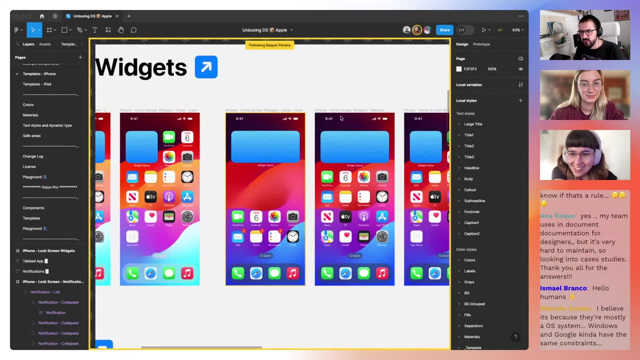 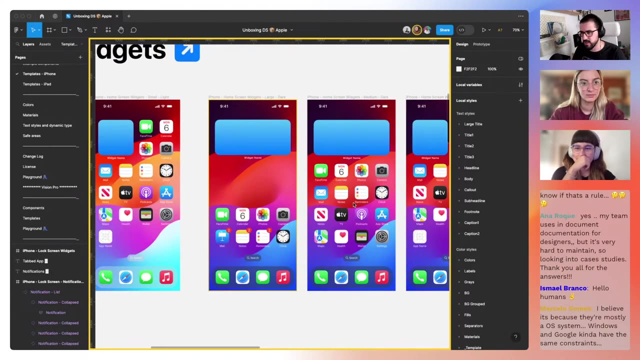 more examples off but more easily available for us to to build with. i was actually sharing that, that video, and i remember that, for example, not figma, but there's this company, i think, called bezel that has like a figma-like tool, but to design for these. let me see if i can find them while you guys. 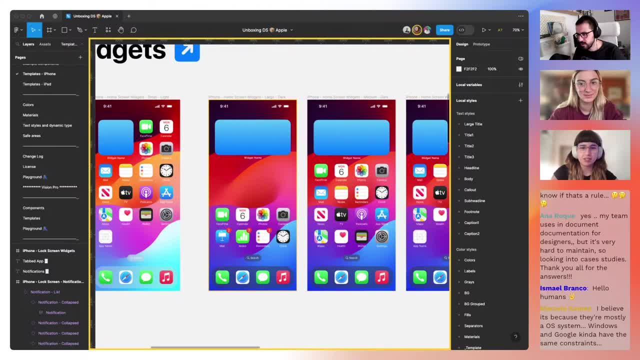 are going around. this is so cool. i'm sorry, i'm just having fun. just personalizing a home page- i'm not sure for who is this- is, uh, you know, suitable, but you can even put a badge of the notification. it's insane, and it's very quickly to change the icon and if you want the name or whatnot, 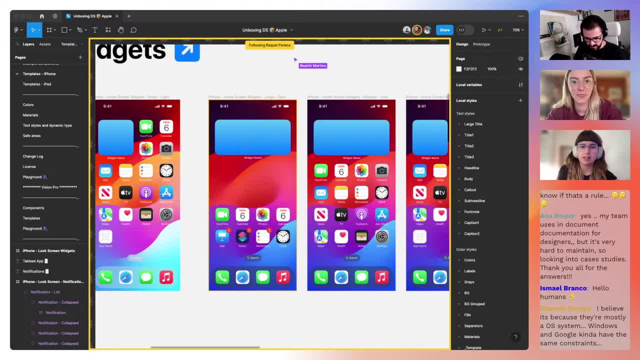 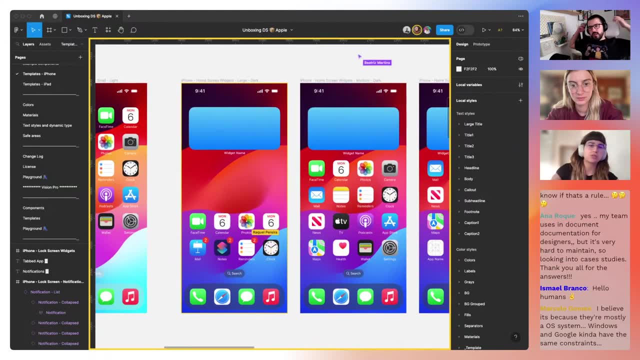 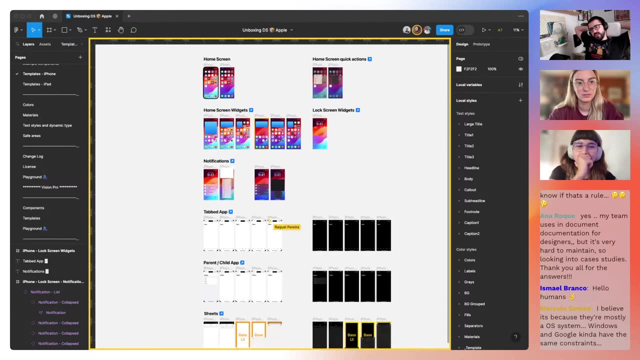 but i'm just guessing again to whom these templates are for us to entertain. or it really someone will like use their application here and try to show their bosses like, look our application, look like this here, perhaps right, not sure. yeah, if you think about it, i would say for starters you can't do that, that you just did like, if you have a 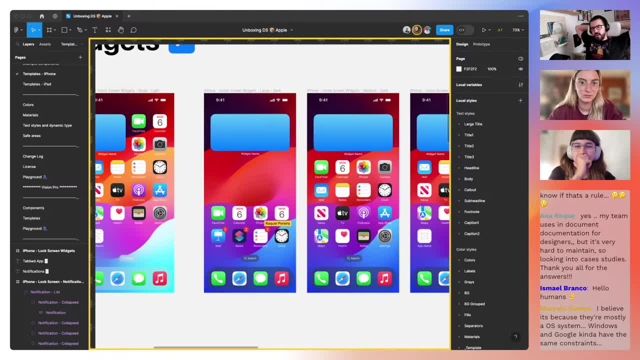 widget like that, all the apps will go up automatically, so not having the outer layout, it's already breaking things, just yeah. but in any case, like, if you look at that, if you look at the way that, um, these tools are here built, like, how many of us and i work in brands, so bear with me. 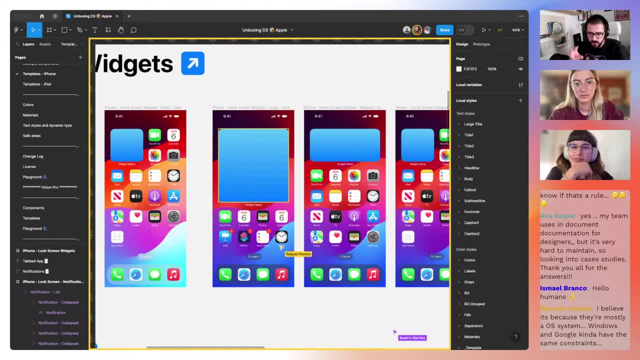 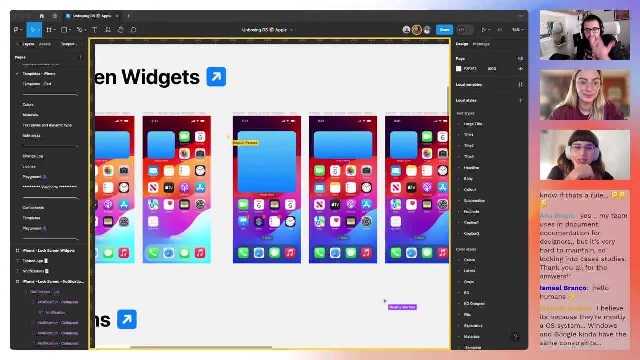 but how many people have never like just picked one of these to put their little app icon when they created the new app? yeah, that's the thing, right. this is, at least you don't spare any more time on it. it's not bad, for example, for the people that have widgets in their apps, right. 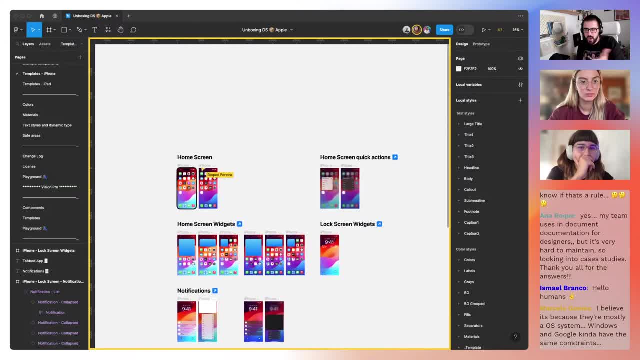 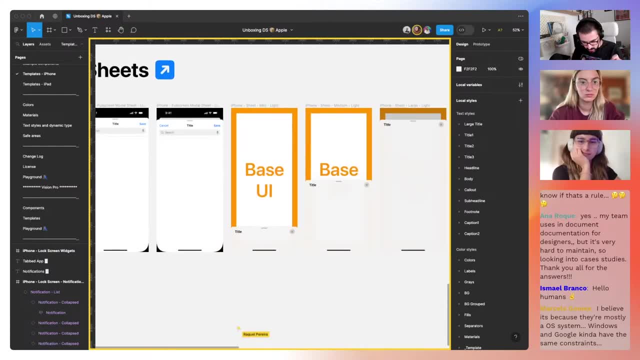 for them to build their widgets and play with them and test them in the context of how they would be used. um, by the way, i'm gonna share a link on the chat and i'm gonna share my screen now, because i found these guys the other day kind of feels like they are using the same tools as figma in. 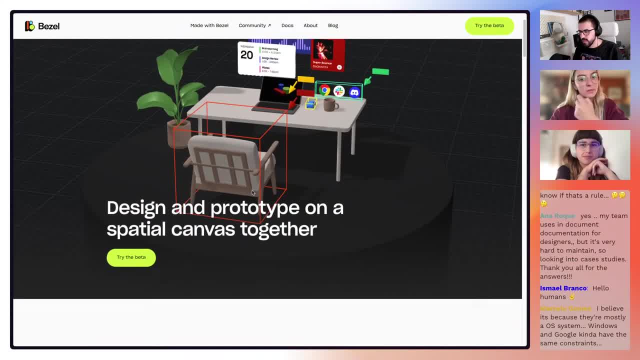 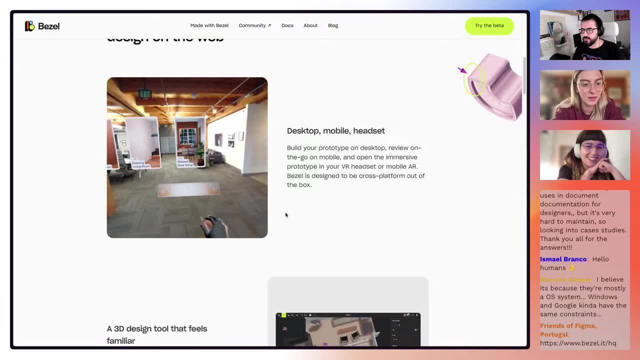 terms of like collaboration, where it's like designing for spatial canvas. oh, that's good. the moment that apple created vision os, these guys already had like everything ready for you to play around and design like this- so cool. so it's it's super interesting because it allows us to 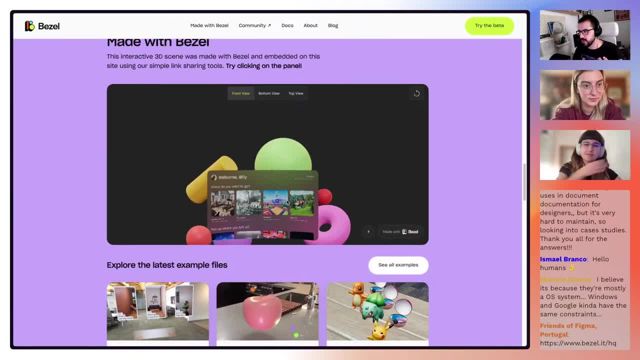 play or play with these things and design and test them out. uh, yeah, for example, this is actually a demo. oh, so cute that we can use it for, like, a demo or something like that. so, yeah, i think it's a good way to do that. yeah, i think it's a good way to do that. yeah, i think it's a good way to do that. yeah, 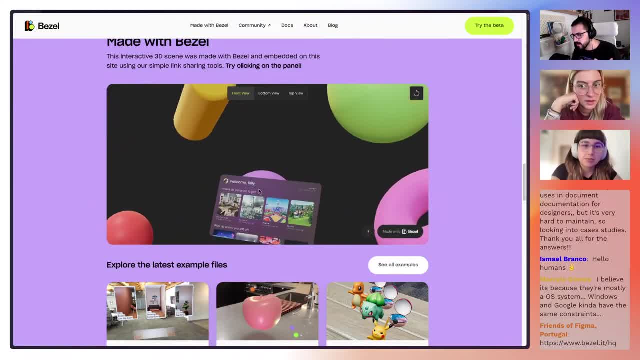 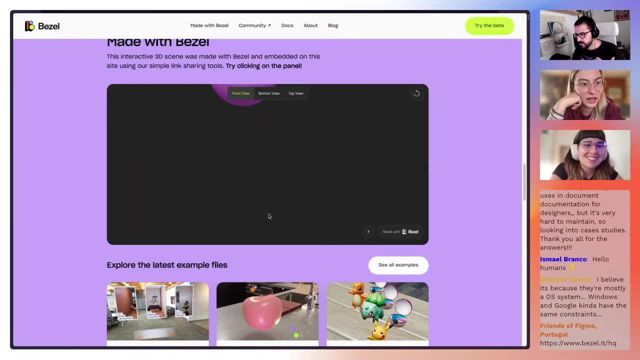 you can kind of just probably from our templates, huh, perhaps, and you can basically see how this could work. i don't know. it's so cool. it looks a lot like apples, actually like the, the. yeah, the background blurs and all of that, but then it gives you the thing that we are not being. let me see if. 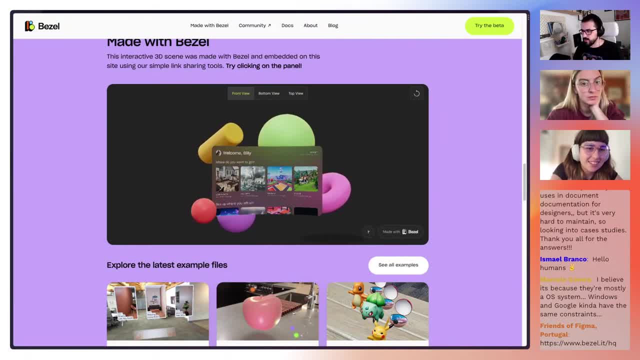 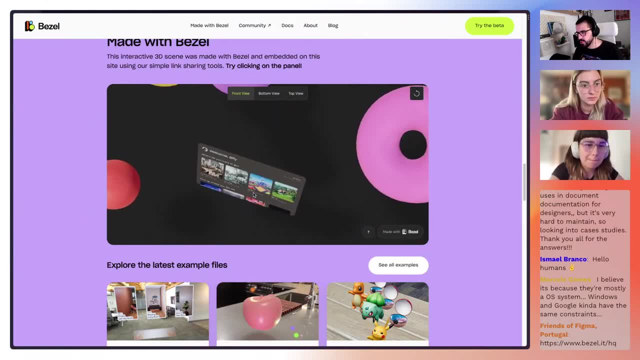 i can click here the thing that we're not seeing with figma, which is again what i was saying, like what i was trying to do with the, the, even the figma file thingy. just you're trying to showcase the, the, the way that, like, these things are gonna get a little bit of disruption, right like you're. 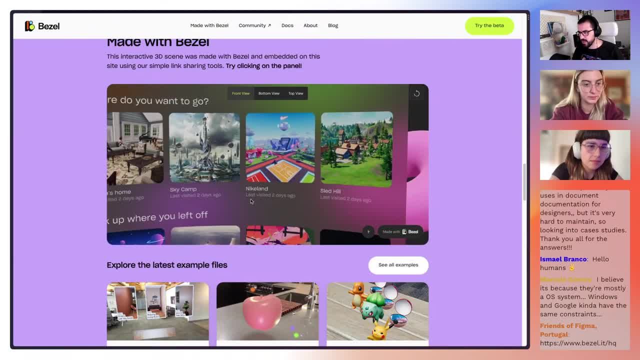 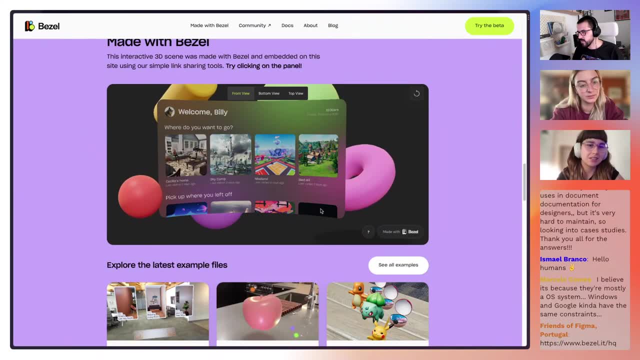 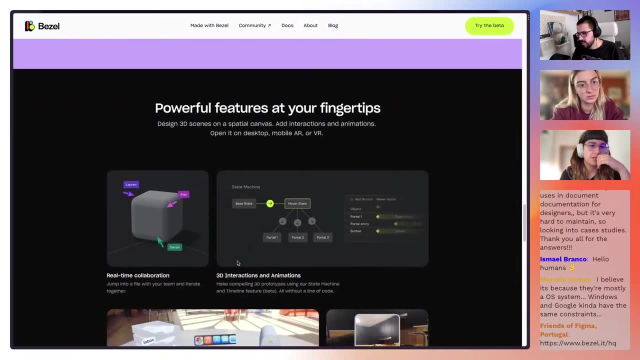 gonna see things that are art because of the way that these windows open and things angle. oh, it's clickable. that's why it was going away. um, oh, okay, and i don't know. i don't think i can like scroll in and anything, but like i can probably at least interact a little bit with it. but it's fun to see. 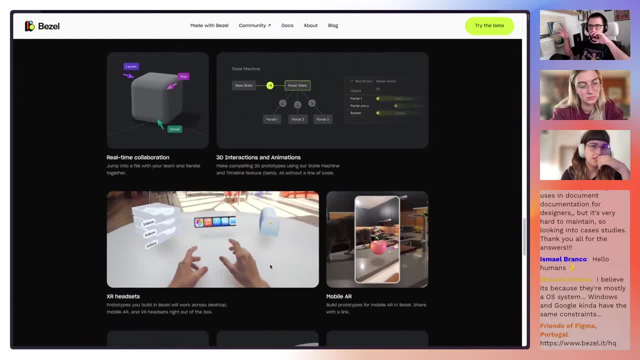 like this is also going to bring us into a new era of design in the way that we're thinking about spaces in the way that we're thinking about spaces in the way that we're thinking about spaces in the in the design like. it doesn't mean that apple will be the only one that's doing this, of course, 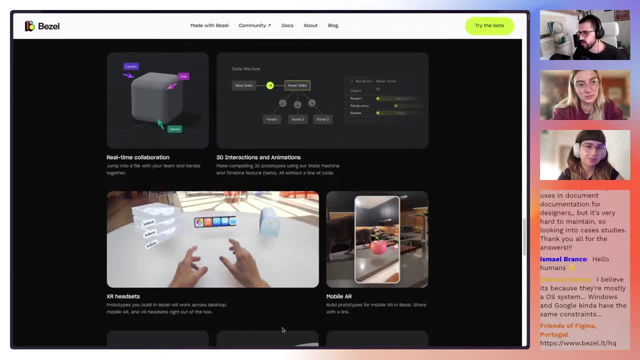 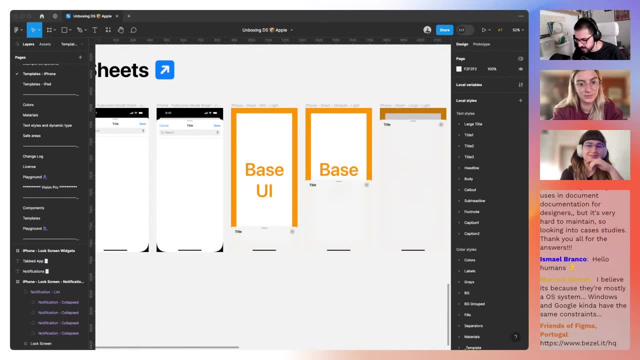 we talked about this in the past. yeah, there's a bunch of age uh vr headsets and things like that. but yeah, guys, it's like three minutes to closing of the stream because we can't keep people here for so long. sorry, everyone, just kidding, just kidding, just kidding. i know you guys love us. 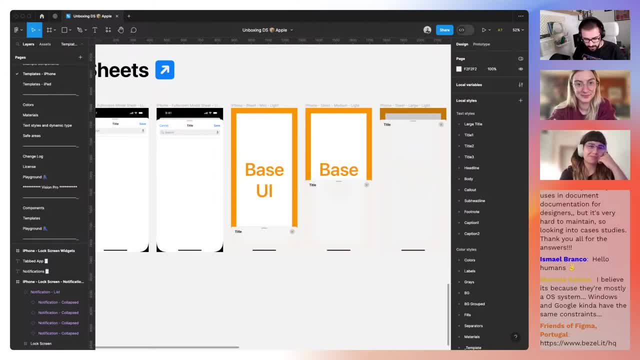 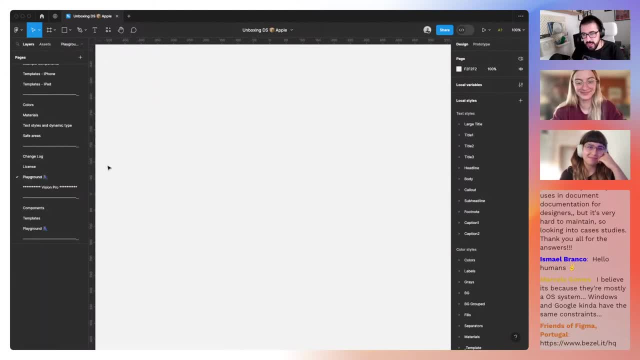 um, but yeah, i think we can probably call it a day because, let's, let's be honest. um, but yeah, i think we can probably call it a day because, let's, let's be honest. um, we've been here for a while. we played around with things we managed to create. 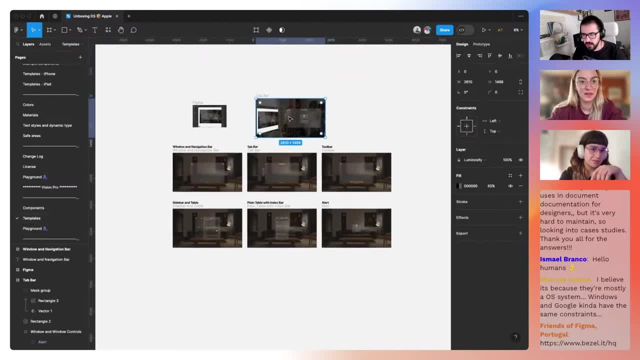 we've been here for a while. we played around with things we managed to create. we've been here for a while we played around with things we managed to create. where is it? where is it? where is it? it's uh, yeah, yeah, there you go somewhere. it's uh, yeah, yeah, there you go somewhere. 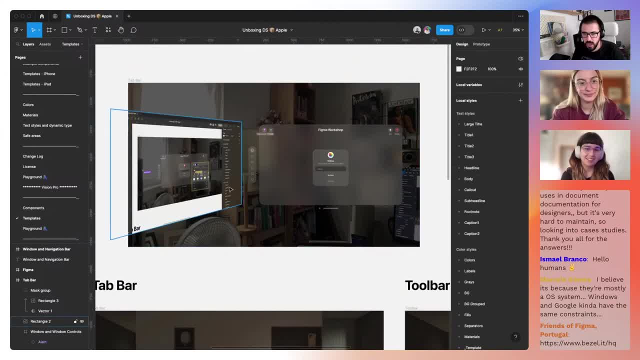 it's: uh, yeah, yeah, there you go somewhere, you managed to create something, doesn't you managed to create something, doesn't you managed to create something? doesn't mean that we created something amazing. mean that we created something amazing. mean that we created something amazing, and i even ignored the whole thing, and 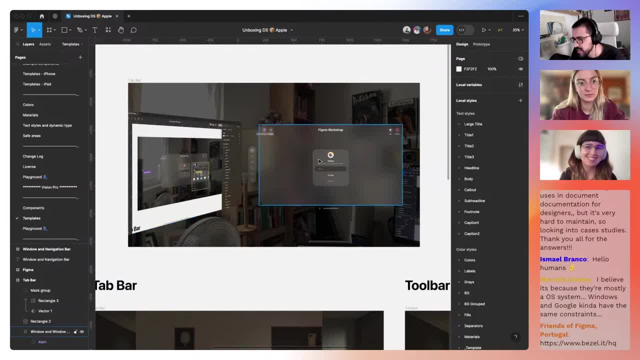 and i even ignored the whole thing, and and i even ignored the whole thing and just played around with the mock-up, just played around with the mock-up, just played around with the mock-up, which, which which. yeah, i've done it, uh, but in any case, yeah, i've done it, uh, but in any case. 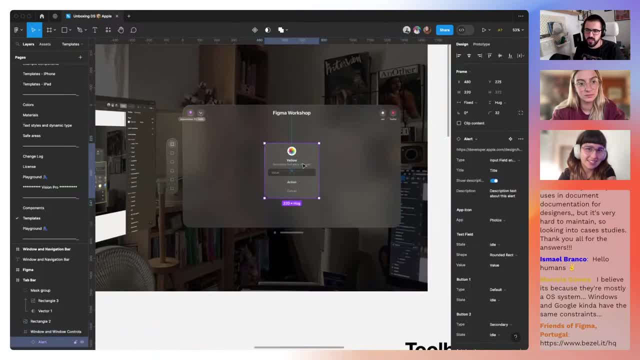 yeah, i've done it, uh, but in any case, in any case, like i think that, in any case, like i think that, in any case, like i think that what this tells us about the systems, that, what this tells us about the systems, that what this tells us about the systems that apple is putting out into the world, 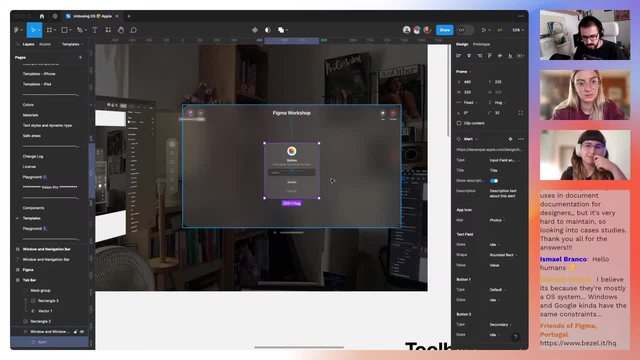 apple is putting out into the world. apple is putting out into the world like it literally is. like it literally is like it literally is the design system for them, like marcelo. the design system for them, like marcelo. the design system for them, like marcelo was saying that he believes that. 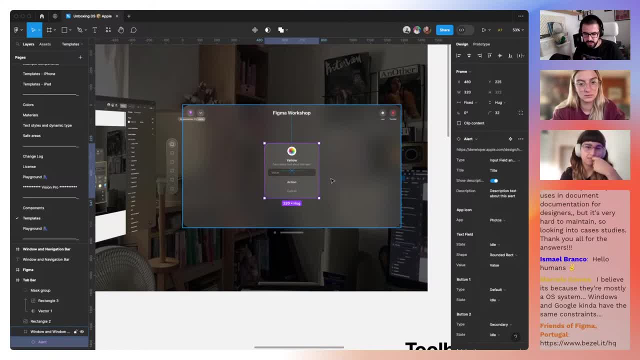 was saying that he believes that was saying that he believes that what happens with these systems is they. what happens with these systems is they. what happens with these systems is they are an operating system, are an operating system, are an operating system system, and that's why they are so close. 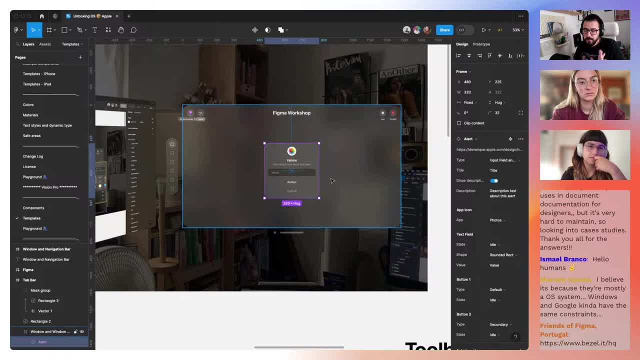 system and that's why they are so close system, and that's why they are so close that they don't allow us to do much, that they don't allow us to do much, that they don't allow us to do much with it. but in fact, it's like you can. 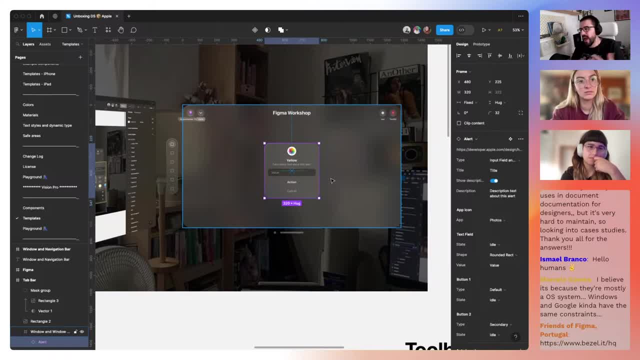 with it, but in fact it's like you can with it, but in fact it's like you can use these, use these, use these and then use visuals or color, and you and then use visuals or color, and you and then use visuals or color, and you have your own app, which is what apple has. 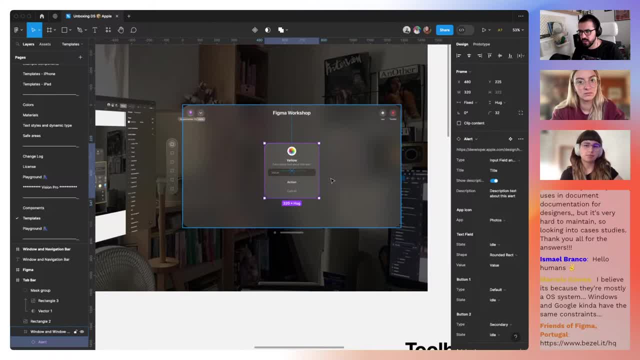 have your own app, which is what apple has. have your own app, which is what apple has always done with their own like, always done with their own like, always done with their own. like reality, like the- the thing that the reality like the. the thing that the reality like the. the thing that the things that they build, they always push. 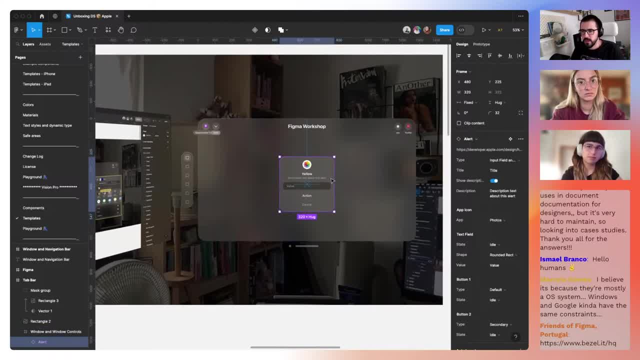 things that they build. they always push things that they build. they always push for people to do, for people to do, for people to do, kind of that like so it's like if you kind of that like, so, it's like if you kind of that like, so, it's like if you need to. 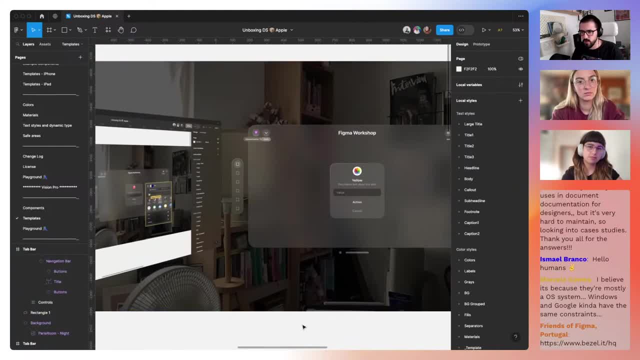 need to need to that first level app. maybe this will that first level app, maybe this will that first level app. maybe this will tell you how that app could work, or tell you how that app could work, or tell you how that app could work, or maybe this will allow you to test how. 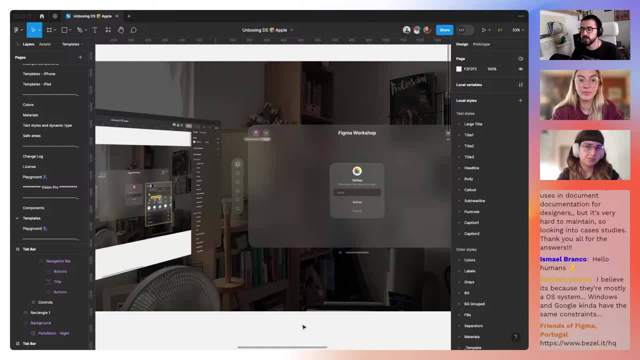 maybe this will allow you to test how. maybe this will allow you to test how that app would that app would that app would feel into the apple ecosystem, right? so feel into the apple ecosystem, right. so feel into the apple ecosystem, right. so i feel like that's more of the use case. 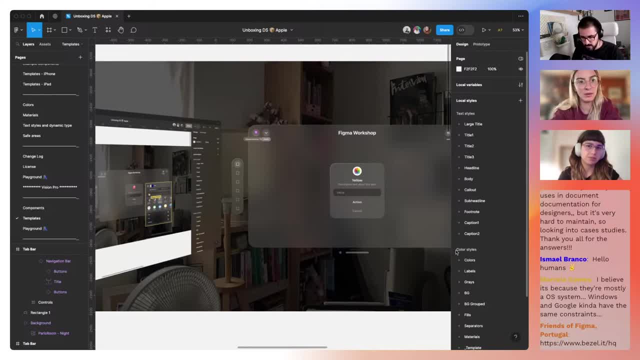 i feel like that's more of the use case. i feel like that's more of the use case here, here, here. uh, yeah, that was actually what happened. uh, yeah, that was actually what happened. uh, yeah, that was actually what happened with instagram at first. instagram was with instagram. at first, instagram was. 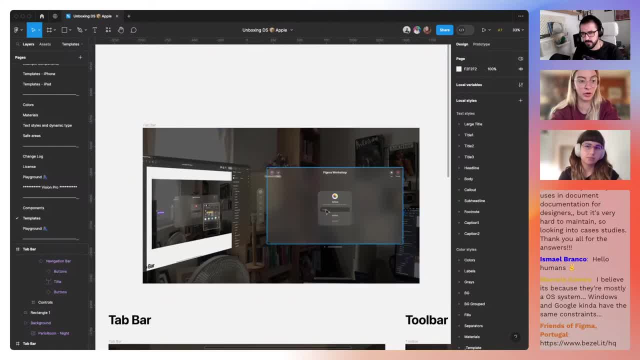 with instagram. at first, instagram was only only only um an apple devices platform, um an apple devices platform, um an apple devices platform. and then, years later, they released. and then years later, they released, and then years later, they released: uh, the app for android. uh, the app for android. 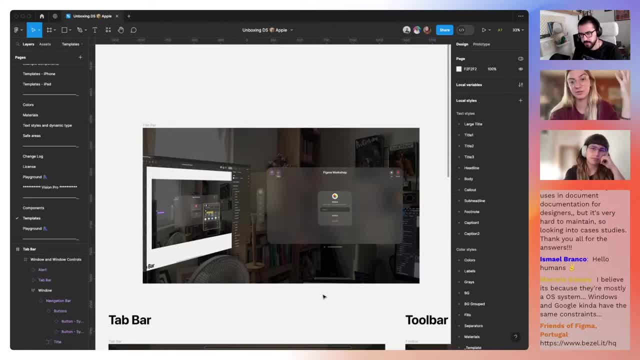 uh, the app for android? yeah, yeah, i mean, of course we're not. yeah, yeah, i mean of course we're not. yeah, yeah, i mean of course we're not talking about like design systems, talking about like design systems, talking about like design systems, because maybe we didn't really talk. 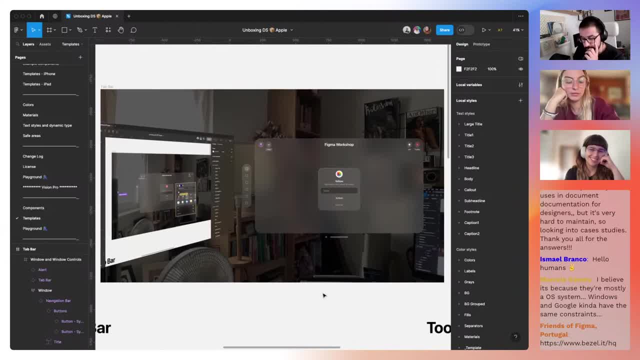 because maybe we didn't really talk, because maybe we didn't really talk about that, about that, about that at that time. yeah, back then, yeah at that time. yeah, back then. yeah at that time. yeah, back then. yeah, but it is, but it is, but it is, and it's not just that right like it's. 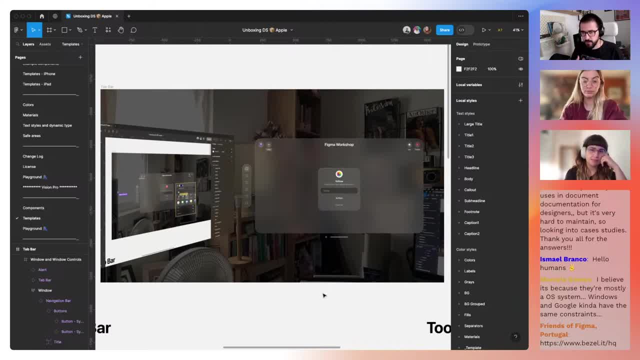 and it's not just that right like it's, and it's not just that right like it's the thing that, the thing that the thing that ecosystem wise, and this was what was said ecosystem wise, and this was what was said ecosystem wise and this was what was said before. 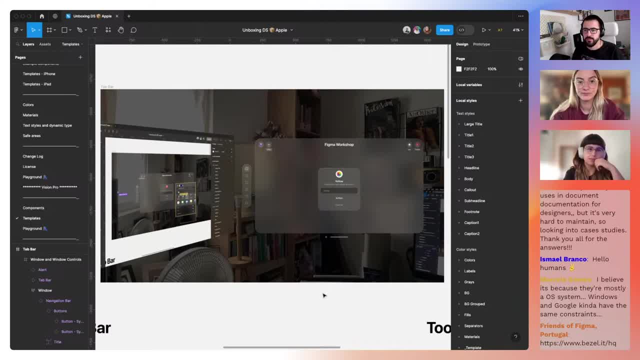 before before. apple makes it very easy for people to apple. makes it very easy for people to apple. makes it very easy for people to build apps, build apps, build apps. um, yeah, their languages and everything, the um, yeah, their languages and everything, the um, yeah, their languages and everything the investment that they have on things like 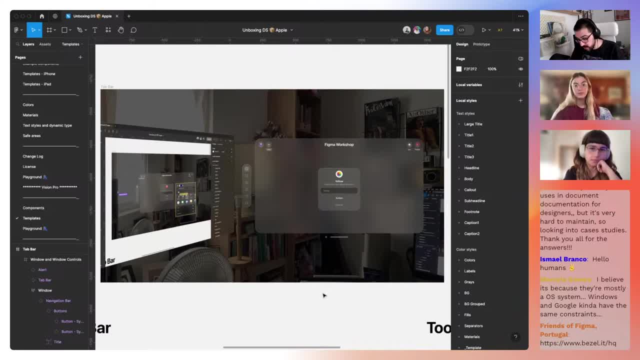 um, yeah, their languages and everything the investment that they have on things like um, yeah, their languages and everything the investment that they have on things like um, um, um, like swift, which is a very simple, like swift, which is a very simple, like swift, which is a very simple programming language. 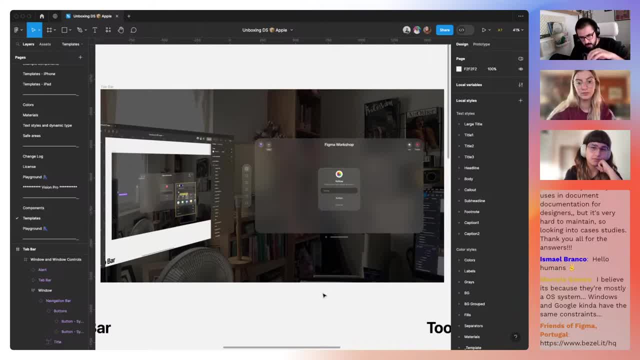 programming language. programming language, of course, that eventually creates an end, of course that eventually creates an end, of course, that eventually creates an end result which is result, which is result, which is being somewhat easy to build, things like being somewhat easy to build, things like being somewhat easy to build, things like this right, like being somewhat easy to 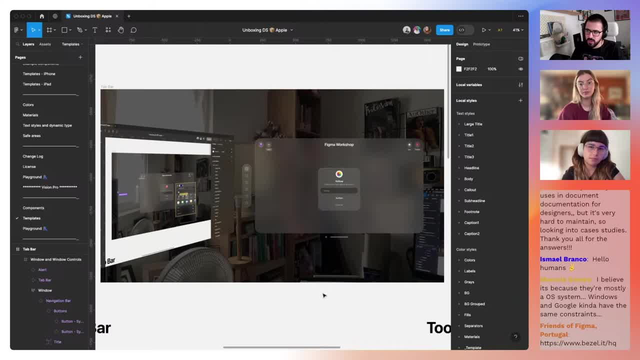 this right like being somewhat easy to this right like being somewhat easy to start and start and start and and create things like their language, and create things like their language. and create things like their language and build something that comes out of, and build something that comes out of. 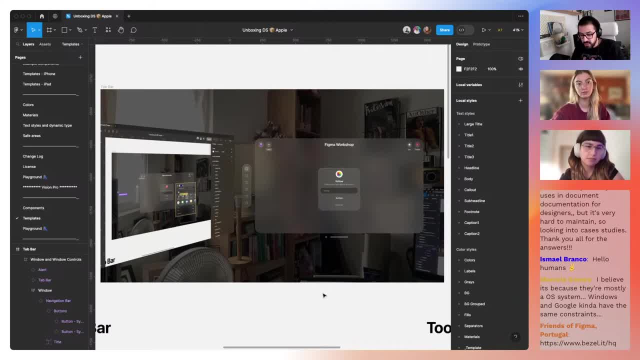 and build something that comes out of apple's, that feels like it comes out of apple's, that feels like it comes out of apple's, that feels like it comes out of apple's ecosystem. so apple's ecosystem, so apple's ecosystem. so their design system and their figma files. their design system and their figma files. their design system and their figma files. feel like they are doing the same for us. feel like they are doing the same for us. feel like they are doing the same for us, which is cool, like right, we can play. 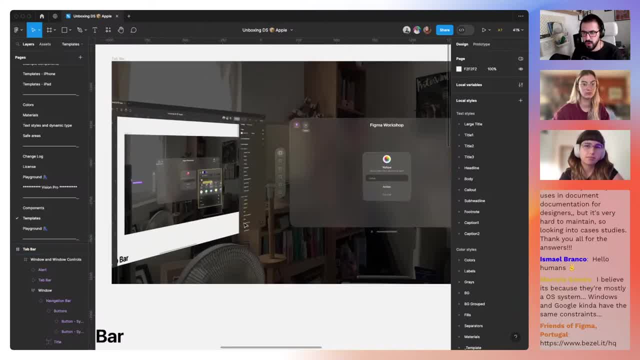 which is cool like right, we can play. which is cool like right, we can play around and we can around and we can around and we can create this idea and play around with create this idea and play around with create this idea and play around with the concepts of. 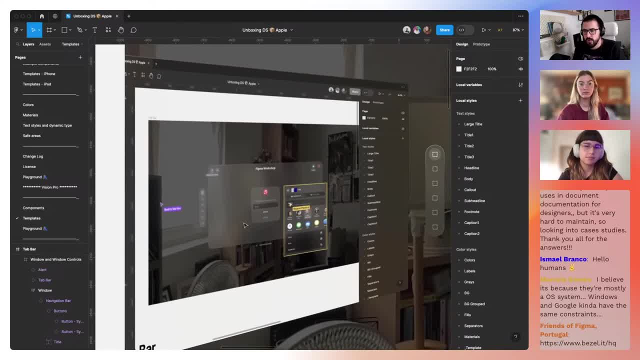 the concepts of the concepts of how we would build for the systems, or how, how we would build for the systems, or how how we would build for the systems, or how we would migrate stuff like figma. for we would migrate stuff like figma, for we would migrate stuff like figma, for example, into the systems and see how. 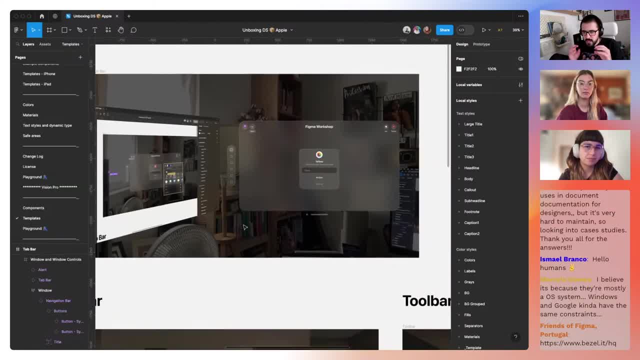 example, into the systems and see how example into the systems and see how they work, and it's fun to do that, but they work and it's fun to do that, but they work and it's fun to do that. but again, again, again, it's, it's, it's almost like the same thing. it's, it's, it's, it's almost like the same thing. it's, it's, it's, it's almost like the same thing that we were talking about on the, that we were talking about on the, that we were talking about on the documentation on their website, right, if? 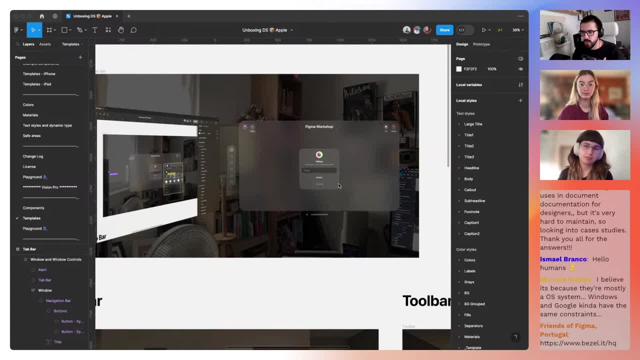 documentation on their website right. if documentation on their website right. if we look at the documentation on their. we look at the documentation on their. we look at the documentation on their website, the fact that they are so much website, the fact that they are so much website, the fact that they are so much focused on. 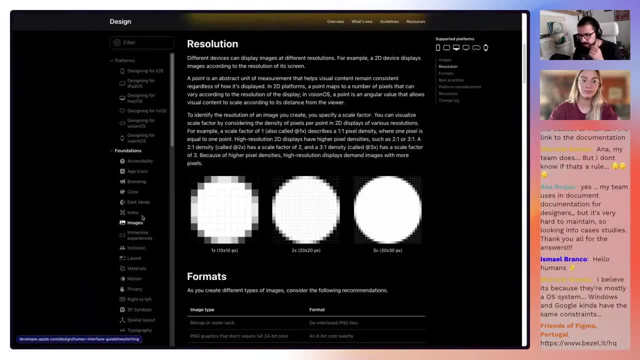 focused on, focused on foundations and things like that. um, foundations and things like that. um, foundations and things like that. um, making sure that people understand that. making sure that people understand that, making sure that people understand that they are designing, they are designing, they are designing four specific goals with- yeah, certain. 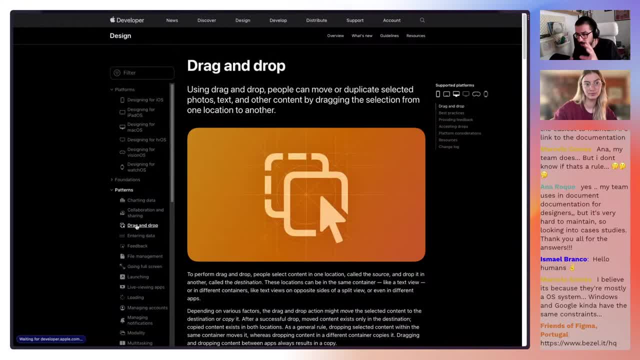 four specific goals with, yeah, certain four specific goals with, yeah, certain things, things, things on their line and with certain patterns on their line and with certain patterns on their line and with certain patterns that already work like apple, that already work like apple, that already work like apple products and people would not have 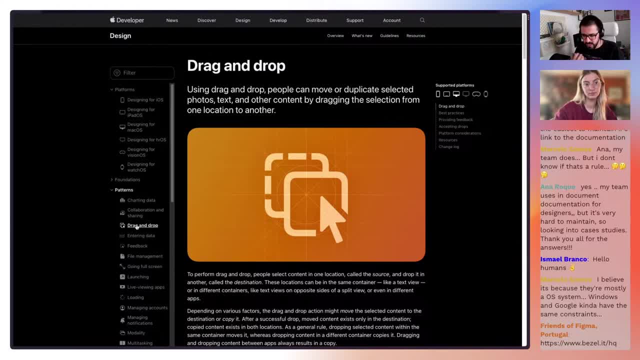 products and people would not have products and people would not have difficulties with it. difficulties with it, difficulties with it. i feel like that's that this system. i feel like that's that this system, i feel like that's that this system sells you the same thing, sells you the same thing. 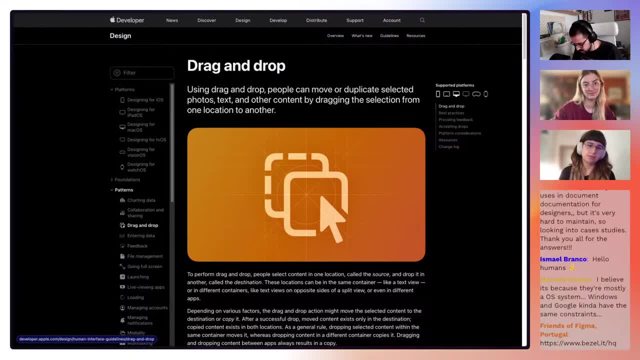 sells you the same thing. actually, yeah, just did something i i hate. actually, yeah, just did something i i hate. actually, yeah, just did something i i hate. raquel for sure for some reason. so raquel for sure for some reason. so raquel for sure, for some reason. so no worries. 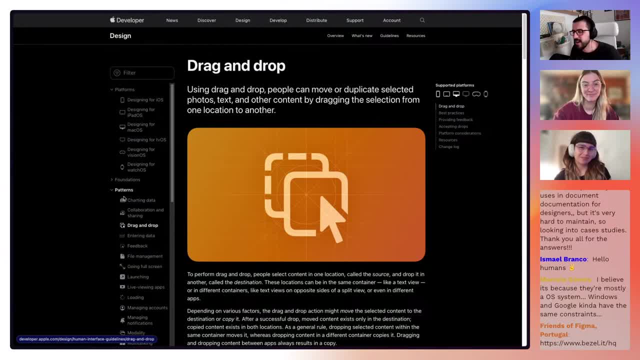 no worries, no, worries, your tablet is not running well. um, your tablet is not running well. um, your tablet is not running well, um, it's an ipad, uh, but in any case, like it's an ipad, uh, but in any case like it's an ipad, uh, but in any case, like, i feel like this works really well. 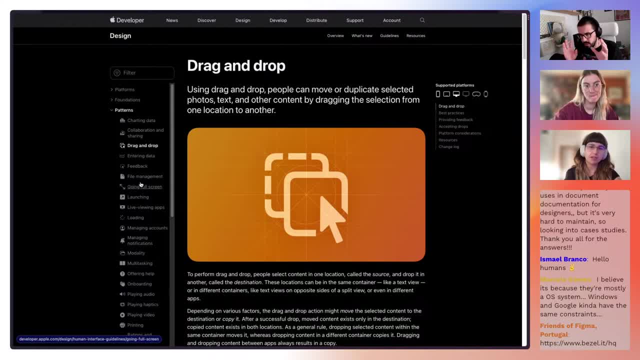 i feel like this works really well. i feel like this works really well side by side because it uses the same side by side, because it uses the same side by side, because it uses the same logic like it, logic, like it, logic like it, yeah, makes you focus on patterns, on. 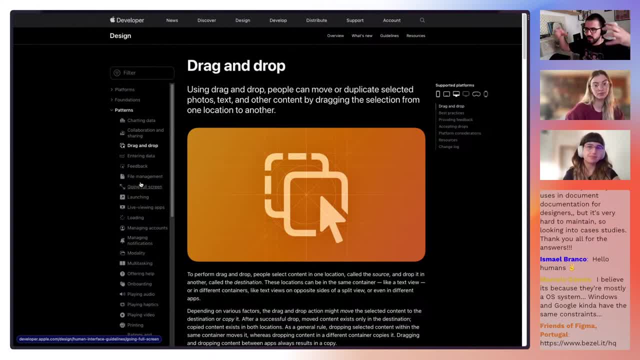 yeah makes you focus on patterns on yeah, makes you focus on patterns on yeah building fast, and then the yeah building fast, and then the yeah building fast, and then the personalization, the components, the personalization, the components, the personalization, the components: the things that we usually 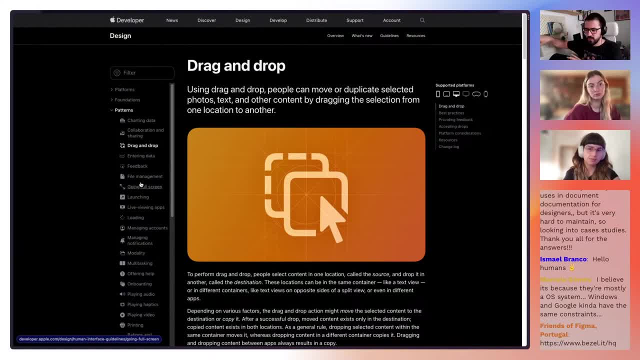 things that we usually things that we usually think about having fun are a second think about having fun are a second think about having fun are a second level and they come at the end of the level and they come at the end of the level and they come at the end of the world and you can actually like 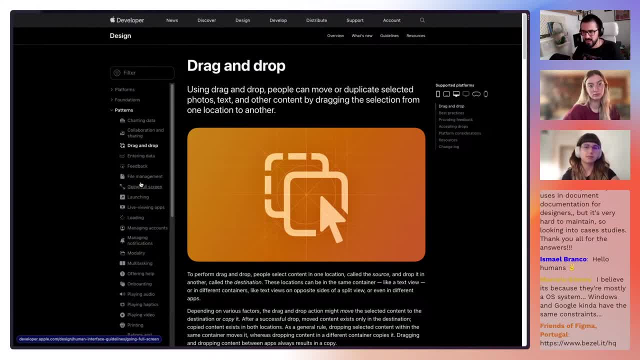 world and you can actually like world and you can actually like, then extend and build and change, and do, then extend and build and change, and do, then extend and build and change and do your systems, your systems, your systems. i think that's interesting. yeah, for sure. i think that's interesting, yeah, for sure. 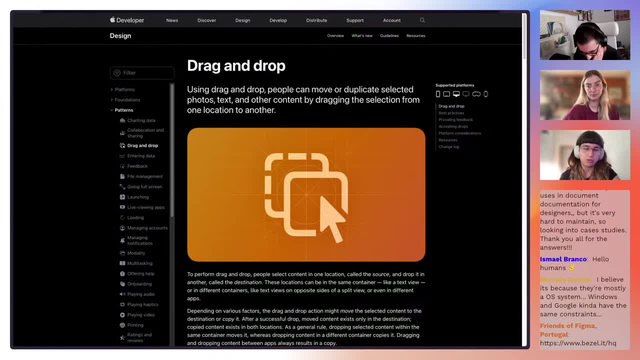 i think that's interesting. yeah, for sure. just like to add that, maybe figma. just like to add that, maybe figma. just like to add that, maybe figma. although that, although that, although that just launched new features, the next one just launched new features, the next one. 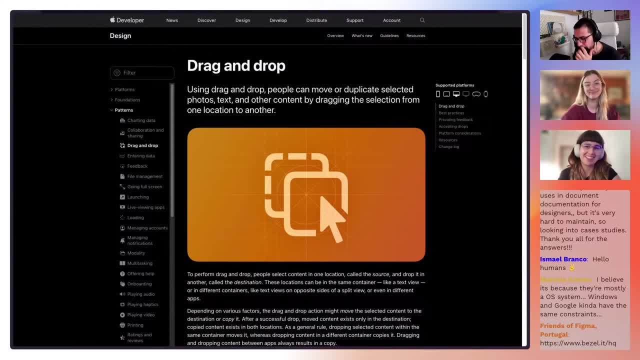 just launched new features. the next one could be prototyped for special design. could be prototyped for special design. could be prototyped for special design. there's no pressure, i'm gonna, i'm gonna. there's no pressure, i'm gonna, i'm gonna. 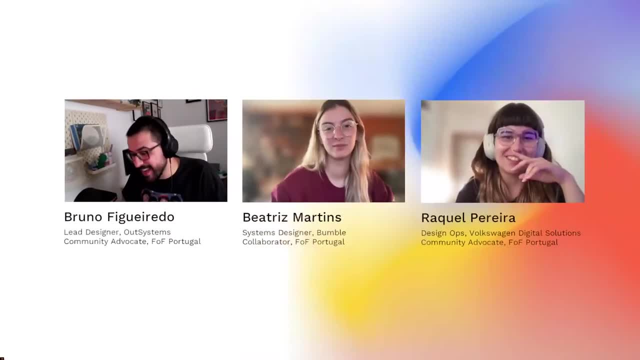 there's no pressure. i'm gonna. i'm gonna be fully honest. i don't think that. be fully honest. i don't think that, be fully honest. i don't think that should be a priority. should be a priority, should be a priority, just saying yeah, i don't think that it. 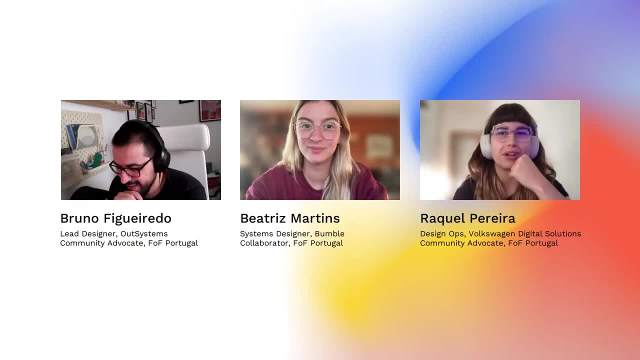 just saying, yeah, i don't think that it should be a priority, but yeah, or maybe partner it up with should be a priority, but yeah, or maybe partner it up with should be a priority, but yeah, or maybe partner it up with someone. perhaps that, maybe someone, perhaps that maybe. 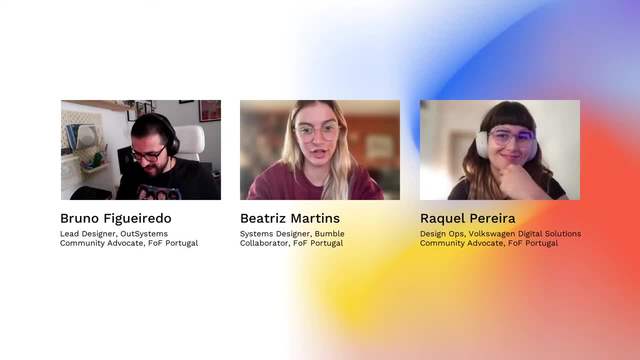 someone, perhaps that maybe there's a bunch of people doing things. there's a bunch of people doing things. there's a bunch of people doing things happy if we have linear gradients and happy if we have linear gradients and happy if we have linear gradients and typography variables. i mean, i don't. 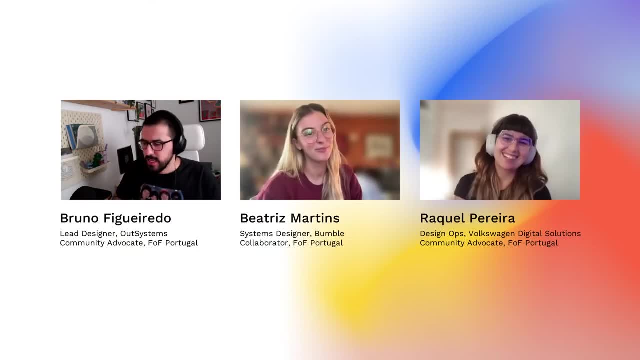 typography variables. i mean i don't typography variables, i mean i don't need anything else. yeah, yeah, need anything else. yeah, yeah, need anything else, yeah, yeah. so yeah, let's see until the end of the. so, yeah, let's see until the end of the. so, yeah, let's see until the end of the year variables are supposed to also have. 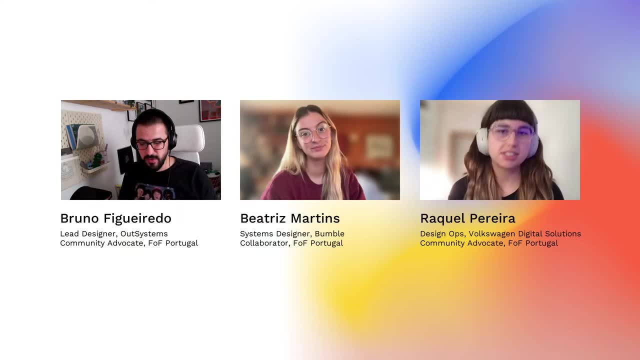 year variables are supposed to also have year variables are supposed to also have uh, the typography and image ones on uh the typography and image ones on uh the typography and image ones on variables, variables, variables, gradients, i don't think i i think that gradients, i don't think i, i think that. 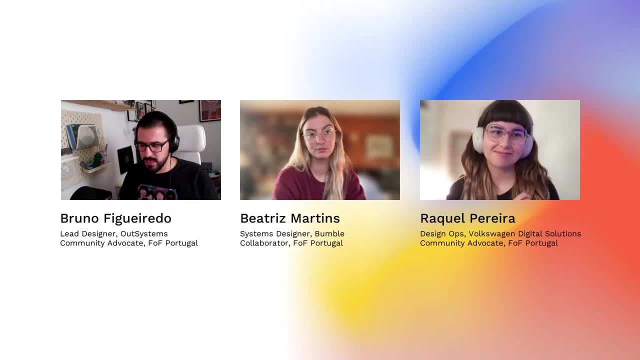 gradients? i don't think i i think that gradients need to be built with variables. gradients need to be built with variables. gradients need to be built with variables in the sense that they build the system, in the sense that they build the system, in the sense that they build the system right, like. 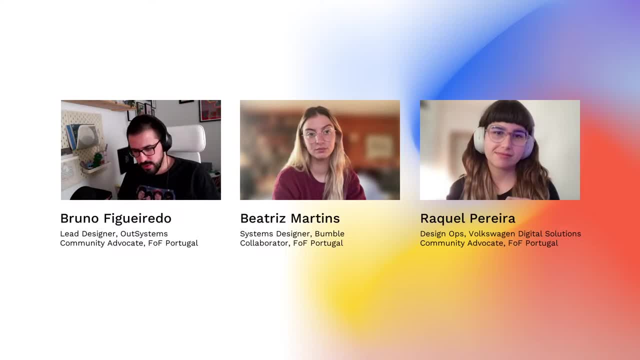 right, like, right, like. variables are um single use. variables are um single use. variables are um single use uh tokens kind of thing like it's one uh tokens kind of thing, like it's one uh tokens kind of thing like it's one value, value, value. so maybe a com, a second level value. 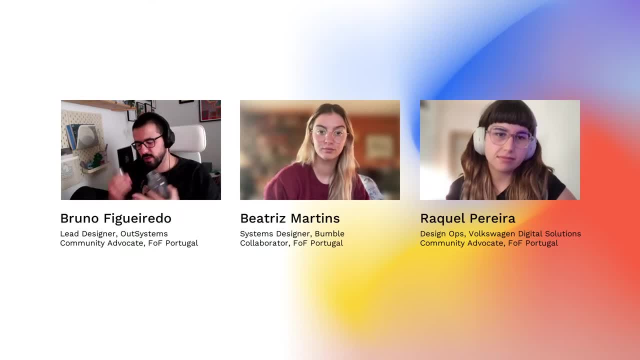 so maybe a com, a second level value. so maybe a com, a second level value thing, like where you have two tokens thing. like where you have two tokens thing. like where you have two tokens for the individual values and then the for the individual values and then the. 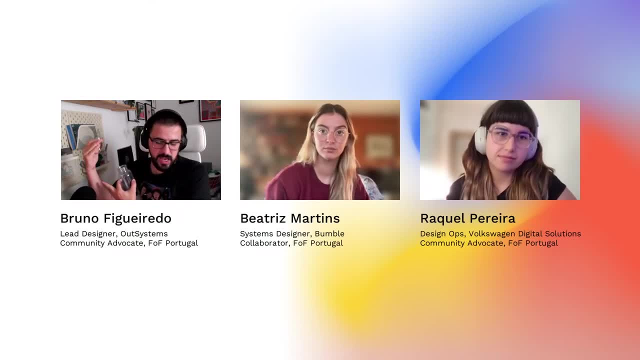 for the individual values and then the gradient is a composite of two tokens. gradient is a composite of two tokens. gradient is a composite of two tokens. that might make sense. that might make sense. that might make sense. i don't know the we still need to see how. 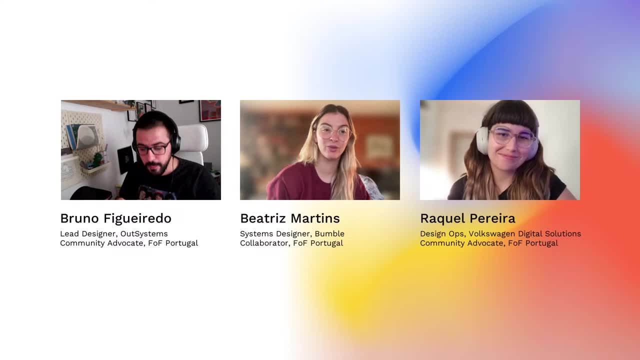 i don't know the. we still need to see how. i don't know the. we still need to see how that system's evolved, that system's evolved, that system's evolved. so, yeah, yeah, but we'll never so. yeah, yeah, but we'll never so. yeah, yeah, but we'll never be without a job. yeah, yeah, yeah, it's. 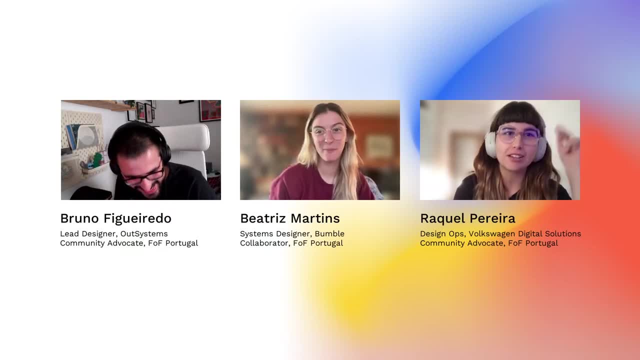 be without a job, yeah, yeah, yeah, it's be without a job, yeah, yeah, yeah, it's always a work in progress, like always a work in progress, like always a work in progress. like yeah, and then on the backlog: oh new, yeah, and then on the backlog: oh new. 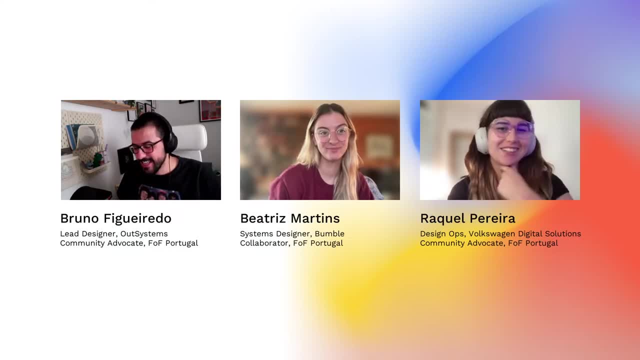 yeah. and then on the backlog, oh, new features on figma. yeah, there you go, okay. features on figma. yeah, there you go, okay. features on figma: yeah, there you go, okay. okay, guys, just to finish things up. okay, guys, just to finish things up. okay, guys, just to finish things up really fast, just reminding everyone. 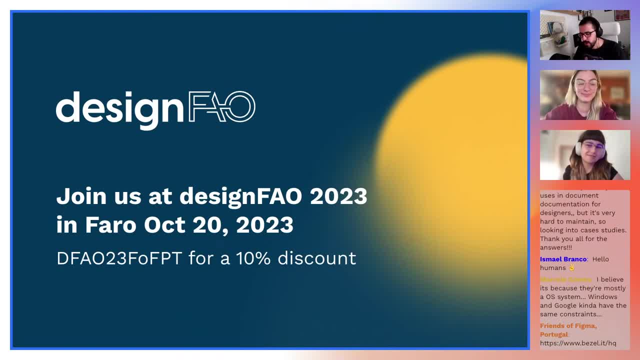 really fast, just reminding everyone, really fast, just reminding everyone. don't forget to uh register for design. don't forget to uh register for design. don't forget to uh register for design. fao- we have a 10 discount, you can come. fao- we have a 10 discount, you can come. 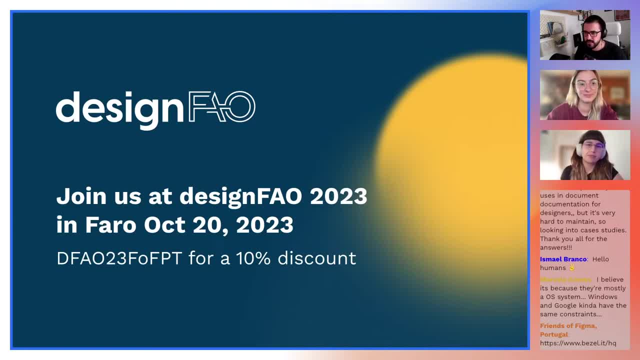 fao, we have a 10 discount. you can come through friendsfigmacom to get it, through friendsfigmacom to get it, through friendsfigmacom to get it. uh, it's uh easy and i'm gonna be honest. uh, it's uh easy and i'm gonna be honest. 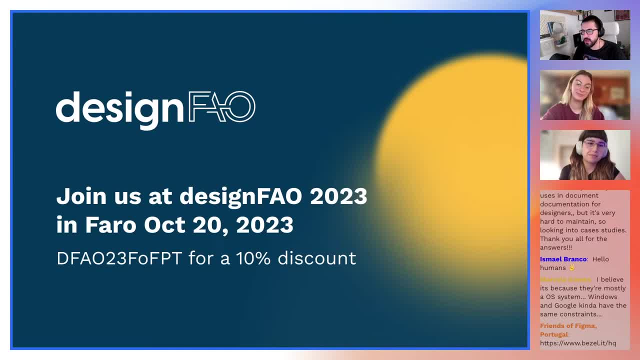 uh, it's uh easy and i'm gonna be honest. it's an amazing conference. it's an. it's an amazing conference. it's an. it's an amazing conference. it's an amazing lineup of speakers. you're not amazing lineup of speakers. you're not amazing lineup of speakers. you're not gonna regret it. i'm just gonna drop the. 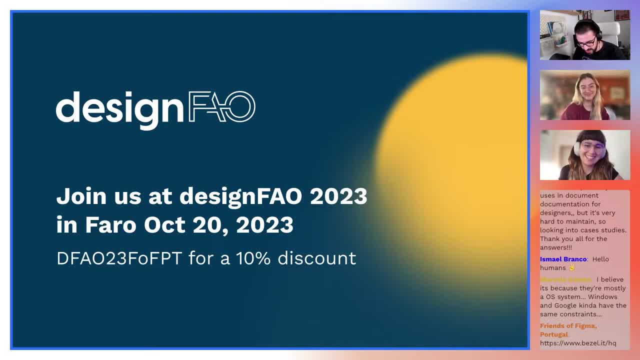 gonna regret it. i'm just gonna drop the gonna regret it. i'm just gonna drop the link here and my cat is getting really link here and my cat is getting really link here and my cat is getting really really loud. so if you hear the cat on, 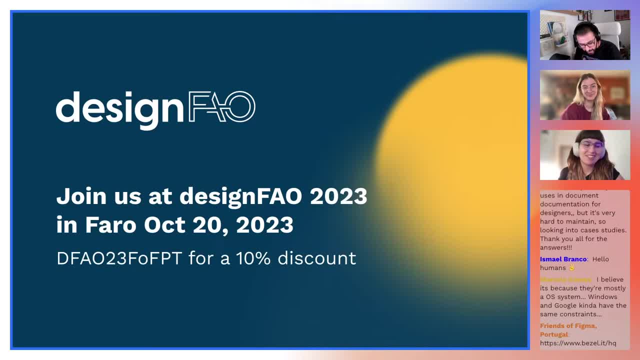 really loud. so if you hear the cat on really loud, so if you hear the cat on the background, i promise you i'm not the background. i promise you i'm not the background. i promise you i'm not torturing her. and again, no, no, we get it. 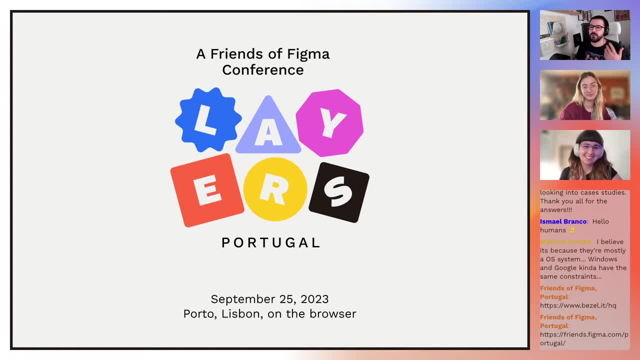 torturing her and again, no, no, we get it. torturing her and again, no, no, we get it. don't forget, we just launched our very. don't forget, we just launched our very. don't forget, we just launched our very own own own regional conference. friends of sigma. 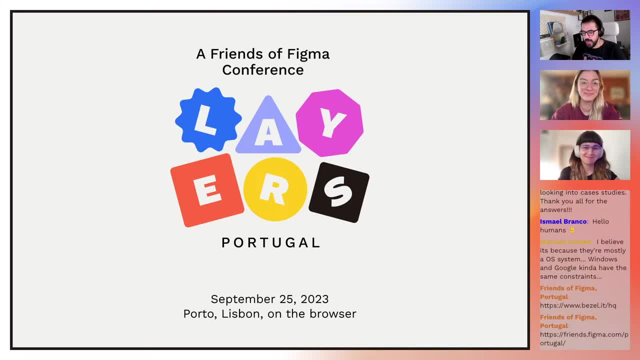 regional conference. friends of sigma regional conference. friends of sigma conference called layers that are going conference. called layers that are going conference. called layers that are going to be to be to be doing here in portugal: um, we're still doing here in portugal. um, we're still. 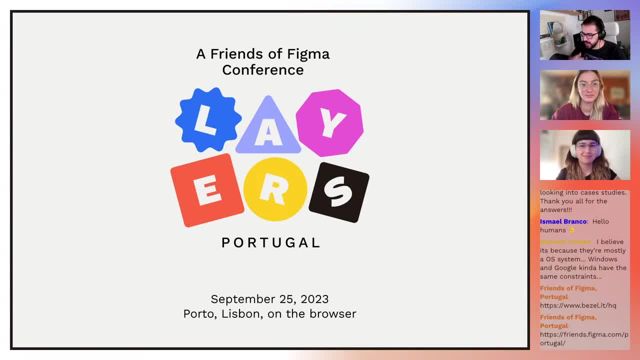 doing here in portugal? um, we're still setting it up a little bit. setting it up a little bit. setting it up a little bit. uh, we're gonna have news very soon. expect, uh, we're gonna have news very soon. expect, uh, we're gonna have news very soon. expect news coming out every week. 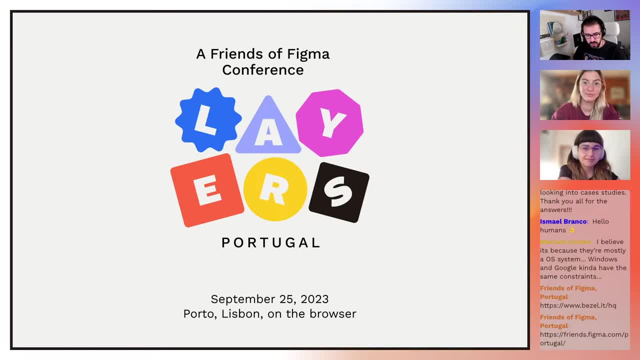 news coming out every week. news coming out every week: we have an open call for people who want. we have an open call for people who want. we have an open call for people who want to join to join, to join the conference as speakers. so, if you have, 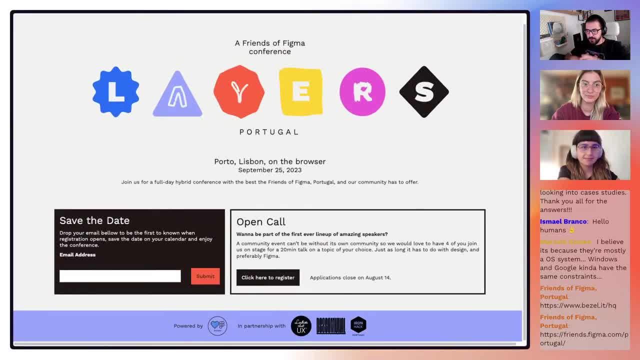 the conference as speakers. so if you have the conference as speakers, so if you have something to say, something to say, something to say, we're here for you, do not be afraid. if we're here for you, do not be afraid. if we're here for you, do not be afraid. if you're a junior, a mid-level, a senior, if you're a junior, a mid-level a senior. if you're a junior, a mid-level a senior, if you you, you think you have something that you would think, you have something that you would think, you have something that you would like to bring out into the world. we're. like to bring out into the world. we're like to bring out into the world. we're here to hear it. we're here to give you a here to hear it. we're here to give you a here to hear it. we're here to give you a stage. 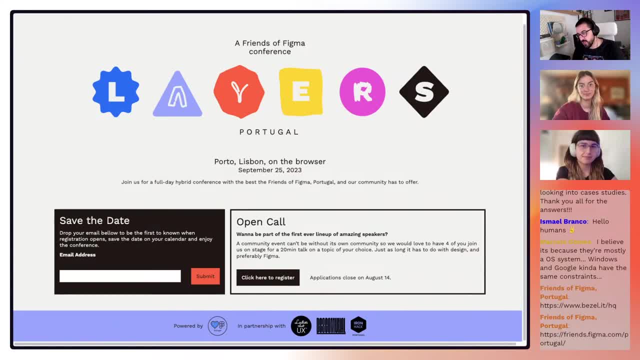 stage, stage, um. we only have four slots with small, um, we only have four slots with small um, we only have four slots with small. talks, unfortunately, but talks unfortunately, but talks, unfortunately, but four people from the community joining us, four people from the community joining us, four people from the community joining us on this like event, would be amazing. so 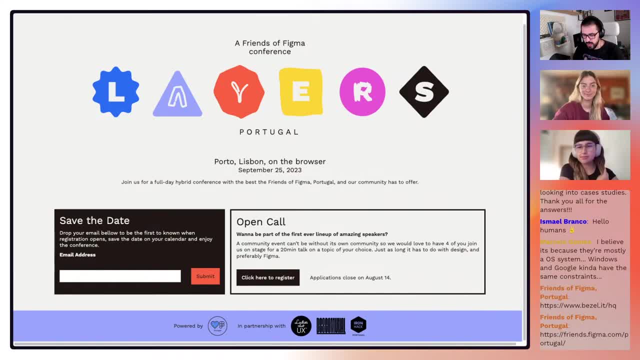 on this like event would be amazing. so on this like event would be amazing. so, if you want to, if you can, if you want to, if you can, if you want to, if you can, um do it and a huge, huge thank you to. um do it and a huge, huge thank you to.